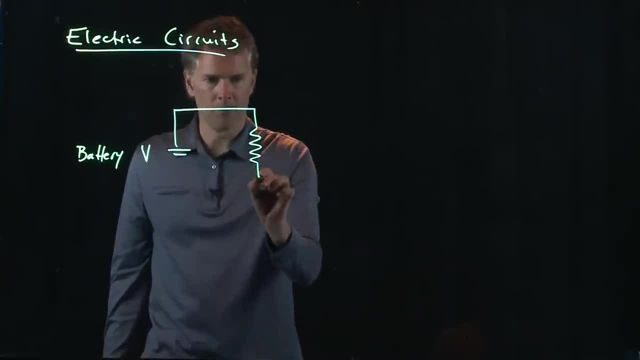 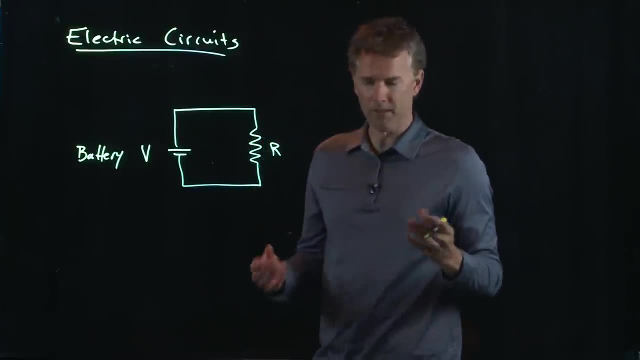 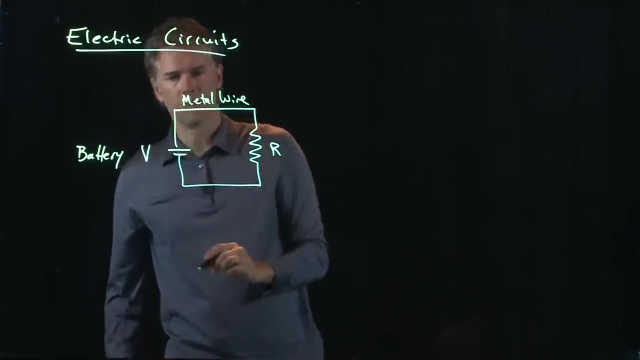 a metal wire. There is a resistor which looks like that And that makes a very simple circuit. This is the most basic circuit that you could have. This portion of the circuit is a metal wire. Everywhere you have this straight line, that's a metal wire. When we get to capacitors, we'll 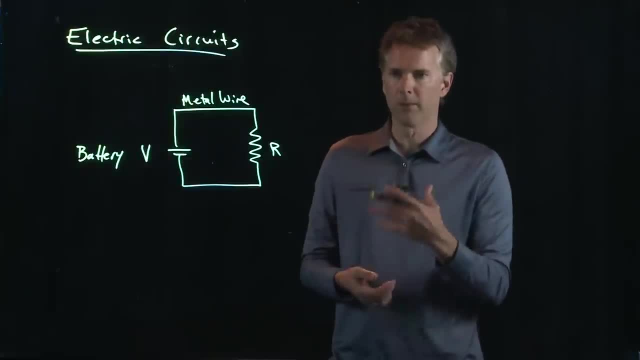 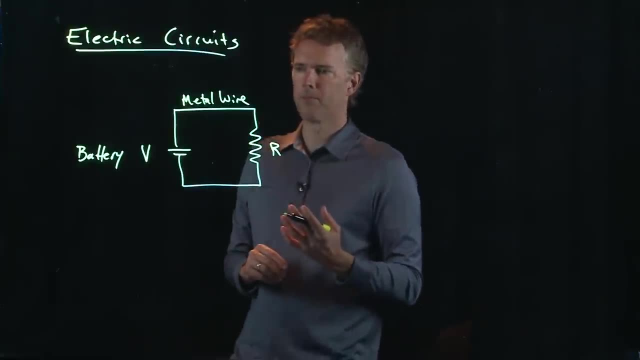 have a different circuit element. When we get to inductors we'll have a different circuit element, But for now we have two. We have a battery and we have a resistor, And they are connected by metal wires. Now, one thing that you've been working on in your labs is: 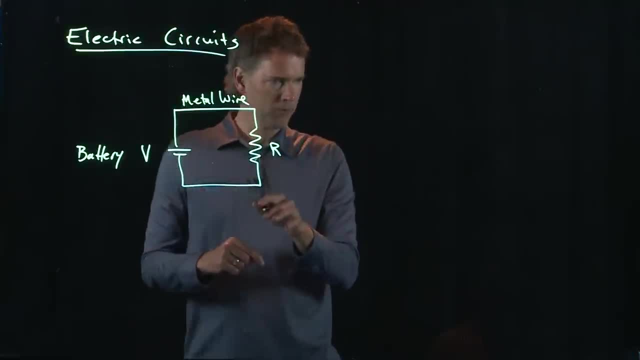 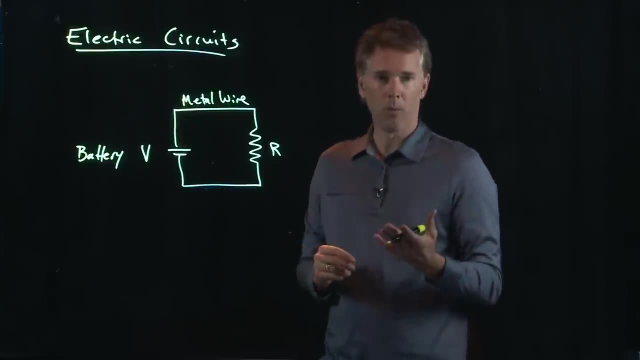 what are the voltages at different points around the circuit? And when you do that, remember about metal wires. What is a metal wire? A metal wire is a piece of metal. Literally it's a long, thin strand of metal. But, as we learned in class, metals are equipotentials. They have the same potential. 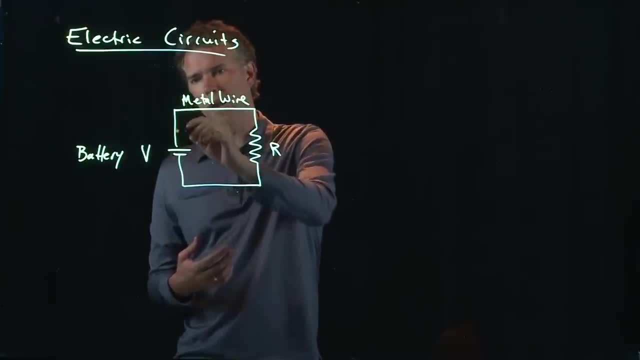 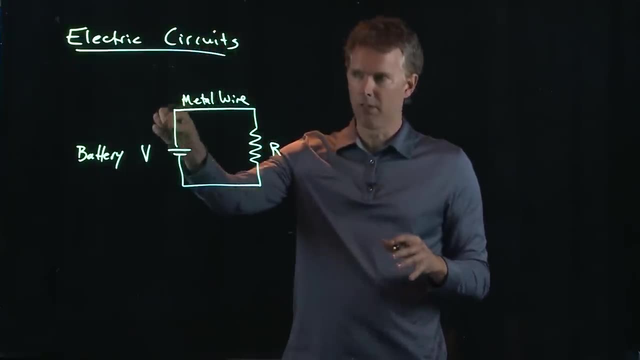 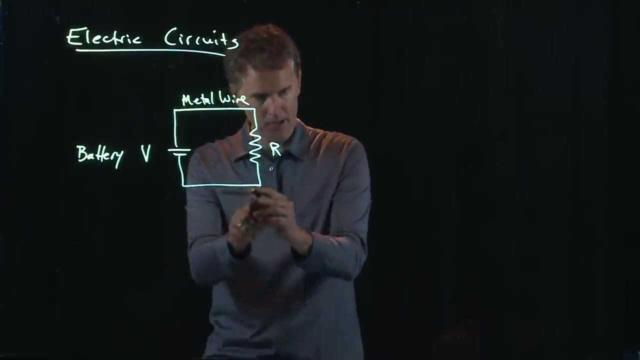 everywhere. So the potential anywhere from this side of the battery all the way around to this side of the resistor is exactly the same. That potential is the same along that wire. Likewise on the bottom side here from the negative side of the battery you have. 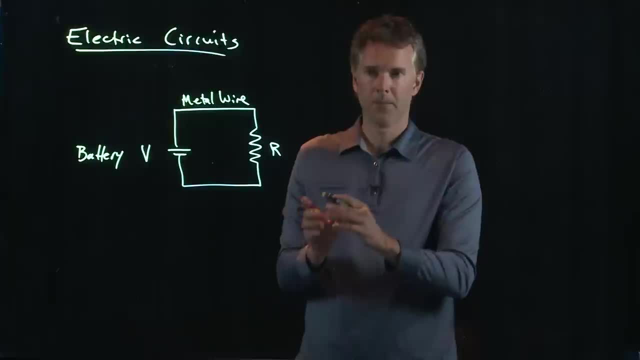 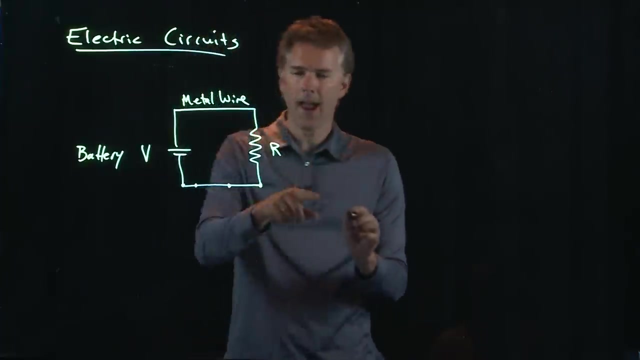 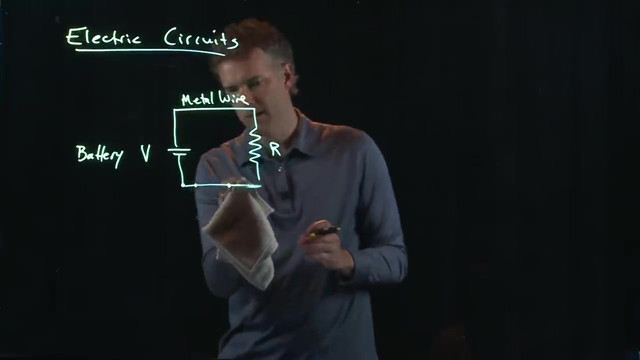 an equipotential. So if I take the voltage there or I take the voltage there, or I take the voltage there or there, anywhere along that wire, I'm going to measure the same voltage likewise along the top wire. What happens in this circuit? 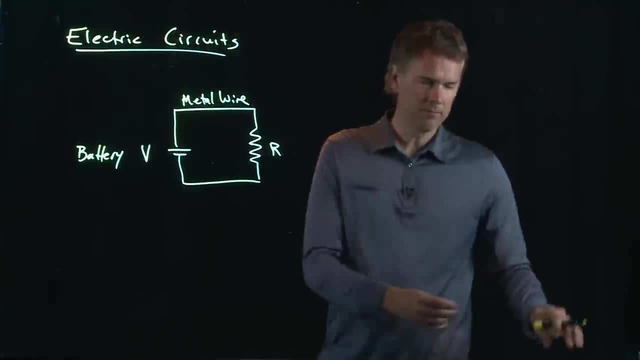 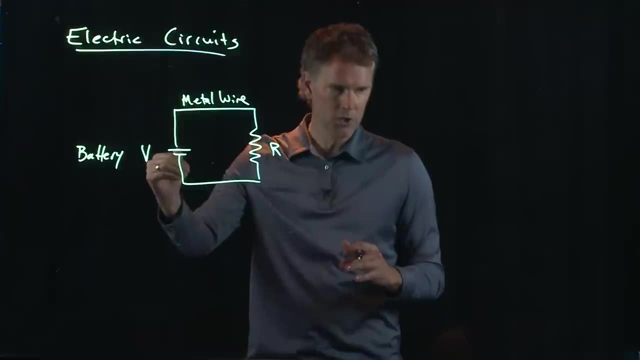 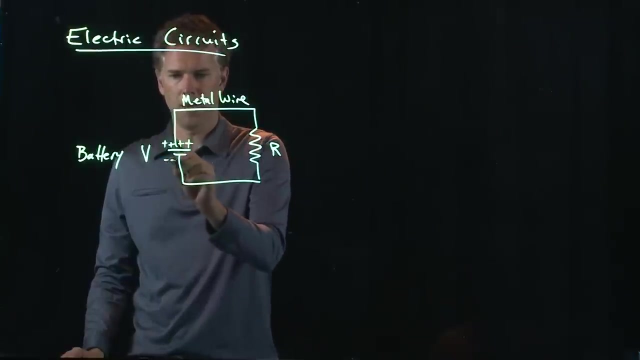 In this circuit. the battery is just like a capacitor. You have a bunch of positive charge on one side, you have a bunch of negative charge on the other. And if I put a bunch of positive charge on this side and I put negative charge on this side, it's going to do something to the 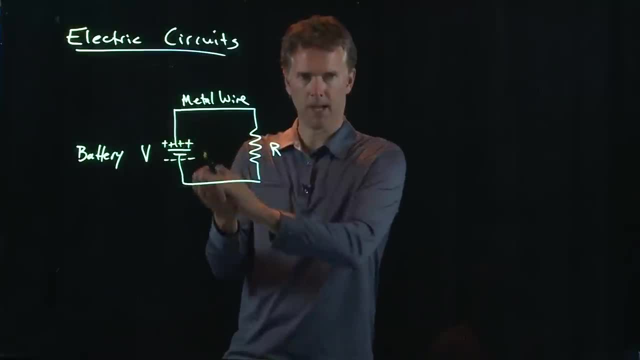 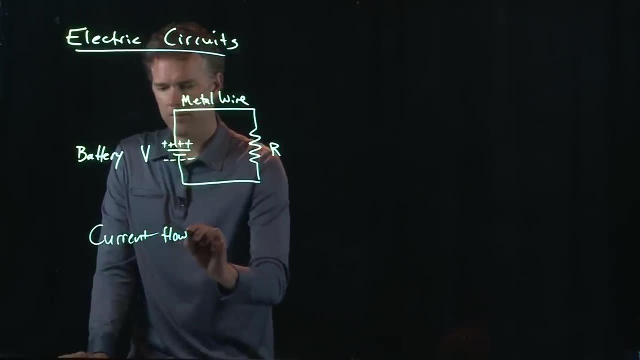 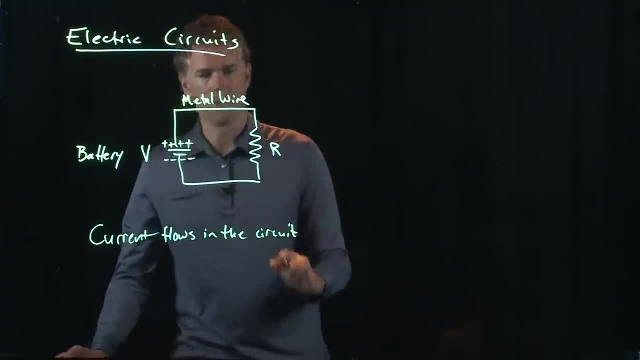 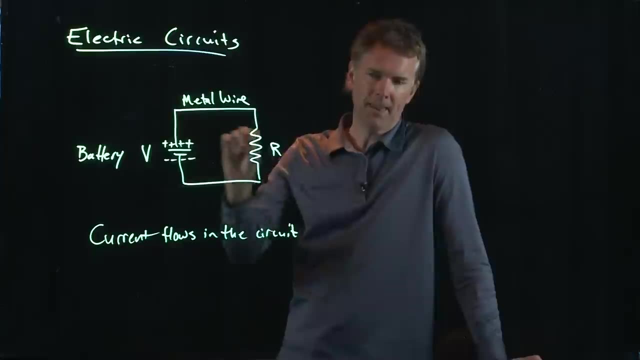 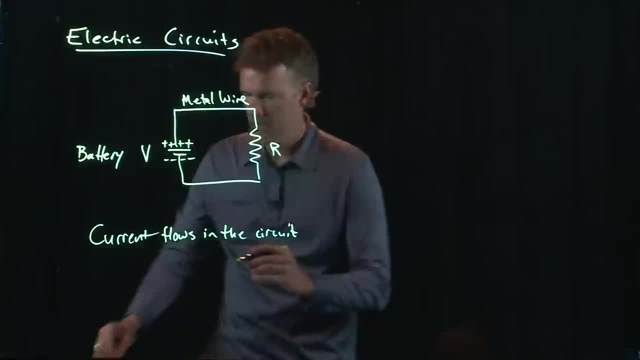 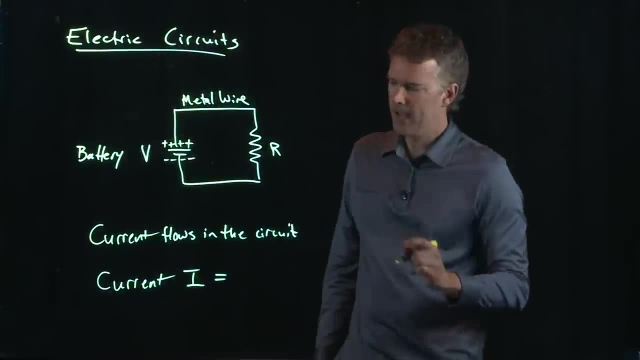 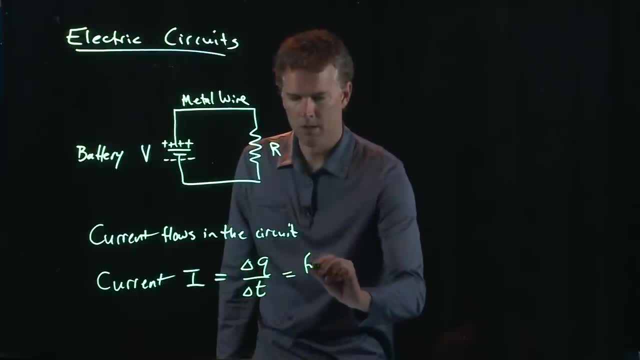 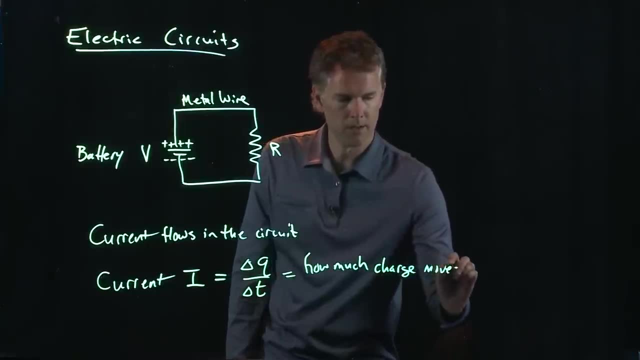 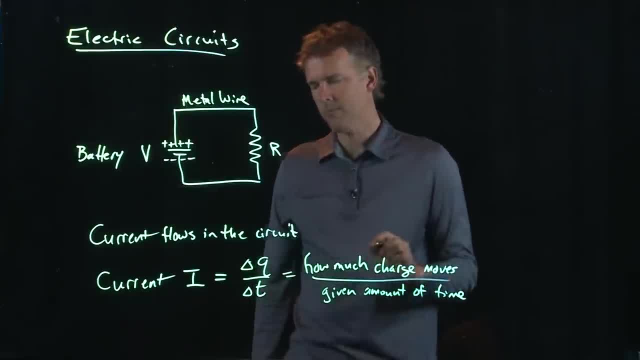 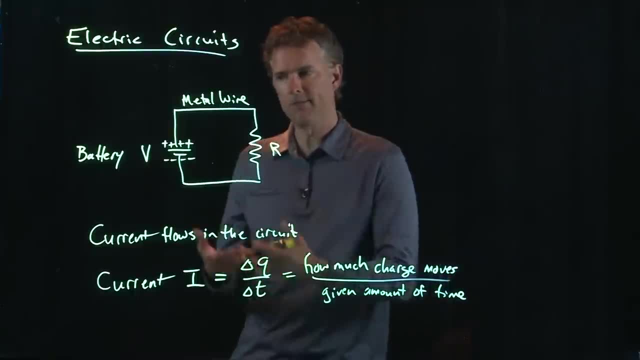 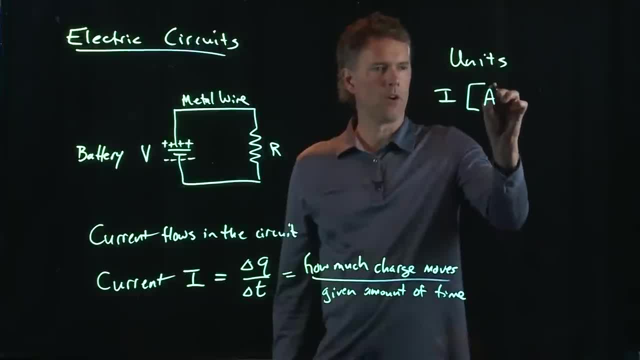 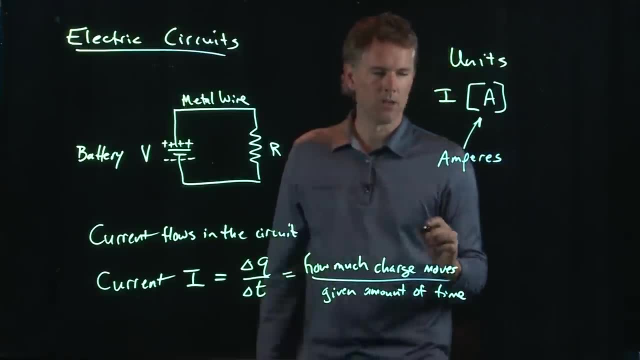 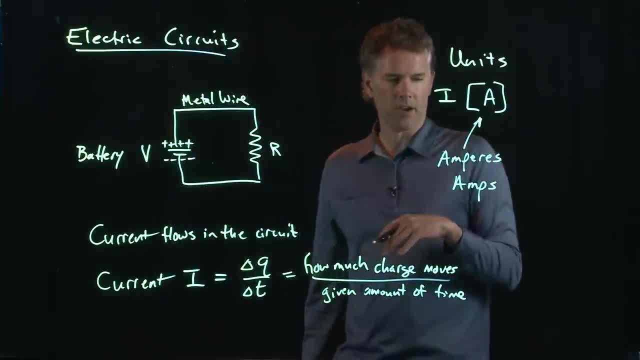 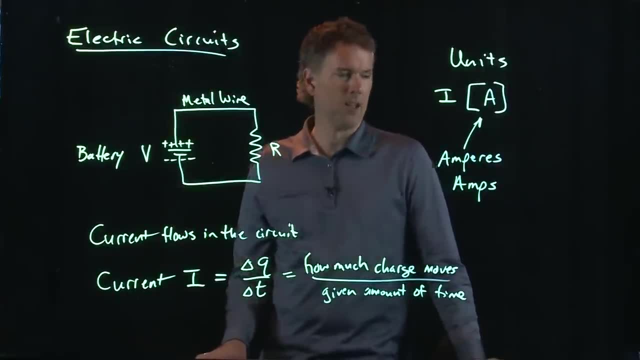 Current flows with my daughters and my oldest daughter said: you know, this is pretty good for an old movie, Like that's old, That's an old movie. They talked a lot about amps in there because they were trying to figure out. 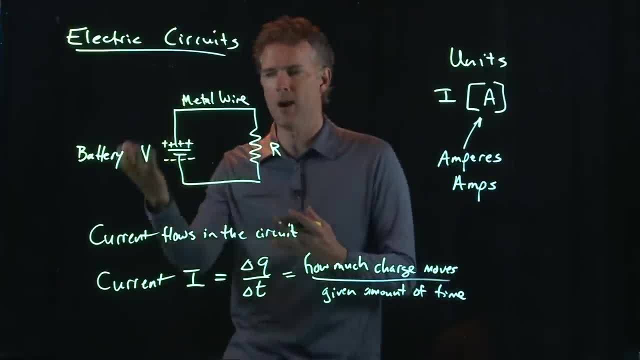 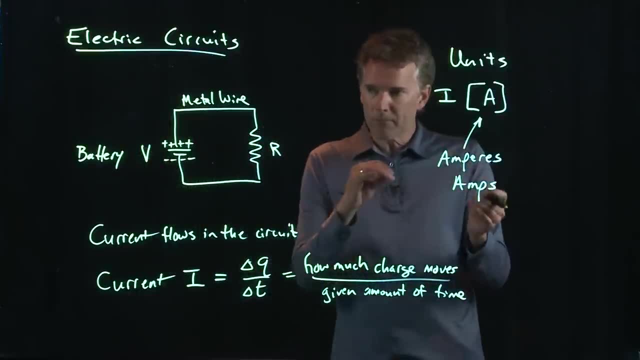 how to power up the spacecraft with a very limited amount of batteries available, very limited amount of battery energy available. So they always talked about: well, how many amps is that gonna draw, How many amps is this gonna draw? And so they had to get really creative. 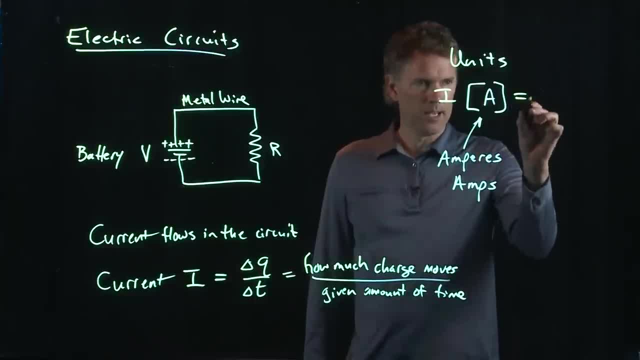 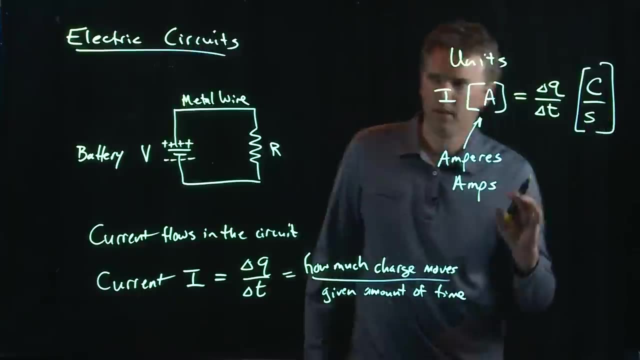 in how they discussed that. What is an amp? Well, it is apparently delta Q over delta T. but we know what that is. Delta Q is coulomb, delta T is seconds. Can you guys still see that over there on the screen? 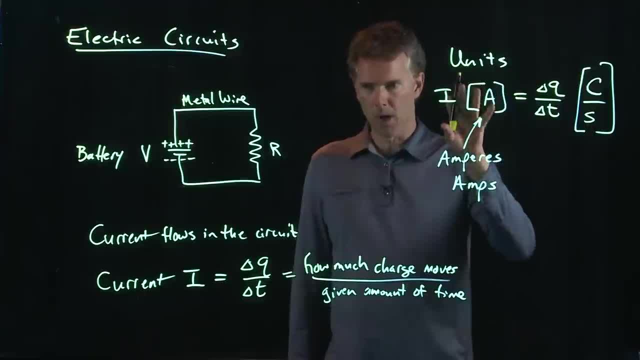 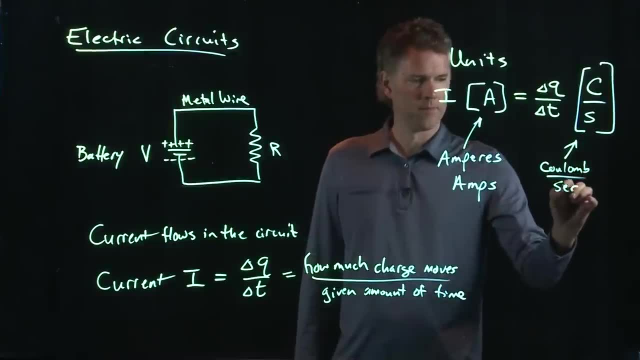 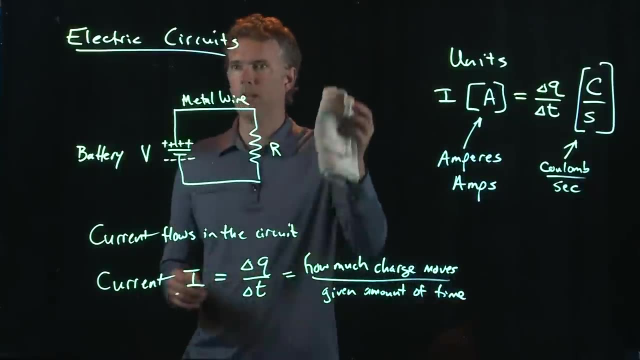 Okay, good, Coulomb per second is an amp. One amp equals one coulomb per second. All right, Let's think about a wire. now Let's think about what is actually happening in this wire. Okay, Let's think about a wire. 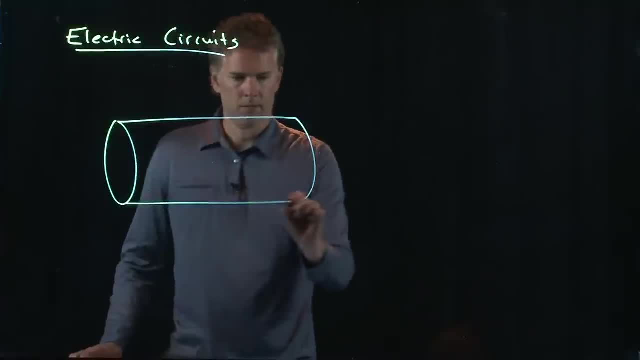 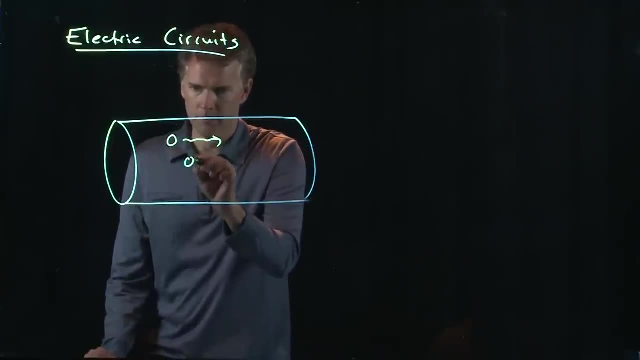 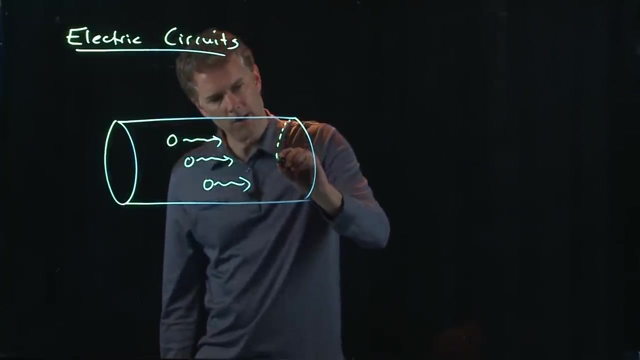 What does a wire look like? A wire looks like this: It's a big chunk of metal, cylindrical in shape. We've got these charges that are gonna move down the wire. If I think about the cross-sectional area A of this wire, 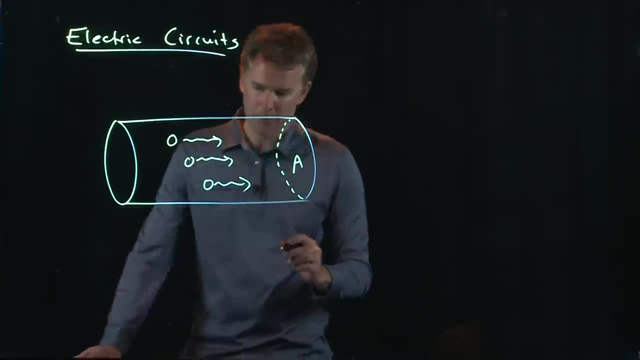 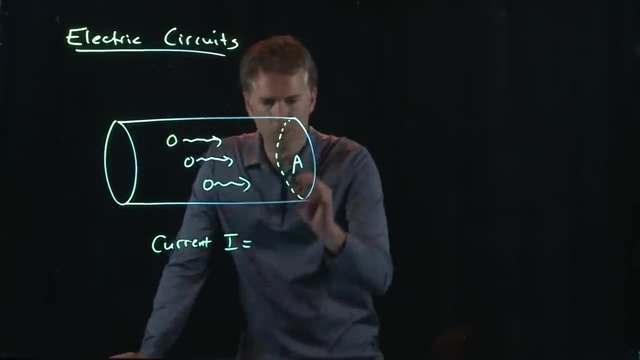 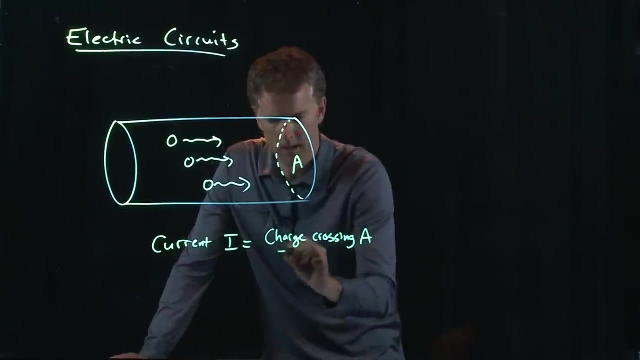 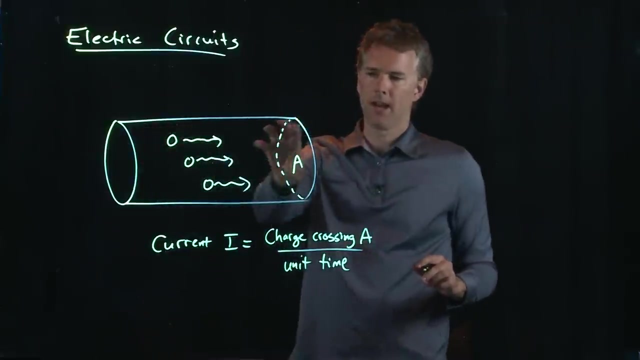 then what can we say about this current I that's flowing in the wire? The current I is equal to the charge crossing that cross-sectional area A in some unit of time. Okay, All that charge is gonna have to go through. 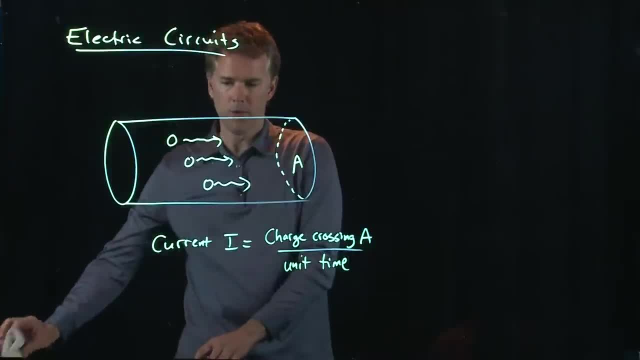 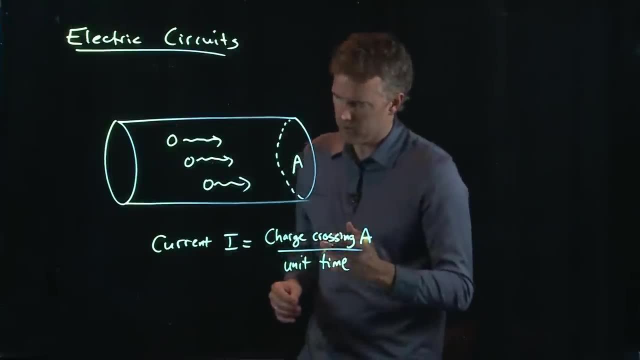 that cross-sectional area A in some amount of time. If you increase the amount of charge doing that, you increase the current. If you decrease the amount of time it takes to do that, you increase the current. Now, when you look at this wire, 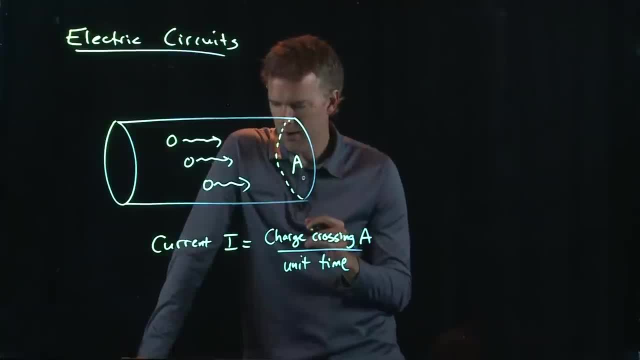 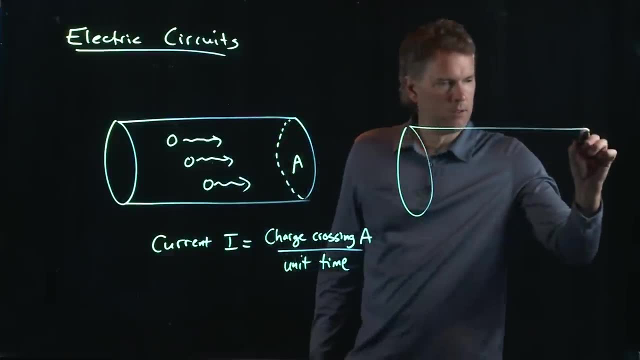 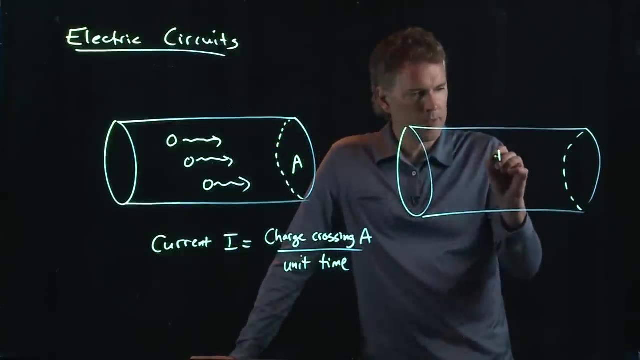 you look at these things that I just drew. they're some sort of charge carrier, But what we really know is a wire has atoms in it that have protons and electrons, And so there is some positive charge, Here's some negative charge. 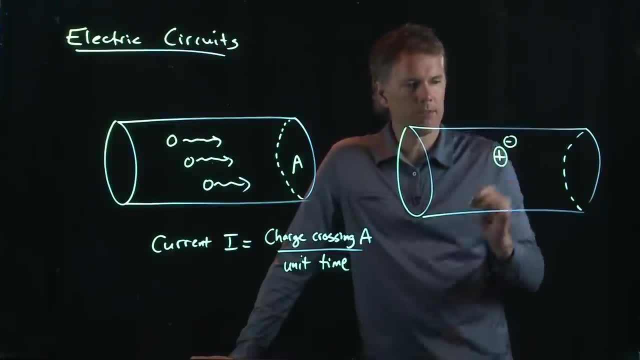 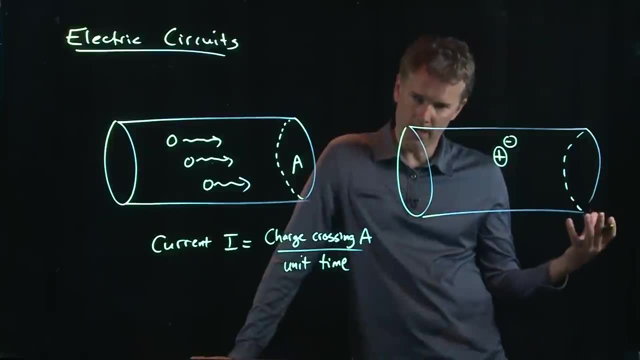 Here's some low-positive charge, And so there's a positive charge here here and there is some negative charge right next to it, And when I apply a field to this thing to generate this current, it's actually the electrons that move. OK. 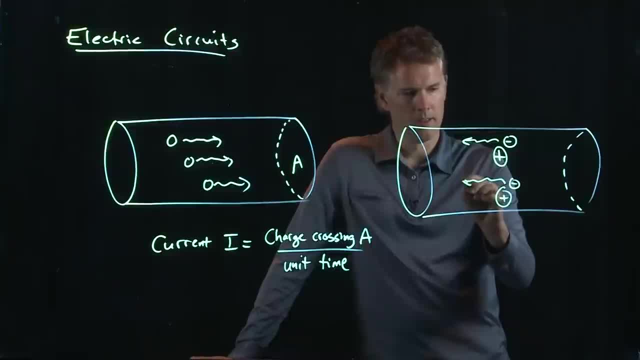 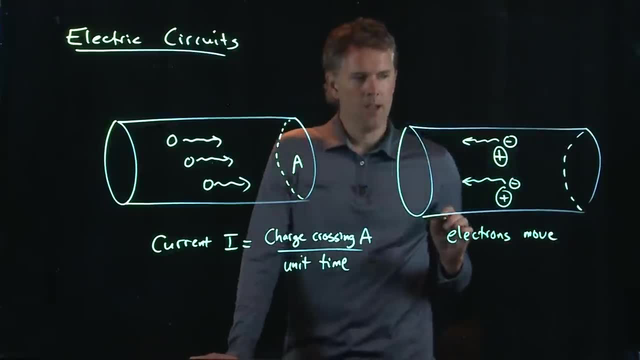 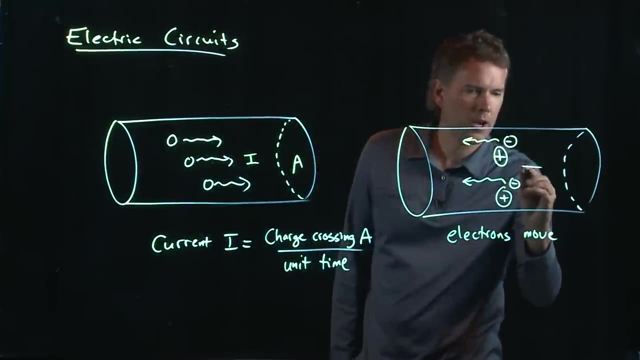 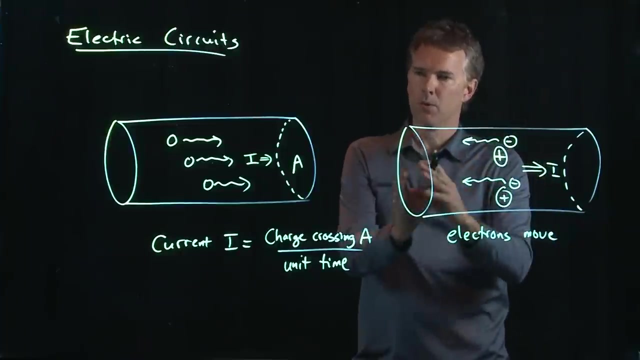 The positives stay where they are. The electrons are the things that move. And here's the deal: If the current I is to the right, then the current I here is still to the right, even though the electrons are moving to the left. OK, 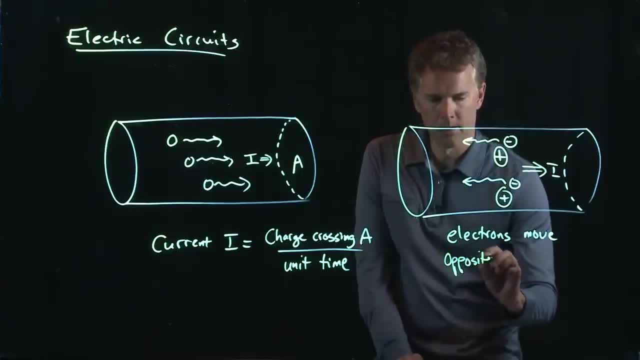 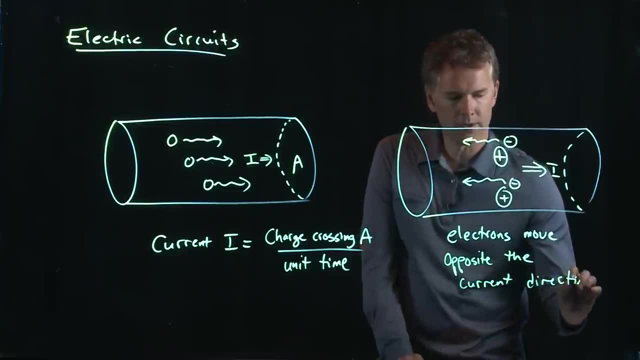 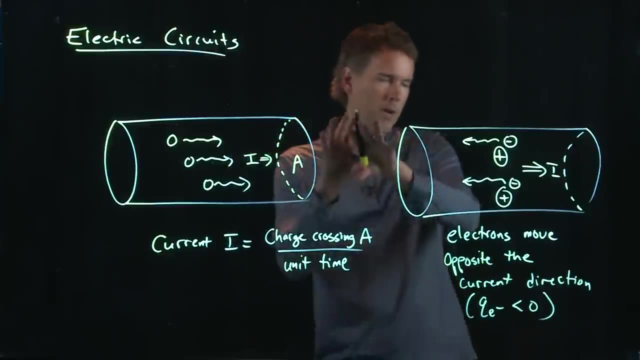 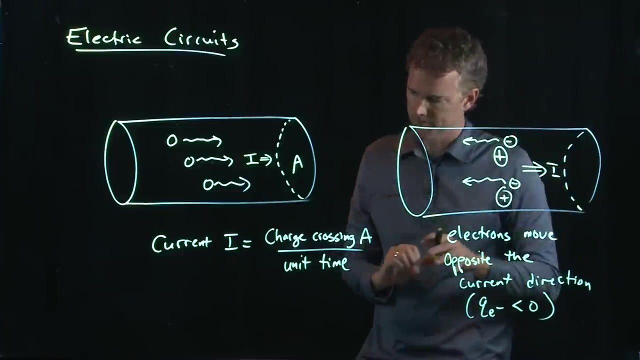 So the electrons move opposite the current direction And that's because they are negatively charged right. Q for an E minus is negative, And so a positive current to the right is really the same as negative electrons moving to the left. So whenever we draw a current, you're always talking. 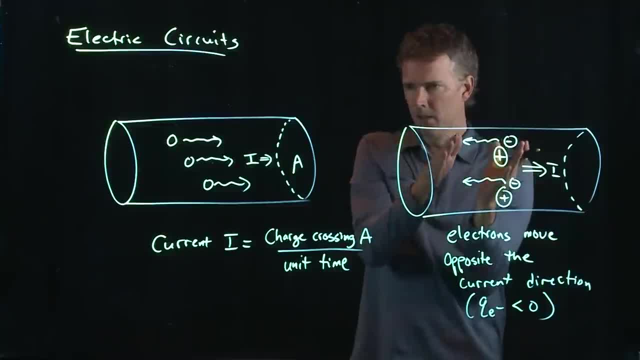 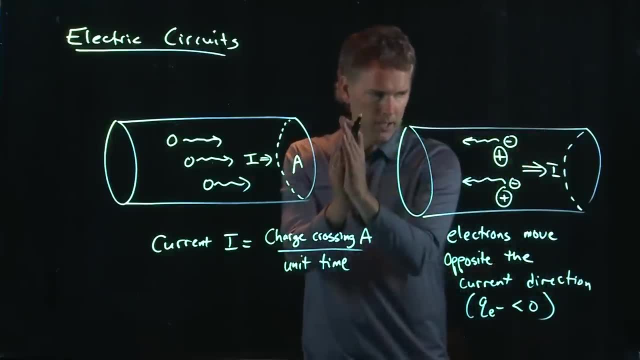 about which way do the positive charges go, Even though in reality we know the positive charges more or less stay where they are. The electrons move this way. Now, if electrons are moving to the left, there ends up a net positive charge over here on the right. 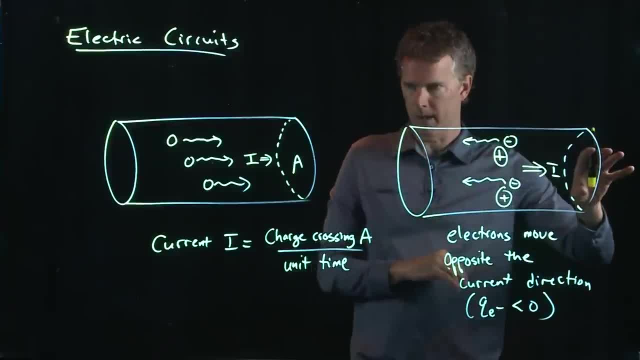 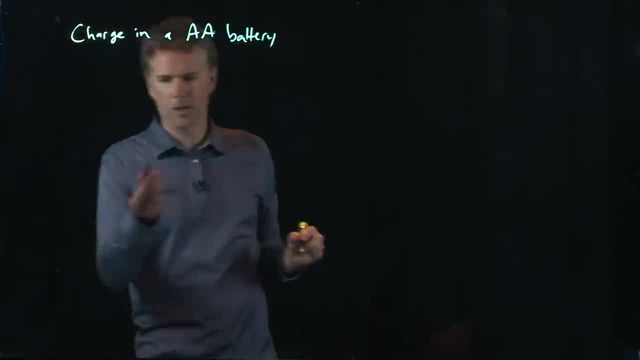 And so it's effectively like those positive charges. OK, So the positive charges move to the right, So the positive charges move to the left, And then the negative charges move to the right, OK, OK, So here's a AA battery, right. 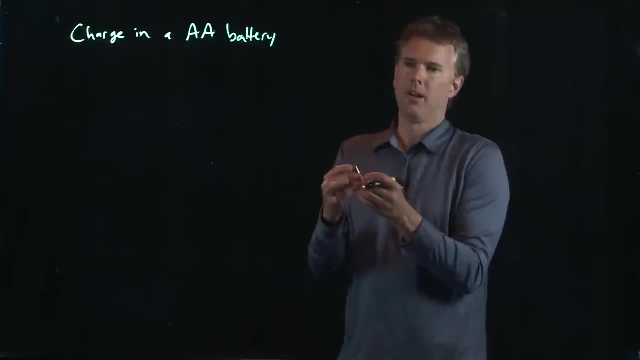 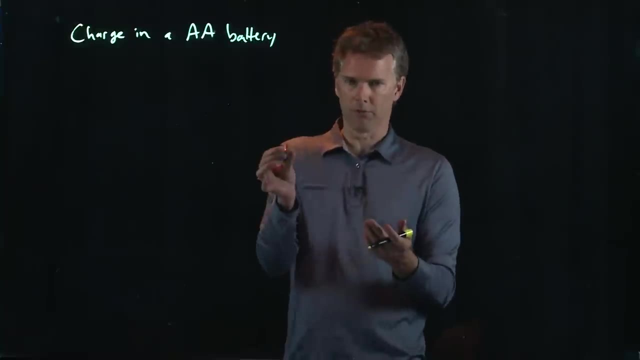 It has some available amount of charge in there. Namely, if I hook this up to a wire, it can power a circuit And it will run for some amount of time, right? You've got these things in all sorts of electronic devices, of course. 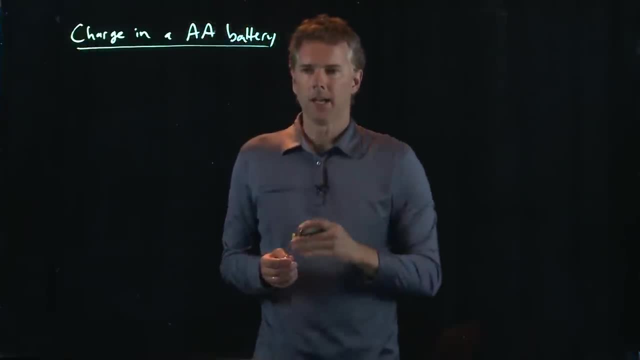 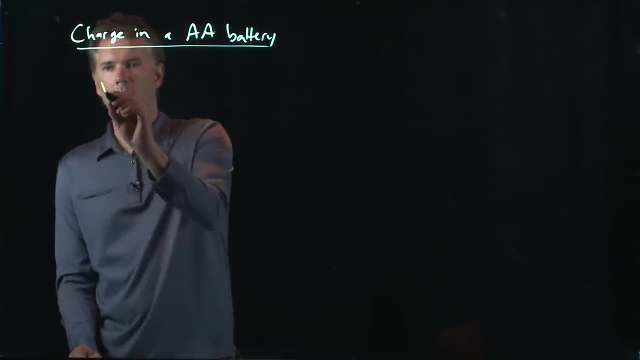 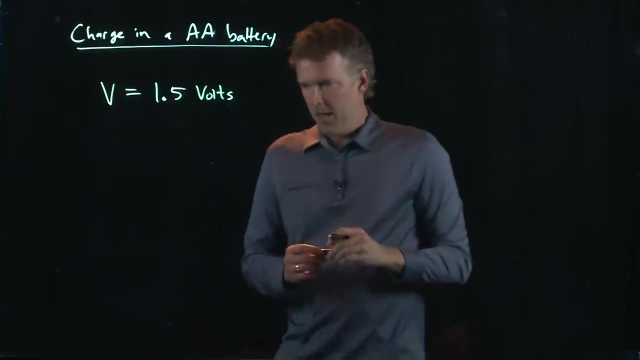 There must be some amount of charge that it can move. Let's figure out what that is. And if you look at the AA battery, it says the voltage is 1.5 volts. If you look up the specs on a AA battery, 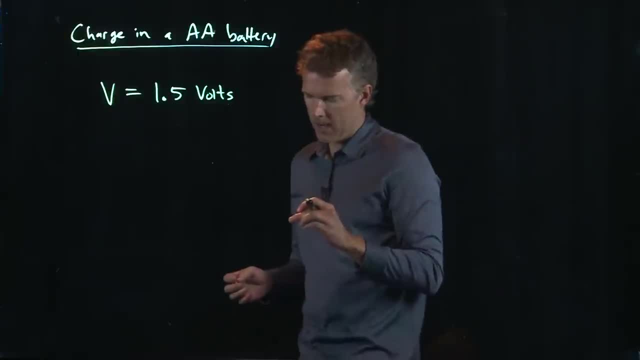 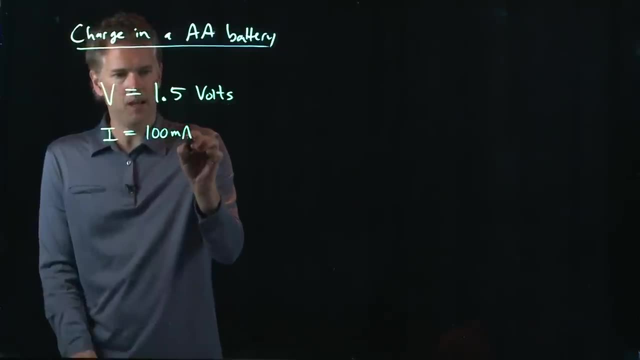 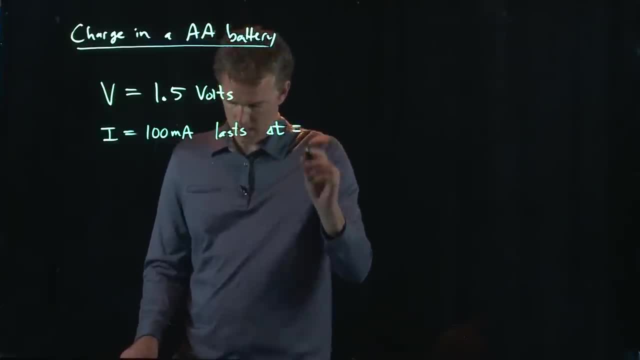 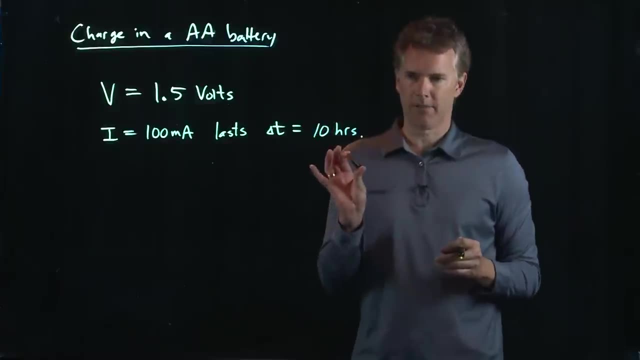 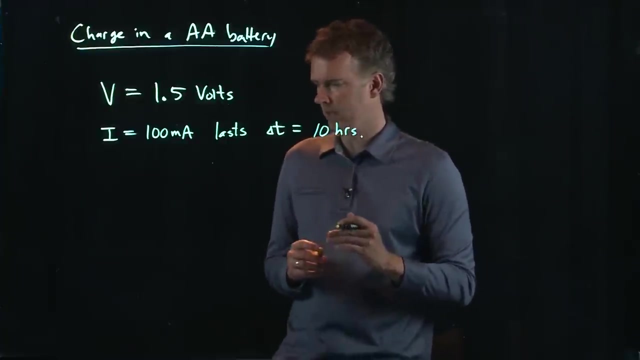 OK, OK For a delta T of about 10 hours. OK, 100 milliamps out of this thing. it'll last for about 10 hours. OK, Let's figure out how much charge that means is coming out of this AA battery. 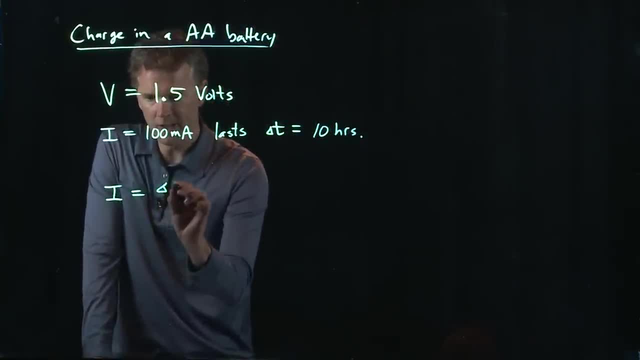 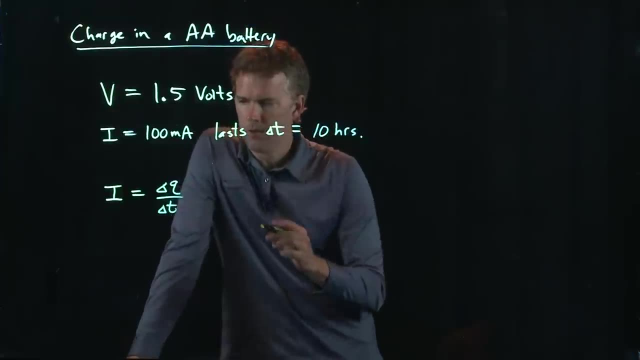 So what do we know? We know I current is delta Q over delta T. We also know that we have I, we have delta T, we're looking for delta Q and that's going to be in coulombs. 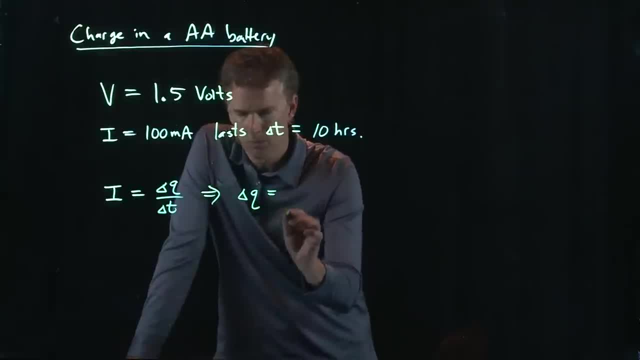 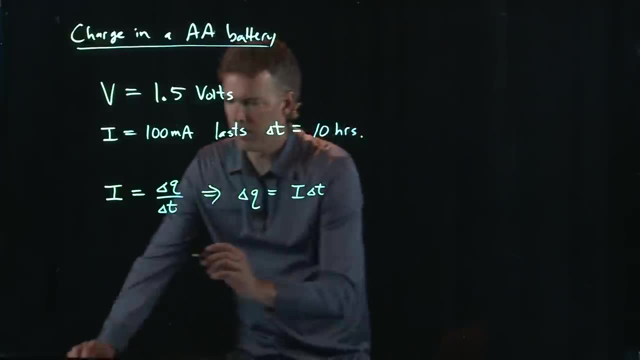 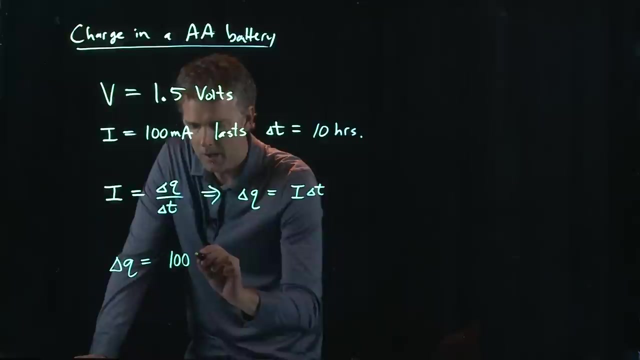 So let's just solve this for delta Q. Delta Q equals I delta T, And we have all those numbers, so let's plug it in: Delta Q equals I delta T, which is 100 milliamps. 100 milliamps is 100. 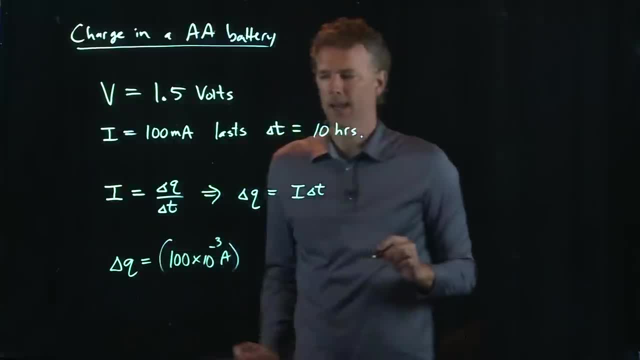 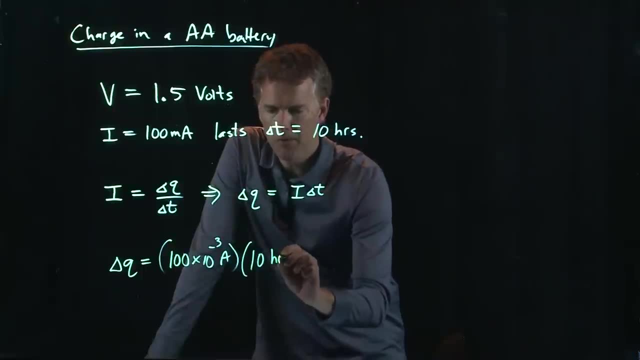 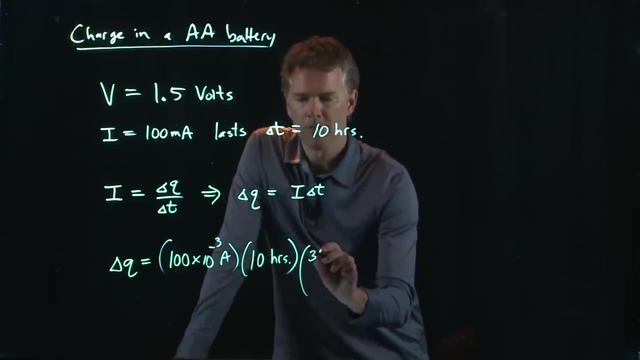 times 10 to the minus 3 amps, And it's going to last for 10 hours. Delta T is 10 hours, but hours is not SI units. We need to get that into seconds, And so we have 3600 seconds. 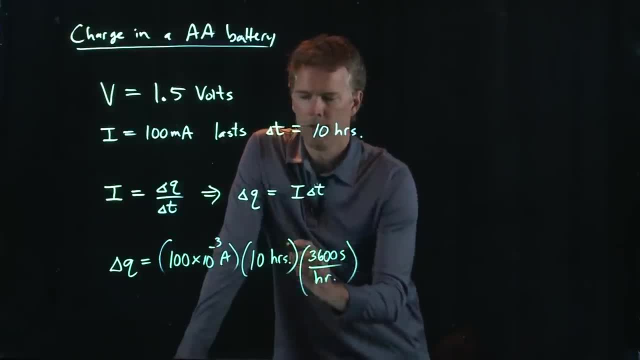 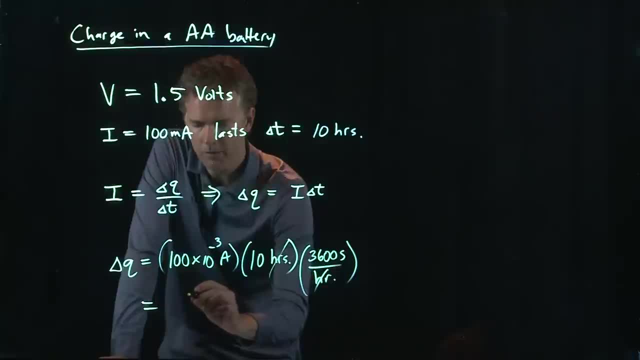 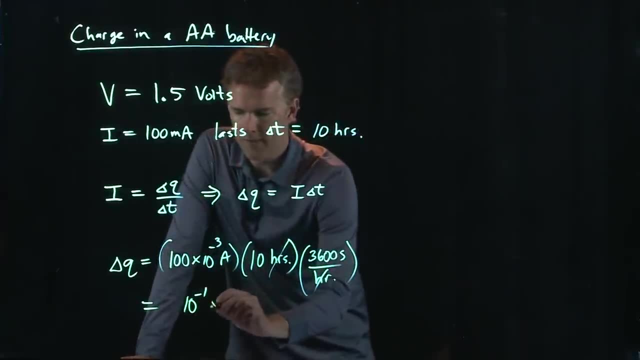 And let's run those numbers and see what we get. So 100 times 10 to the minus 3 is the same as 10 to the minus 1. And then we have a 10 from the 10 hours, And then we have 3600,. 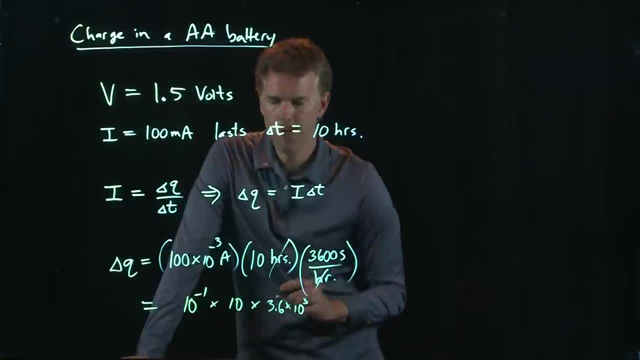 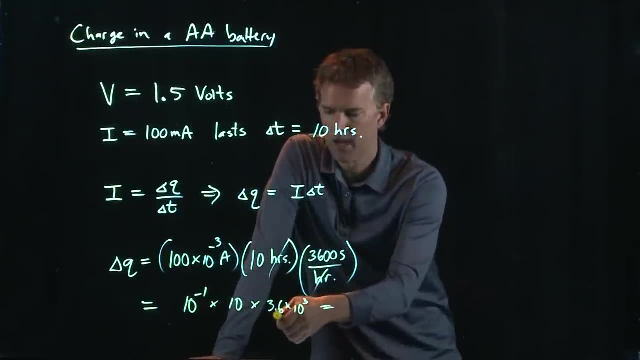 which is 3.6 times 10 to the 3.. And if we plug in all those numbers into your head, it's not so bad right? We've got a 3.6, and then we've got a 10 to the 3.. 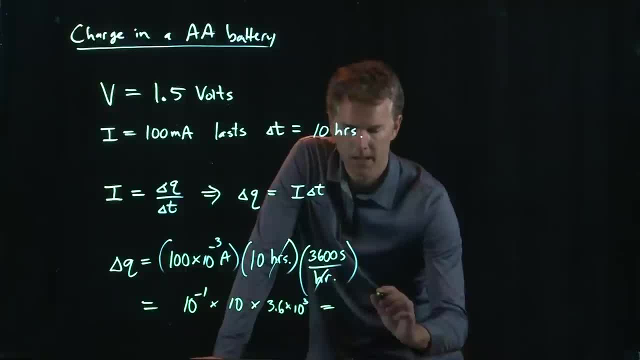 And then we've got a 10 to the 4. And then we're subtracting 1, so it's a 10 to the 3 again, And so we just end up with 3.6 times 10 to the 3.. 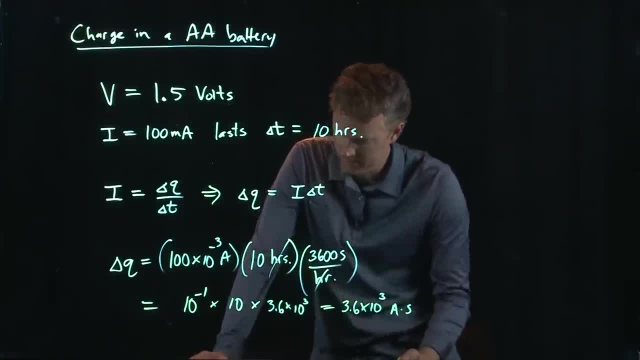 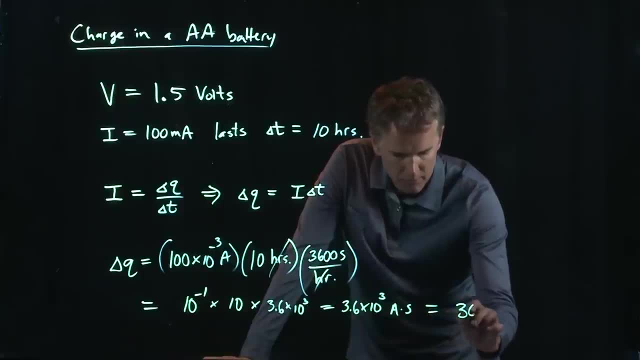 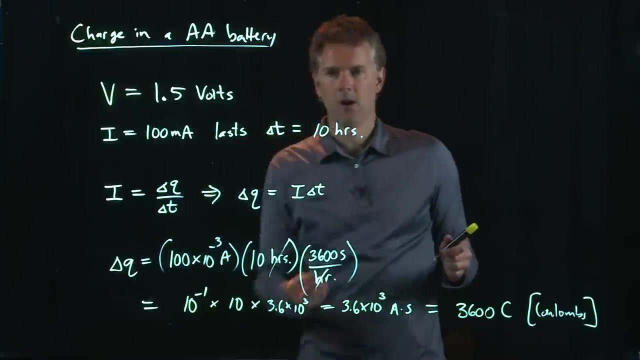 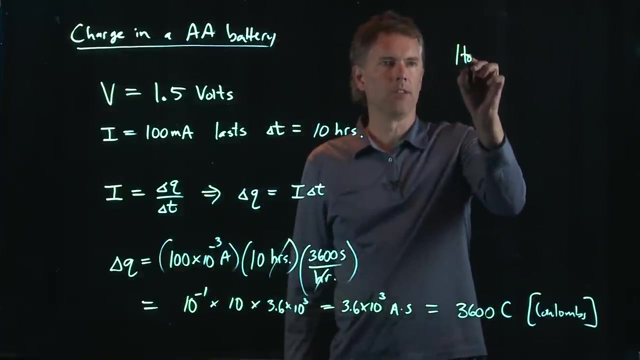 And the units are amp seconds. okay, And that is coulombs. right, We said 1 amp. second is a coulomb. Okay, Okay, So 3600 coulombs of charge in a AA battery that is available for your use. How many electrons? 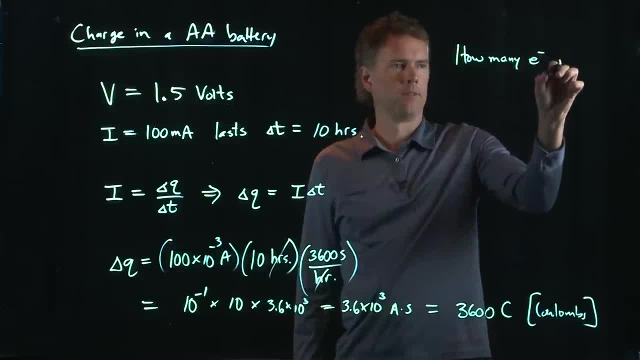 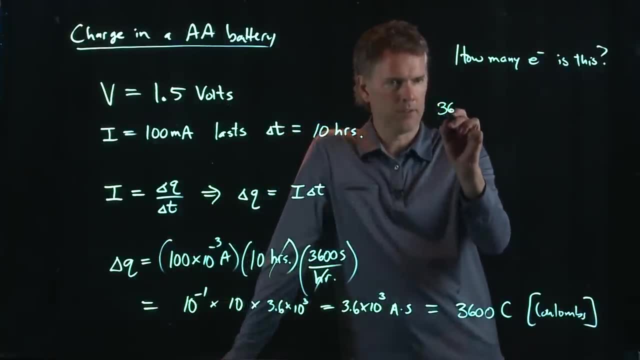 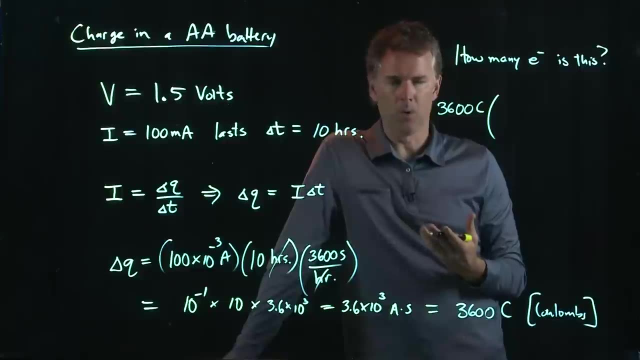 is that? Well, 3600 coulombs. I want to convert that to electrons, so all I have to do is multiply by 1.. So coulombs has to go in the bottom, electrons has to go in the top. and now I need to put. 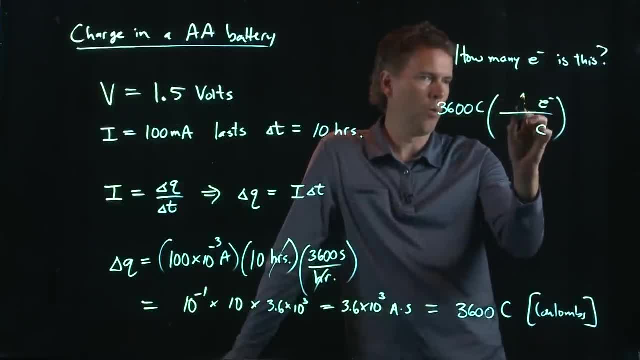 a number here somewhere. What do I know? I know that 1 electron has a charge of 1.6 times 10 to the minus 19 coulombs, And so we get 3.6 times 10 to the 3, divided by 1.6 times 10 to the minus 19.. 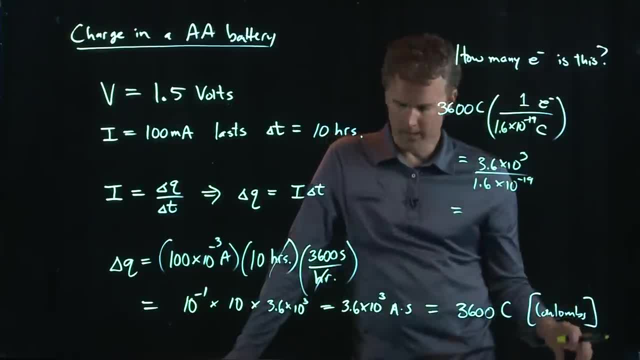 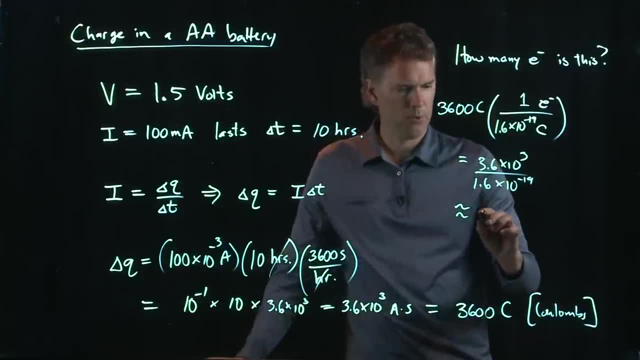 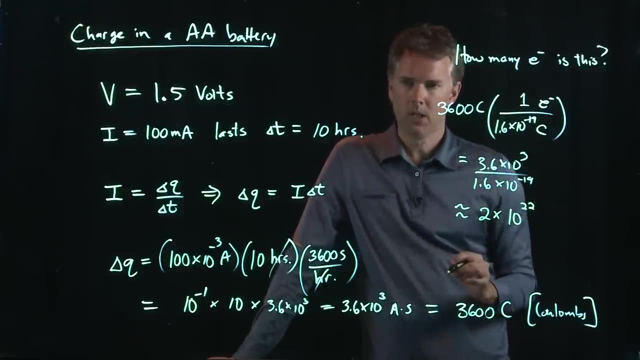 3.6 over 1.6 is pretty close to 2, it's a little bit more than 2, but that's approximately 2.. 2 times 10, I have to add 19 to the top, So I get 2 times 10 to the 22.. 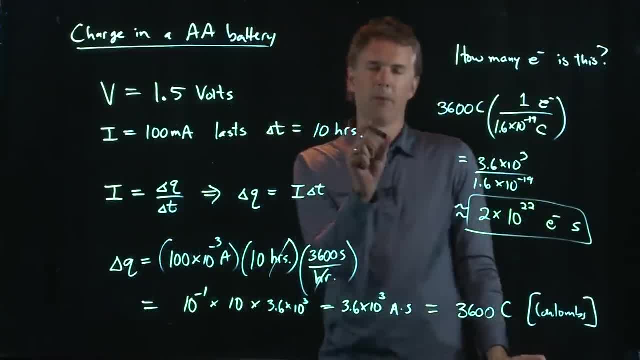 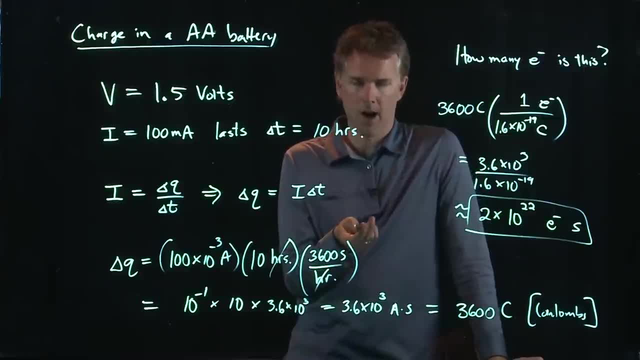 That is a lot of electrons, right. We're thinking about how many electrons are going to come out of this thing. when you run it 2 times 10 to the 22 electrons, that's a phenomenal number. shouldn't scare you, though, right, because we've talked about 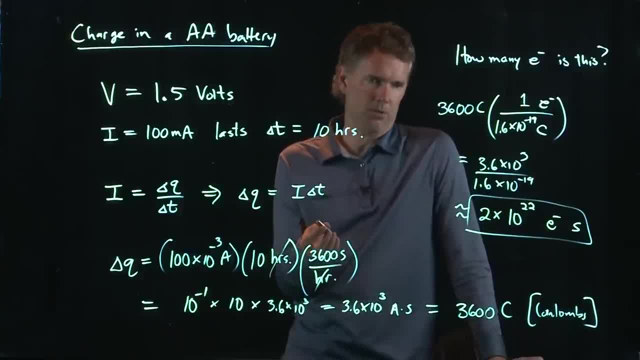 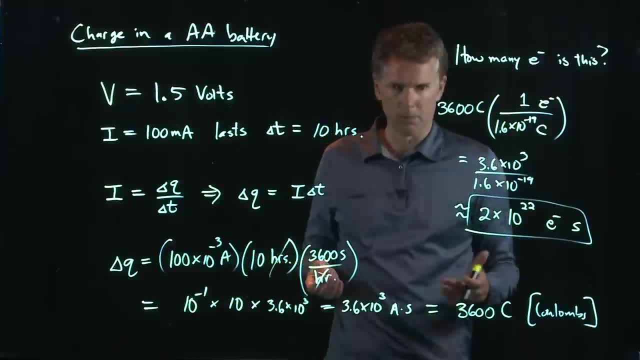 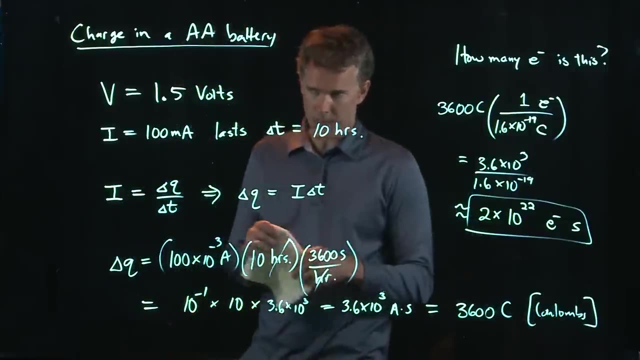 big numbers before Avogadro's number is 6.02 times 10 to the 23, right. so this is on the order of that, which sounds reasonable. okay, let's ask one more follow-up question. let's ask how much energy is available in the double-a. 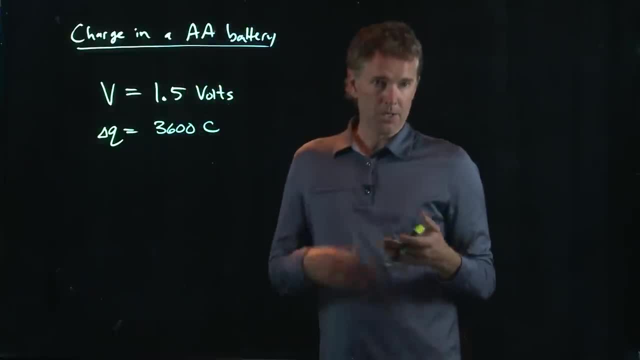 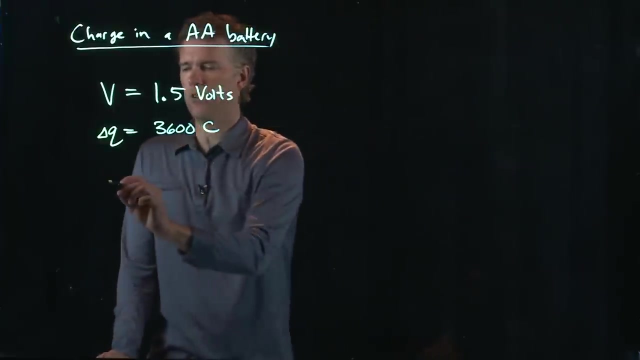 battery. how do I calculate energy? well, we talked a little bit about work, and what you should remember is: oh, energy is in units of electron, volts. electron is charged, V is, of course, volts, so EV is energy. so work or energy is just equal to the number of electrons that are in the double-a battery. so that's the. 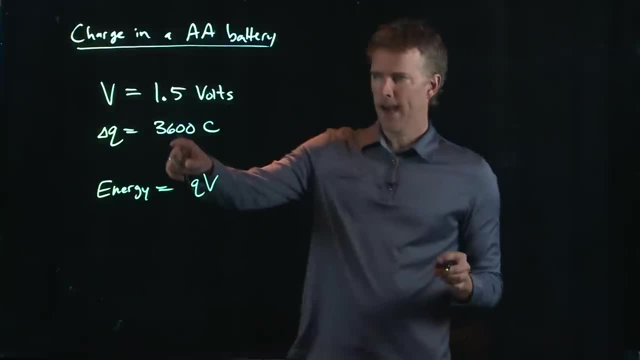 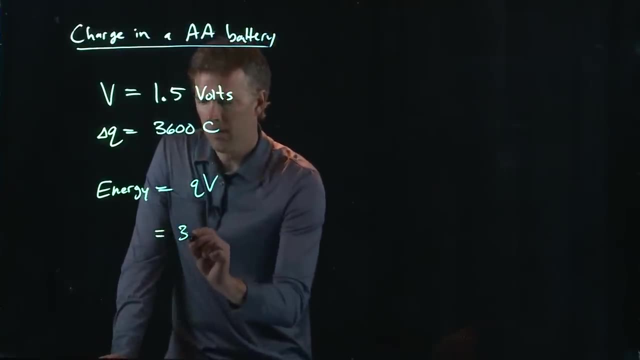 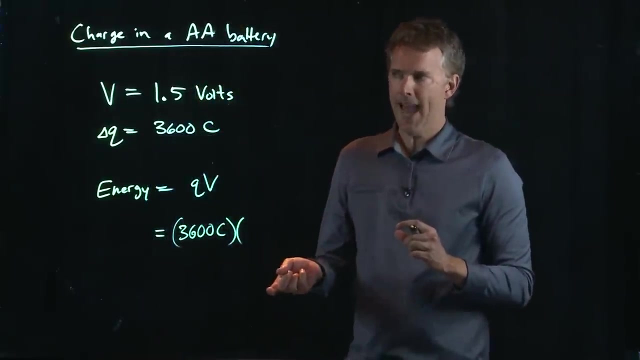 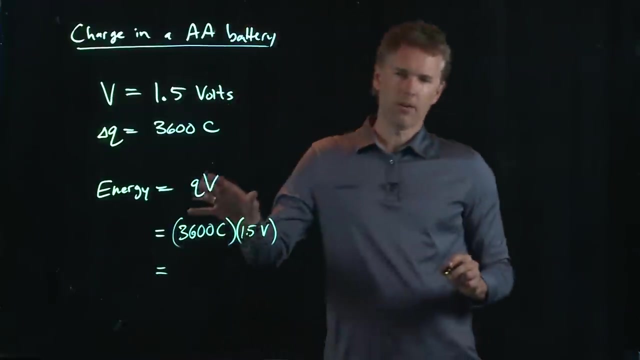 power of energy. so energy is equal to Q times V. and look, we have our Q right here: it's 3600 coulombs, and so energy is 3600 coulombs times the voltage that they come out of that battery at, which is 1.5 volts. and these are all SI units. 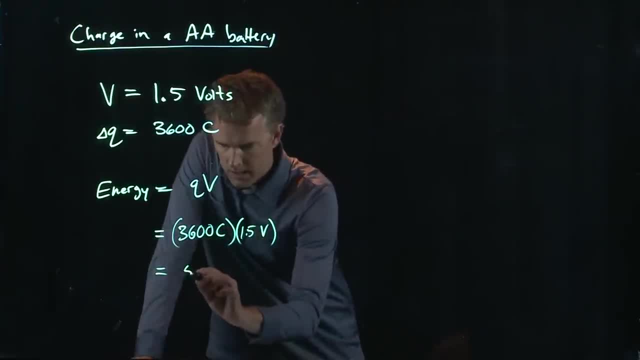 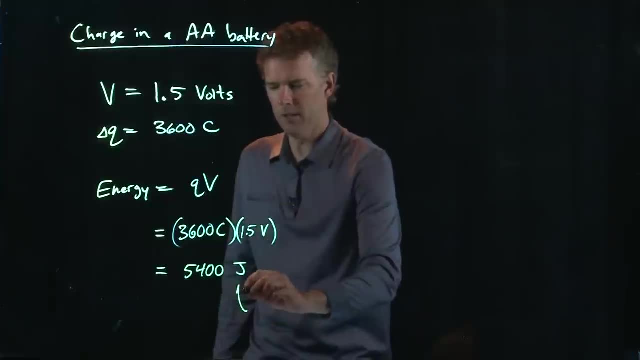 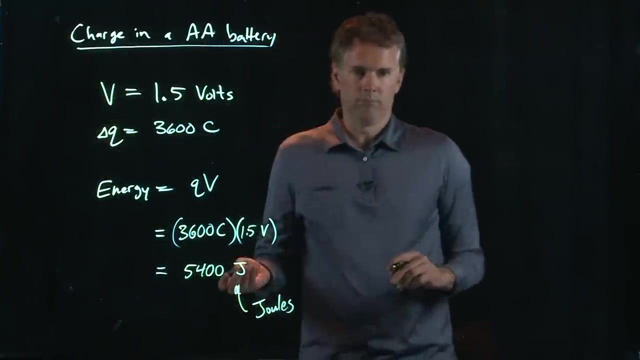 coulombs and volts are all SI units, and so the SI unit of energy is, of course, joules, and you get 5400 joules. this is how much energy is in a double-a battery. so that is a number. we got to decide if that's a big number or a small number. 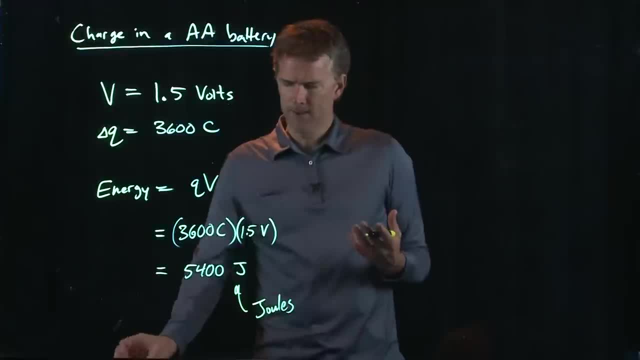 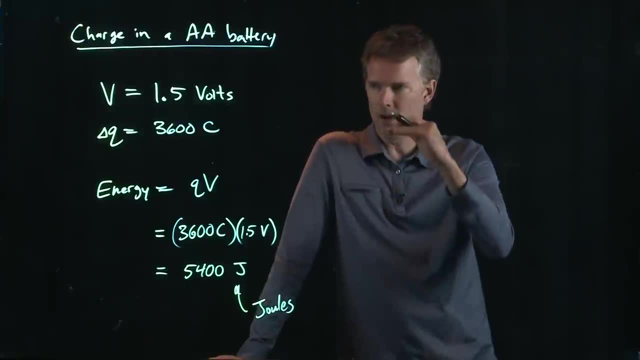 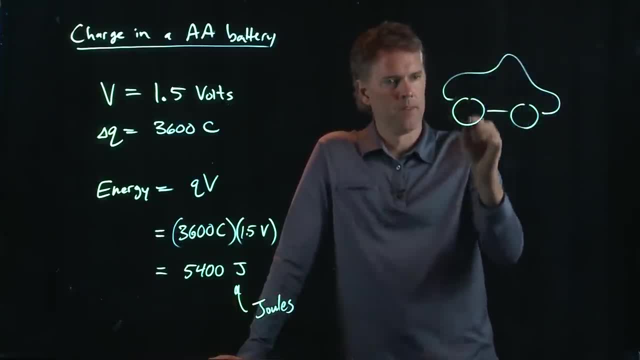 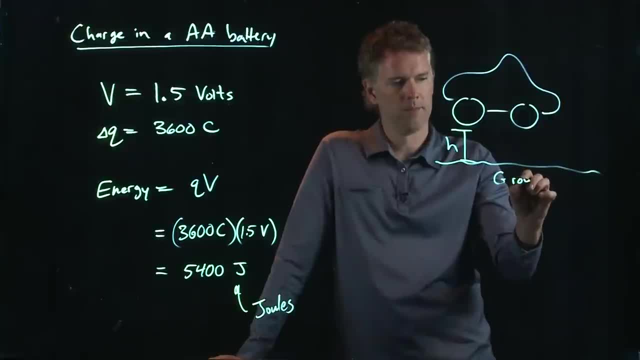 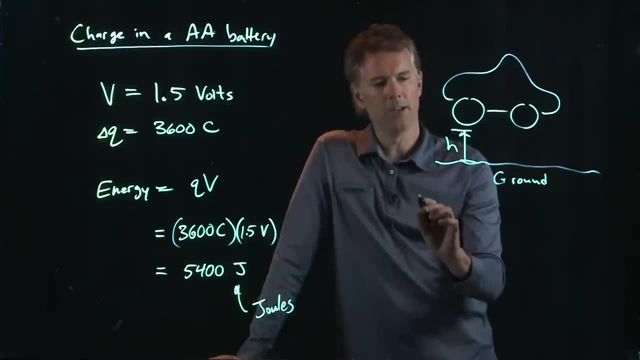 you jack up a car and you lift it a height. you jack up a car and you lift it a height H above the ground. it takes energy to do H above the ground. it takes energy to do H above the ground. it takes energy to do that right. it takes an energy of mg H to. 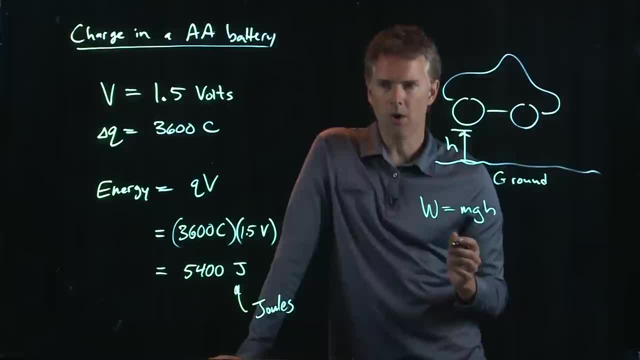 that right. it takes an energy of mg H to that right. it takes an energy of mg H to do that now. a typical car has a maximum. do that now. a typical car has a maximum. do that now. a typical car has a maximum mass M of a thousand two thousand. 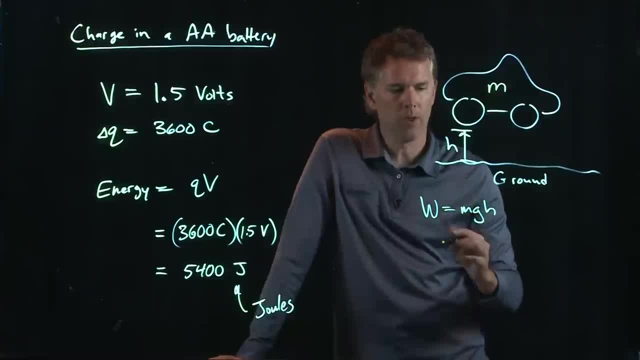 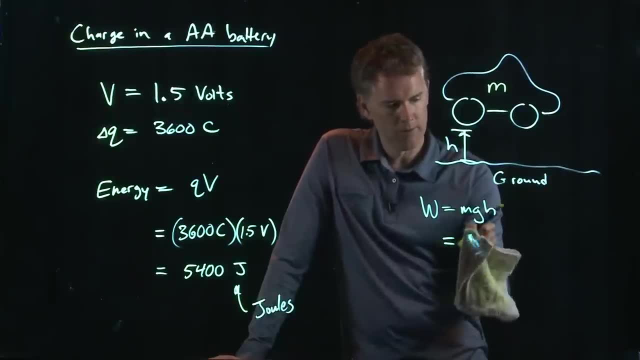 mass M of a thousand two thousand. mass M of a thousand two thousand kilograms. okay, so let's say it's 2,000 kilograms. okay, so let's say it's 2,000 kilograms. okay, so let's say it's 2,000 kilograms. we'll write 2,000 here for M G. 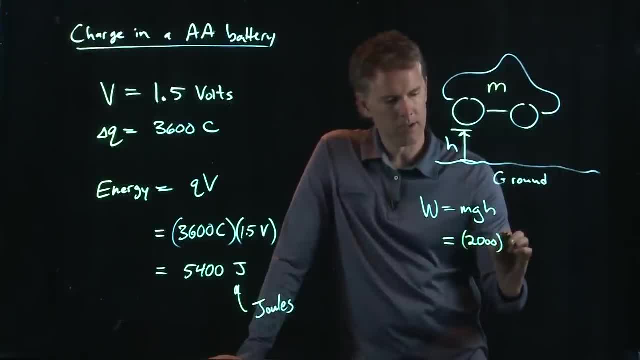 kilograms. we'll write 2,000 here for M G kilograms. we'll write 2,000 here for M G, we know, is of course 9.8. and then we, we know, is of course 9.8, and then we, we know, is of course 9.8. and then we have H, and now let's set it equal to the. 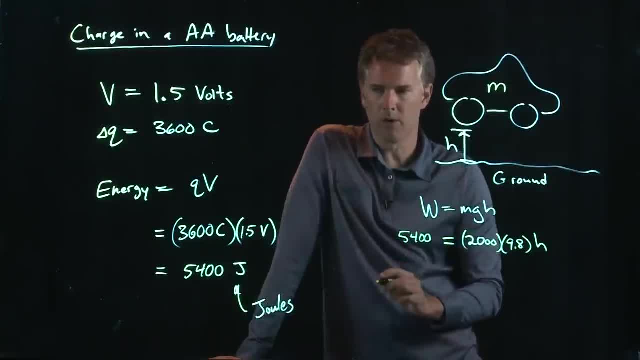 have H, and now let's set it equal to the have H, and now let's set it equal to the work from the double-a battery. work from the double-a battery. work from the double-a battery. fifty four hundred joules, all right, how. fifty four hundred joules, all right, how. 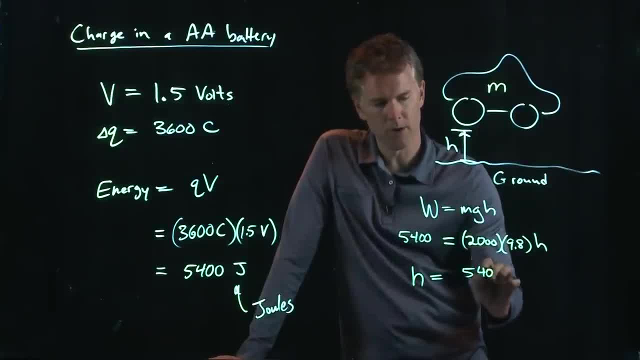 fifty four hundred joules, all right, how high can we raise that car? well, we've high. can we raise that car? well, we've high, can we raise that car? well, we've got 5,400 divided by 2,000 times 9.8. 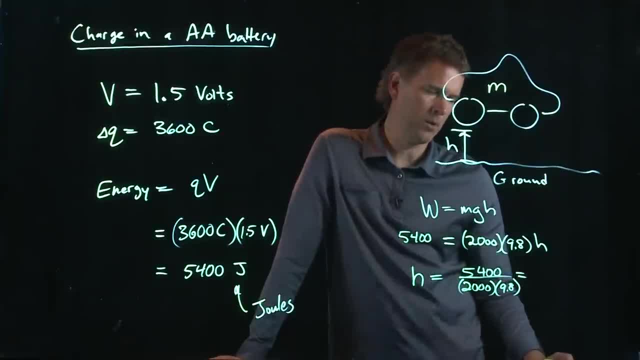 got 5,400 divided by 2,000 times 9.8. got 5,400 divided by 2,000 times 9.8. somebody punch that into your calculator. somebody punch that into your calculator. somebody punch that into your calculator and tell me what you get, and we'll. 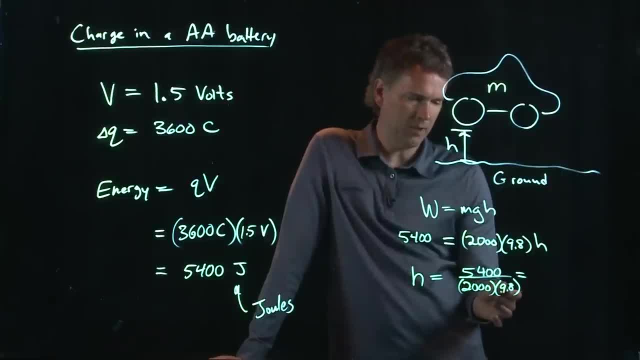 and tell me what you get and we'll, and tell me what you get and we'll approximate it here. 2,000 times 9.8 is approximate it here. 2,000 times 9.8 is approximate it here. 2,000 times 9.8 is pretty close to 3,000. and then I have. 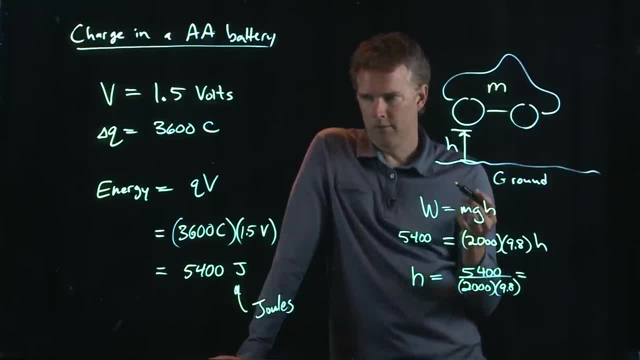 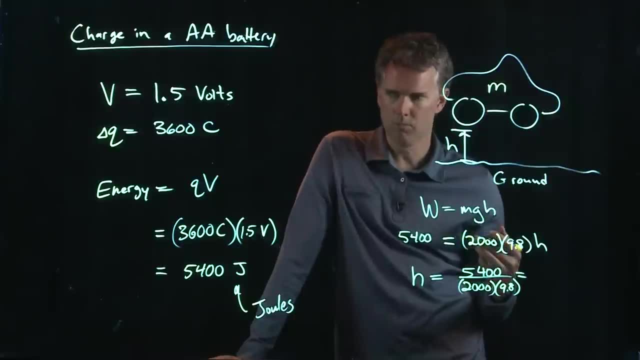 pretty close to 3,000, and then I have pretty close to 3,000, and then I have 5,400 over 3,000, which is 5.4 over 3 and 5.4 over 3, and 5.4 over 3 and 5.4 over 3 is not quite 2, it's maybe 1.7. 5.4 over 3 is not quite 2, it's maybe 1.7. 5.4 over 3 is not quite 2, it's maybe 1.7 or something like that. anybody get a or something like that. anybody get a. 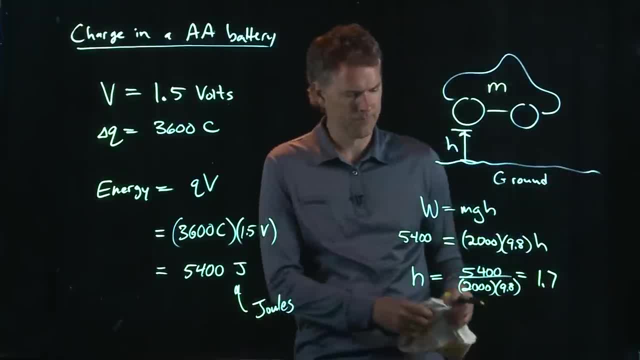 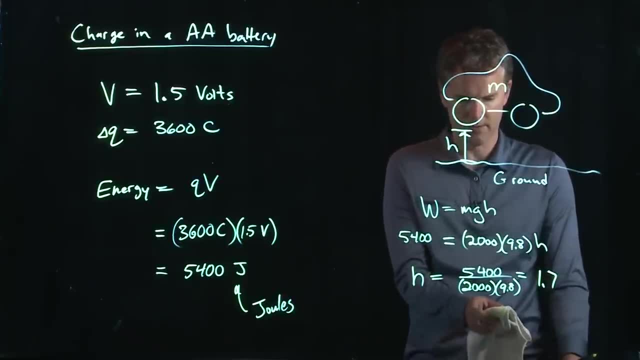 or something like that. anybody get a real number there? you got 0.27. did we do real number there? you got 0.27. did we do real number there? you got 0.27. did we do something wrong? oh yeah, we forgot this something wrong. oh yeah, we forgot this. 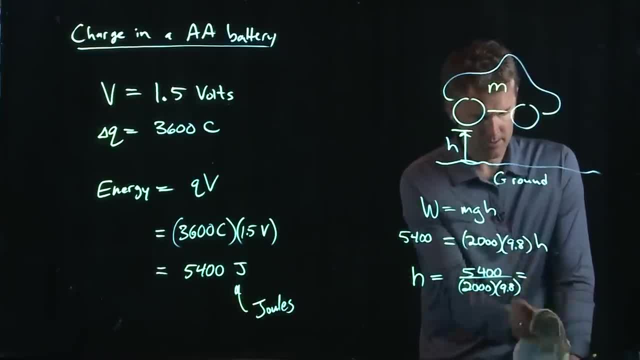 something wrong. oh yeah, we forgot this thing right here, right? no, that's you're thing. right here, right? no, that's you're thing. right here, right? no, that's you're right. I was wrong, right because we've right. I was wrong, right because we've right. I was wrong, right because we've got 5,400, which is 5.4 times 10 to the. got 5,400, which is 5.4 times 10 to the, got 5,400, which is 5.4 times 10 to the 3, and then we've got 2,000 times 9.8 I 3, and then we've got 2,000 times 9.8 I. 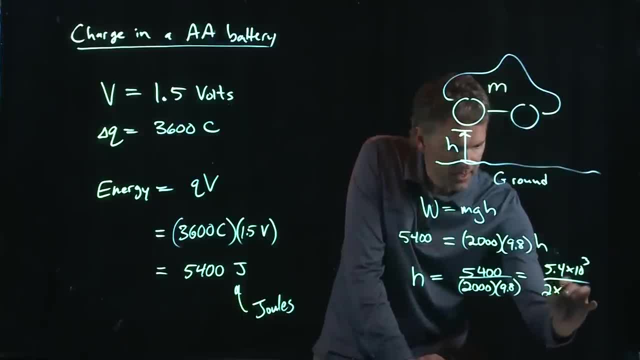 3, and then we've got 2,000 times 9.8. I don't know what I was talking about. don't know what I was talking about. don't know what I was talking about there. this is 2 times 10 to the 4. 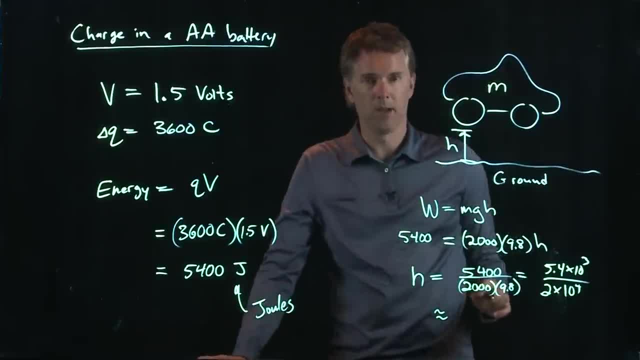 there, this is 2 times 10 to the 4. there, this is 2 times 10 to the 4 approximately good. anybody watching at approximately good. anybody watching at approximately good. anybody watching at home? nobody's watching? okay, fine, so home nobody's watching? okay, fine, so. 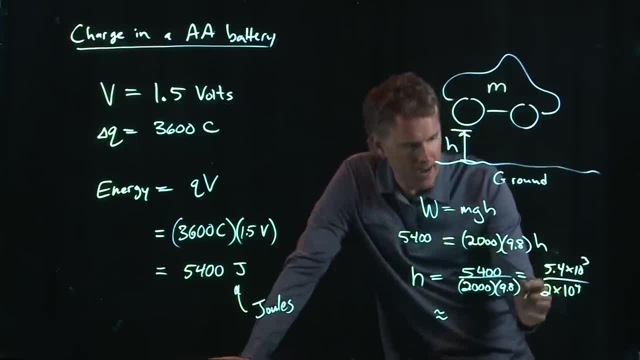 home, nobody's watching. okay, fine, so 5.4 over 2 times 10 to the 4. now we're 5.4 over 2 times 10 to the 4. now we're 5.4 over 2 times 10 to the 4. now we're gonna get what you said, right, because 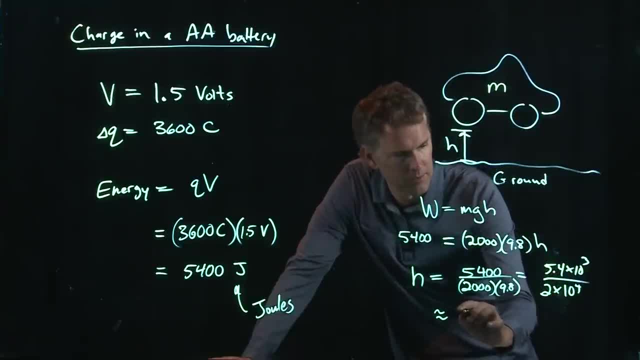 gonna get what you said right. because gonna get what you said right, because this is 5.4 over 2 is 2 and a little bit. this is 5.4 over 2 is 2 and a little bit. this is 5.4 over 2 is 2 and a little bit more, 2.7. but then we have a 10 to the. 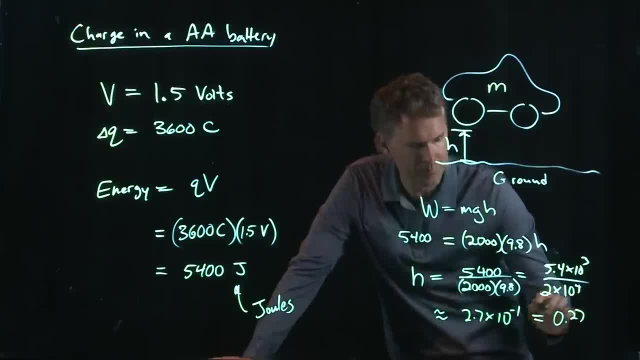 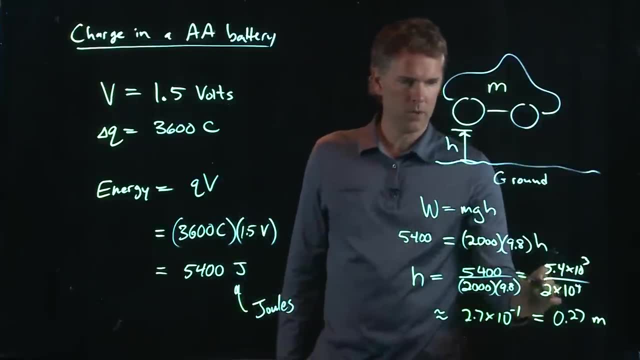 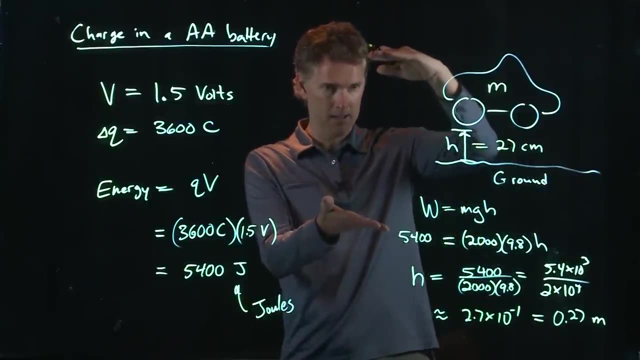 more 2.7. but then we have a 10 to the more 2.7. but then we have a 10 to the meters right, which is 27 centimeters. meters right, which is 27 centimeters. meters right, which is 27 centimeters. that's like that high. so wait a minute. 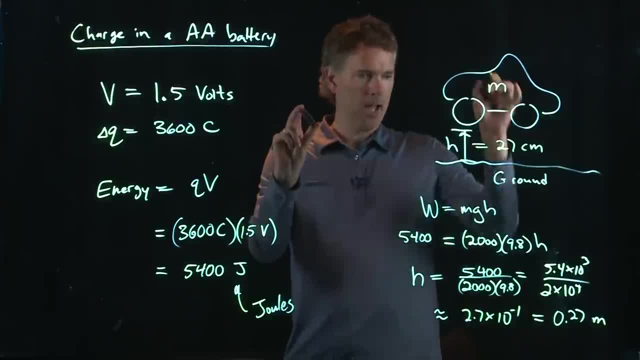 that's like that high, so wait a minute. that's like that high, so wait a minute. are we saying that you could take a? are we saying that you could take a? are we saying that you could take a double-a battery and jack up your car by? 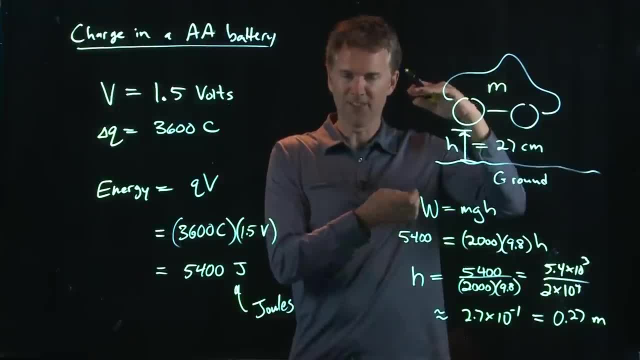 double-a battery and jack up your car by double-a battery and jack up your car by 27 centimeters. yes, that's exactly what- 27 centimeters. yes, that's exactly what- 27 centimeters. yes, that's exactly what we're saying. okay, you would have to gear. 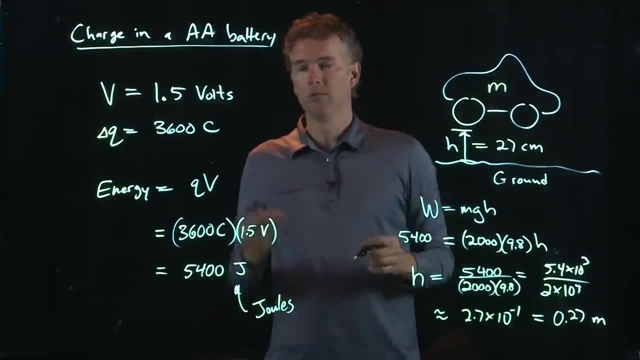 we're saying, okay, you would have to gear. we're saying, okay, you would have to gear down this and it would take you 10 down this, and it would take you 10 down this and it would take you 10 hours to do it, but eventually your car. 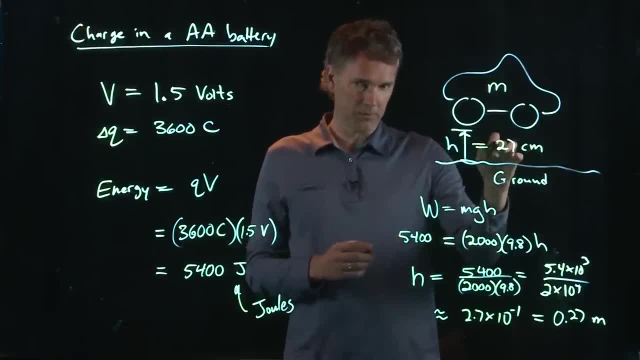 hours to do it, but eventually your car. hours to do it, but eventually your car would lift off the ground now. this is if would lift off the ground now. this is if would lift off the ground now. this is if all the energy was used. right, you're? 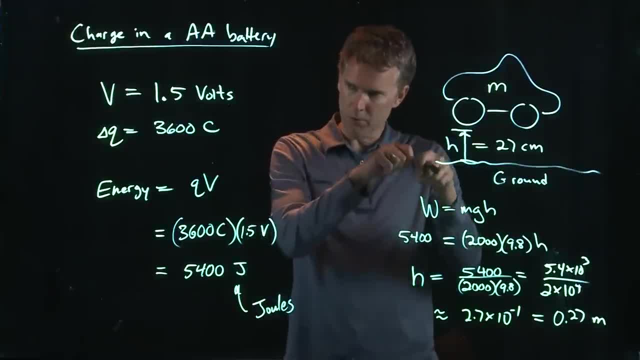 all the energy was used right. you're. all the energy was used right. you're gonna lose some energy in the transfer. gonna lose some energy in the transfer. gonna lose some energy in the transfer. to the electrical motor to crank the. to the electrical motor to crank the. 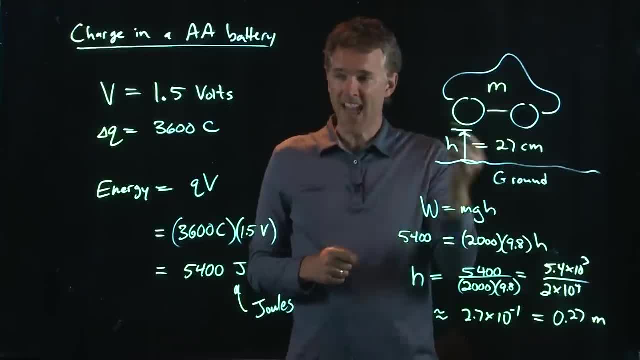 to the electrical motor to crank the gears and so forth. but even if it's off gears and so forth, but even if it's off gears and so forth, but even if it's off by a factor of 10, you could still raise. by a factor of 10 you could still raise. 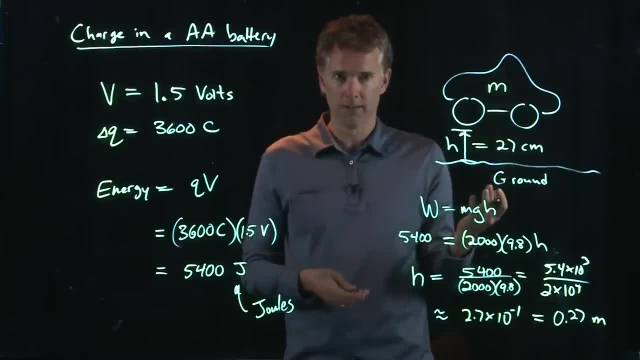 by a factor of 10, you could still raise your car three centimeters, that's enough, your car. three centimeters, that's enough. your car. three centimeters, that's enough to change the tire. so they should just to change the tire. so they should just to change the tire. so they should just start selling. you know, car jacks powered. 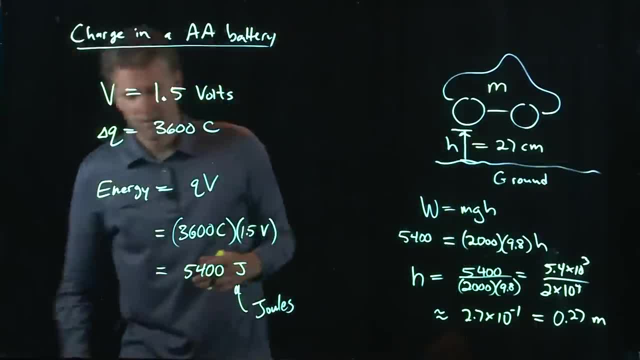 start selling, you know, car jacks powered. start selling, you know, car jacks powered by double-a batteries. I think that'd be by double-a batteries. I think that'd be by double-a batteries. I think that'd be cool: plug it in and wait for 10 hours. cool plug it in and wait for 10 hours. cool plug it in and wait for 10 hours, and then you can change your tire. okay, and then you can change your tire. okay, and then you can change your tire. okay. let's talk about current for a second. 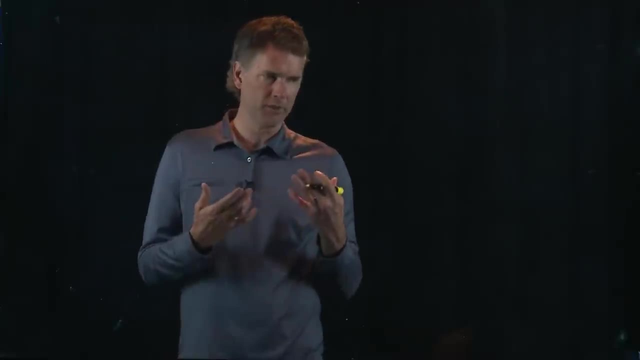 let's talk about current for a second. let's talk about current for a second, this idea that different devices are, this idea that different devices are, this idea that different devices are going to use different amounts of going to use different amounts of going to use different amounts of current, and let's see if we can come up. 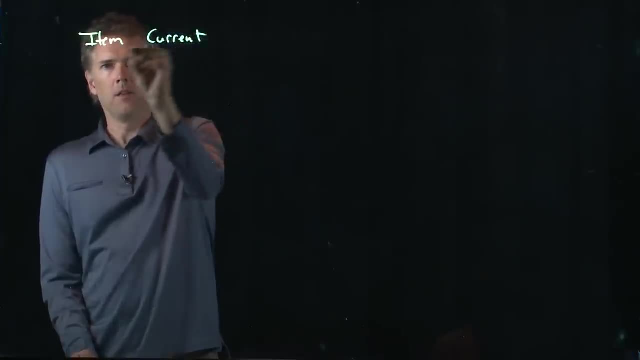 current and let's see if we can come up current and let's see if we can come up with some typical numbers here, for with some typical numbers here, for with some typical numbers here for different items, how much current they're. different items, how much current they're. 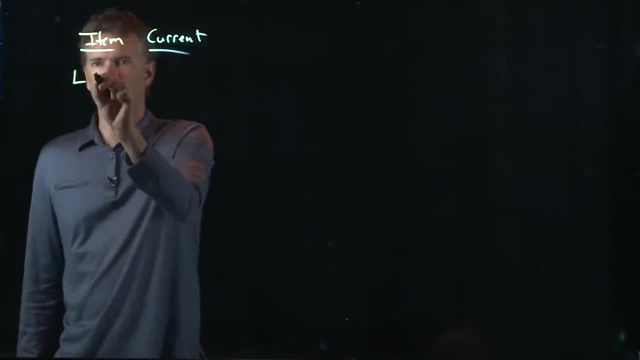 different items how much current they're going to use. so let's say I have an LED going to use. so let's say I have an LED going to use. so let's say I have an LED. right if I turn on just a little red LED. right if I turn on just a little red LED. 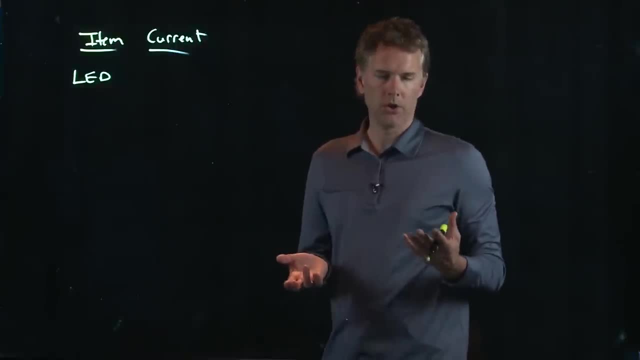 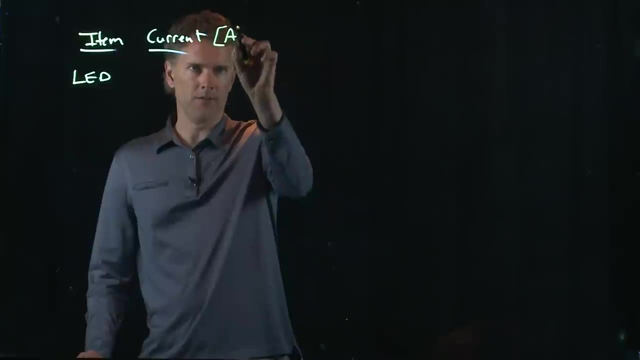 right if I turn on just a little red LED, green LED: how much current does it? green LED, how much current does it? green LED? how much current does it draw any ideas? and we're talking about in. draw any ideas and we're talking about in. draw any ideas and we're talking about in the scale of amps. right, that's our SI. 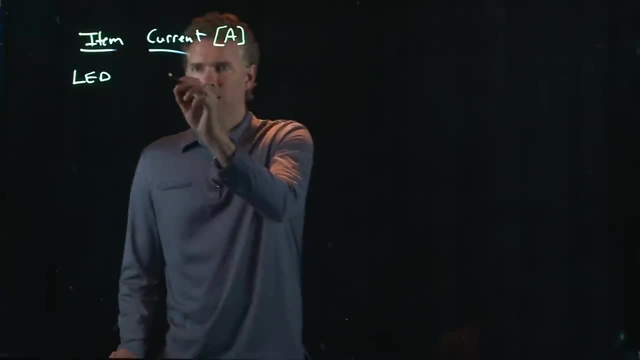 the scale of amps. right, that's our SI the scale of amps- right, that's our SI unit. well, it turns out a LED draw unit. well, it turns out a LED draw unit. well, it turns out a LED draw. somewhere around 10 milliamps, okay, somewhere around 10 milliamps, okay. 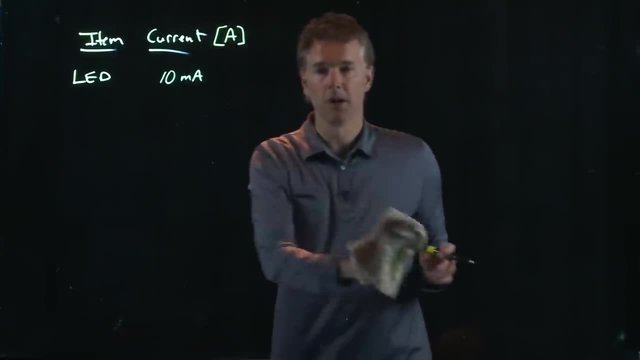 somewhere around 10 milliamps. okay, there's kind of a wide scale, but this is there's kind of a wide scale, but this is there's kind of a wide scale, but this is a typical number there for an LED 10- a typical number there for an LED 10. 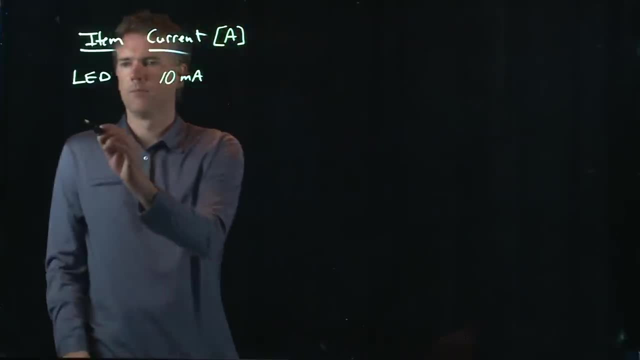 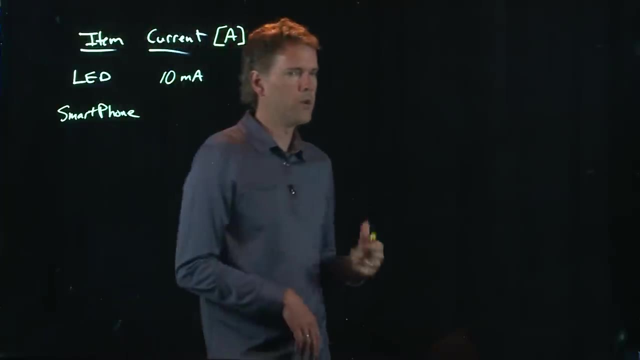 a typical number there for an LED: 10 milliamps. what about your smartphone milliamps? what about your smartphone milliamps? what about your smartphone? okay when you're walking around with. okay when you're walking around with. okay, when you're walking around with your smartphone. 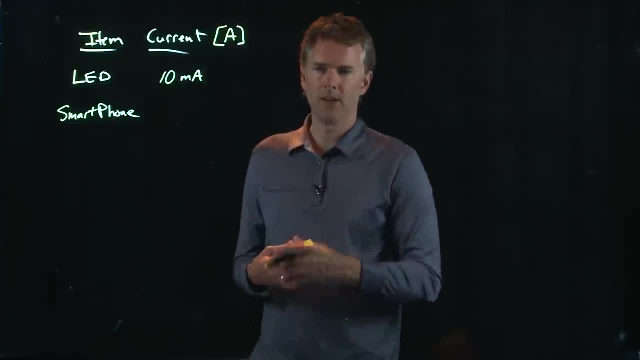 your smartphone, your smartphone. how much power does it draw? let's say how much power does it draw. let's say how much power does it draw. let's say: you're not even talking on the phone. you're not even talking on the phone. you're not even talking on the phone right now, it's just doing its normal. 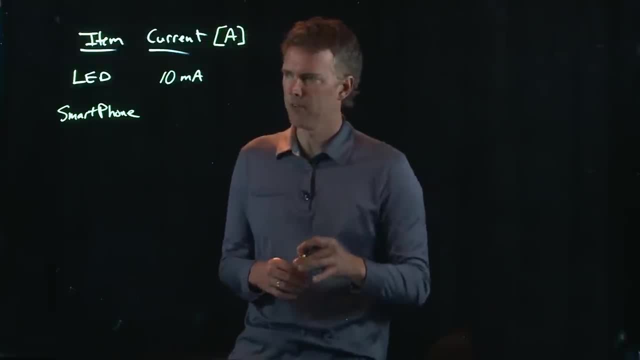 right now it's just doing its normal. right now it's just doing its normal thing, talking to the cellular towers thing, talking to the cellular towers thing, talking to the cellular towers doing some internal processing. a doing some internal processing, a doing some internal processing. a smartphone is about a hundred milliamps. 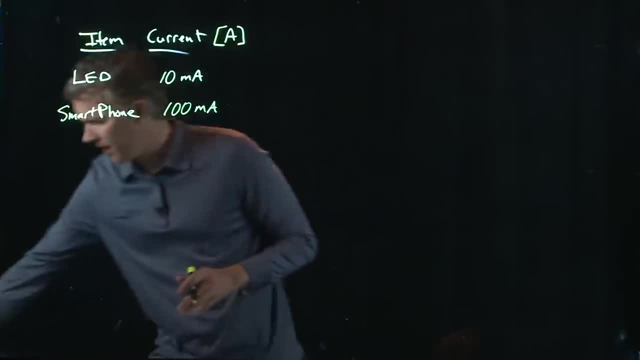 smartphone is about a hundred milliamps. smartphone is about a hundred milliamps. now that should make sense to you. now that should make sense to you. now that should make sense to you because we just talked about a double a, because we just talked about a double a. 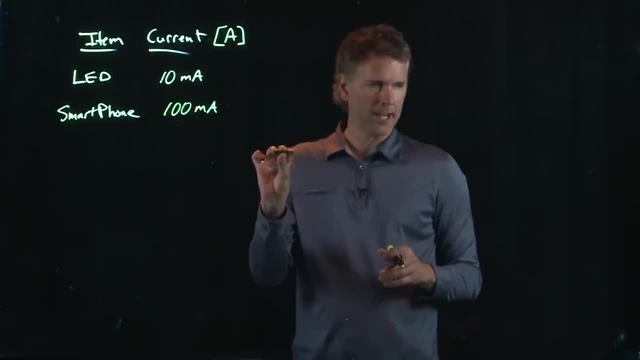 because we just talked about a double a battery right. a double a battery running battery right. a double a battery running battery right. a double a battery running a hundred milliamps will last about ten. a hundred milliamps will last about ten. a hundred milliamps will last about ten hours, your smartphone doing its normal. 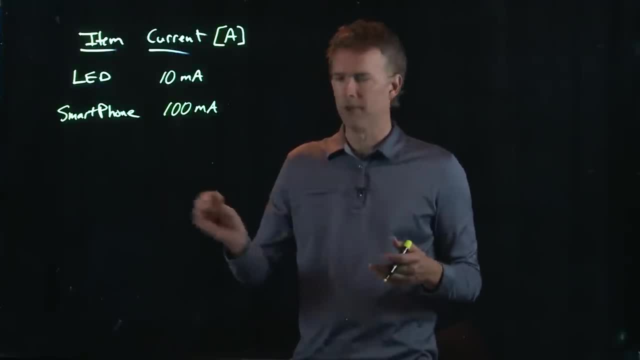 hours. your smartphone doing its normal hours. your smartphone doing its normal thing will last the full day, right ten thing will last the full day, right ten thing will last the full day, right, ten hours. or two batteries in there 20 hours. hours. or two batteries in there- 20 hours. 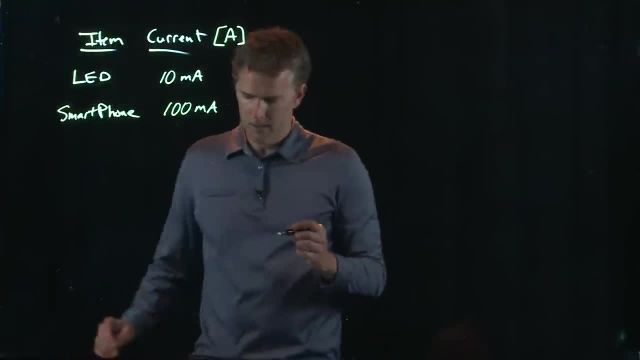 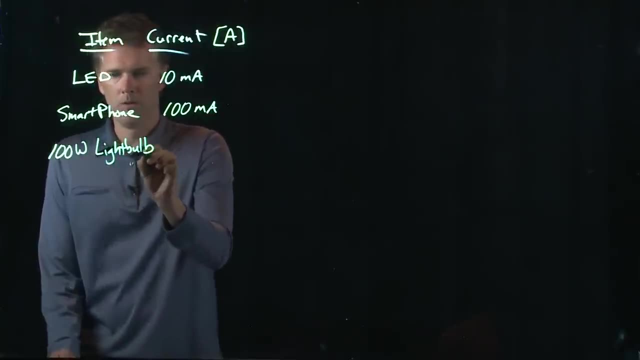 hours, or two batteries in there 20 hours. okay, what about a light bulb? let's say, okay, what about a light bulb? let's say, okay, what about a light bulb? let's say you go to Home Depot in the past. because you go to Home Depot in the past because you go to Home Depot in the past because you can't buy a hundred watt light bulb. you can't buy a hundred watt light bulb. you can't buy a hundred watt light bulb anymore. but let's say you go to Home anymore. but let's say you go to Home. 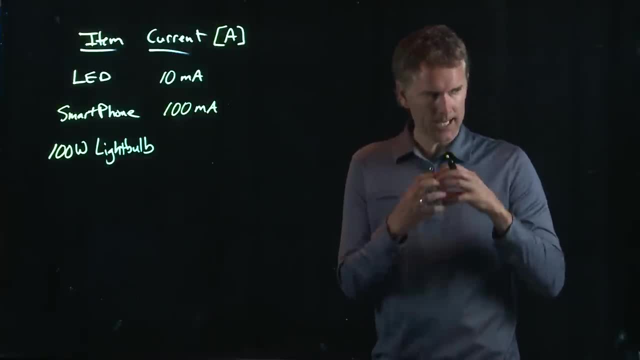 anymore. but let's say, you go to Home Depot- right, and you buy a hundred watt Depot- right, and you buy a hundred watt Depot- right and you buy a hundred watt light bulb- the incandescent light bulb, light bulb, the incandescent light bulb. light bulb- the incandescent light bulb, not the new compact fluorescence, not the. 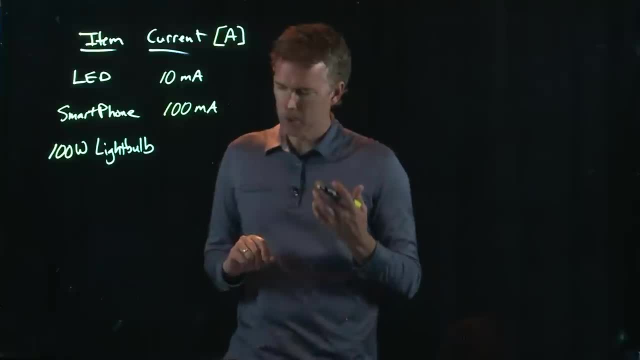 not the new compact fluorescence, not the, not the new compact fluorescence, not the new LED. you buy a normal hundred watt new LED. you buy a normal hundred watt new LED. you buy a normal hundred watt light bulb. how much current does that light bulb? how much current does that? 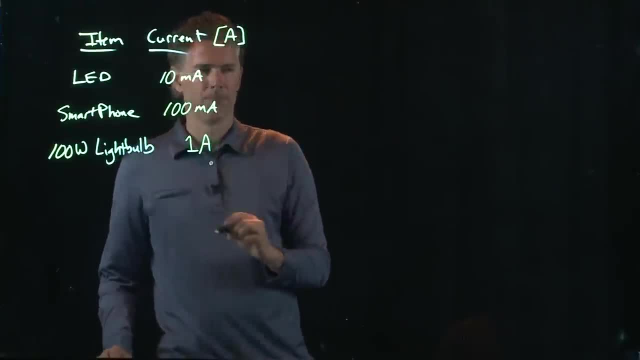 light bulb. how much current does that draw? it's about one amp, okay, so we've draw. it's about one amp. okay, so we've draw. it's about one amp. okay, so we've gone up by an order of 10 each time I gone up by an order of 10 each time I. 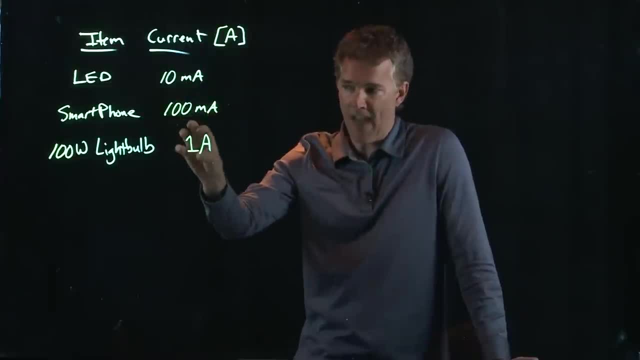 gone up by an order of 10. each time I got 10 milliamps, 100 milliamps. a got 10 milliamps, 100 milliamps. a got 10 milliamps, 100 milliamps, a thousand milliamps, which is one amp. 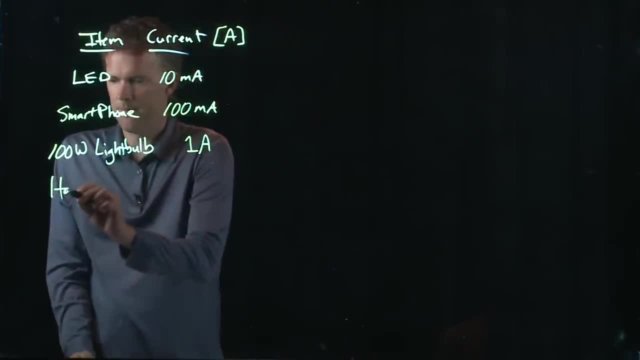 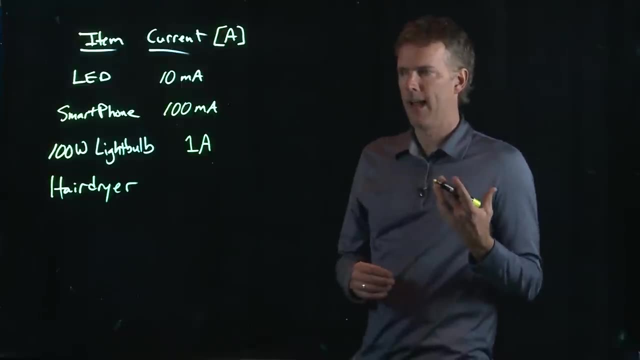 thousand milliamps, which is one amp. thousand milliamps, which is one amp. what about your hairdryer and when you? what about your hairdryer and when you? what about your hairdryer and when you fire up your hairdryer? how much current. 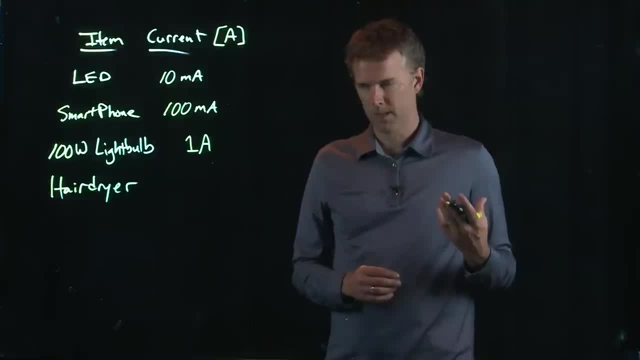 fire up your hairdryer. how much current fire up your hairdryer? how much current does it draw well? we talked about the. does it draw well? we talked about the: does it draw well? we talked about the power of the hairdryer right and when. power of the hairdryer right and when. power of the hairdryer right and when you turn on your hairdryer. you can you turn on your hairdryer, you can you turn on your hairdryer? you can actually see the lights dim in your. 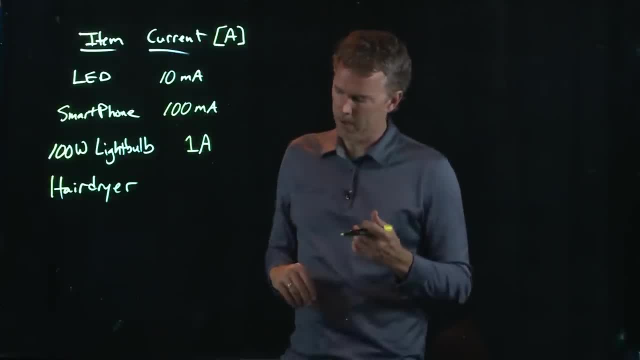 actually see the lights dim in your actually see the lights dim in your house a little bit. so it seems like it's house a little bit. so it seems like it's house a little bit. so it seems like it's got to be considerably more than a. 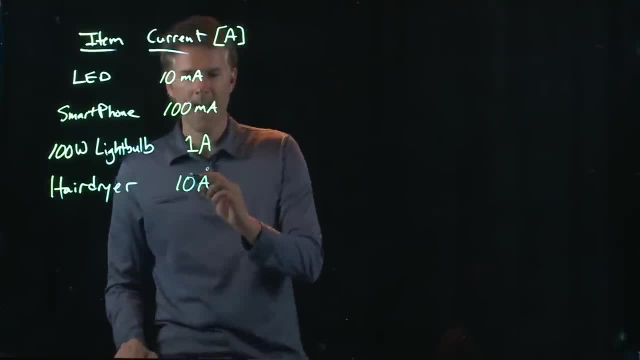 got to be considerably more than a, got to be considerably more than a light bulb, and in fact it is. it's on the light bulb and in fact it is it's on the light bulb and in fact it is it's on the order of 10 amps. so look, we've already. 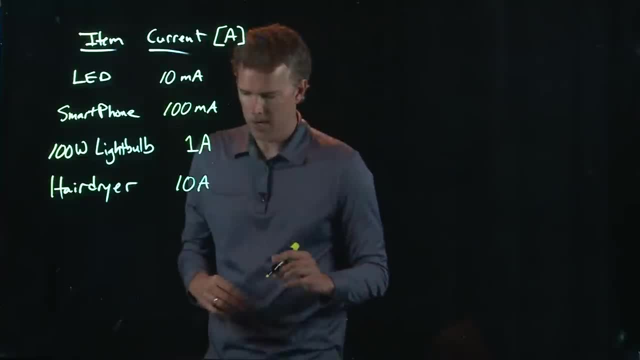 order of 10 amps. so look, we've already order of 10 amps. so look, we've already gone four orders of magnitude here up to gone. four orders of magnitude here up to gone. four orders of magnitude here up to a hairdryer. what about the total current? 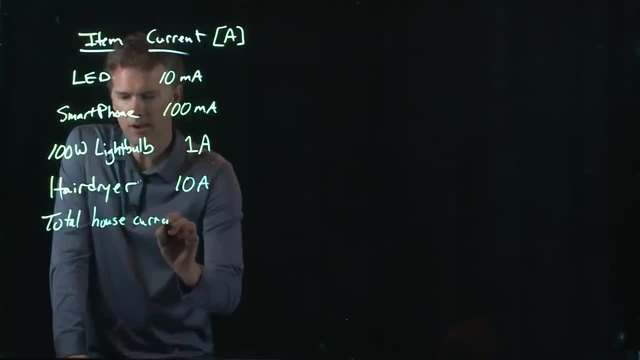 a hairdryer. what about the total current? a hairdryer. what about the total current? that's available coming into your house. that's available. coming into your house. that's available. coming into your house. right, there's a big power line on the right. there's a big power line on the. 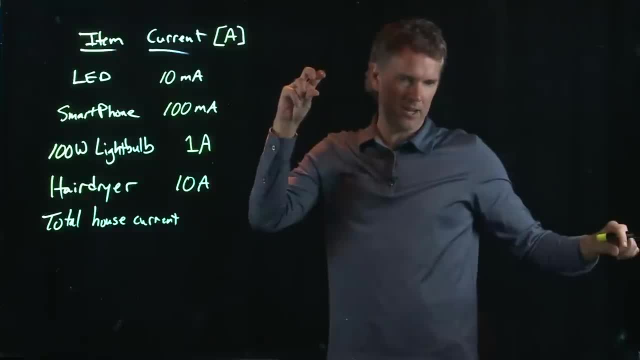 right, there's a big power line on the telephone pole. there's a big metal wire telephone pole. there's a big metal wire telephone pole. there's a big metal wire that comes down to your house and there that comes down to your house and there that comes down to your house and there is some amount of current that is. 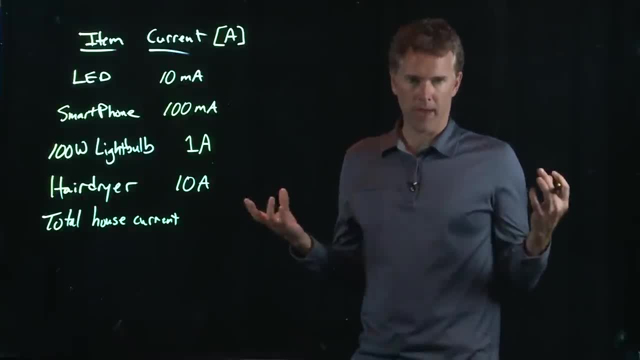 is some amount of current, that is is some amount of current that is available to your house, and that's it if available to your house, and that's it if available to your house, and that's it. if you draw more than that the electricity, you draw more than that, the electricity. 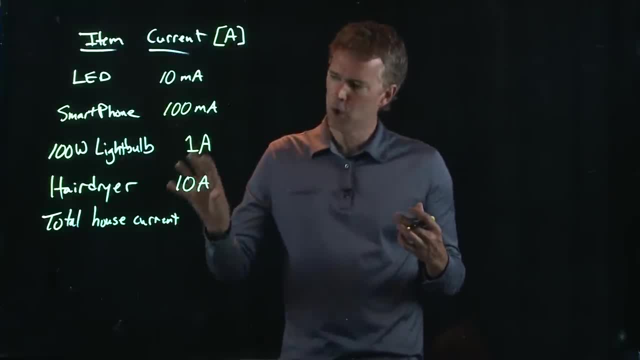 you draw more than that, the electricity company is going to have a problem with company, is going to have a problem with company, is going to have a problem with you. so how much is that total house you? so how much is that total house you? so how much is that total house current available? well, it's basically. 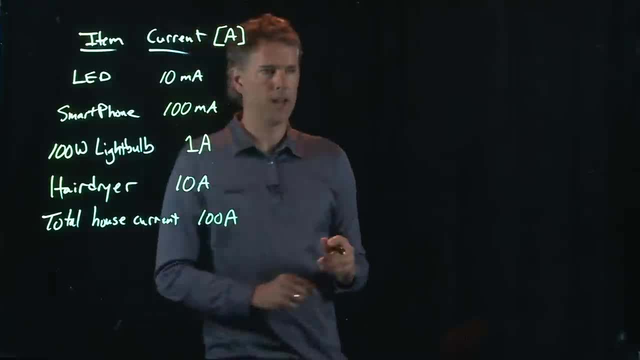 current available. well, it's basically current available. well, it's basically another factor of ten a hundred amps. another factor of ten a hundred amps. another factor of ten a hundred amps. okay when you go out in the morning and okay when you go out in the morning, and 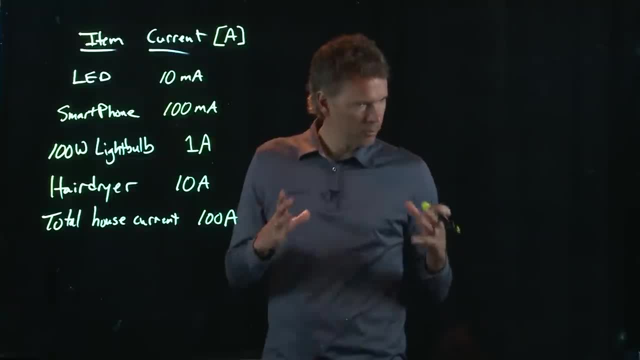 okay, when you go out in the morning and you start your car, there's a 12-volt. you start your car, there's a 12-volt. you start your car, there's a 12-volt battery in there and there's cables. battery in there and there's cables. 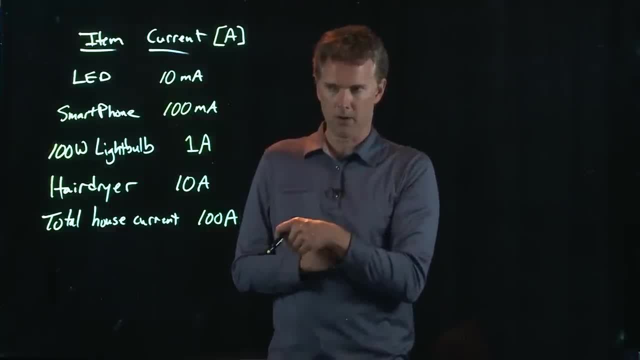 battery in there and there's cables that are connected to the starter motor, that are connected to the starter motor, that are connected to the starter motor in your car. and when you turn the in your car and when you turn the in your car and when you turn the ignition, what happens is it powers up the. 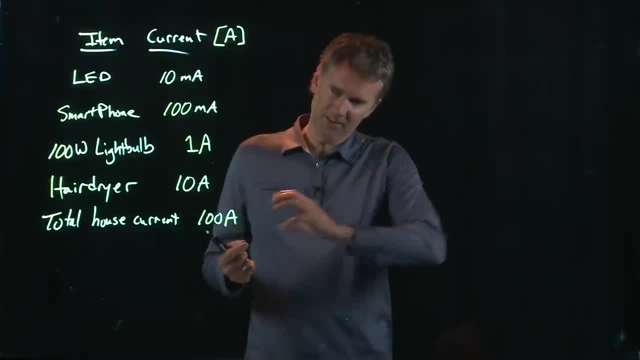 ignition. what happens is it powers up the ignition. what happens is it powers up the starter motor, that starter motor starter motor. that starter motor starter motor. that starter motor pushes against a gear that attaches to, pushes against a gear that attaches to, pushes against a gear that attaches to your engine and that electric motor. 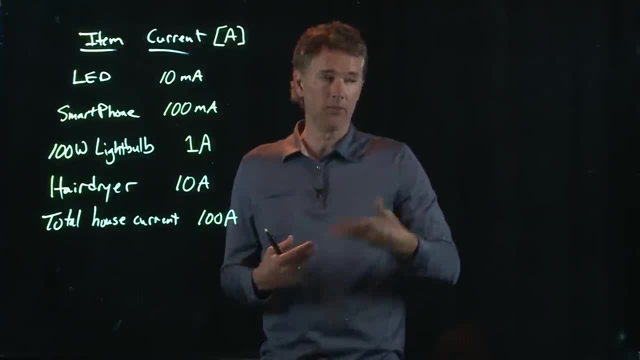 your engine and that electric motor, your engine and that electric motor actually spins your whole engine for a, actually spins your whole engine for a, actually spins your whole engine for a little bit until the engine starts, little bit. until the engine starts little bit, until the engine starts firing and the gas takes over, okay, and 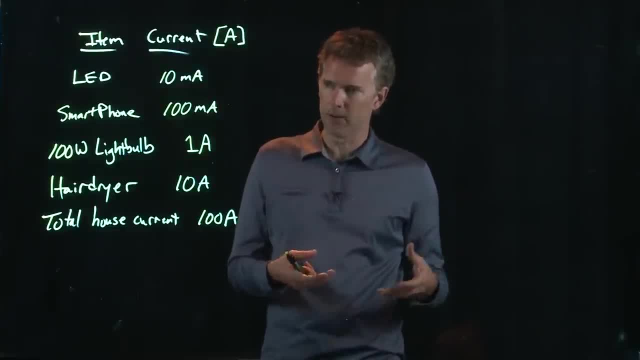 firing and the gas takes over, okay, and firing and the gas takes over, okay. and then the thing retracts, and then the, then the thing retracts, and then the, then the thing retracts, and then the electric motor just sits there, idle. electric motor just sits there, idle. 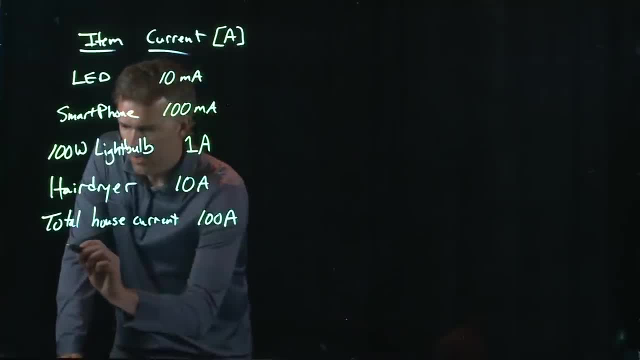 electric motor just sits there, idle, until you need to start the car again, until you need to start the car again, until you need to start the car again, but, but. but during that start, the battery has to provide. the battery has to provide, the battery has to provide a lot of current. 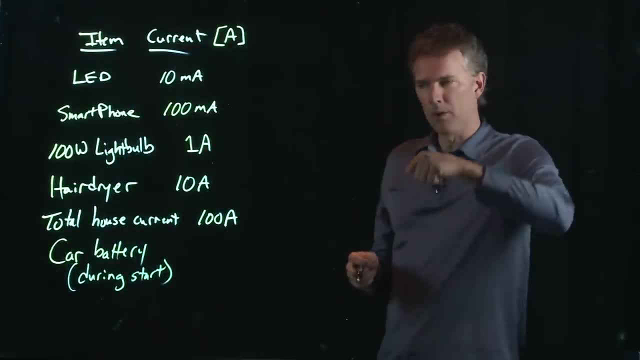 a lot of current, a lot of current, okay, okay, okay. and you know this right because if- and you know this right because if- and you know this right because if you're sitting there holding the key and you're sitting there holding the key and you're sitting there holding the key and your car is not starting, 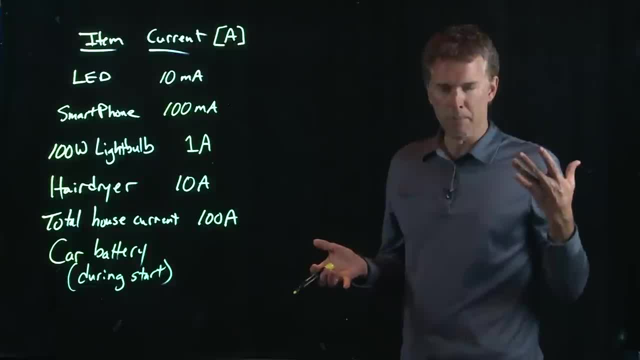 your car is not starting. your car is not starting. you can only do that for a few minutes. you can only do that for a few minutes. you can only do that for a few minutes before your battery just drains, before your battery just drains, before your battery just drains. doesn't work anymore, right, so you're. 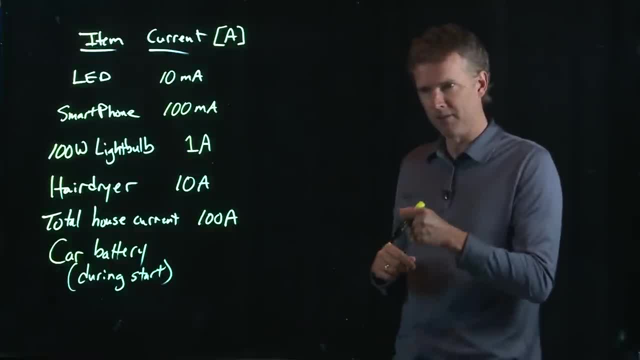 doesn't work anymore, right, so you're doesn't work anymore, right so you're hoping you're crossing your fingers. come hoping you're crossing your fingers. come hoping you're crossing your fingers. come on, start on this one. i know this is on. start on this one. i know this is. 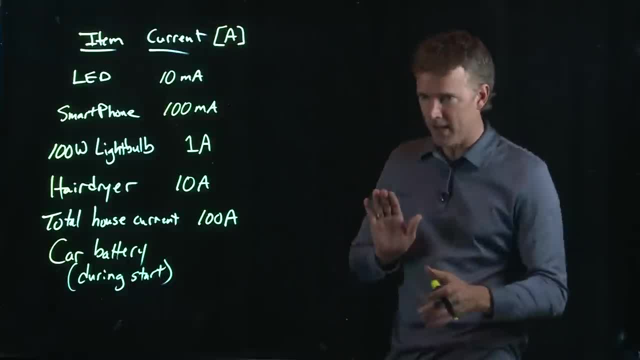 on start on this one. i know this is going to be it. then you try and decide going to be it. then you try and decide going to be it. then you try and decide: should i push real hard on the? should i push real hard on the? should i push real hard on the accelerator or not? you know this whole. 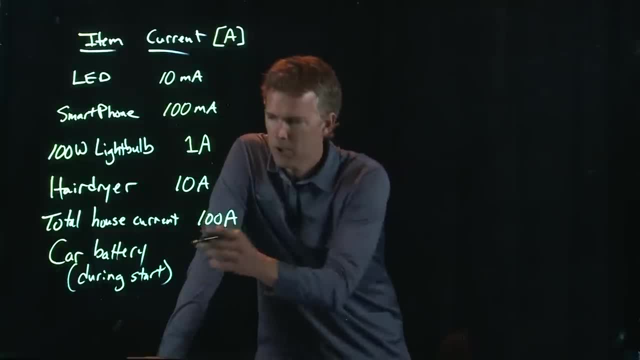 accelerator or not? you know this whole accelerator or not? you know this whole science of flooding the engine or not, science of flooding the engine or not, science of flooding the engine or not. how much current is available during the. how much current is available during the. how much current is available during the start? 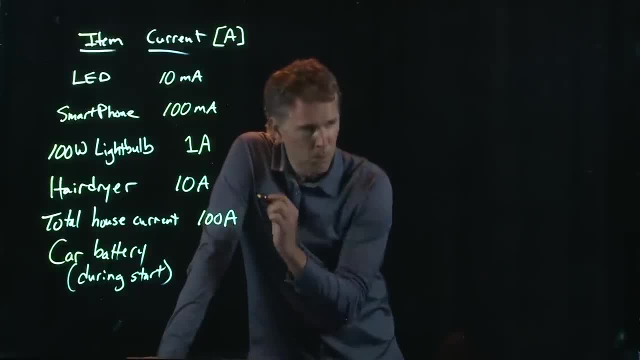 start, start of your car, of your car, of your car. is it really more than your whole house? is it really more than your whole house? is it really more than your whole house? current, current, current, it is it's like 300, it is it's like 300. 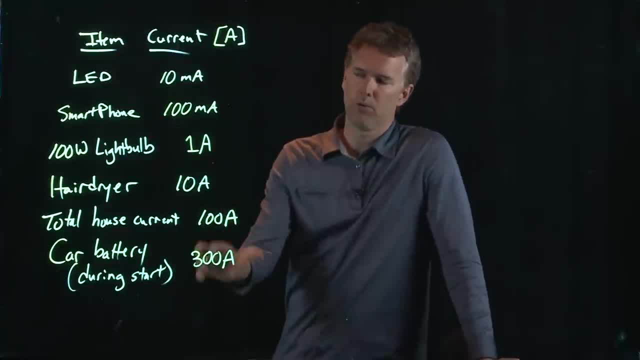 it is. it's like 300 amps. okay, they call this the cold amps. okay, they call this the cold amps. okay, they call this the cold cranking power of your battery and it cranking power of your battery and it cranking power of your battery, and it can be hundreds of amps. 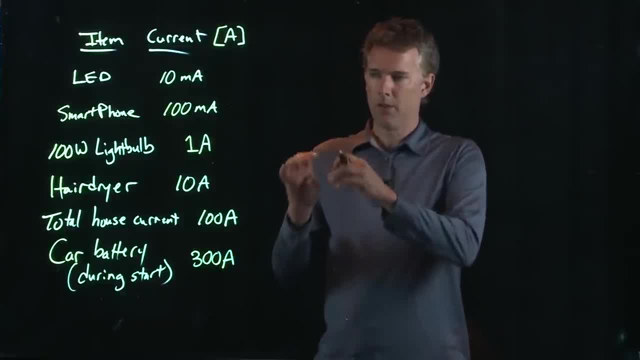 can be hundreds of amps, can be hundreds of amps. how do you know this well when you look. how do you know this well when you look? how do you know this well when you look at your car battery, those cables that at your car battery, those cables that. at your car battery. those cables that are attaching from the terminals of the, are attaching from the terminals of the, are attaching from the terminals of the battery down to the starter motor battery, down to the starter motor battery, down to the starter motor. those are big, heavy, thick cables. 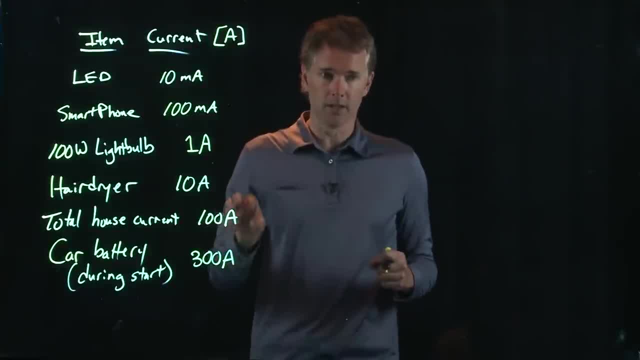 those are big, heavy, thick cables. those are big, heavy, thick cables. they need to be carrying a lot of. they need to be carrying a lot of. they need to be carrying a lot of current, a lot of electrons per second to current, a lot of electrons per second to. 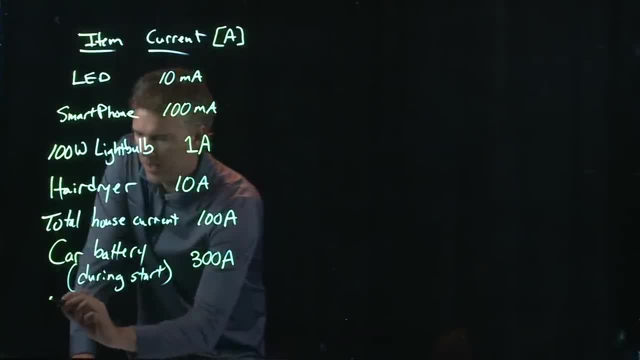 current a lot of electrons per second to get that car to start. get that car to start, get that car to start. okay, so that can be like 300 amps. okay, so that can be like 300 amps. okay, so that can be like 300 amps. all right, let's get to something really. 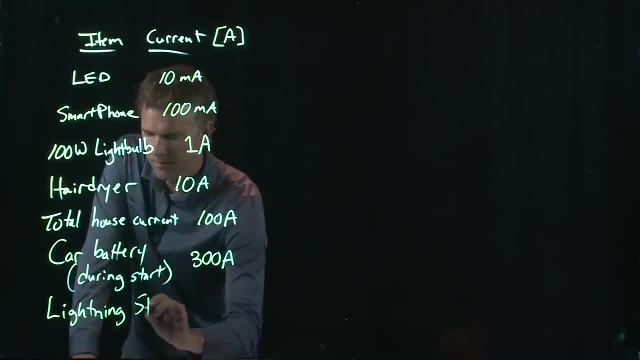 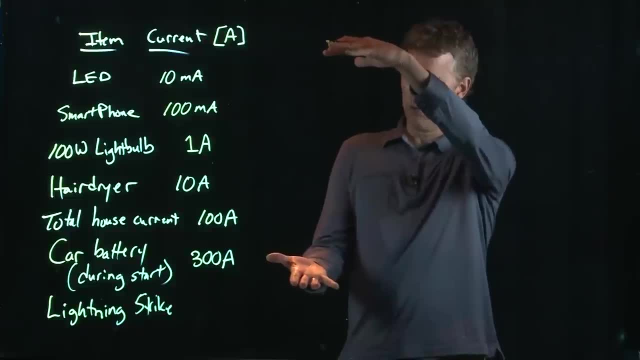 all right, let's get to something really. all right, let's get to something really: big, big, big lightning strike. a lightning strike is when there's a big a lightning strike is when there's a big a lightning strike is when there's a big voltage difference between the cloud and 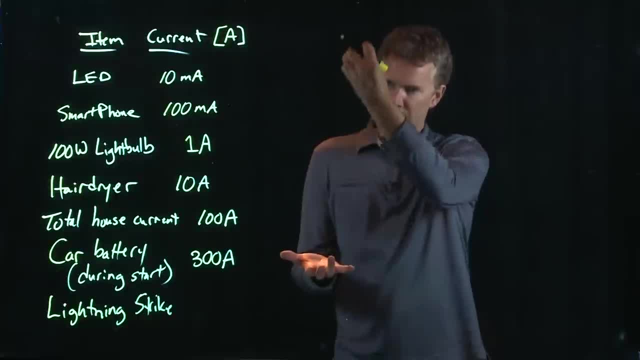 voltage difference between the cloud and voltage difference between the cloud and the ground. the ground, the ground. so much so that the electric field, so much so that the electric field, so much so that the electric field strips the electrons off of the, strips the electrons off of the. 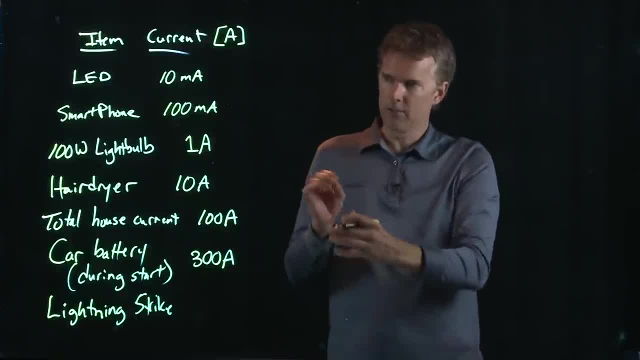 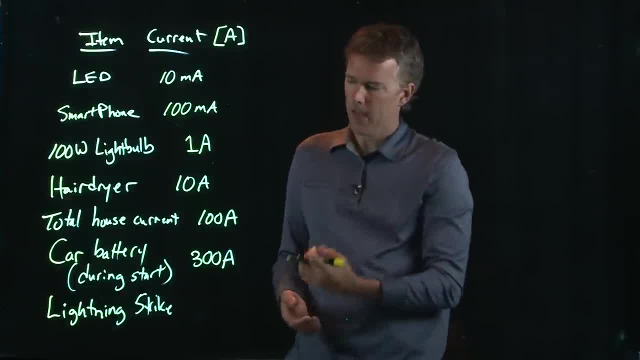 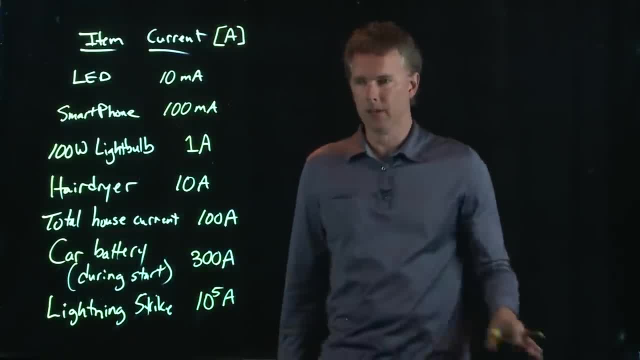 lightning strike, and that can be lightning strike, and that can be a hundred thousand amps, a hundred thousand amps, a hundred thousand amps, up to a million amps. okay, ten to the up to a million amps. okay, ten to the up to a million amps. okay, ten to the five, to ten to the six amps. 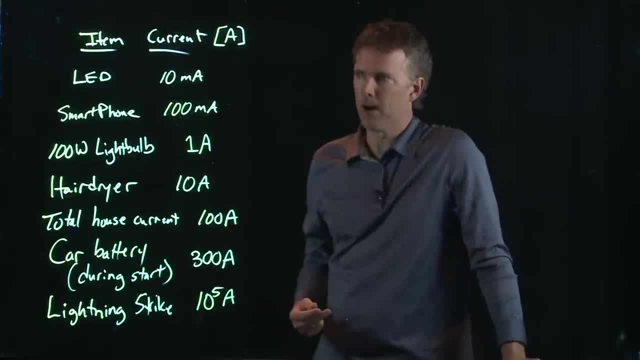 five to ten to the six amps. five to ten to the six amps. all right, so this is the sort of scale. all right, so this is the sort of scale. all right, so this is the sort of scale of things that you're talking about, of things that you're talking about. 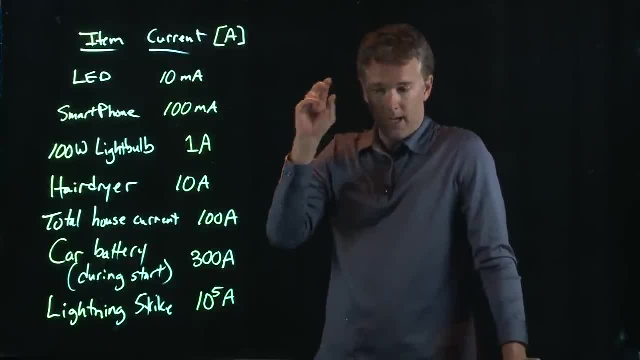 of things that you're talking about. we've got you know eight orders of. we've got you know eight orders of. we've got you know eight orders of magnitude. here it's magnitude, here it's magnitude. here it's interesting thinking about stuff like. interesting thinking about stuff like. 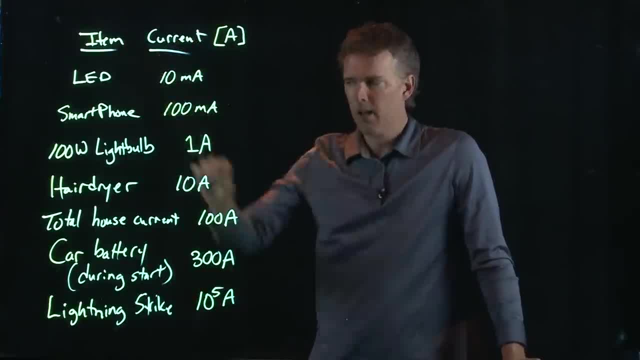 interesting thinking about stuff like leds right, how little current they draw. leds right, how little current they draw. leds right, how little current they draw compared to things like your hair dryer, compared to things like your hair dryer, compared to things like your hair dryer. and this is why there's this big push. 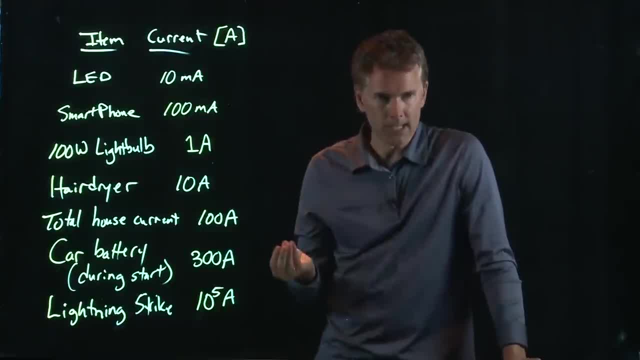 and this is why there's this big push. and this is why there's this big push for led lighting. okay, because led lights for led lighting okay, because led lights for led lighting. okay, because led lights just draw a lot less current and still just draw a lot less current and still. just draw a lot less current and still produce the same amount of light. produce the same amount of light. produce the same amount of light. a 100 watt light bulb- an incandescent. a 100 watt light bulb- an incandescent. a 100 watt light bulb- an incandescent light bulb. 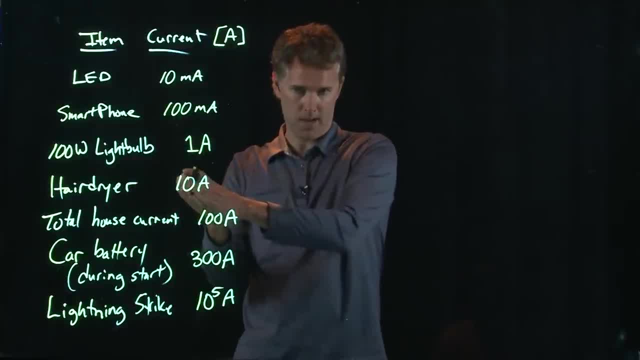 light bulb. light bulb is not very good at converting electric is not very good at converting electric is not very good at converting electric power into optical power, whereas power into optical power, whereas power into optical power, whereas something like an led is much more, something like an led is much more. 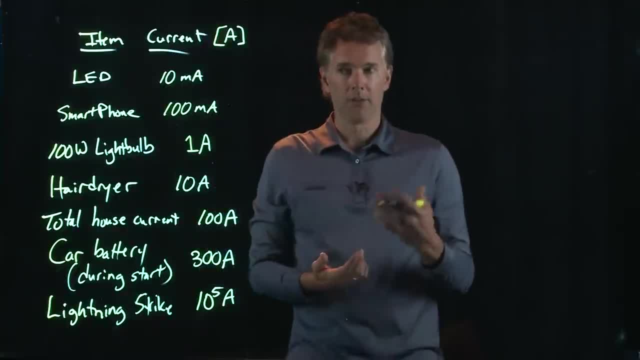 something like an led is much more efficient at converting electrical power, efficient at converting electrical power, efficient at converting electrical power into optical power, and so now you should into optical power, and so now you should into optical power, and so now you should all be buying led bulbs when you go to all be buying led bulbs. when you go to, all be buying led bulbs. when you go to home depot: right, buy the led bulb. and home depot right buy the led bulb. and home depot right buy the led bulb. and it'll say, oh, it's a 75 watt equivalent. 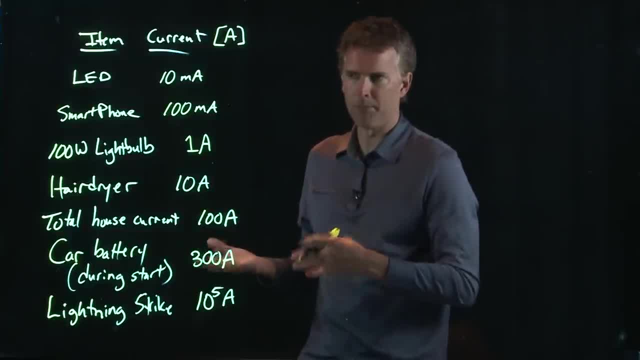 it'll say, oh, it's a 75 watt equivalent. it'll say, oh, it's a 75 watt equivalent and it only uses 7 watts, something like, and it only uses 7 watts, something like, and it only uses 7 watts, something like that. okay, it's like 10 times as. 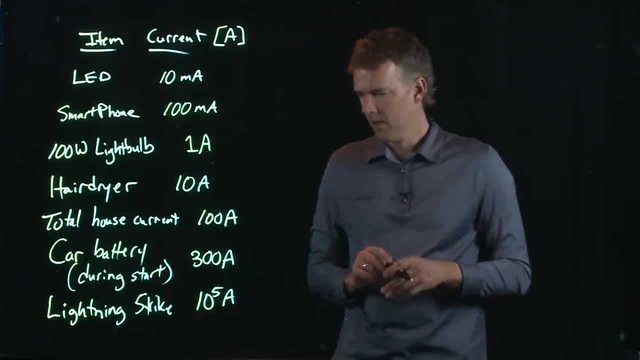 that okay, it's like 10 times as that. okay, it's like 10 times as efficient as an incandescent light bulb. efficient as an incandescent light bulb. efficient as an incandescent light bulb- all right when you think about types of. all right when you think about types of. 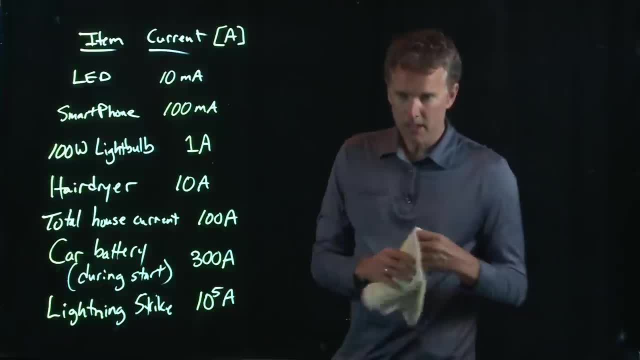 all right. when you think about types of current, you also need to think about: is current? you also need to think about is current. you also need to think about: is it DC or is it AC, and let's talk about it. DC or is it AC, and let's talk about. 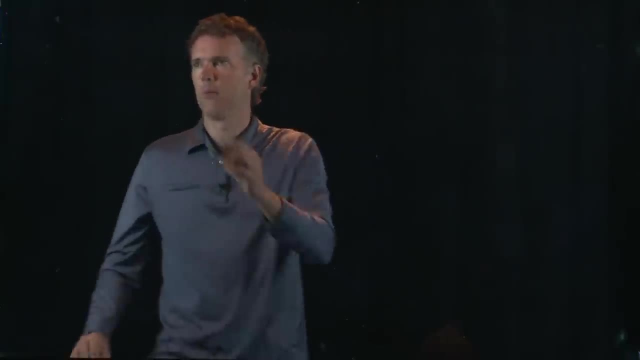 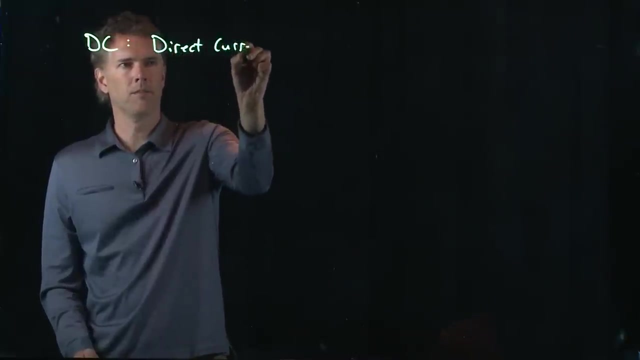 it DC or is it AC? and let's talk about that. okay, let's talk about DC, current DC- that okay, let's talk about DC, current DC- that okay, let's talk about DC. current DC means direct current versus AC. current means direct current versus AC. current means direct current versus AC current, which is alternating current, and they're. 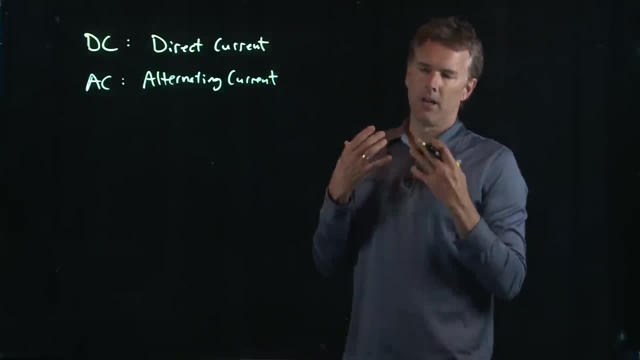 which is alternating current and they're which is alternating current and they're good. this goes back to the early days of good. this goes back to the early days of good. this goes back to the early days of electricity. people like Thomas Edison, electricity, people like Thomas Edison. 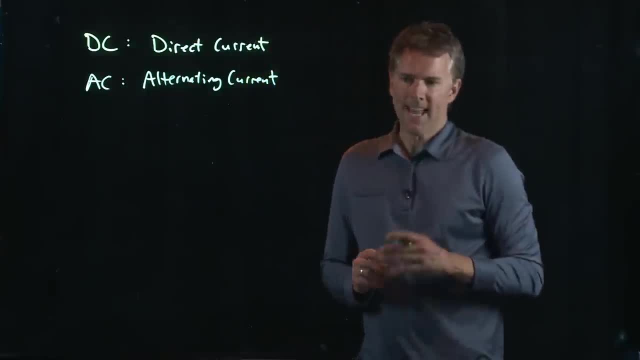 electricity, people like Thomas Edison and Ben Franklin and Ben Franklin and Ben Franklin and Tesla. and there was this big debate and Tesla. and there was this big debate and Tesla and there was this big debate about should we just power the United, about should we just power the United. 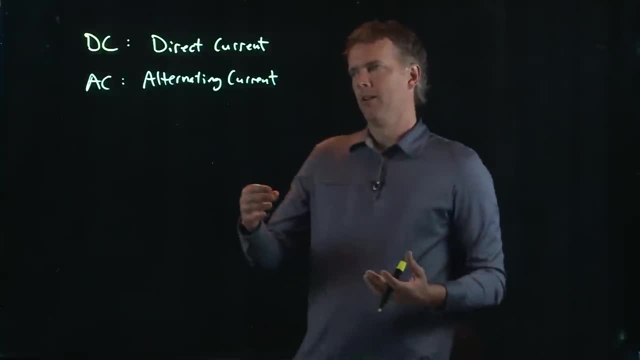 about? should we just power the United States by DC current or AC current? what States by DC current or AC current? what States by DC current or AC current? what one out of course was AC and when you one out of course was AC, and when you one out of course was AC and when you plug into the wall, it is AC current. but 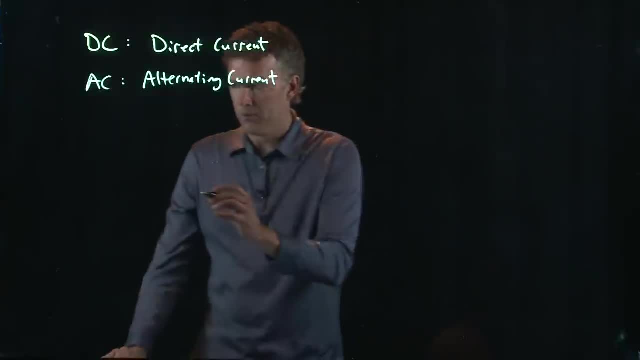 plug into the wall, it is AC current. but plug into the wall, it is AC current. but batteries are all direct current. so batteries are all direct current. so batteries are all direct current. so direct current just means the following: direct current just means the following: direct current just means the following: the current I doesn't change as a 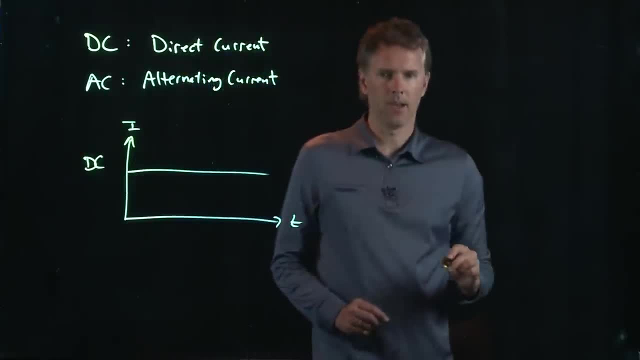 the current, I doesn't change as a. the current, I doesn't change as a function of time. it's that okay, it's all function of time. it's that okay, it's all function of time. it's that okay, it's all heading in one direction. AC current of. 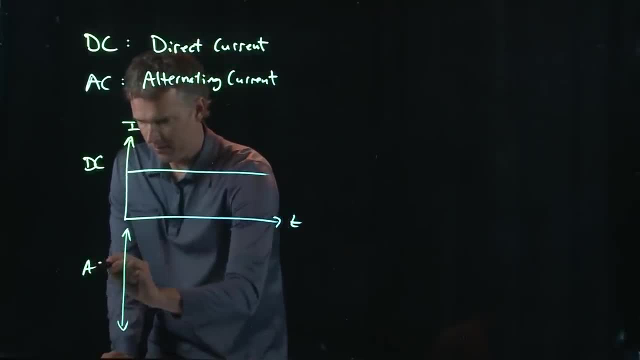 heading in one direction: AC current of heading in one direction. AC current of course means that it alternates, so as a course means that it alternates, so as a course means that it alternates, so as a function of time. AC current looks like. function of time. AC current looks like. 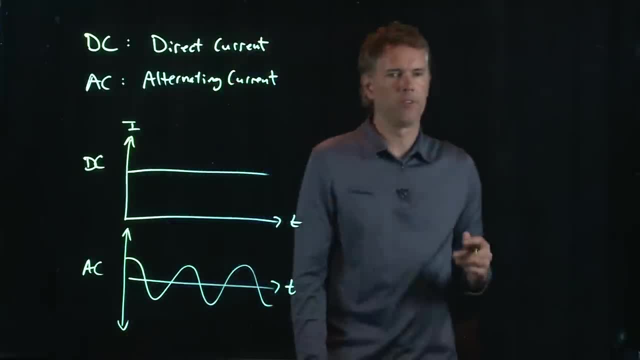 function of time. AC current looks like this: it's sort of sinusoidal. it's going this: it's sort of sinusoidal. it's going this: it's sort of sinusoidal: it's going positive for part of the time and then positive for part of the time, and then. 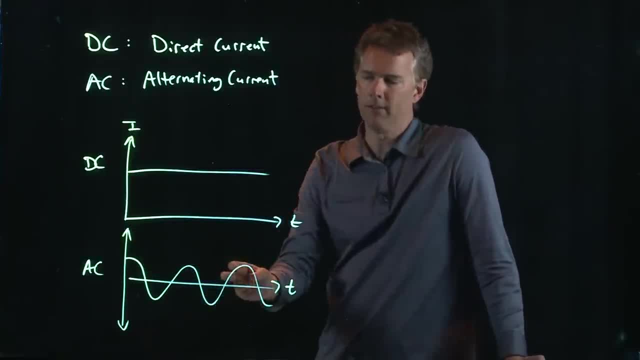 positive for part of the time and then it's going negative for part of the time. it's going negative for part of the time. positive and the negative- okay. so when positive and the negative, okay. so when positive and the negative, okay. so when you fire up your double-a battery, you 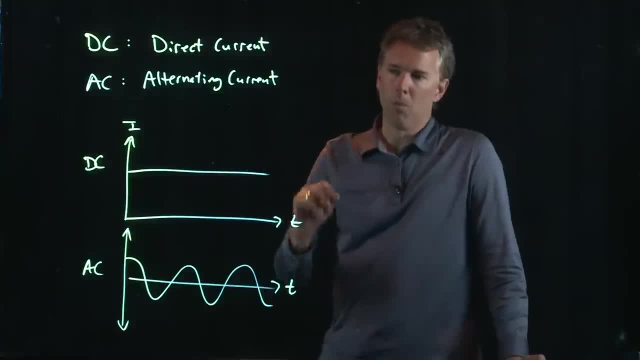 you fire up your double-a battery, you, you fire up your double-a battery, you get 1.5 volts and that's it. but when you get 1.5 volts and that's it. but when you get 1.5 volts and that's it. but when you plug something into the wall, you get 120. 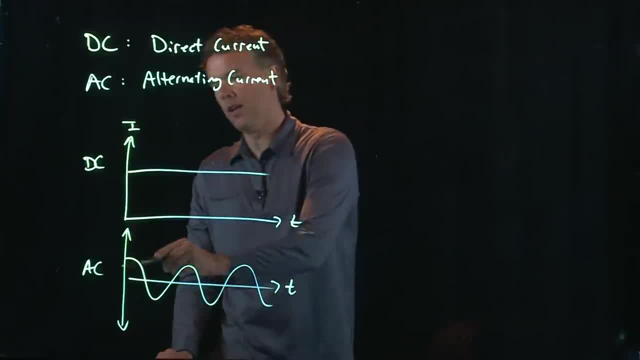 plug something into the wall, you get 120. plug something into the wall, you get 120 volts AC, and that AC means that it's volts AC and that AC means that it's volts AC and that AC means that it's going positive for part of the time. and 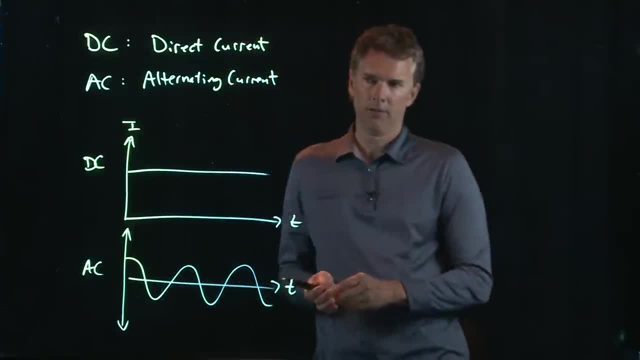 going positive for part of the time and going positive for part of the time, and then it's going negative for part of the, then it's going negative for part of the, then it's going negative for part of the time. positive and negative, and so the time positive and negative, and so the. 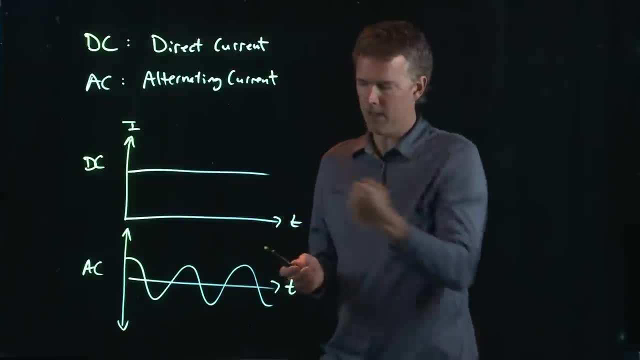 time positive and negative, and so the current is actually going this way and current is actually going this way, and current is actually going this way, and then that way, this way, and that's why then that way, this way, and that's why then that way, this way, and that's why it's pushing and pulling all the time. 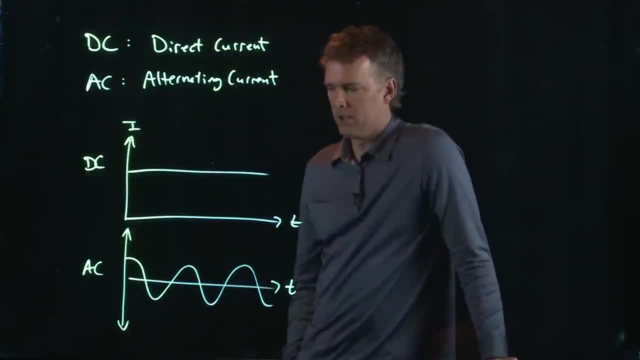 it's pushing and pulling all the time. it's pushing and pulling all the time, all right. how do we think about current? all right. how do we think about current, all right. how do we think about current in terms of other things that we like to, in terms of other things that we like to? 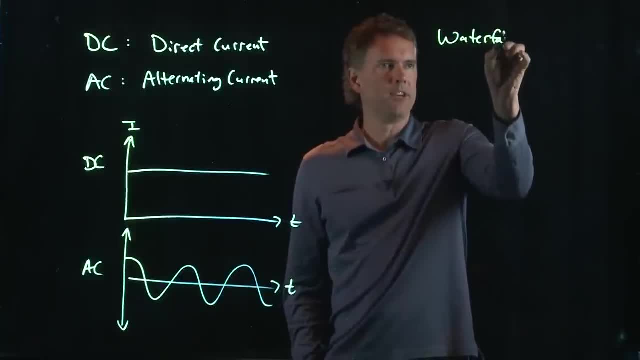 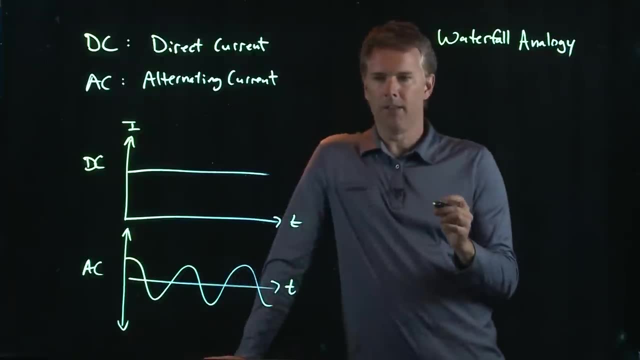 in terms of other things that we like to understand, like gravity well for DC. understand like gravity well for DC. understand like gravity well for DC, currents- at least there is a nice currents, at least there is a nice currents, at least there is a nice waterfall analogy, and it's this, if I 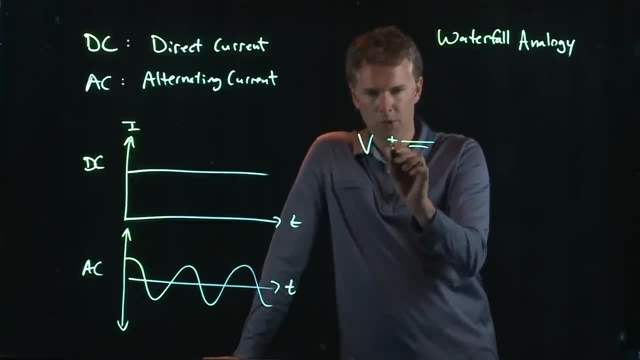 waterfall analogy and it's this if I waterfall analogy and it's this: if I take a battery and remember the long take a battery and remember the long take a battery and remember the long side is positive, the short side is side is positive, the short side is. 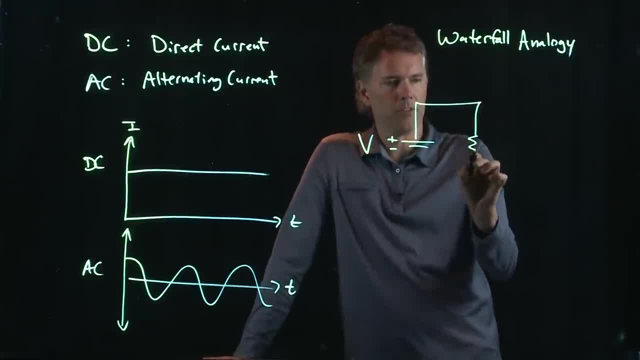 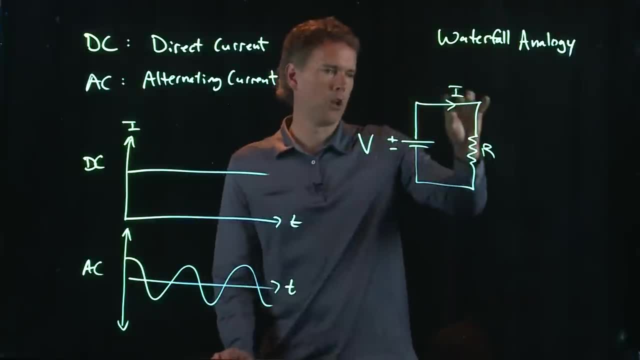 side is positive, the short side is negative and I hook it up to a resistor negative and I hook it up to a resistor negative and I hook it up to a resistor, then there is current that's going to, then there is current that's going to, then there is current that's going to run around that circuit. current I like. 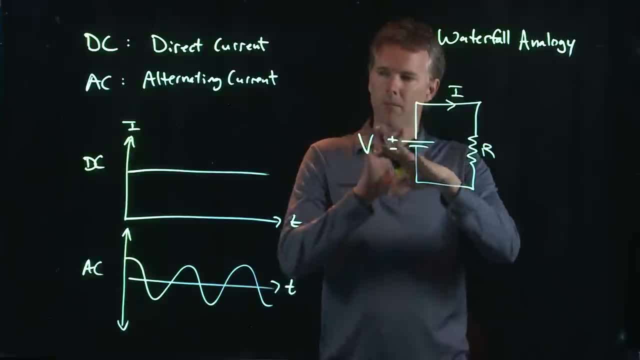 run around that circuit current. I like run around that circuit current. I like that. we know that it's electrons going that. we know that it's electrons going that. we know that it's electrons going the other way, but forget about that the other way, but forget about that. 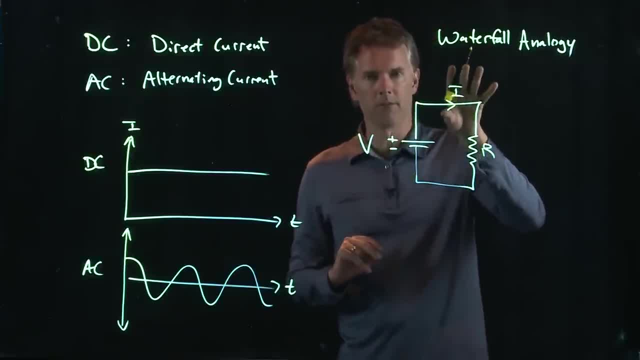 the other way. but forget about that. whenever you draw I, it's always referring. whenever you draw I, it's always referring. whenever you draw I, it's always referring to positive current. which way is the to positive current? which way is the to positive current? which way is the positive sign? this is just like a 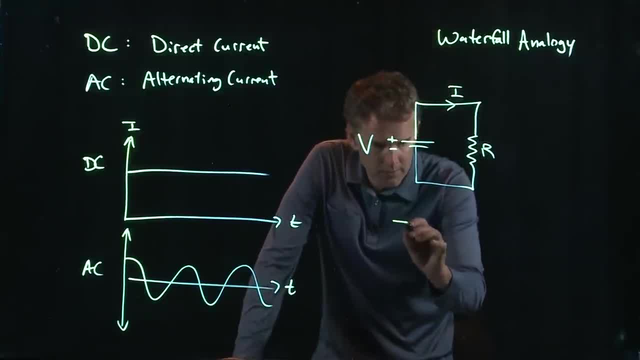 positive sign. this is just like a positive sign. this is just like a waterfall okay, and the analogy is the waterfall okay, and the analogy is the waterfall okay, and the analogy is the following: here is our waterfall and here following here is our waterfall and here following here is our waterfall and here comes the river and it goes over the. 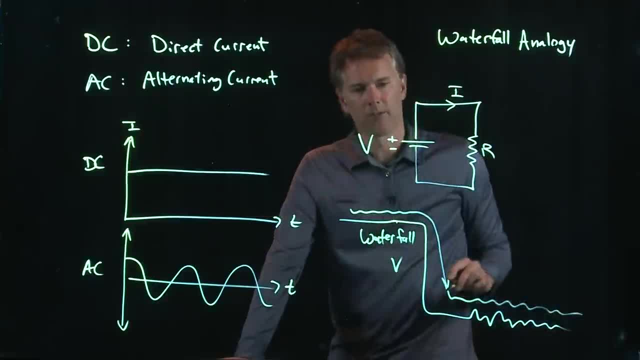 comes the river and it goes over the comes the river and it goes over the waterfall and then it goes down across waterfall and then it goes down across waterfall and then it goes down across the rocks. V is the height of the. the rocks V is the height of the. 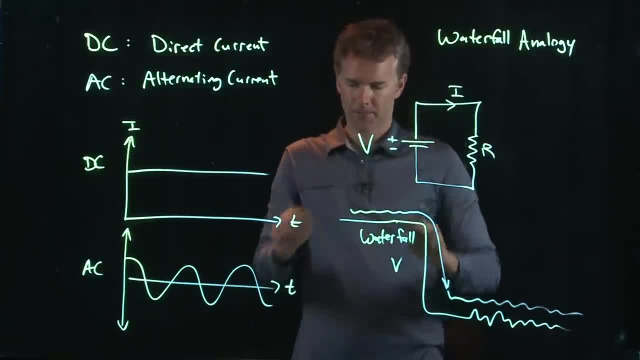 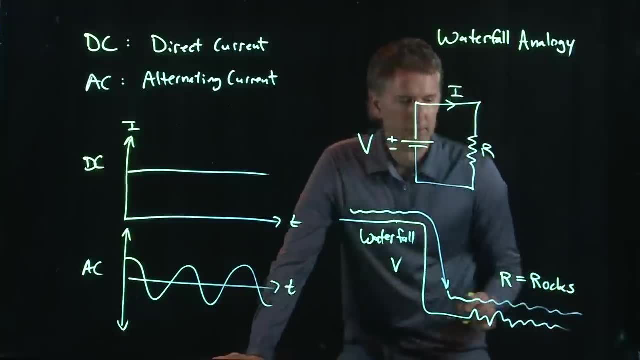 the rocks. V is the height of the waterfall. okay, that's the battery. R is waterfall. okay, that's the battery. R is waterfall. okay, that's the battery. R is the rocks. and what rocks do? is they try the rocks and what rocks do? is they try the rocks. and what rocks do is they try to slow down the current. they try to. 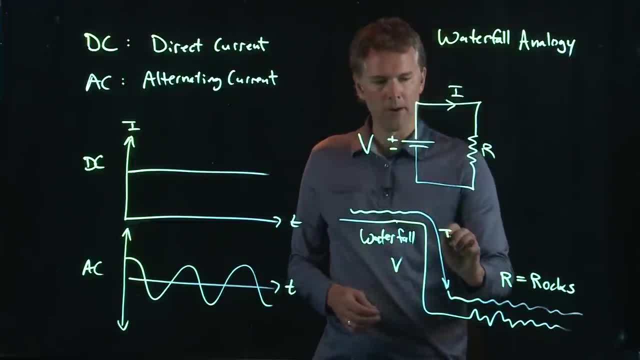 to slow down the current. they try to to slow down the current, they try to prevent the current. the water is of prevent the current. the water is of prevent the current. the water is, of course, the current, all right height, of course, the current, all right height of. 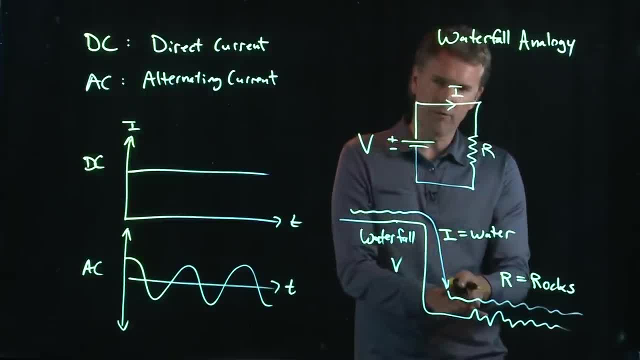 course, the current all right height of the waterfall is the battery. the waterfall is the battery. the waterfall is the battery. the amount of water flowing is the. the amount of water flowing is the. the amount of water flowing is the current. the rocks in the river, those are 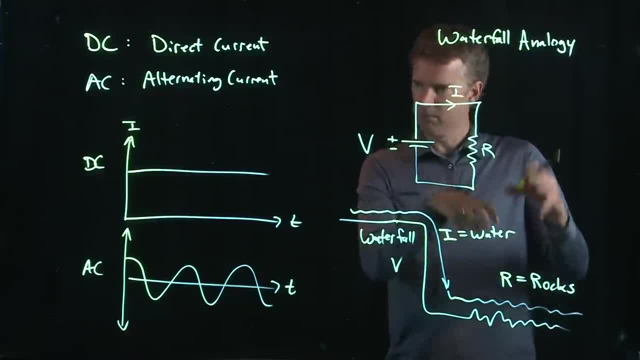 current the rocks in the river. those are current the rocks in the river. those are the resistance. put a bunch more rocks in the resistance. put a bunch more rocks in the resistance. put a bunch more rocks in there. it's going to agitate the water there. it's going to agitate the water. 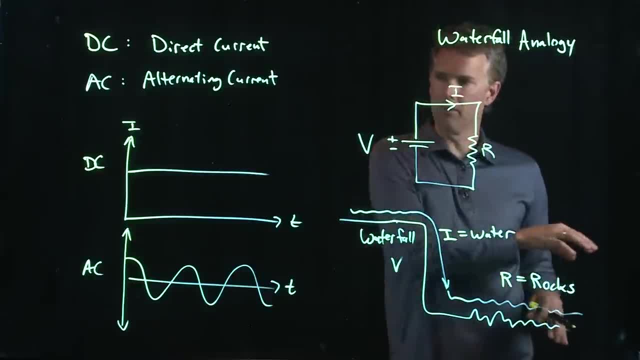 there. it's going to agitate the water and slow it down a whole bunch no rocks and slow it down a whole bunch no rocks and slow it down a whole bunch no rocks. the water is going to flow much more. the water is going to flow much more. 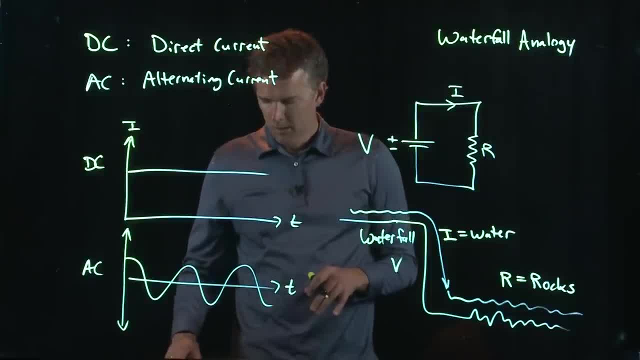 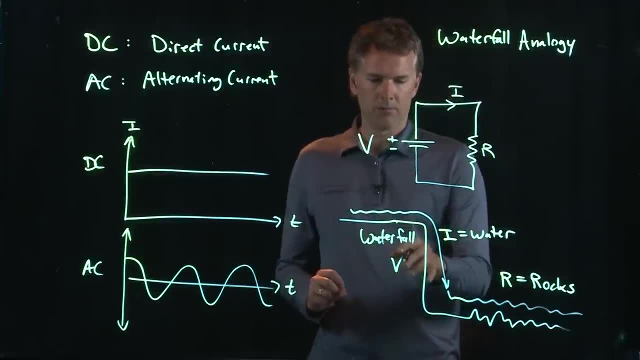 the water is going to flow much more smoothly. okay, so, when you think about a smoothly okay. so, when you think about a smoothly okay. so when you think about a battery- one thing that you might battery, one thing that you might battery, one thing that you might consider is: well, how do I recharge the? 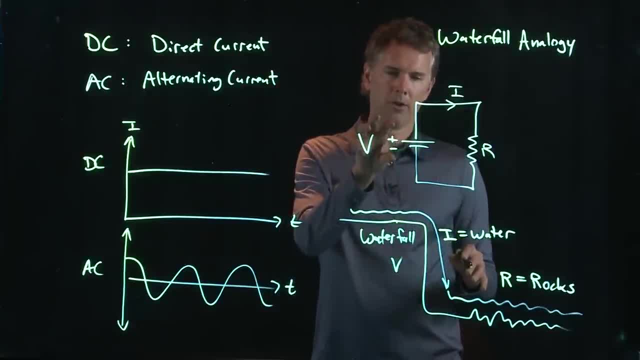 consider is well, how do I recharge the? consider is well, how do I recharge the battery? right, the battery in your battery. right, the battery in your battery. right, the battery in your smartphone drains. okay, I need to refill smartphone drains. okay, I need to refill smartphone drains. okay, I need to refill it. and that is the pumping station. 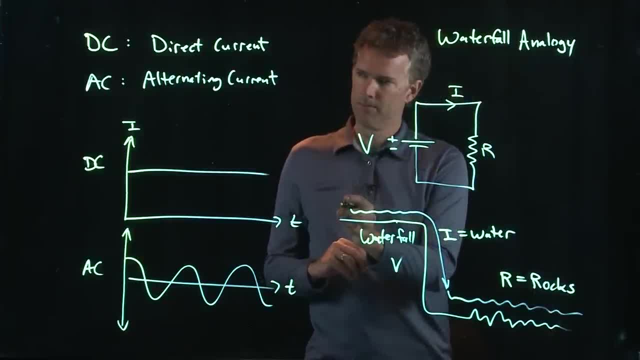 it and that is the pumping station. it and that is the pumping station that's going to pump the water back up. that's going to pump the water back up. that's going to pump the water back up to the top of the waterfall. all right, to the top of the waterfall, all right. 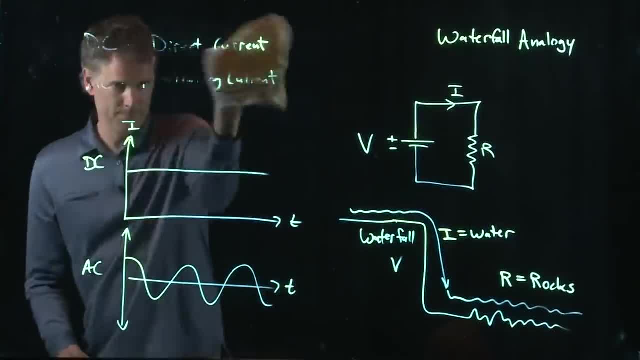 to the top of the waterfall. all right, any questions up to this point? you guys, any questions up to this point? you guys, any questions up to this point? you guys doing all right, okay. so one of your doing all right, okay. so one of your doing all right, okay. so one of your homework problems is number eighteen. 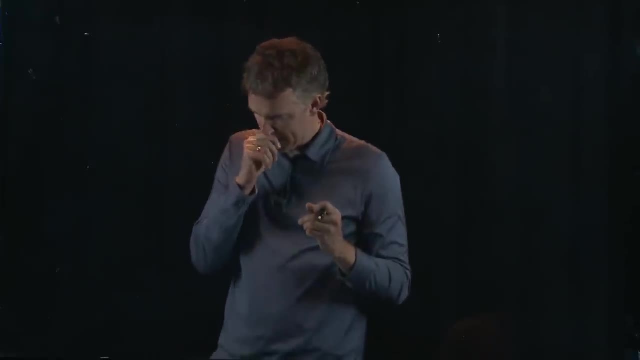 homework problems is number eighteen. homework problems is number eighteen, point oh one in your chapter, and also on point oh one in your chapter, and also on point oh one in your chapter, and also on mastering anytime. it has a number on mastering anytime. it has a number on. 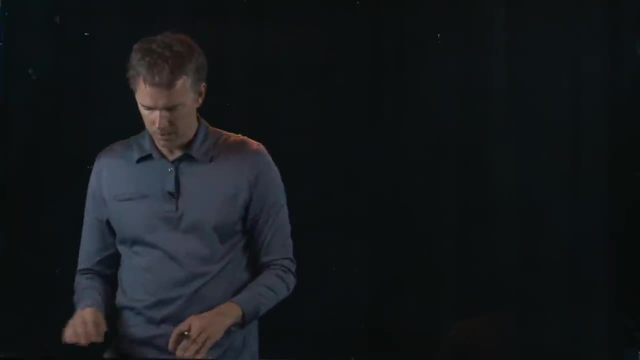 mastering. anytime it has a number on mastering that refers to problems out of mastering. that refers to problems out of mastering. that refers to problems out of the textbook. so let's look at eighteen, the textbook. so let's look at eighteen, the textbook. so let's look at eighteen. point, oh one. eighteen, two point, oh one. 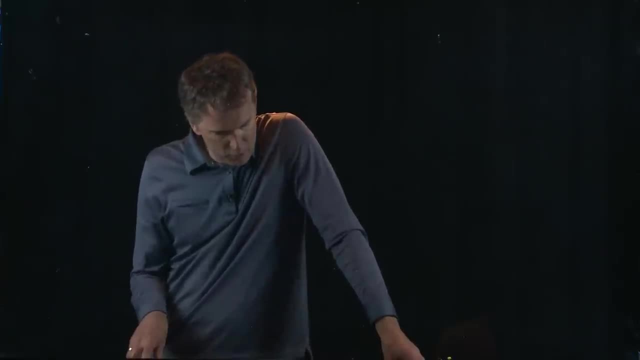 point. oh one. eighteen two point. oh one point. oh one. eighteen two point. oh one. says a current of one amp flows in a. says a current of one amp flows in a. says a current of one amp flows in a wire: how many electrons are flowing past wire? how many electrons are flowing past? 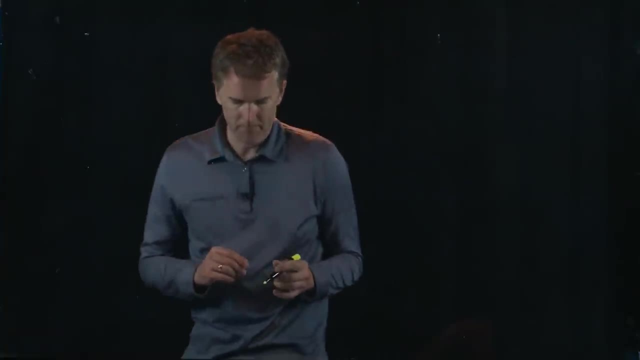 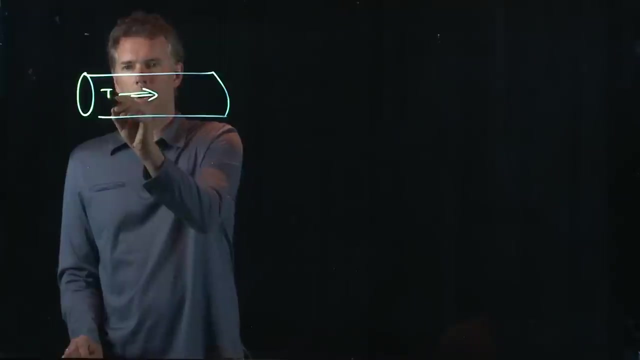 wire. how many electrons are flowing past any point in the wire per second? all any point in the wire per second, all any point in the wire per second. all right, here's our wire. we've got current right. here's our wire. we've got current right. here's our wire, we've got current I, and it tells us that I and we can use. 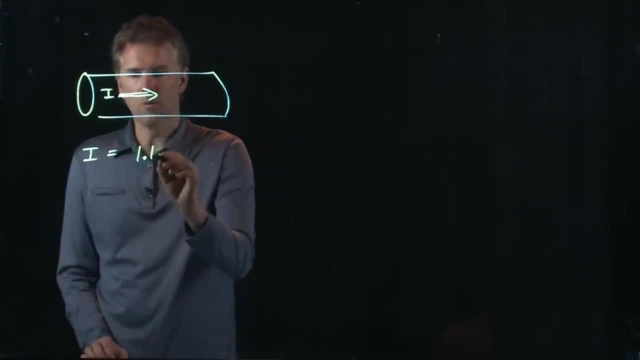 I and it tells us that I and we can use I and it tells us that I and we can use my numbers here just for fun is one. my numbers here, just for fun is one. my numbers here just for fun is one point one, zero amps. and it wants to know. 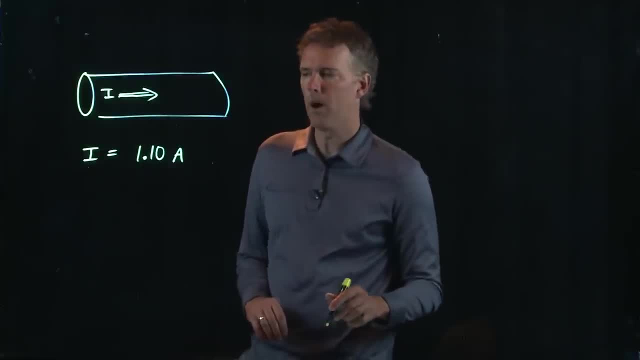 point one: zero amps. and it wants to know point one- zero amps. and it wants to know how many electrons are flowing past any. how many electrons are flowing past any. how many electrons are flowing past any point in the wire per second point in the wire per second? 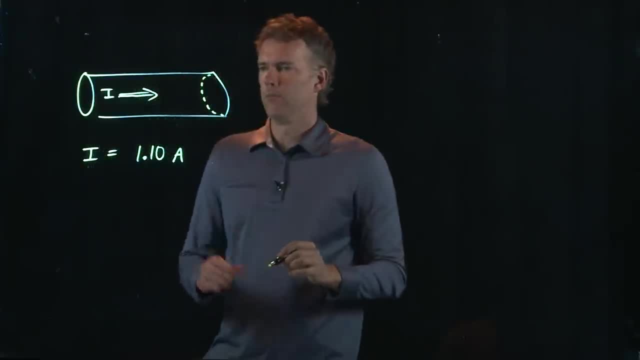 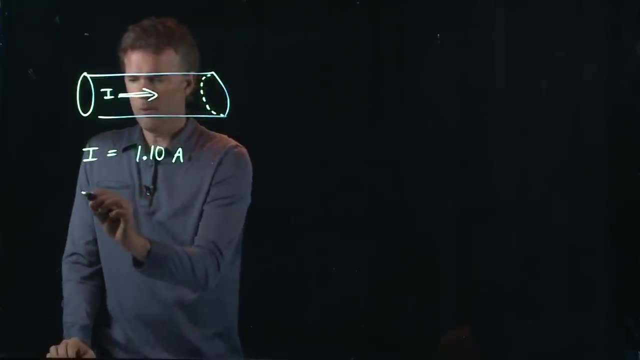 point in the wire per second, all right. pick a point in the wire and say, all all right. pick a point in the wire and say, all all right. pick a point in the wire and say, all right, how many electrons are right? how many electrons are right, how many electrons are flowing past it? well, we probably know that. 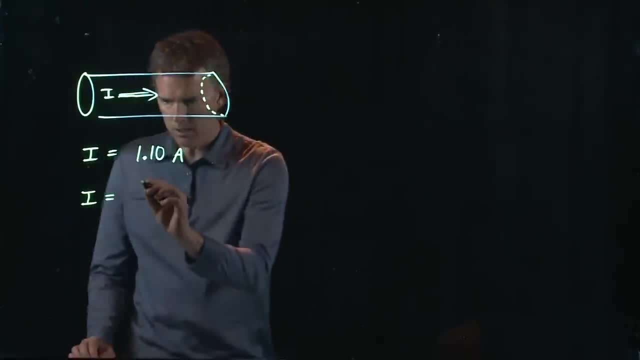 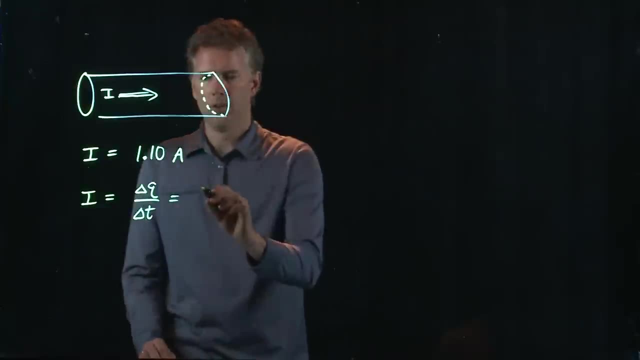 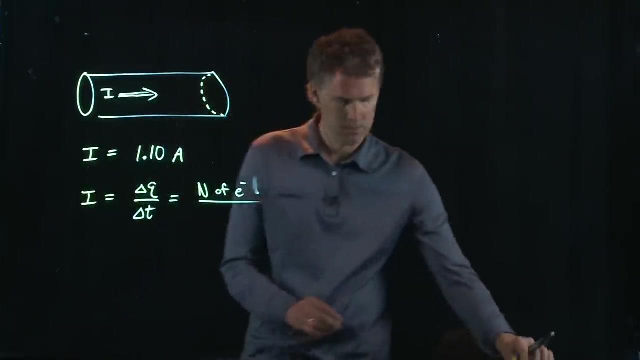 flowing past it. well, we probably know that. flowing past it. well, we probably know that. right, because I is Delta Q over Delta. right, because I is Delta Q over Delta. right, because I is Delta Q over Delta. T, which is number of electrons per T, which is number of electrons per 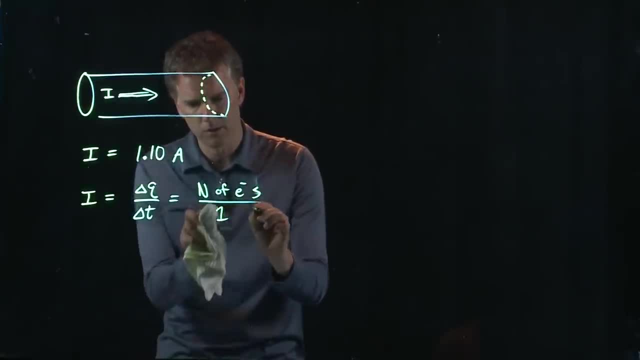 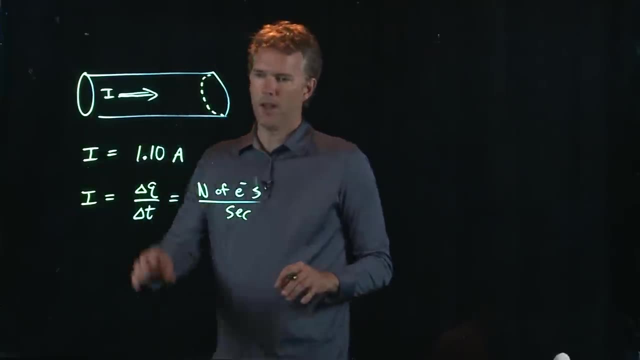 T, which is number of electrons per Delta T, which we can just call a second Delta T, which we can just call a second Delta T, which we can just call a second right. so all we have to do is convert, right. so all we have to do is convert. 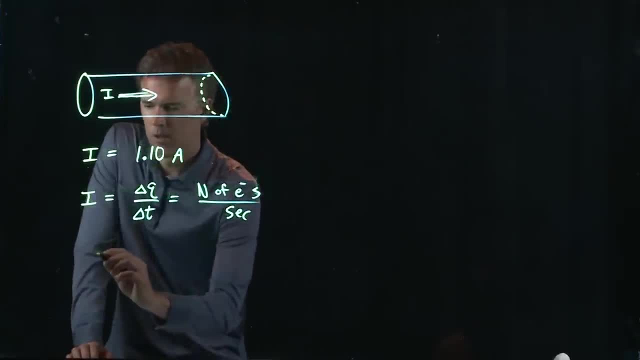 right, so all we have to do is convert 1.1 amps to electrons. 1.1 amps is 1.1, 1.1 amps to electrons. 1.1 amps is 1.1. 1.1 amps to electrons. 1.1 amps is 1.1 coulombs per second, and we just want to. 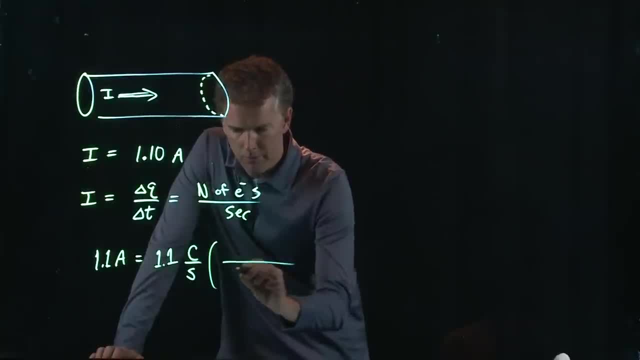 coulombs per second, and we just want to coulombs per second and we just want to convert coulombs to electrons. so like we convert coulombs to electrons, so like we convert coulombs to electrons, so like we said before, 1.6 times 10 to the minus 19. 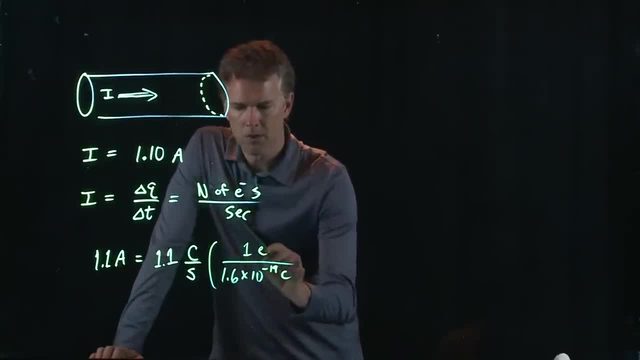 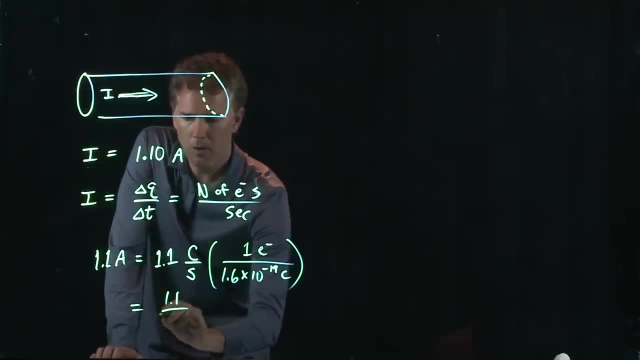 said before, 1.6 times 10 to the minus 19, said before 1.6 times 10 to the minus 19. coulombs is the charge of one electron, coulombs is the charge of one electron coulombs is the charge of one electron. and so we get 1.1 over 1.6 times 10 to. 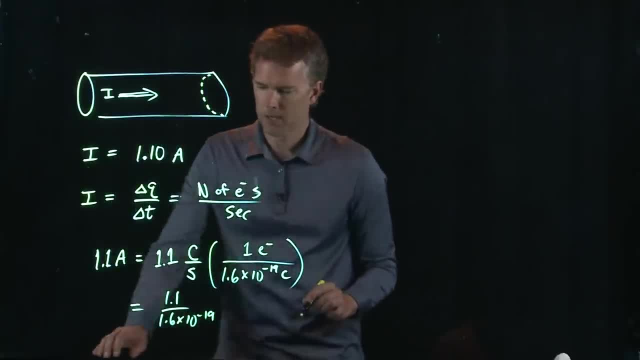 and so we get 1.1 over 1.6 times 10 to. and so we get 1.1 over 1.6 times 10 to the minus 19. somebody punch that into the minus 19. somebody punch that into the minus 19. somebody punch that into your calculator and tell me what you get. 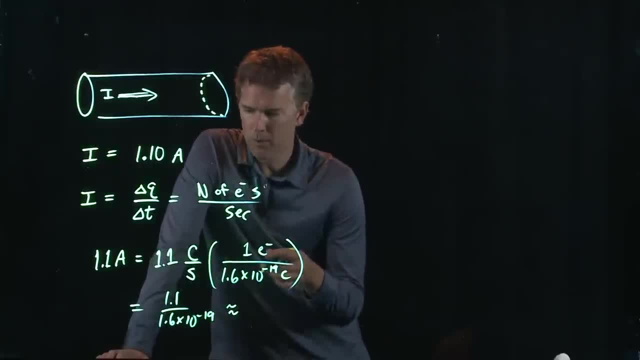 your calculator and tell me what you get. your calculator and tell me what you get. 1.1 over 1.6- that's got to be really 1.1 over 1.6. that's got to be really 1.1 over 1.6. that's got to be really close to 0.6, something maybe closer to. 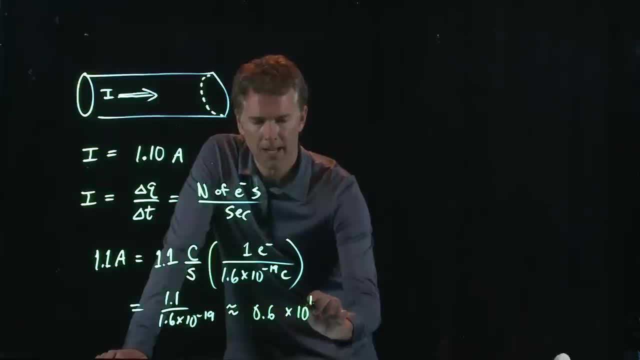 close to 0.6, something maybe closer to close to 0.6, something maybe closer to 0.7. and then we have times 10 to the 19- 0.7. and then we have times 10 to the 19- 0.7. and then we have times 10 to the 19. that thing ends up on the top. anybody? 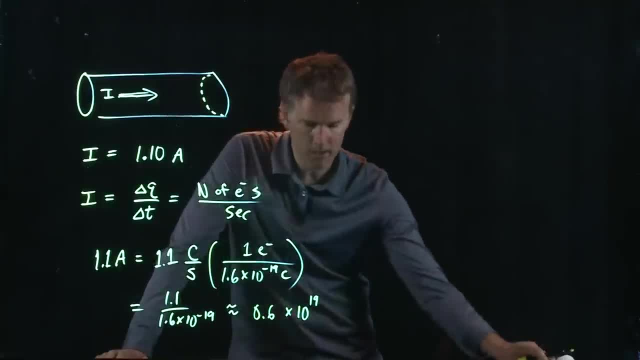 that thing ends up on the top, anybody. that thing ends up on the top, anybody. get a real answer there: 0.1 6- 9, okay. so get a real answer there: 0.1 6- 9, okay. so get a real answer there: 0.1 6 9, okay. so that is. 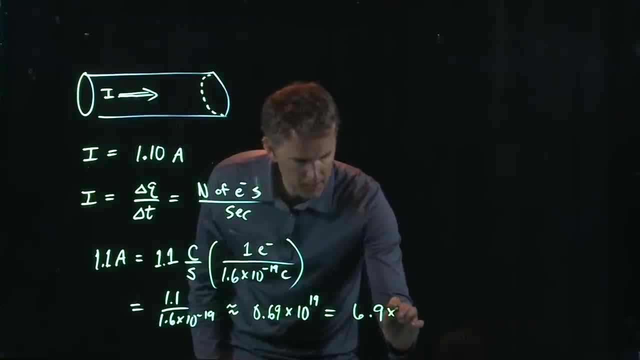 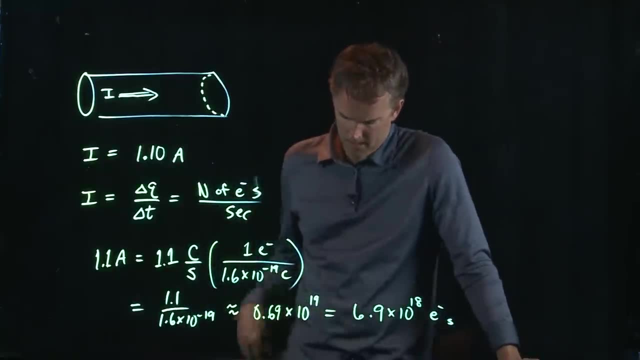 that is, that is equal to equal to. equal to 6.9 times 10 to the 18 electrons. okay, I, 6.9 times 10 to the 18 electrons. okay, I, 6.9 times 10 to the 18 electrons. okay, I don't know if it'll, let me punch it in. 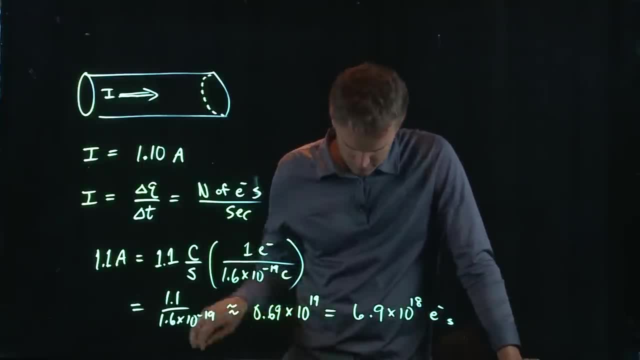 don't know if it'll let me punch it in. don't know if it'll let me punch it in here or not. let's try it, Samuel. do this here or not? let's try it, Samuel. do this here or not? let's try it, Samuel. do this thing work yet no. 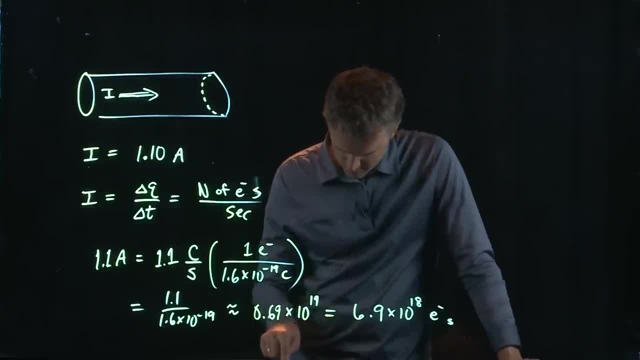 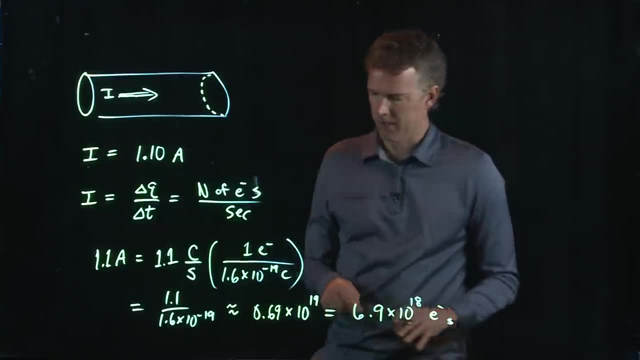 that's alright. that's alright, that's alright. let's see if the number pad works 6. let's see if the number pad works 6. let's see if the number pad works 6. enter- no, okay, doesn't work on there. but enter. no, okay, doesn't work on there. but 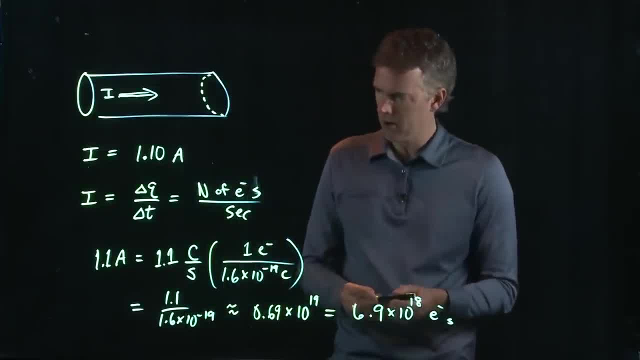 enter. no, okay, doesn't work on there, but I'm pretty sure that's going to be the. I'm pretty sure that's going to be the. I'm pretty sure that's going to be the right number. so when you get your right number. so when you get your. 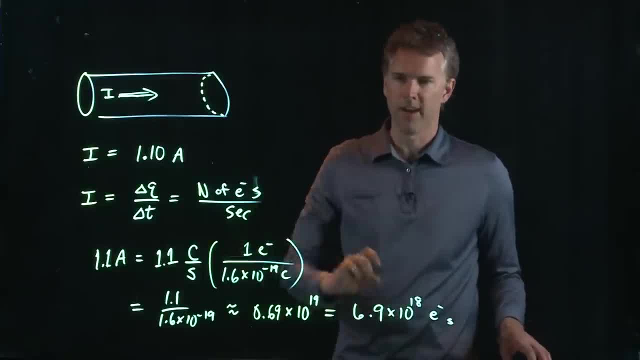 right number. so when you get your current, just multiply by this factor current, just multiply by this factor current, just multiply by this factor. right here, and you should be okay, all right here, and you should be okay, all right here and you should be okay, all right. let's talk about one of the big 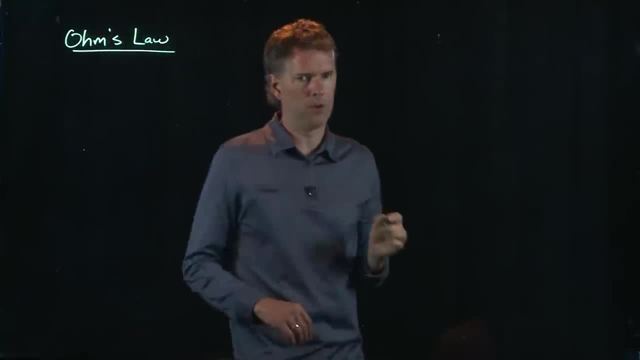 right, let's talk about one of the big right. let's talk about one of the big ones for dealing with circuits, which is ones for dealing with circuits, which is ones for dealing with circuits, which is, of course, Ohm's law. George Simon Ohm was, of course, Ohm's law. George Simon Ohm was. 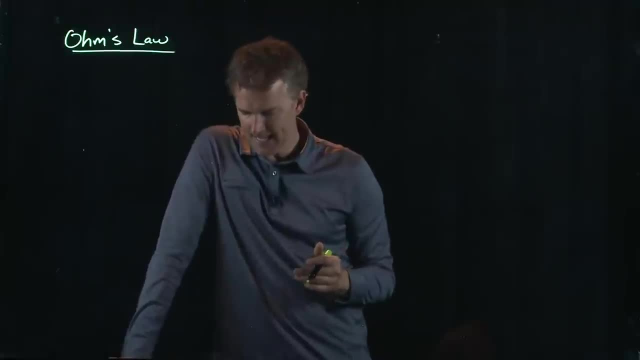 of course, Ohm's law. George Simon Ohm was a German, lived from 1789 to 1854 and he, a German, lived from 1789 to 1854. and he, a German, lived from 1789 to 1854 and he came up with the law that we now of. 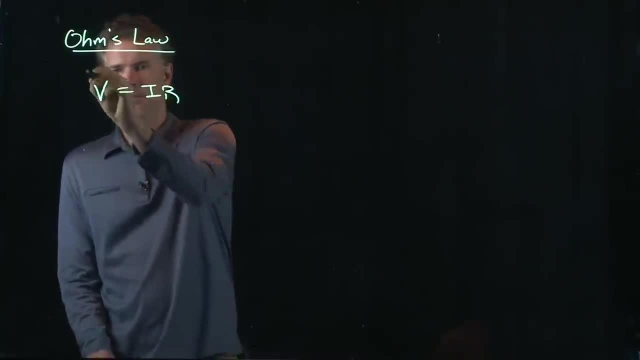 came up with the law that we now of came up with the law that we now of course call Ohm's law, which is simply course call Ohm's law, which is simply course call Ohm's law, which is simply this: V equals IR. okay, V is of course. 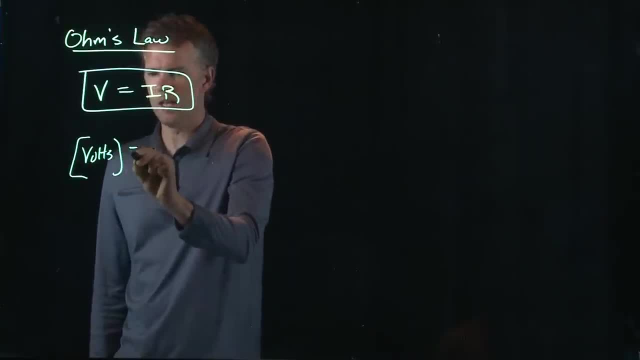 this V equals IR. okay, V is of course. this V equals IR. okay, V is, of course, volts. I is current, which is amperes R is volts. I is current, which is amperes R is volts. I is current, which is amperes R is ohms. 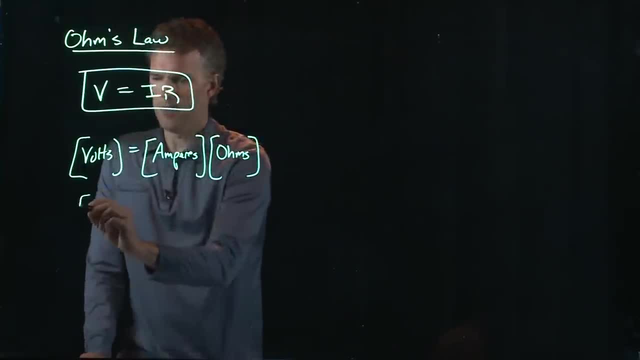 ohms, ohms, ohms, ohms, ohms, ohms, and the way we write this stuff is, and the way we write this stuff is, and the way we write this stuff is capital V for volts. capital a for amps. capital V for volts. capital a for amps. 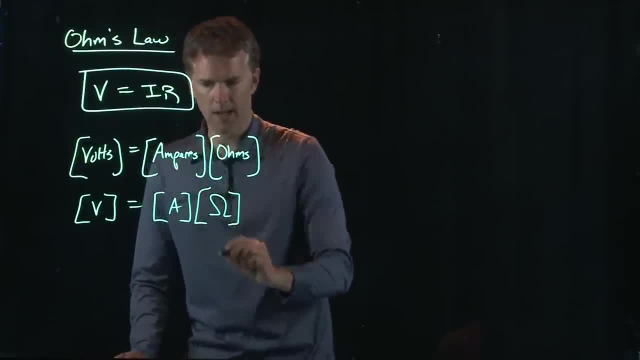 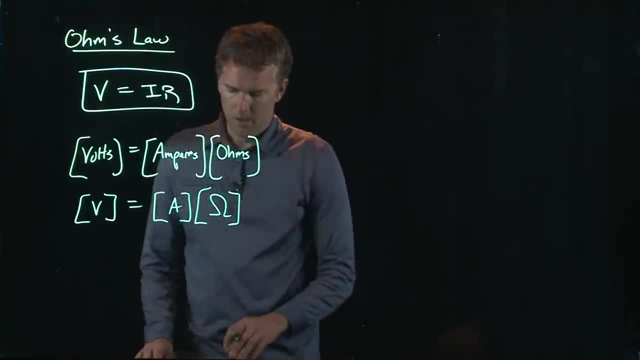 capital V for volts, capital a for amps and the Greek letter for ohms right and the Greek letter for ohms right and the Greek letter for ohms right. there, just capital Omega. all right, there, just capital Omega. all right. there, just capital Omega. all right, let's try a very simple Ohm's law. 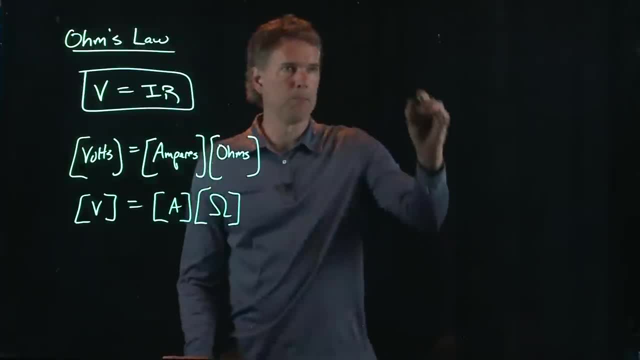 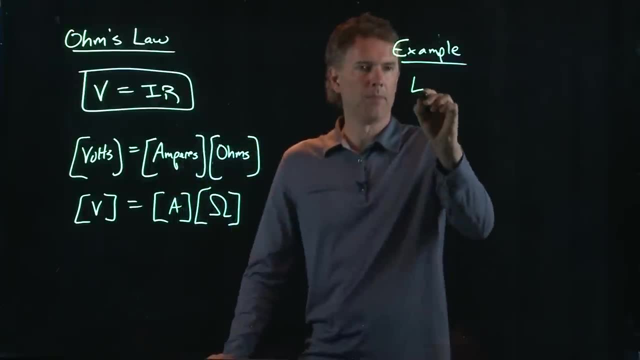 let's try a very simple Ohm's law. let's try a very simple Ohm's law problem and it's the light bulb problem problem. and it's the light bulb problem problem. and it's the light bulb problem and we're gonna say that we have a light. 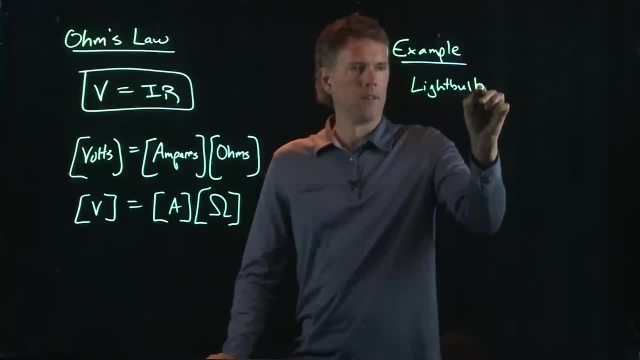 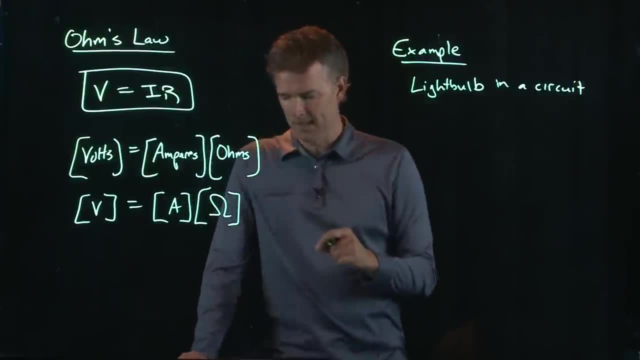 and we're gonna say that we have a light, and we're gonna say that we have a light bulb that's connected in a circuit, a bulb that's connected in a circuit, a bulb that's connected in a circuit, a light bulb, an incandescent light bulb, is. 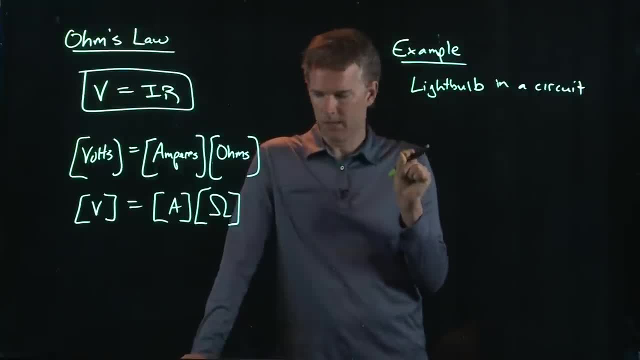 light bulb. an incandescent light bulb is light bulb. an incandescent light bulb is like a very thin resistor. okay, it's a like a very thin resistor. okay, it's a like a very thin resistor. okay, it's a wire. essentially, that's in a glass. 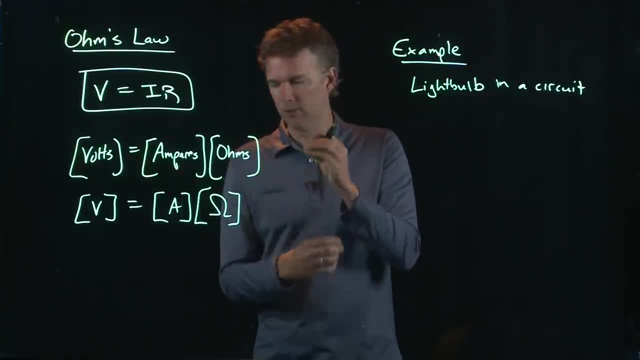 wire, essentially that's in a glass wire, essentially that's in a glass housing that is in a vacuum, and so the housing that is in a vacuum, and so the housing that is in a vacuum, and so the thing won't oxidize and when it gets, thing won't oxidize and when it gets. 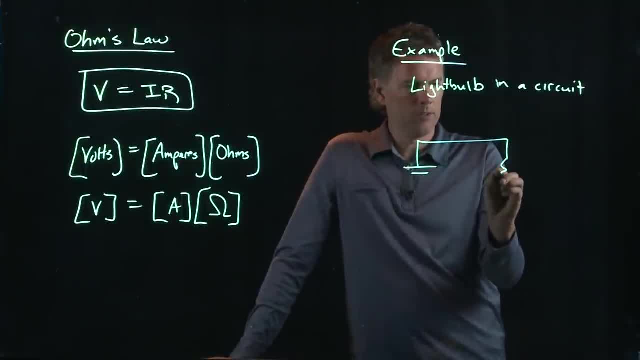 thing won't oxidize. and when it gets hot, it emits light. okay, so it looks just hot, it emits light. okay, so it looks just hot, it emits light. okay, so it looks just like a resistor, even though there is like a resistor, even though there is like a resistor even though there is this glass housing around it. this is our. 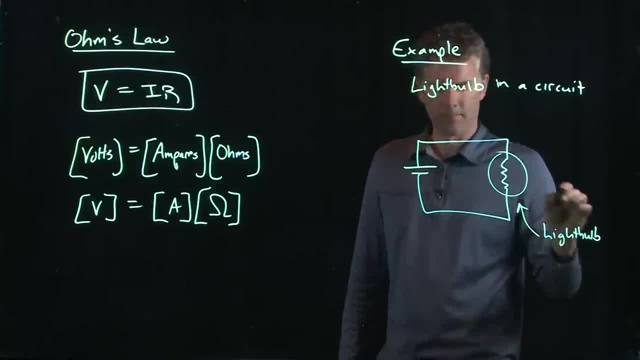 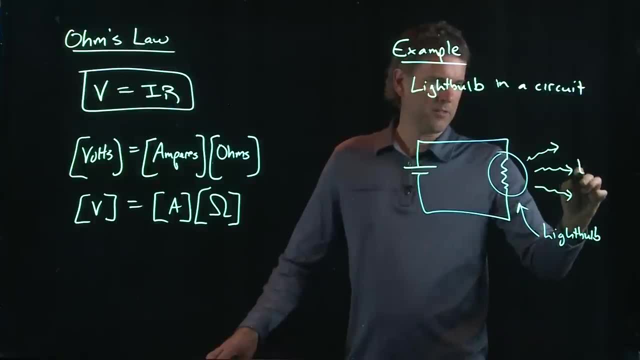 this glass housing around it, this is our, this glass housing around it, this is our light bulb. and when you get that little light bulb, and when you get that little light bulb, and when you get that little filament, hot enough, it starts to emit filament, hot enough, it starts to emit. 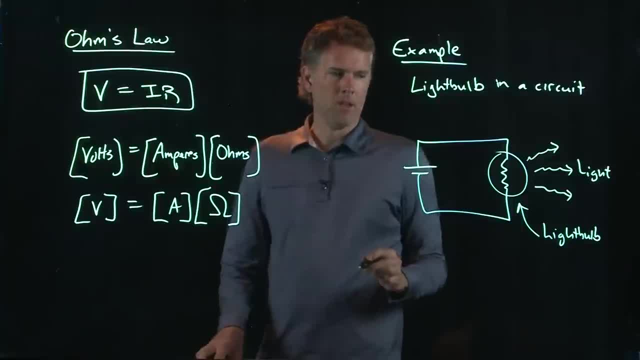 filament hot enough, it starts to emit light. if you puncture a hole in the light light, if you puncture a hole in the light light, if you puncture a hole in the light bulb breaks the vacuum. the filament- light bulb breaks the vacuum. the filament- light bulb breaks the vacuum. the filament breaks the vacuum. the filament. 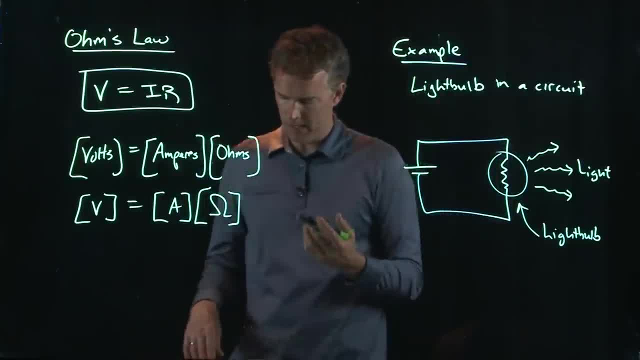 breaks the vacuum, the filament burns out very quickly. but if you can keep a burns out very quickly, but if you can keep a burns out very quickly, but if you can keep a good vacuum in there, then it'll good vacuum in there, then it'll good vacuum in there, then it'll last a reasonably long time. all right, let's. 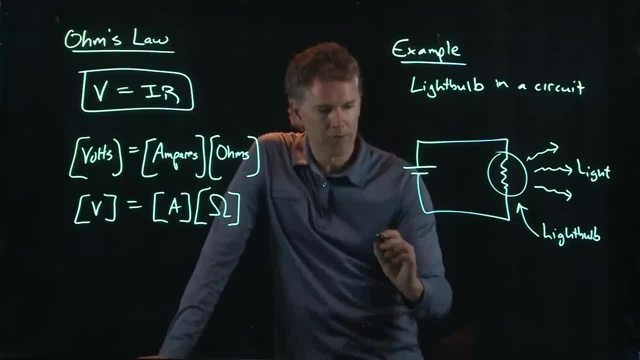 last a reasonably long time. all right, let's last a reasonably long time. all right, let's say that this is a- not a house. say that this is a- not a house. say that this is a- not a house light bulb, but a flashlight bulb. okay, so in. 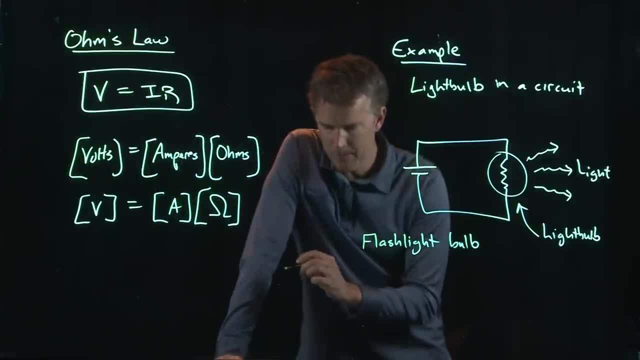 light bulb but a flashlight bulb. okay so, in light bulb, but a flashlight bulb. okay so in your flashlight. you've got a couple, your flashlight, you've got a couple your flashlight. you've got a couple. D batteries: a D battery also has a voltage. D batteries: a D battery also has a voltage. 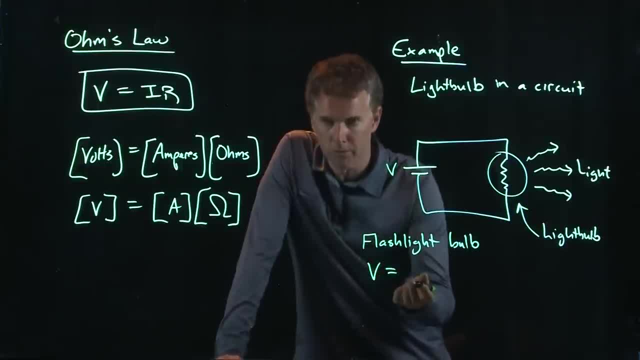 D batteries. a D battery also has a voltage of 1.5 volts, but let's say we have of 1.5 volts. but let's say we have of 1.5 volts, but let's say we have two of them in a row, so we'll say V is 3. 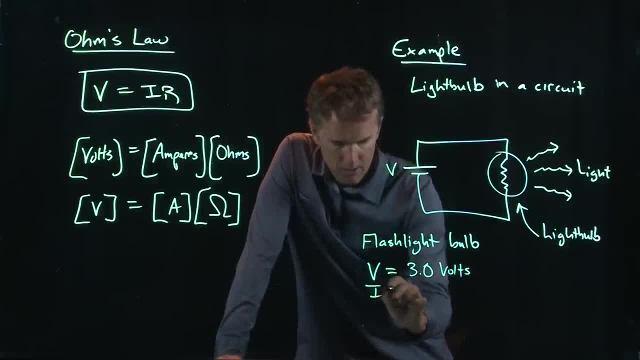 two of them in a row, so we'll say V is 3, two of them in a row, so we'll say V is 3 volts and the current that runs through volts and the current that runs through volts and the current that runs through it is maybe 400 milliamps, which is 0.4. 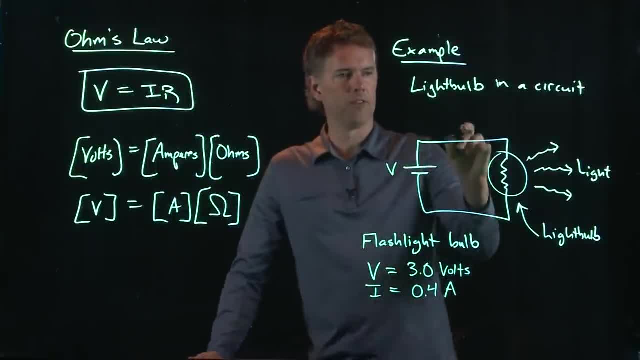 it is maybe 400 milli amps, which is 0.4. it is maybe 400 milli amps, which is 0.4 amps, and let's figure out what the amps and let's figure out what the amps and let's figure out what the resistance of the bulb is, current I 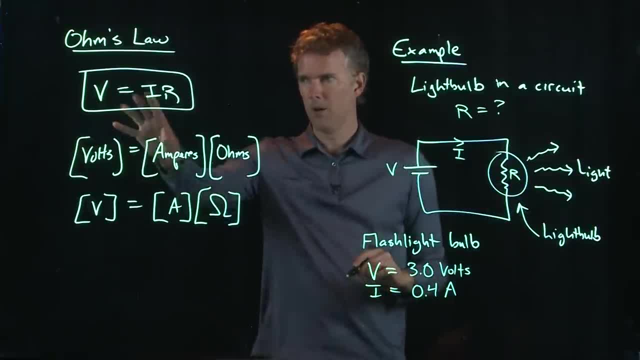 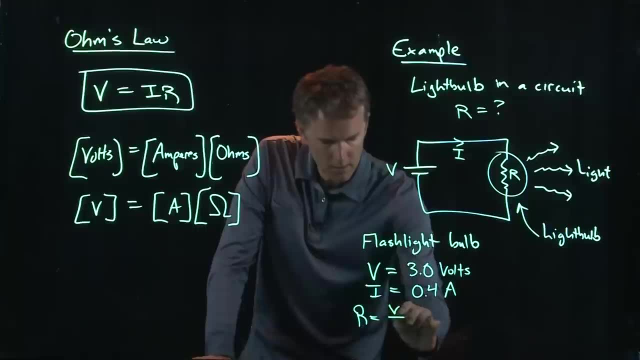 resistance of the bulb is current. I resistance of the bulb is current. I resistance are all right. resistance are all right. resistance are all right. Ohm told us how to do that piece of cake. Ohm told us how to do that piece of cake. Ohm told us how to do that piece of cake right. R is just V over I and we know V V. 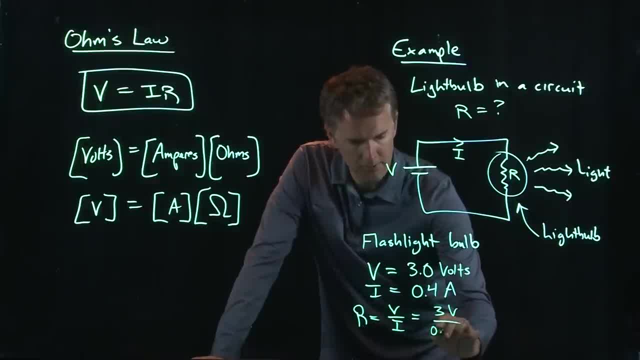 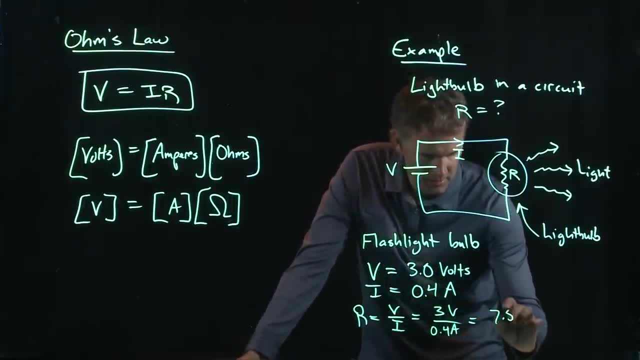 right. R is just V over I, and we know V V right. R is just V over I and we know V. V is 3 volts I 0.4 amps, and that means is 3 volts I 0.4 amps, and that means: is 3 volts I 0.4 amps, and that means we're going to get a resistance of 7.5. 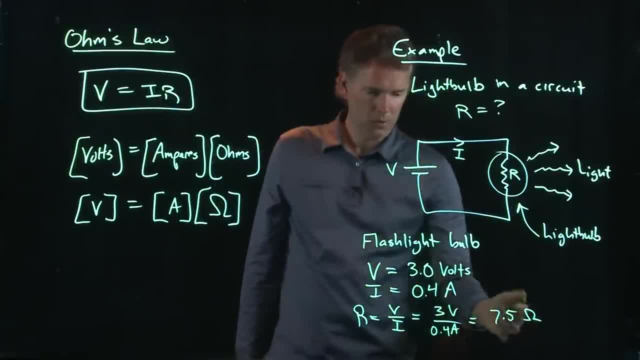 we're going to get a resistance of 7.5. we're going to get a resistance of 7.5 Ohms okay, which is pretty small when you Ohms okay, which is pretty small when you Ohms okay, which is pretty small when you guys were playing with circuits. 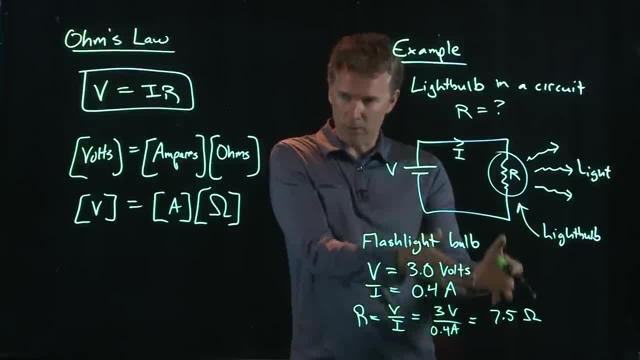 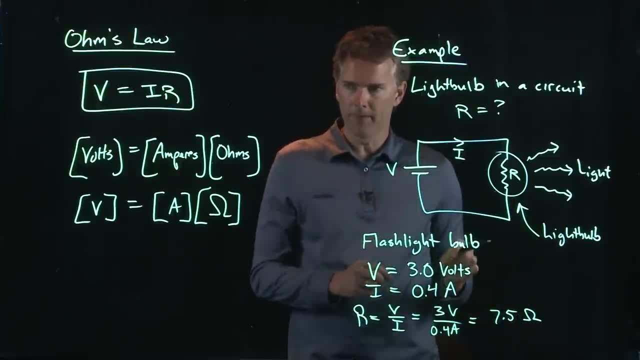 guys were playing with circuits in the lab. you were dealing with hundreds of ohms, thousands of ohms. okay, A light bulb has a very low resistance because it's essentially a piece of wire. okay, It's a little piece of wire. 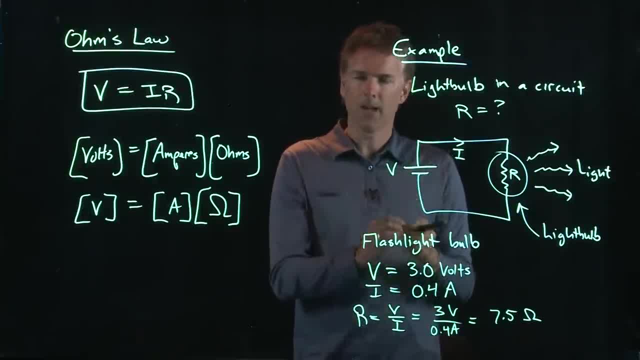 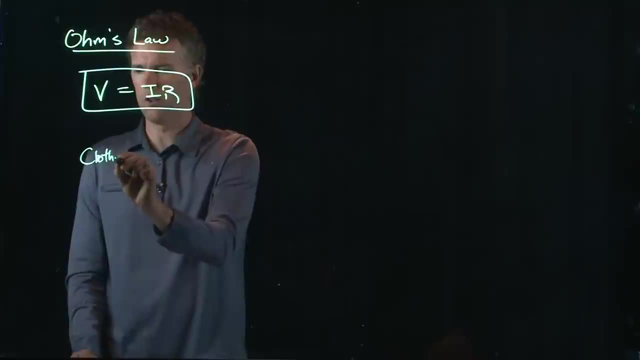 that you run current through and that thing gets hot. You're not trying to necessarily impede the current, You're trying to get that thing to get really hot and so it will emit light. All right, let's try your closed dryer. You have an electric closed dryer at home. and let's ask the question: how much current is going to go through the closed dryer? Now, electric closed dryers are typically run off of the 240 volt supply and the resistance is on the order of 11 ohms. and let's ask the question. 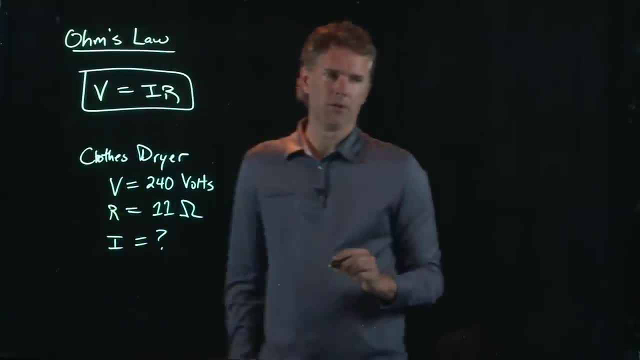 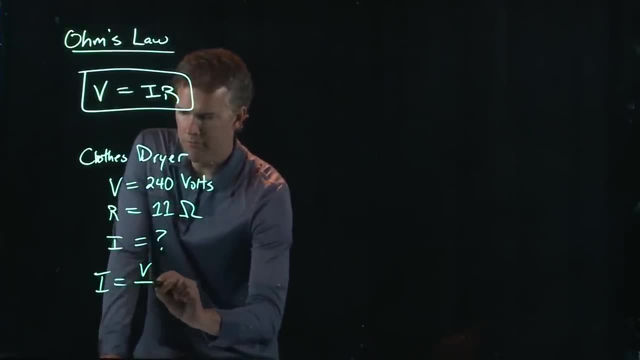 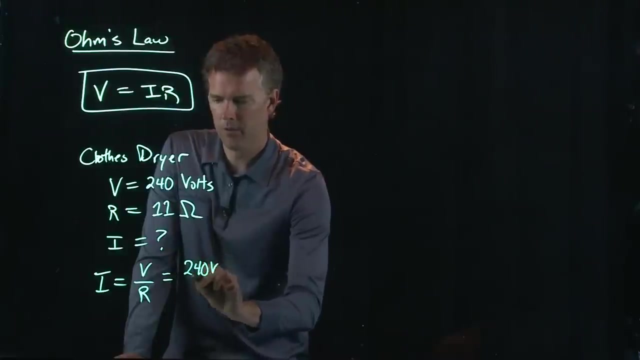 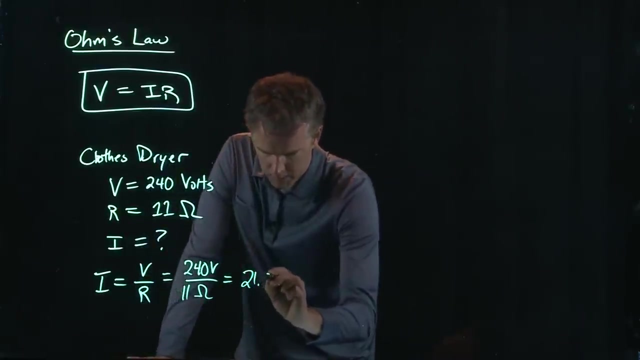 question: what is the current that's going to your clothes dryer? All right, no problem, I is V over R and we have those numbers. So this is 240 volts divided by the resistance, 11 ohms, and if you punch in those numbers you should get 21.8 amps. 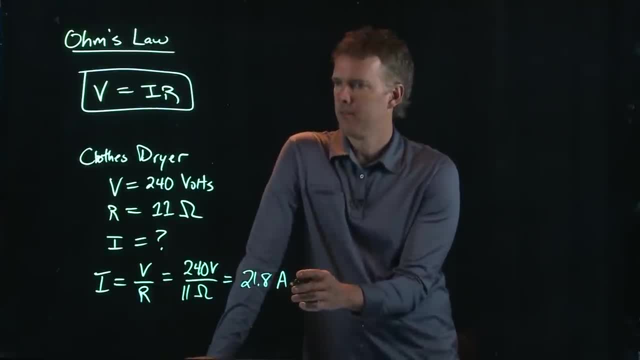 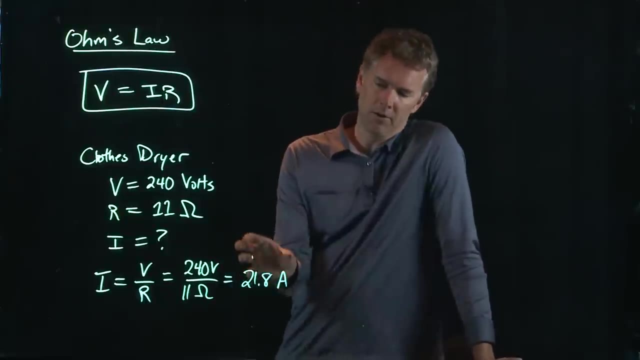 Now that is a lot of current right- 21.8 amps. So when you think about the current that's going into your house- right, We had 100 amps that was going into our house, but now on one device you're using a fifth of that 21.8 amps. And when the power comes, 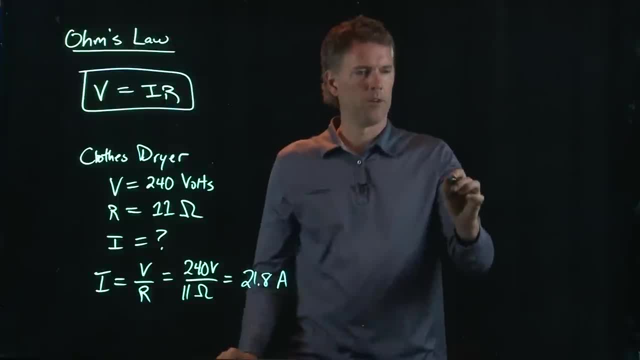 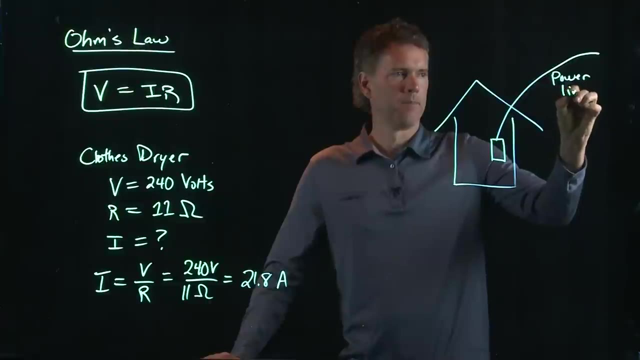 into your house. it goes into this big metal box, right, Here's your house, And the power comes in from the line, and then there is a big box, which is the first thing that it attaches to. This is the power line. Okay, and then inside your house somewhere. 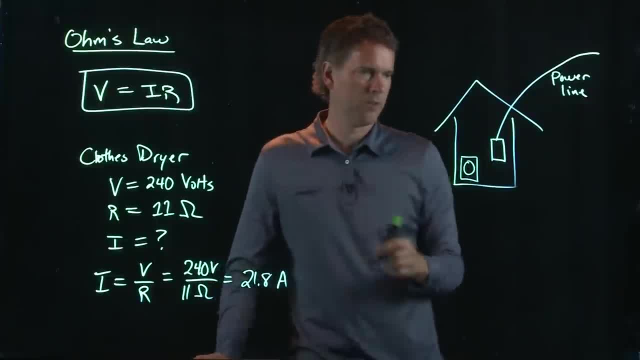 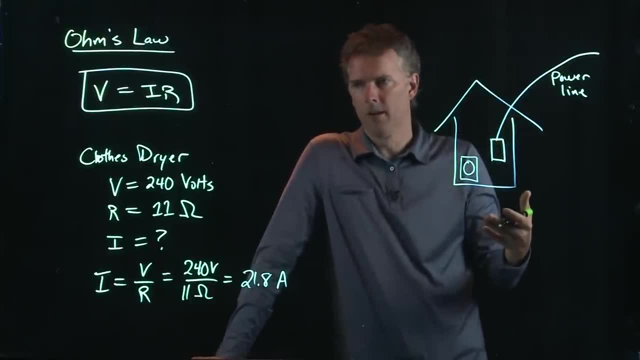 you have the clothes dryer? Yeah, question: Doesn't it work the same way when the power line's underground? Yeah, same idea. Doesn't really matter if it's above ground or underground. Typically in older neighborhoods it was all above ground In newer neighborhoods. 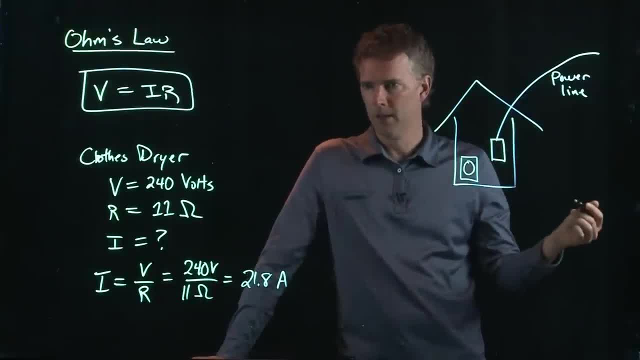 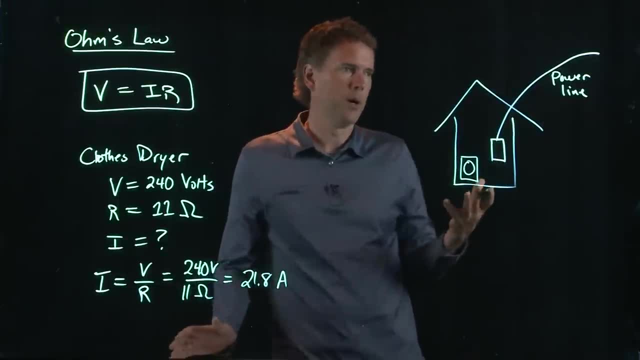 it was underground. It just depends on where they put the power lines, And it turns out to be a little cheaper to put them above ground than to dig all these big trenches underground. But it's a little bit nicer for the community and ultimately safer if they're under the 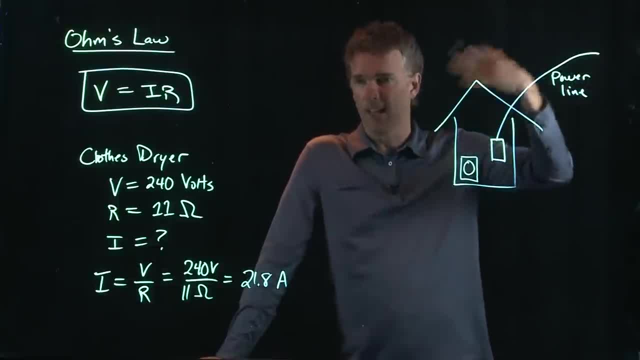 ground. right, Because if they're under the ground you don't have these big telephone poles that can get blown over in hurricanes and, you know, injure people or animals or things. So when the power line comes into your house, right the first thing that it. 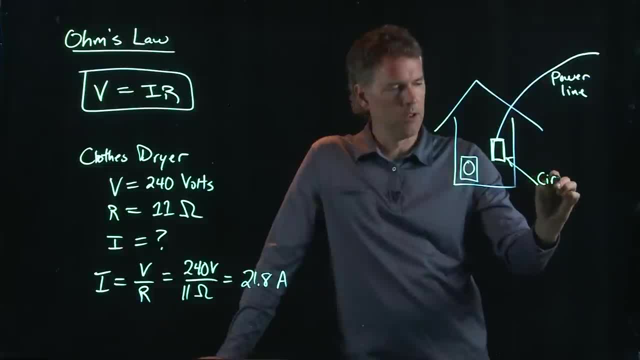 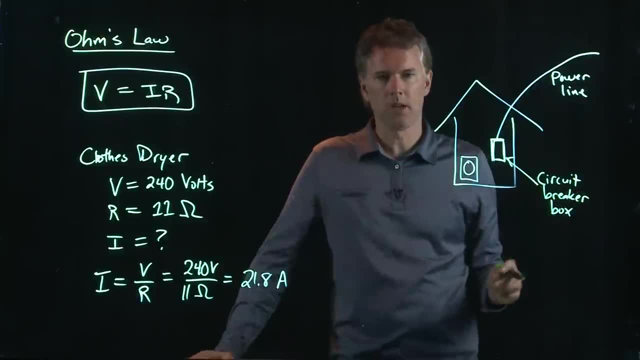 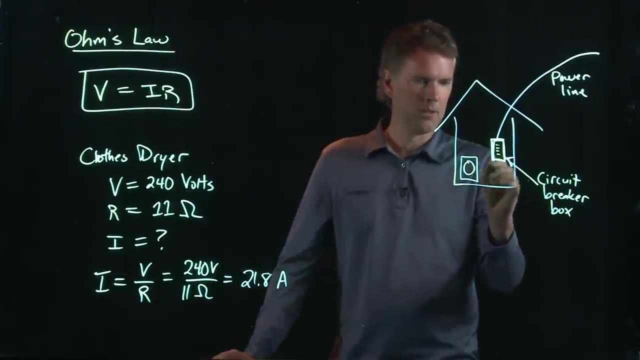 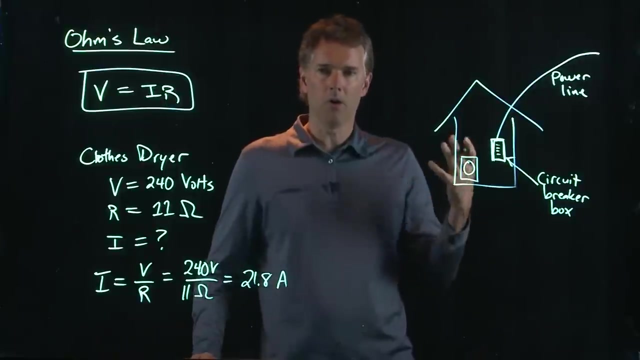 hits right here. Okay, let's look at a circuit breaker. Okay, let's see. Okay, that is called the circuit breaker or the break-out box, Okay, and usually it's outside next to your garage And in there there's a whole bunch of switches. What do those switches do? Every now and then? 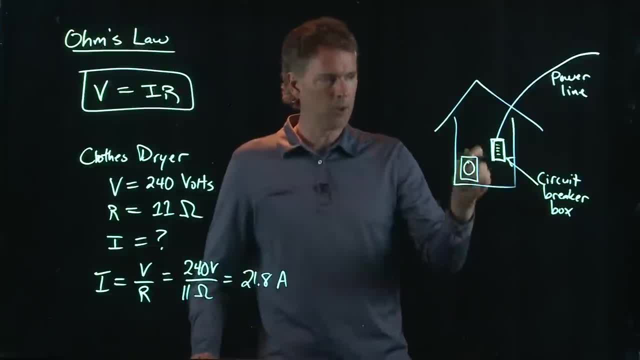 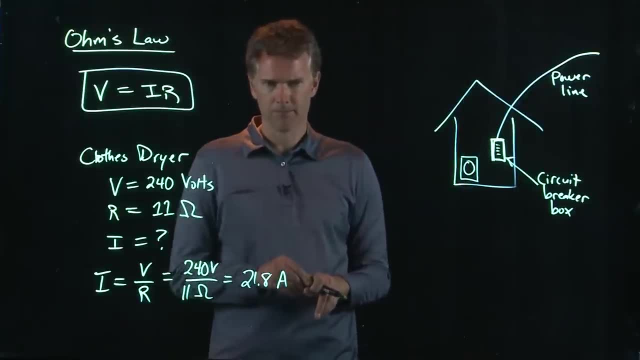 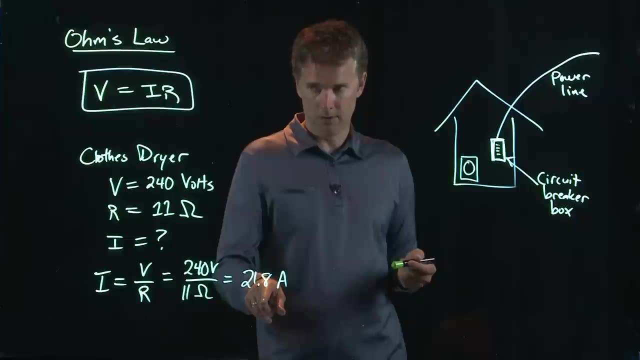 you have to go flip one of those switches, right? You say, oh, we tripped the circuit breaker back on again. What is that there for? Anybody know? Your closed dryer is trying to draw 21.8 amps. But let's say, the closed dryer malfunctions and it starts to draw four times. 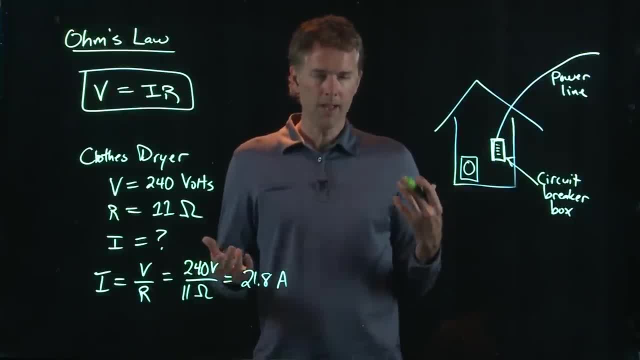 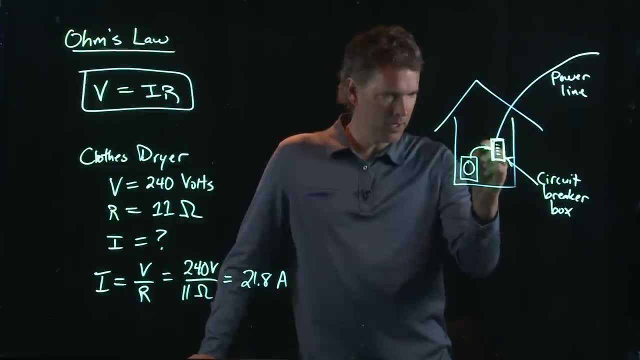 that amount, 40 amps. If it does that, bad things can happen, Namely the wires that are going to the closed dryer can get hot and burn up, And if they do that, then your house can burn down. And so, to prevent that, they put circuit breakers right here, which 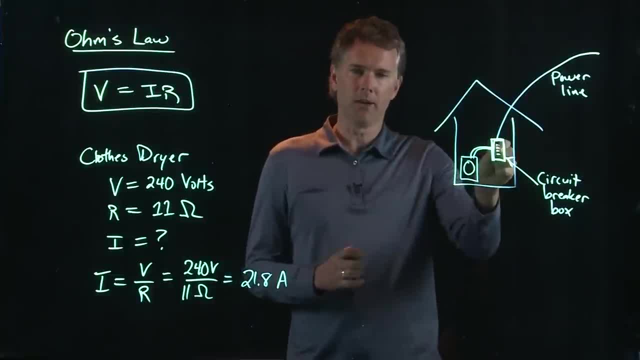 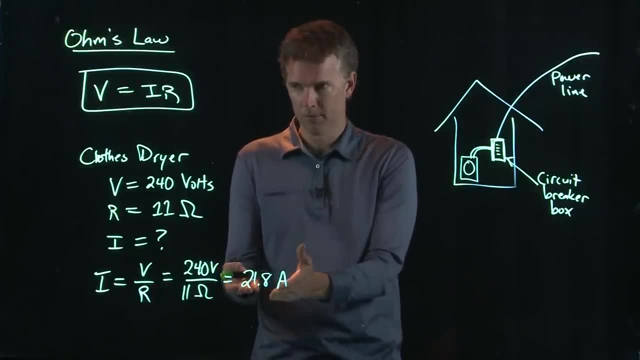 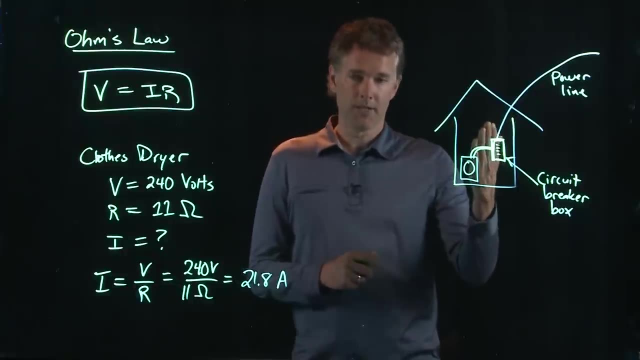 is essentially a little safety switch And what the circuit breaker does is: I'm going to let through up to 25 amps or 30 amps, But I'm not going to let through 40 amps or 50 amps. And if it does that, if it tries to draw too much current, the circuit breaker flips and 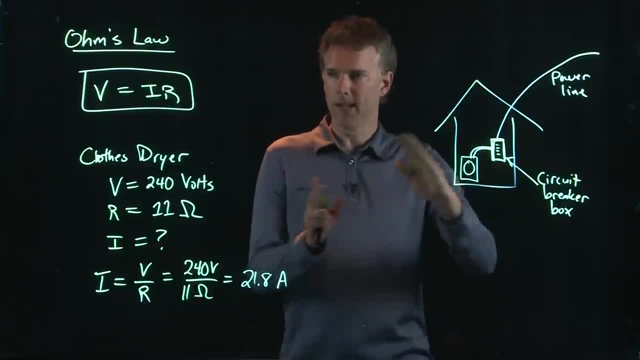 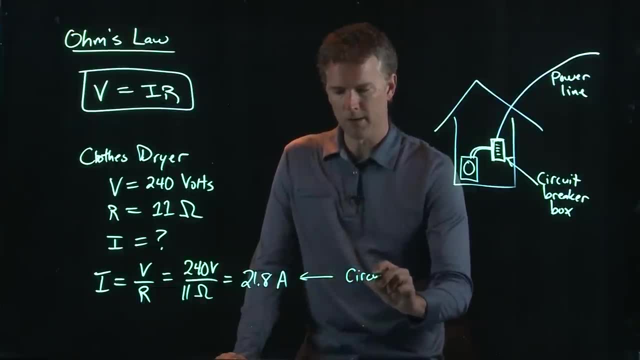 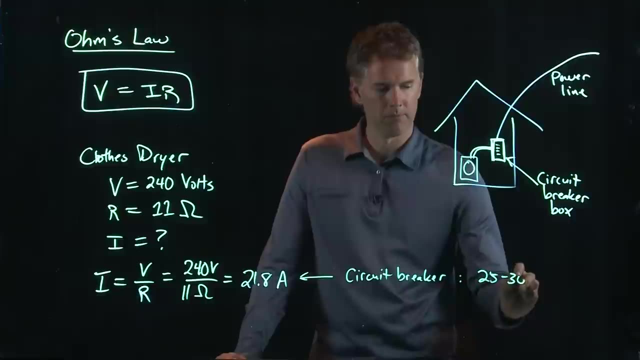 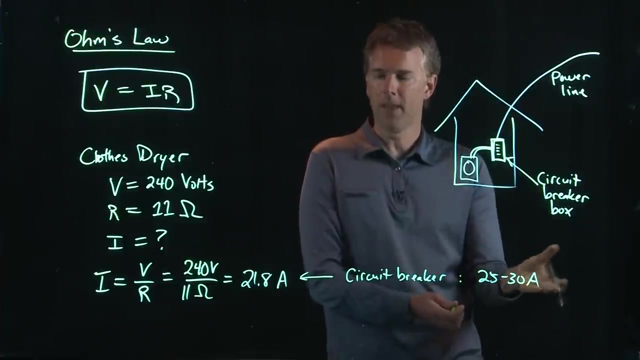 it disconnects the supply And so it immediately cuts off the electricity. And so for this number right here, your circuit breaker value will be 25 to 30 amps, So it allows this much current. But if any more current comes through, any more than 25 or 30, then it closes it off, And that's what you're doing. 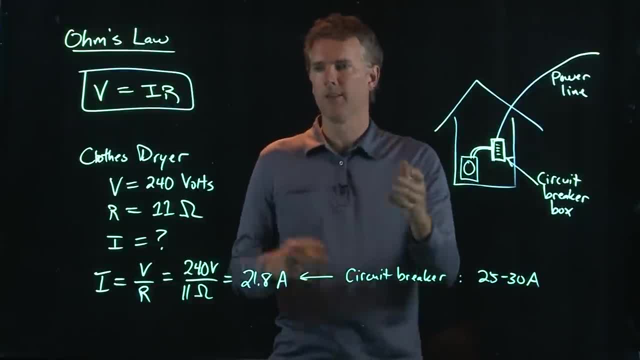 when you go reset it. You're just resetting the switch and saying, OK, I fixed the problem, I'm going to do it again. If that circuit breaker keeps flipping a lot, then you probably need to look at the problem a little more closely. Maybe hire an electrician and say: 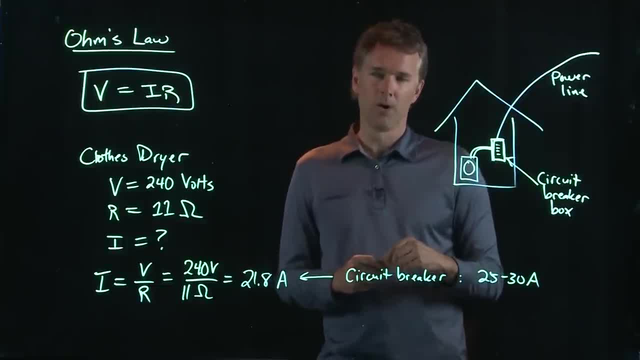 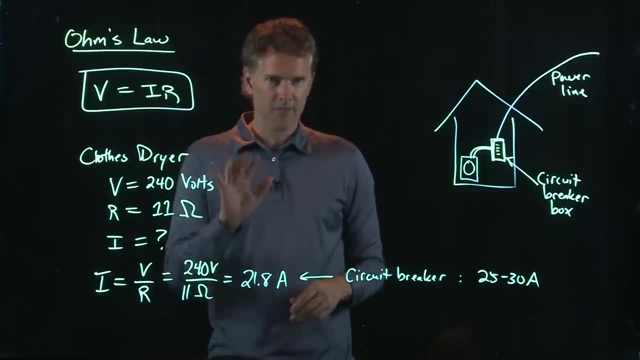 this thing keeps flipping back and forth. What you don't want to do is just tape it closed and hold it shut. All right, Let's take a five-minute break, and then we will be back here in just a few to continue this discussion. 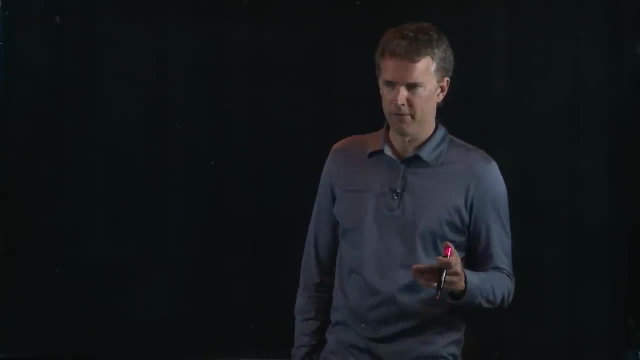 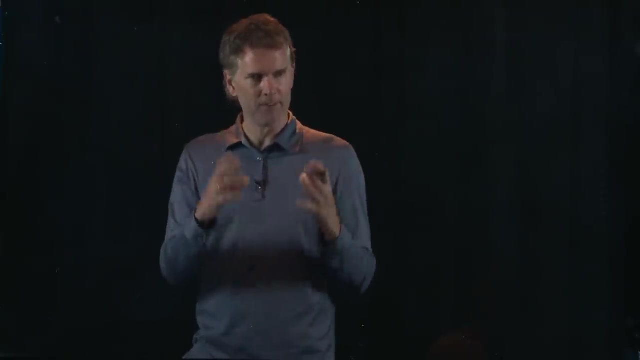 Hello everybody, Welcome back. How's everybody feeling Good? You hanging in there, I know It's Monday, like right around lunchtime and you're just crashing. I understand We should. just you know we could all take a nap here and then the people watching at. 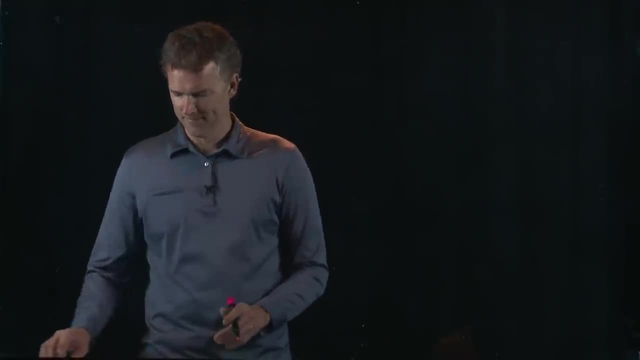 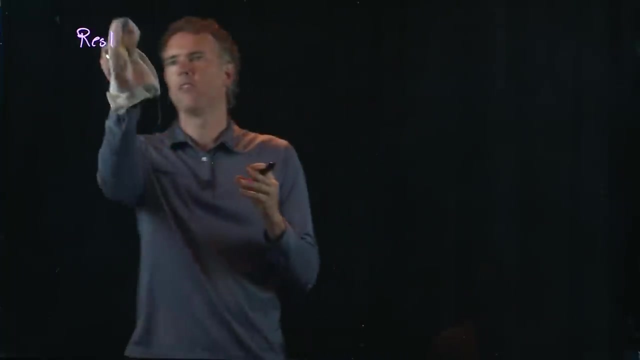 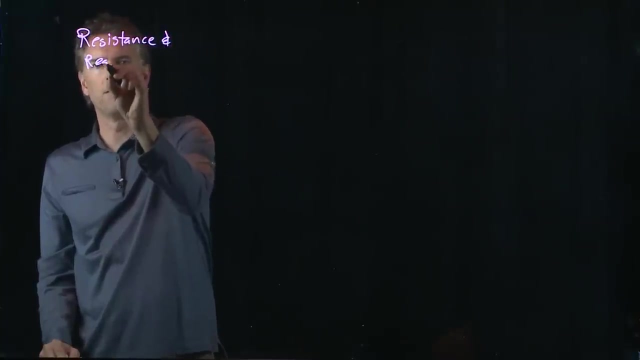 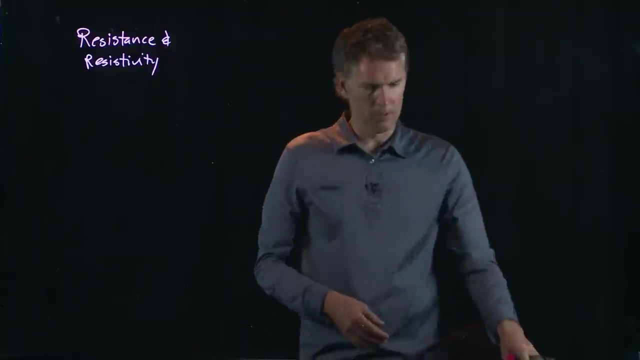 home would be like what happened: It went dark. All right, Let's continue our discussion. Let's talk about? All right, Let's talk about resistance, if I can spell it: resistance and resistivity. OK, We've talked a little bit about resistance, right? Resistance is measured in ohms and 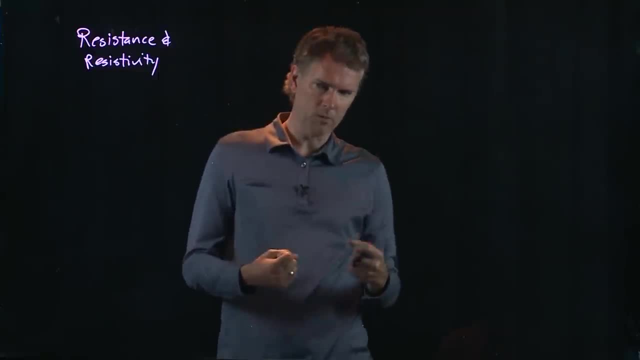 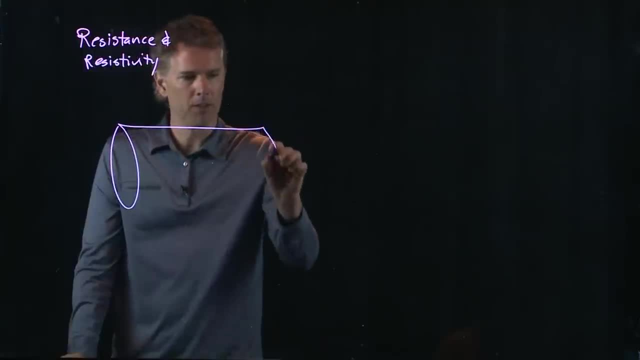 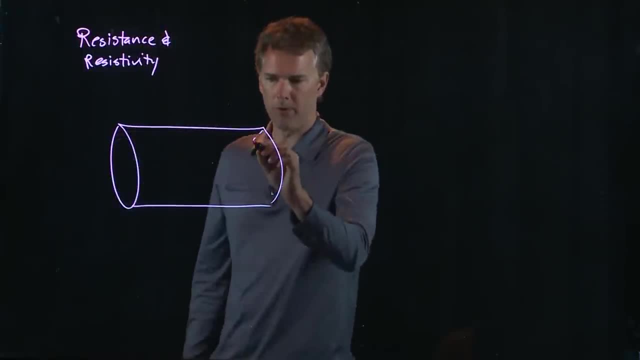 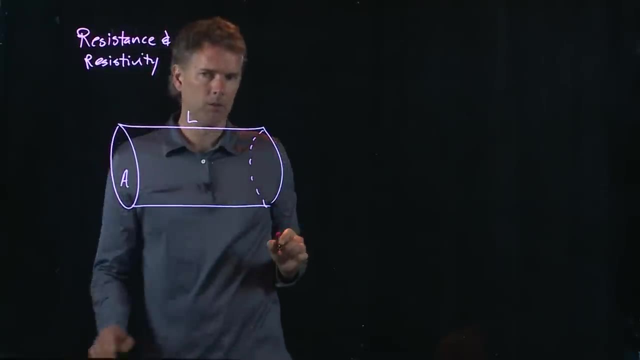 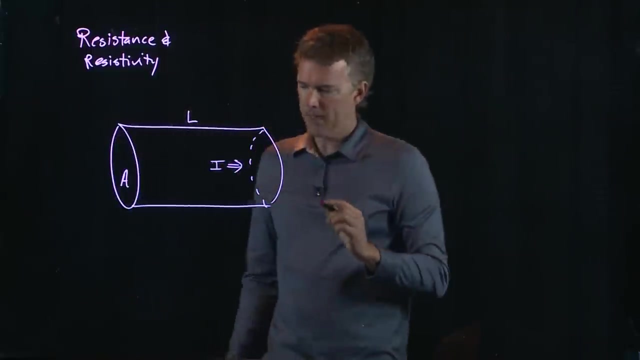 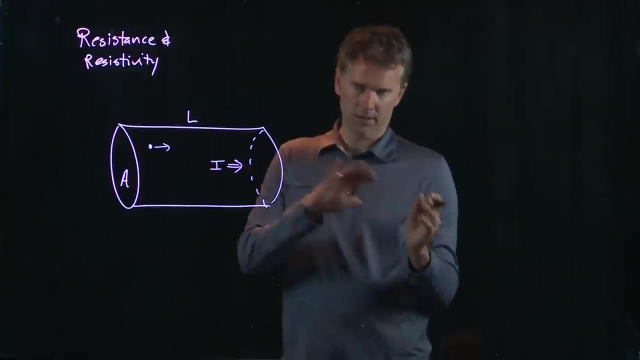 this in terms of this wire that we've been drawing. OK, Here's our wire. It's got cross-sectional area A, It's got some length to it, L, And, as current is flowing to the right, what that means is there are some sort of charge carriers that are going to move. OK, And we know its. 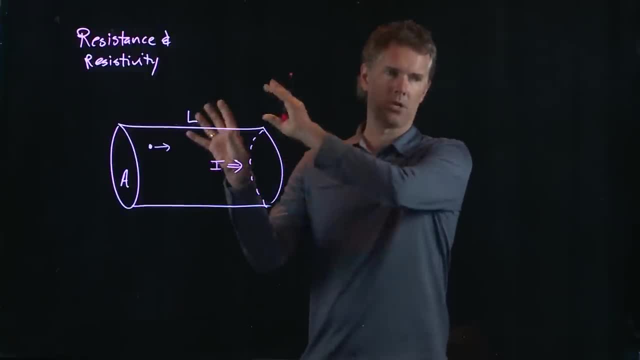 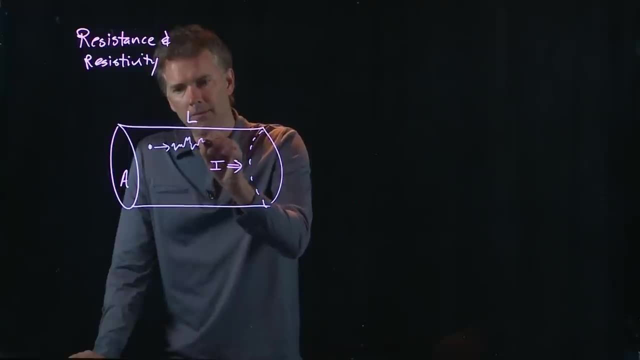 electrons moving to the left, but don't worry about that, Just pretend they're positive charge carriers moving to the right. And when those things move, they don't move in a straight line, They bounce around. OK, Why do they bounce around like that? Well, because there's other things in there Right. There's all sorts. 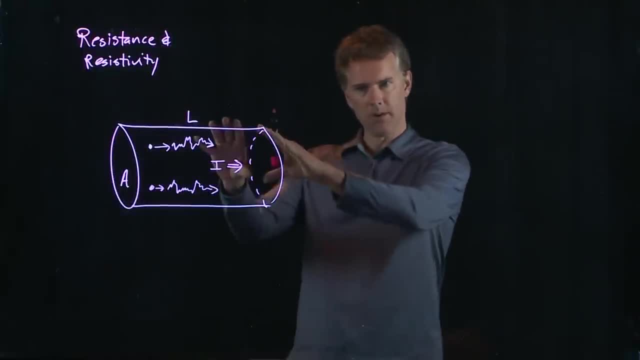 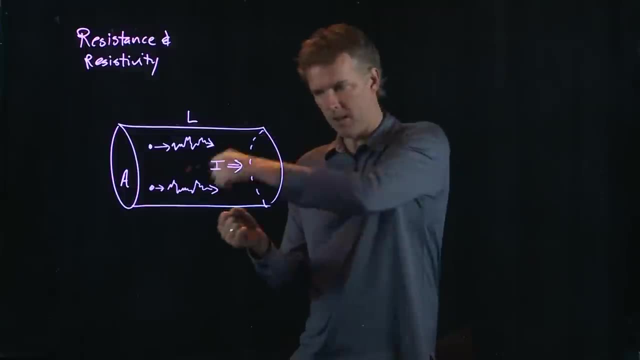 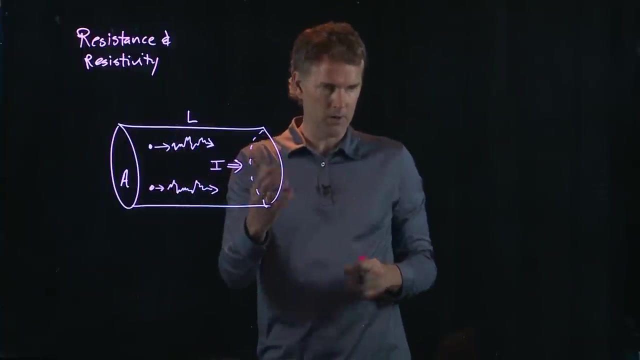 of atoms and molecules that are in this material, and the electron, jumping from one to the next, wants to move to the left a little bit and then to the right for a few, and then maybe straight and then to the left. OK, And so there is this general drift of the charges in the direction of the current. 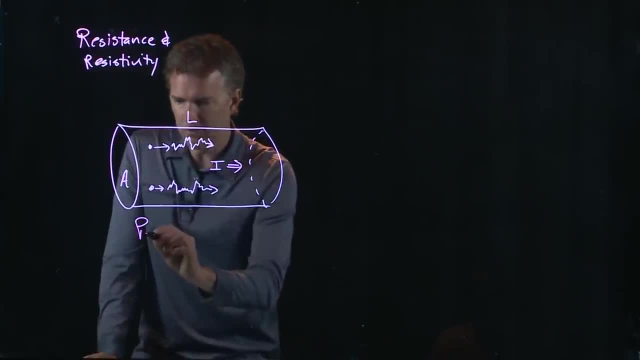 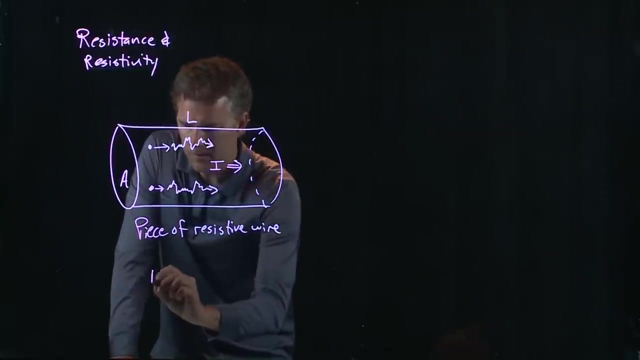 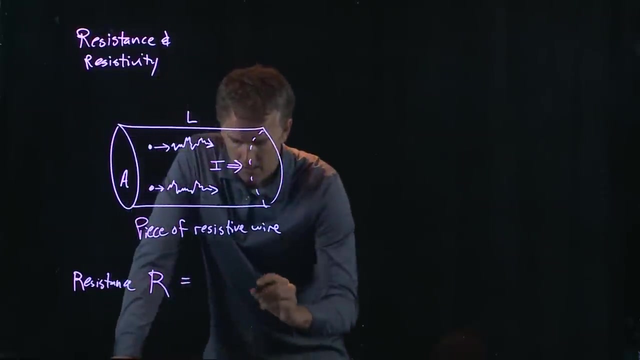 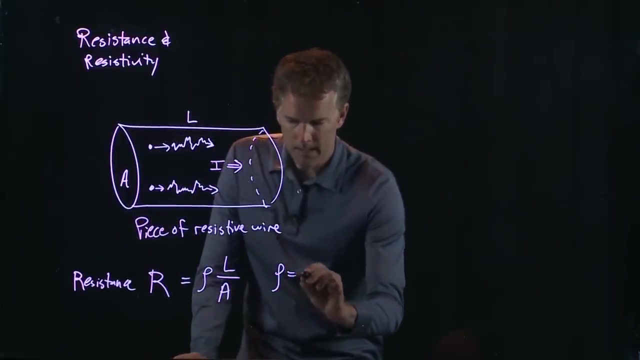 but they bounce around all over the place. So this is our piece of wire. It is resistive. How do we characterize the resistance of this wire? The way we do it is the following: Resistance, R. Resistance is Rho times L over A, where Rho is the resistivity which is kind of like 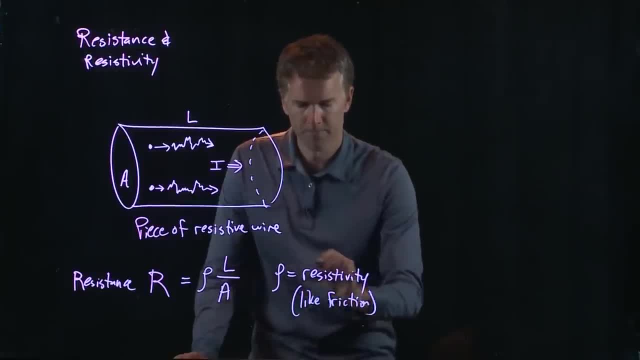 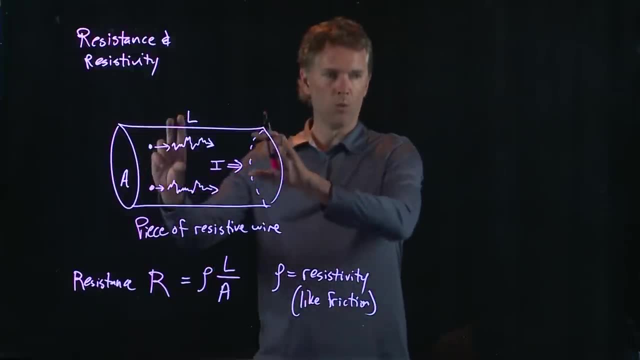 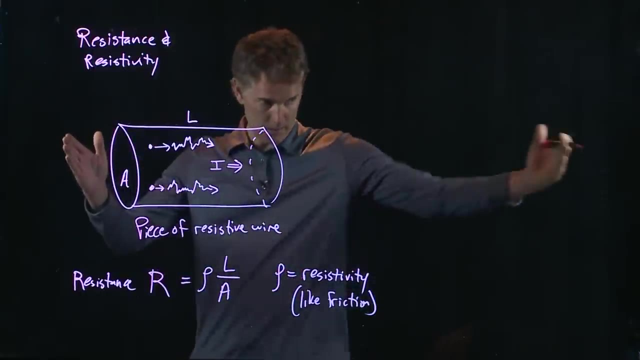 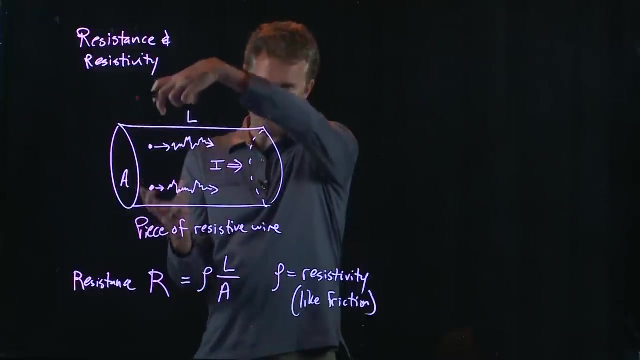 friction. OK. Resistance is Rho times L over R. If you have a wire that is more resistive, then it has a bigger overall resistance. If it is longer, then there is a bigger overall resistance. But if it is thicker, if it has, 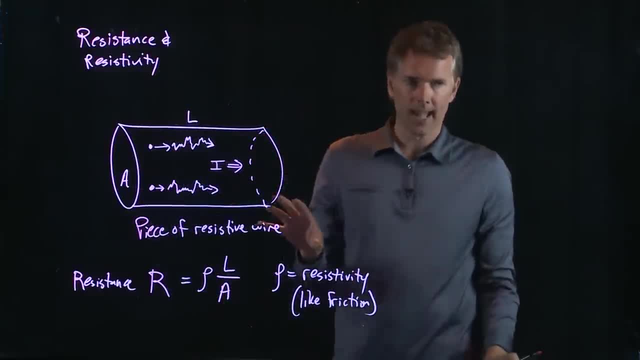 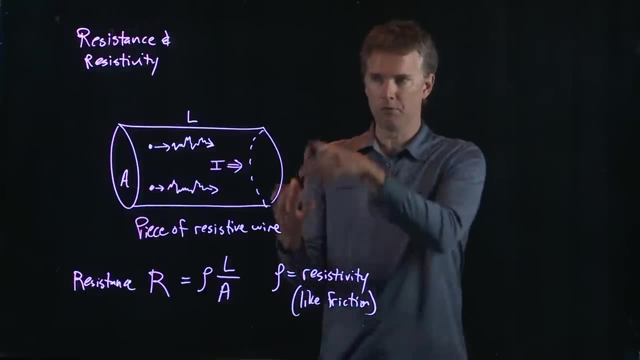 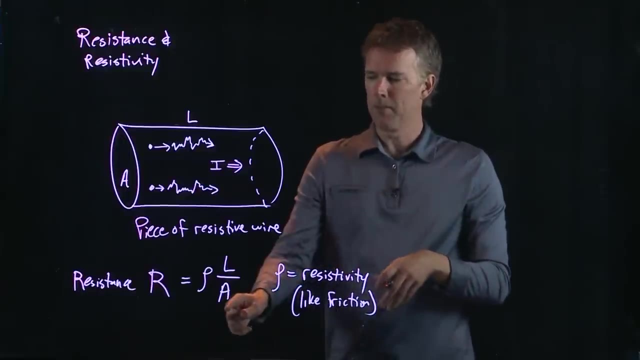 a bigger cross-sectional area A, then it is less resistive, And this is why, when the car battery is attached to the starter motor, they use big, thick cables, because they want to lower the resistance of the cable and so they make the cross-sectional area very. 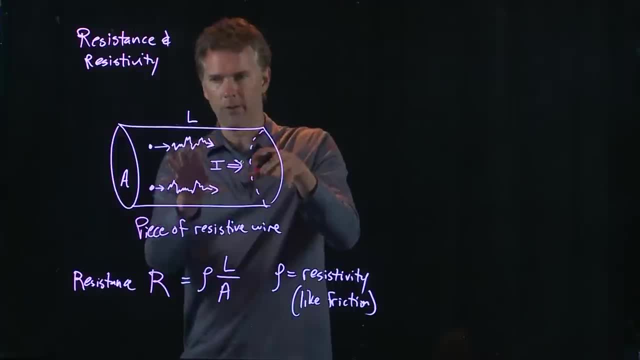 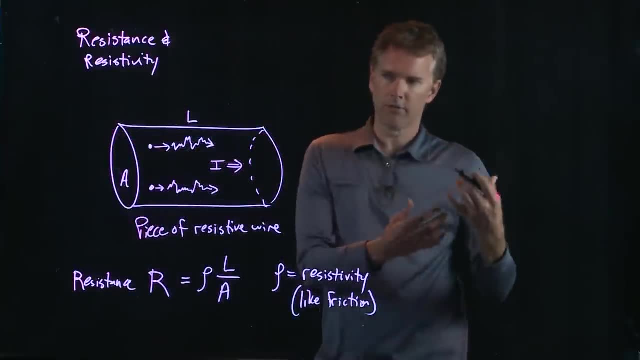 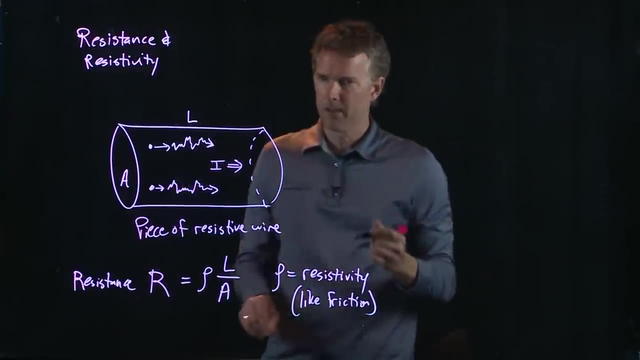 elastic, And this should make sense, right? If this really was a river, then A would determine sort of how wide the river is, And the wider it is, the easier it is for current to flow down that river. All right, Resistivity is characteristic of the materials, So every material has its own. 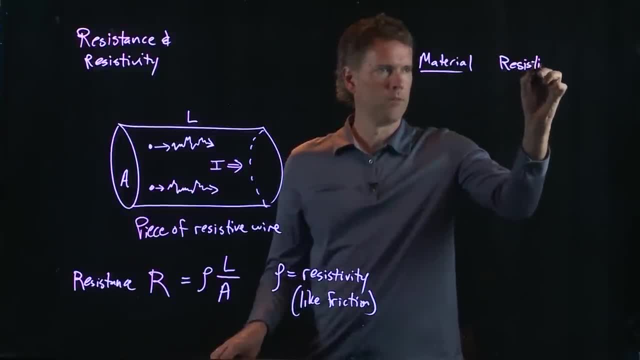 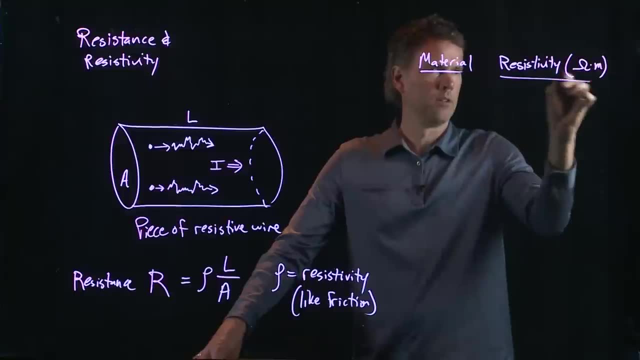 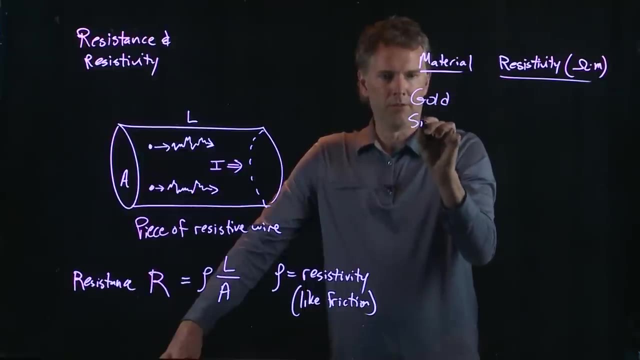 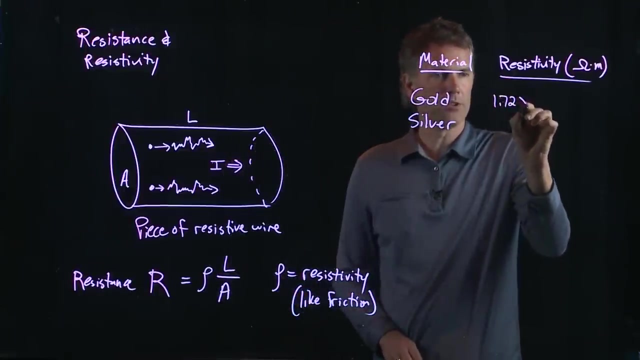 resistivity: Rho. OK, OK, OK, OK, OK are ohm meters. So, for instance, gold and silver have a resistivity of the following: 1.72 times 10 to the minus 8, or 1.59 times 10 to the minus minus 8. 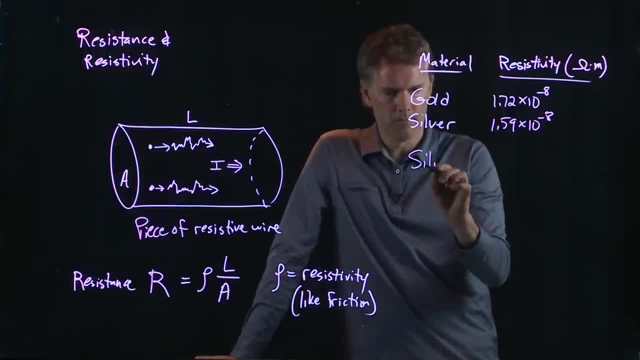 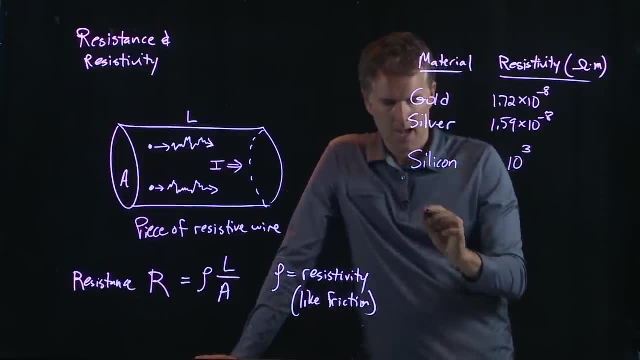 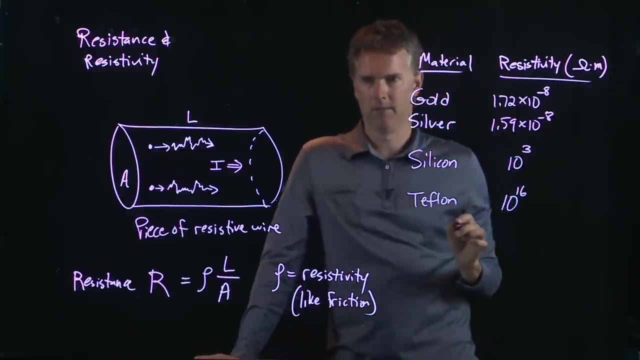 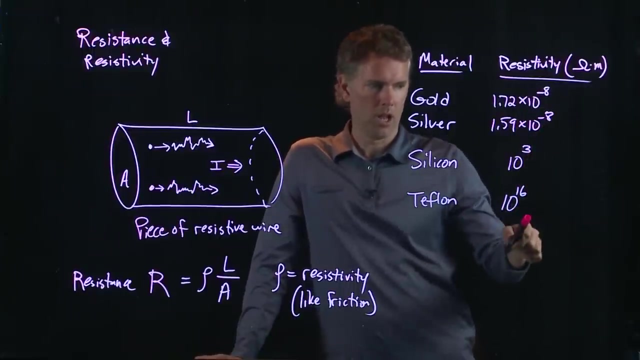 whereas something like silicon has a resistivity of 10 to the 3 and Teflon has a resistivity of 10 to the 16.. Okay, 10 to the minus 8, up to 10 to the 16, that's a lot. that's 24 orders of magnitude difference between those two. 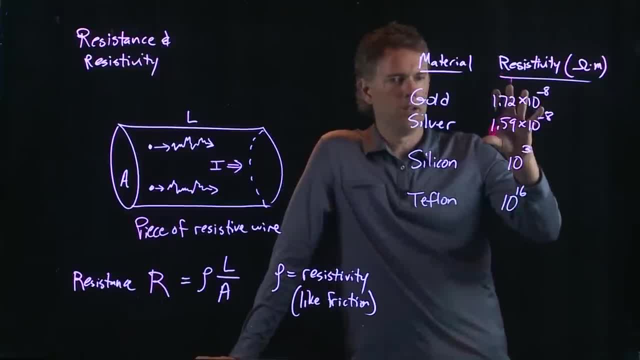 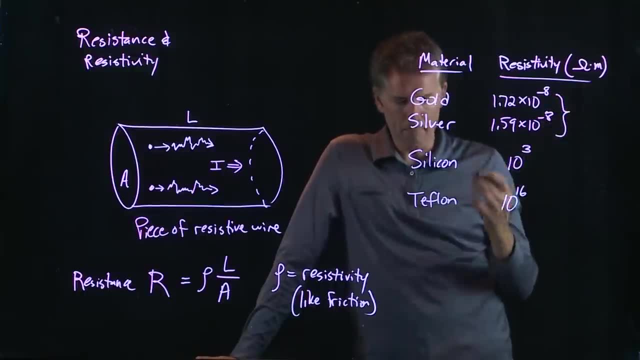 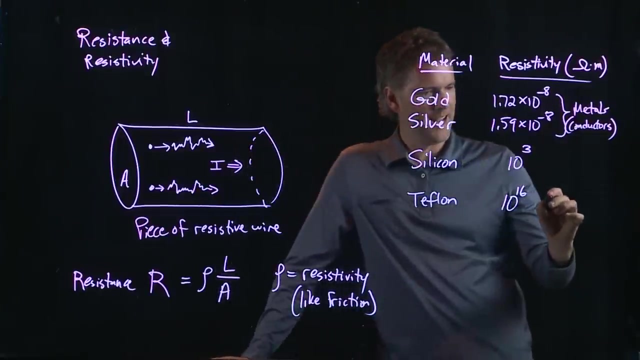 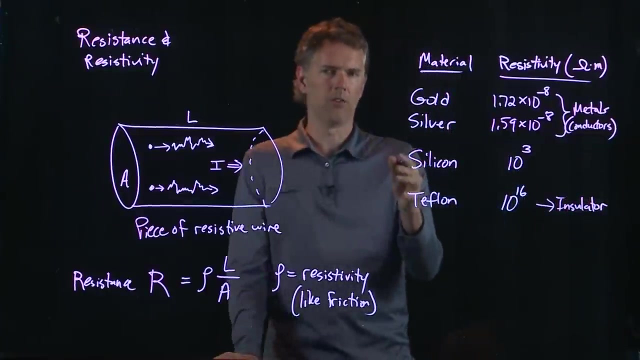 and there must be some key here- right. gold and silver. what types of material are those? those are metals, right? those are conductors. Teflon, with this huge resistivity, is, of course, an insulator. silicon is one of these interesting materials that is sort of in between the. 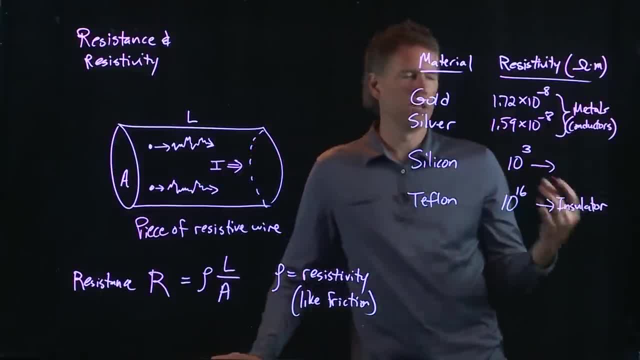 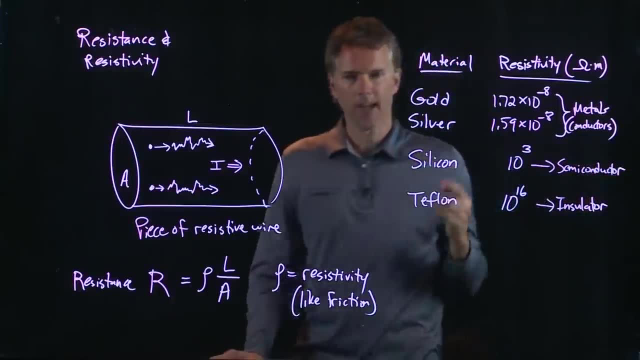 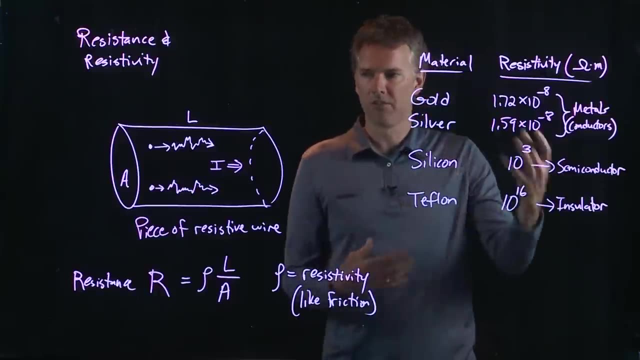 two, and in fact it can act like an insulator or a conductor, and that's why we call it a semiconductor. so that's a word that you've heard a lot- a semiconductor: it somewhat conducts, or it conducts some of the time. semiconductors are, of course, what powers all of your computer chips. 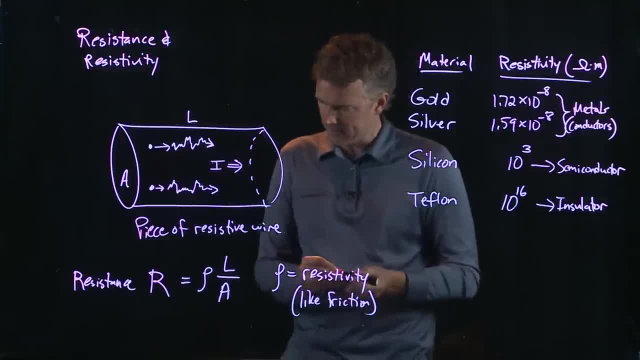 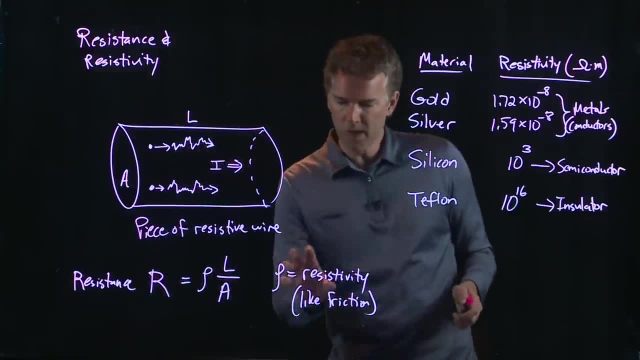 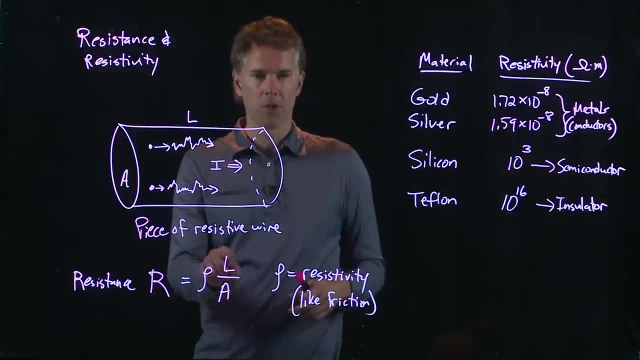 All right, so let's try an example of calculating some resistances of different things. The important thing to remember here is that resistivity depends on the atomic structure. Resistance depends on the dimensions, what it's made out of, but also how long it is and how thick the cable is. 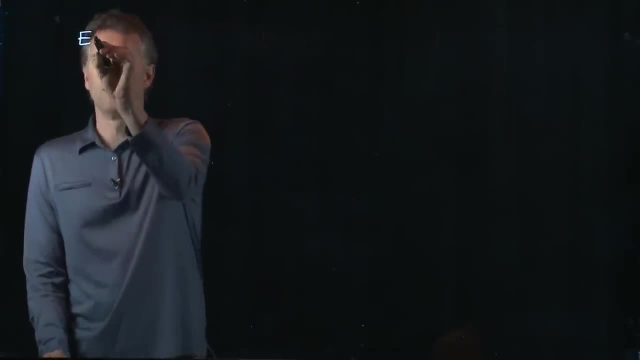 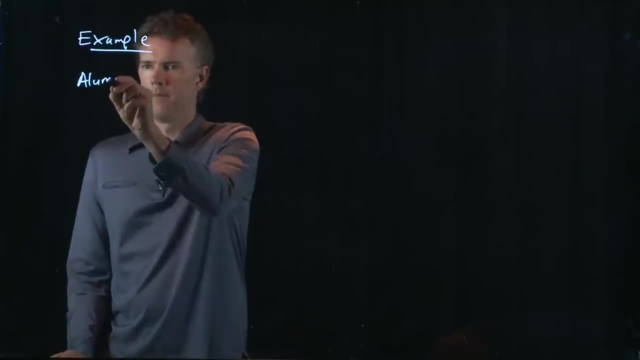 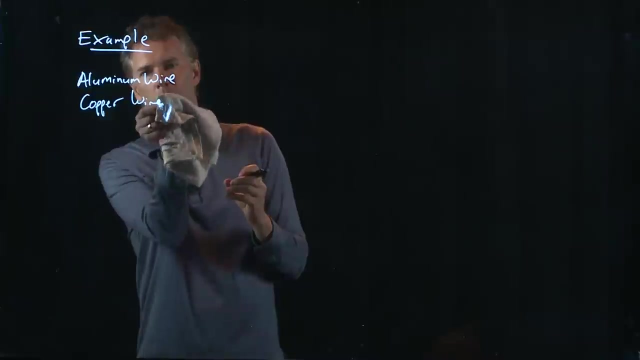 Okay, let's try an example And let's do an aluminum wire and a copper wire And let's say that these things have the same dimensions. Okay, the aluminum wire and the copper wire are the same thickness and also the same length. 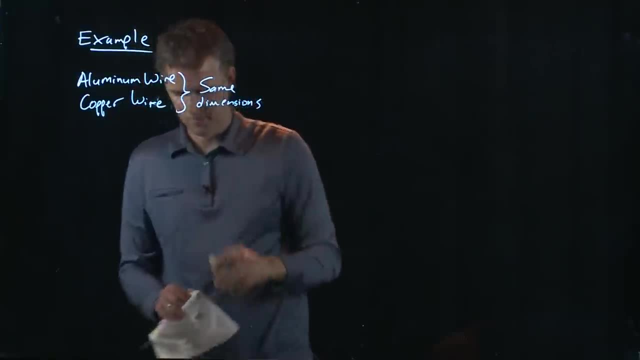 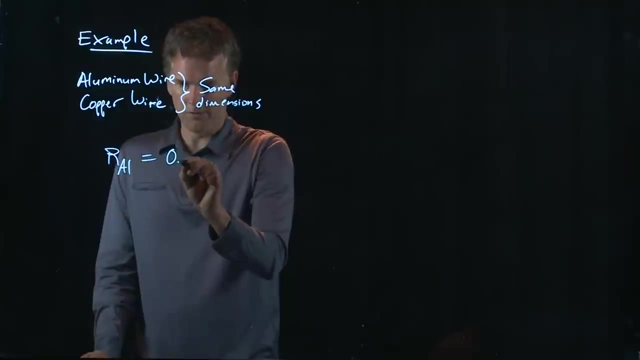 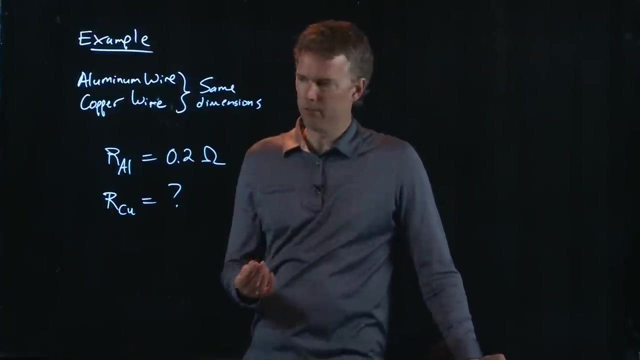 Okay, and let's tell you that the resistance of the aluminum wire is 0.2 ohms. And let's ask the question: what is the resistance of the copper wire? Okay, let's go back to our definition of resistance, right? 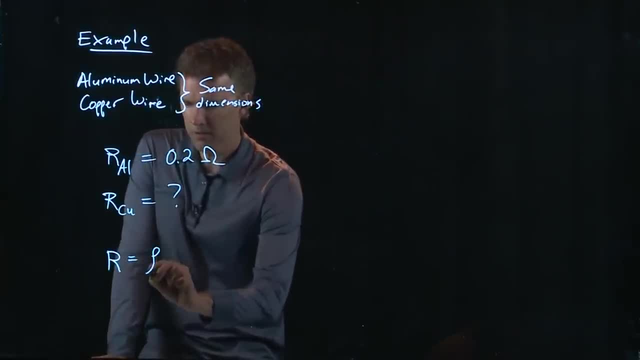 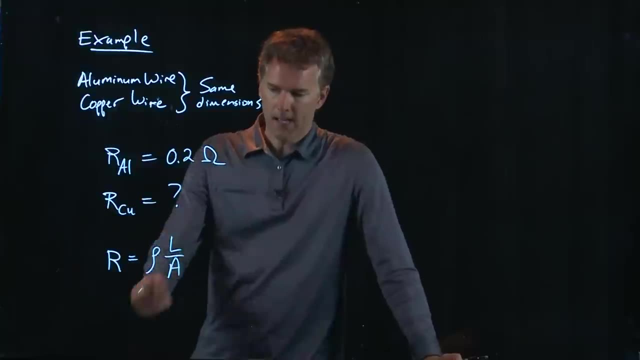 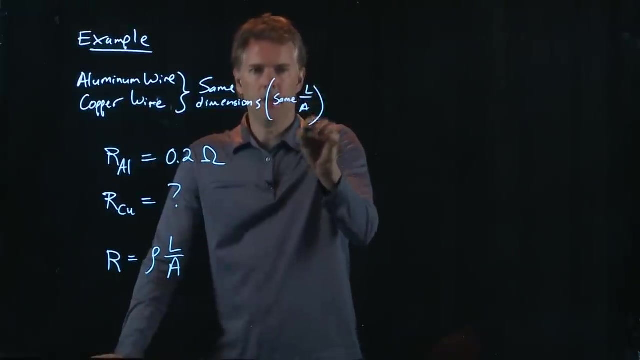 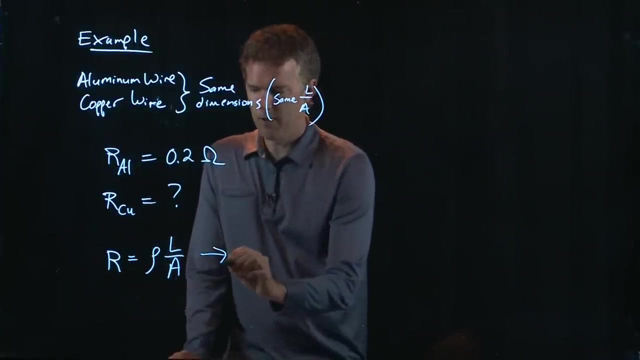 Okay, resistance was resistivity. rho, Rho times L over A. L over A is the same for both. okay, Same L over A if all those dimensions are the same, And so we can rewrite this equation slightly as the following: L over A equals R over rho. 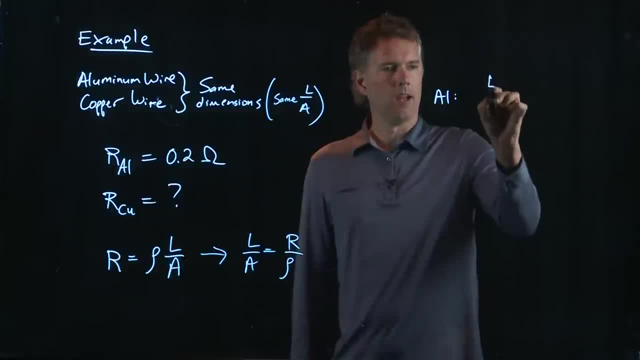 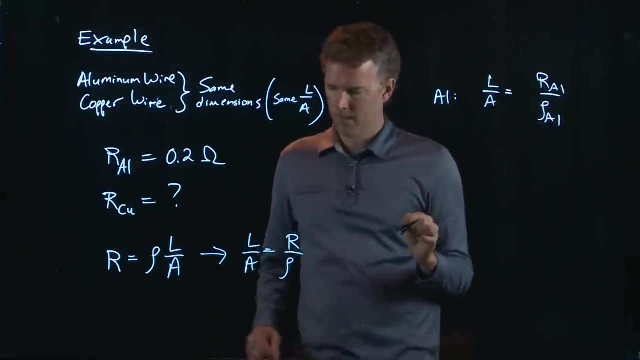 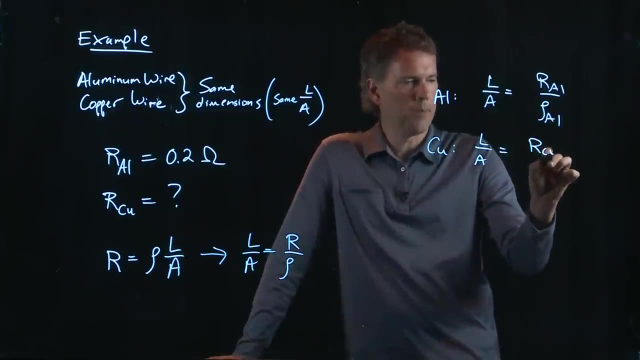 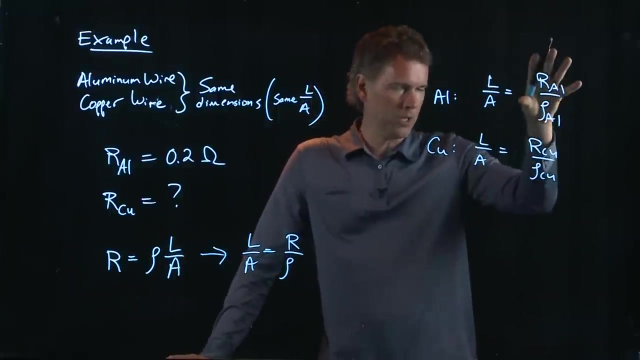 And now we can write this: for aluminum, L over A equals R for aluminum over rho for aluminum. And for copper, L over A is equal to R for copper over rho for copper. And now we can put these things together right: L over A is the same, so we can equate the right sides. 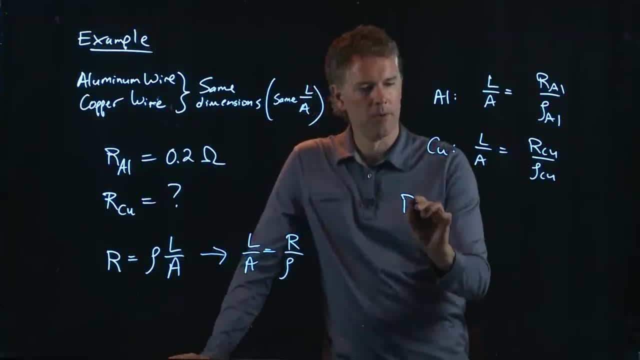 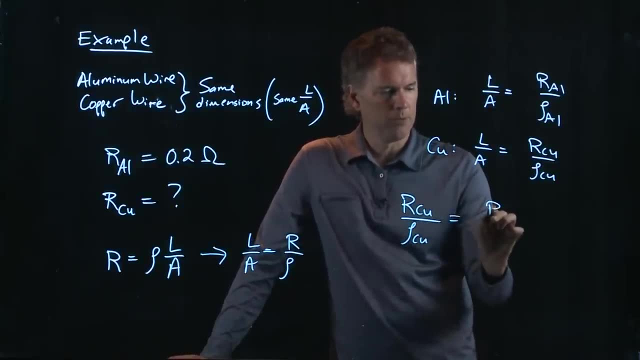 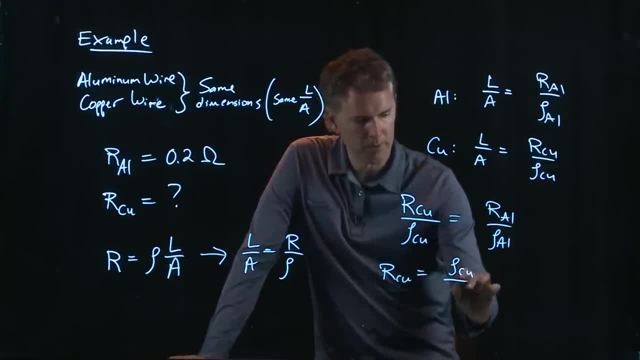 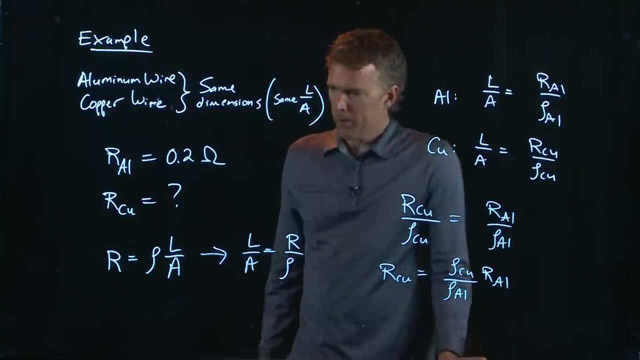 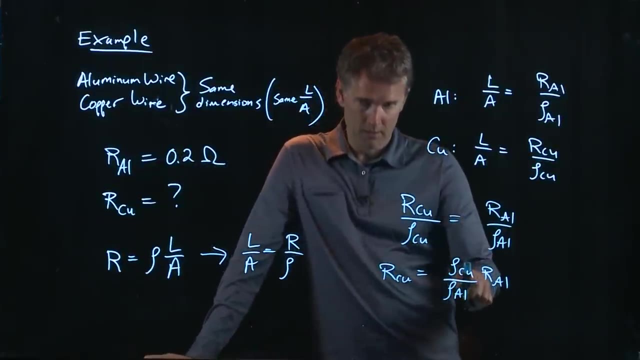 So what is R of copper? It is rho of copper divided by rho of aluminum times R of aluminum. What we told you was resistance for aluminum. What we need is the resistivity for aluminum. What we need is the resistivity for aluminum and copper. right there. 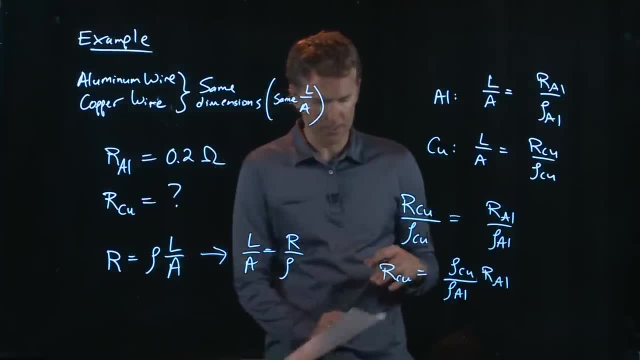 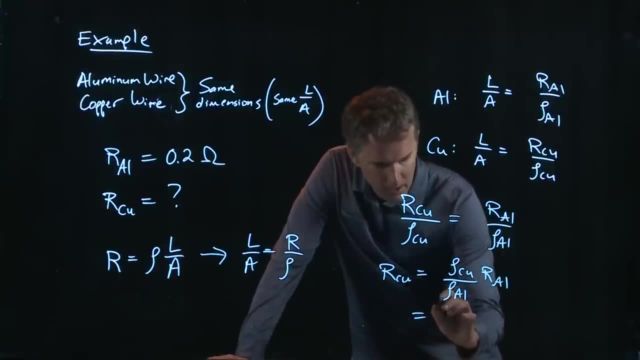 And that you have to look up in the textbook. okay, So if you flip open the textbook and you find the correct table in this chapter, you should get this following: Resistivity of copper is 1.72 times 10 to the minus 8 ohm meters. 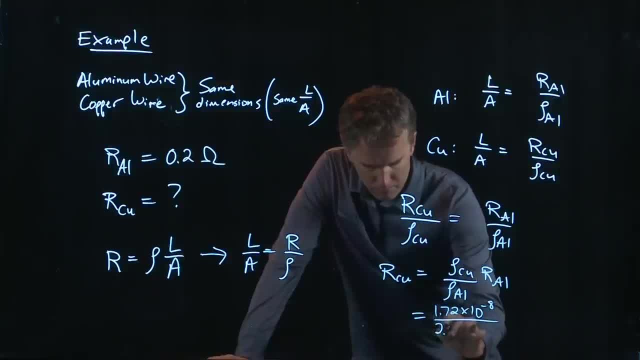 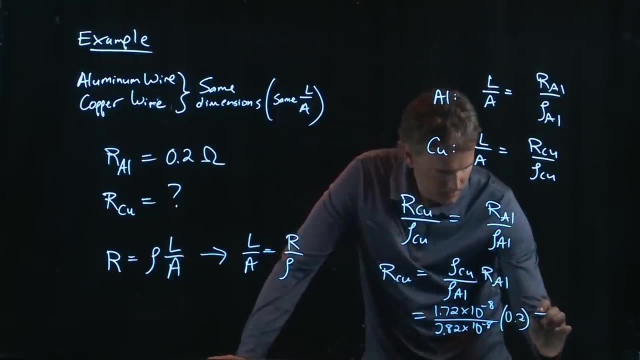 Those are SI units. Aluminum is 2.82 times 10 to the minus 8 ohm meters, Also ohm meters- And we have a resistance now of 0.2 ohms, which was given to us. So if you plug in all those numbers, I did it earlier. 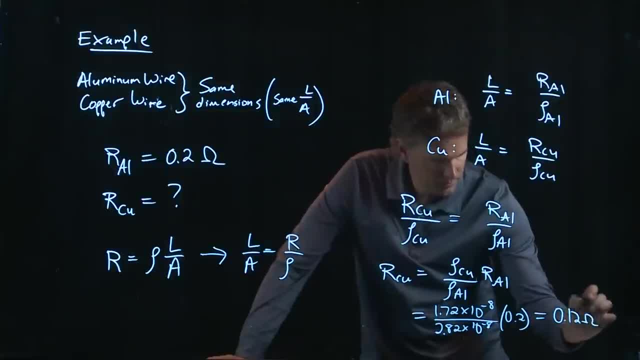 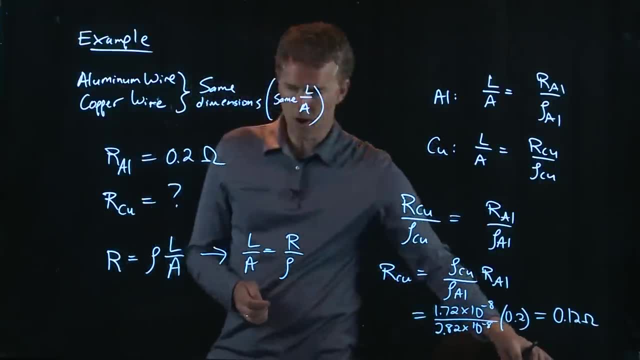 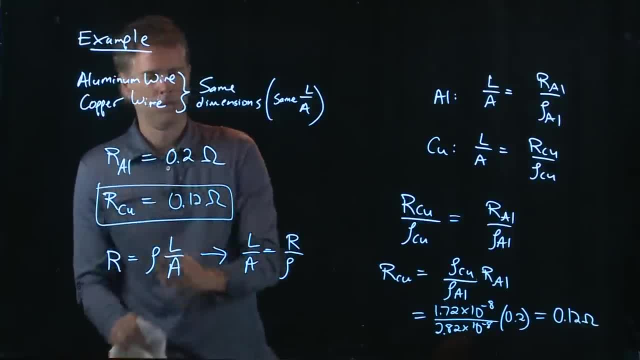 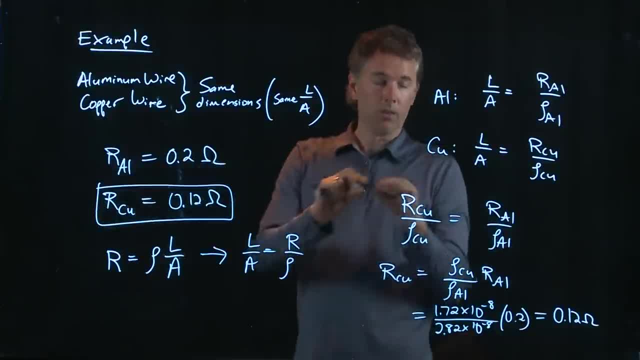 And so when you go to Home Depot and you buy a big long extension cord, those cables that are inside the thing, those are going to be made of something like copper, a good conductor. Aluminum turns out to be not a very good conductor. all right. If you spend more money on your extension cable, it will also be, you know, thicker. So what you'll notice is in the extension cord aisle there will be a 25-foot extension cord for $10.. And then next to it there will be a 25-foot extension cord for $20.. 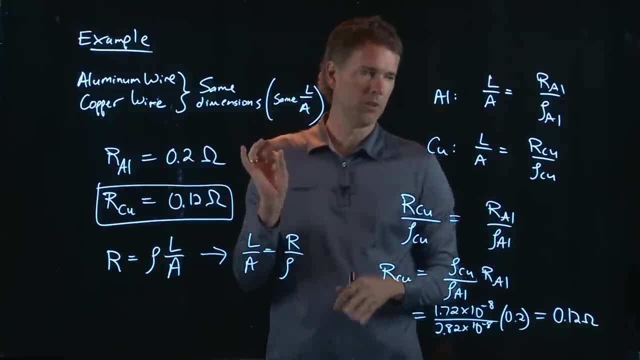 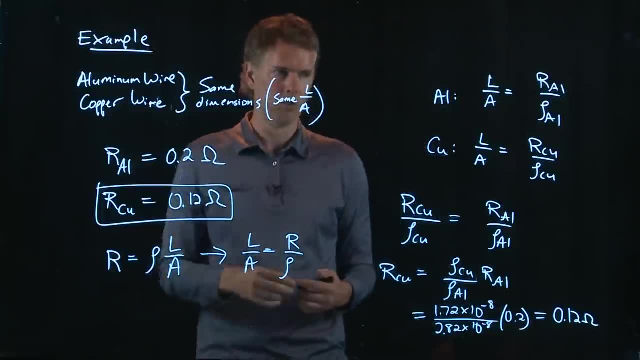 Look at the cross-sectional area A and what you'll notice is the more expensive one is thicker, It has a bigger A, which is ultimately going to get you a lower overall resistance. Okay, So let me just go ahead and show you a little bit more. 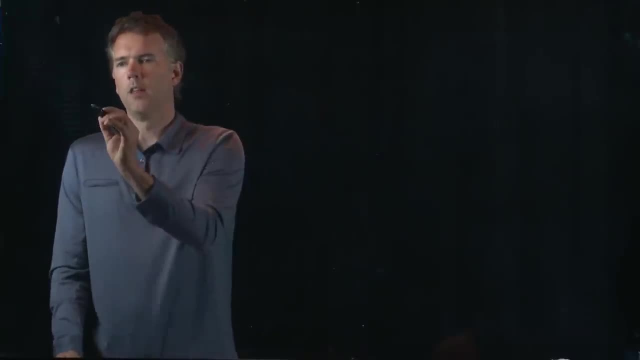 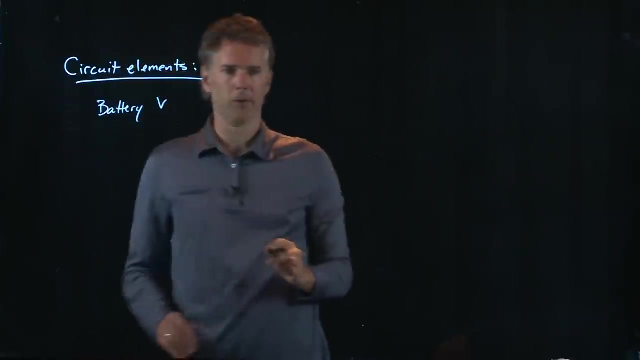 Okay, You can see a little bit of a difference. So let me just say a couple of things about Austin's question. There are a few circuit elements that are going to be key. One, of course, is the battery Battery. we write with a V and the way you write it. 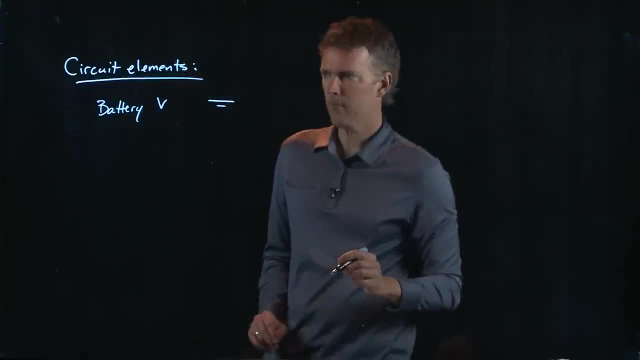 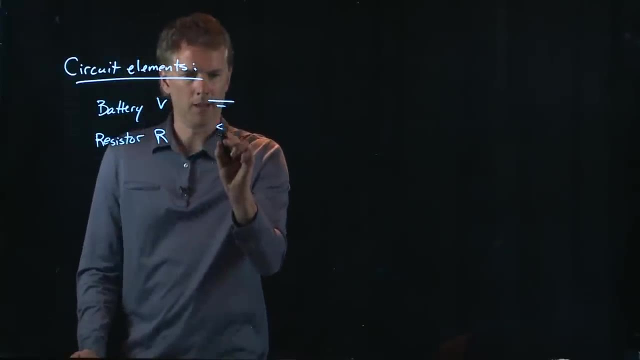 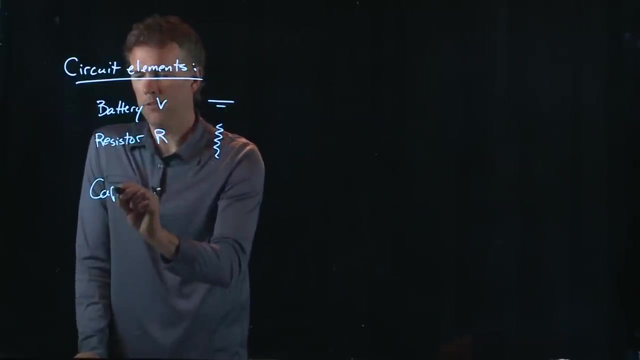 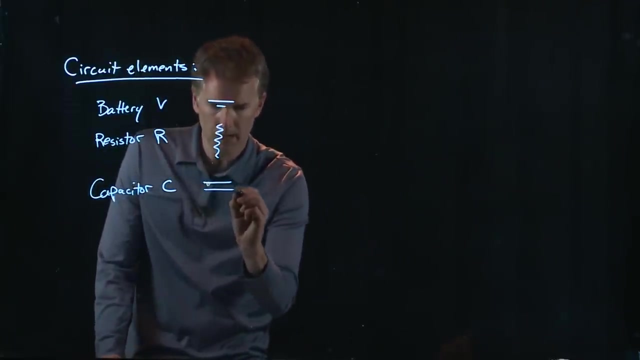 in a circuit is a long line and a short line. There's of course, the resistor R That you write with a sort of squiggly line like that: There is a capacitor C. A capacitor is two parallel lines. 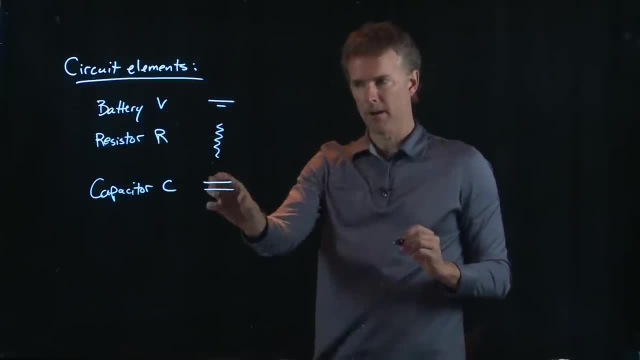 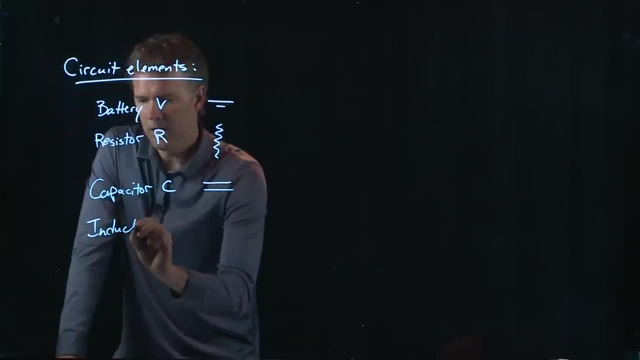 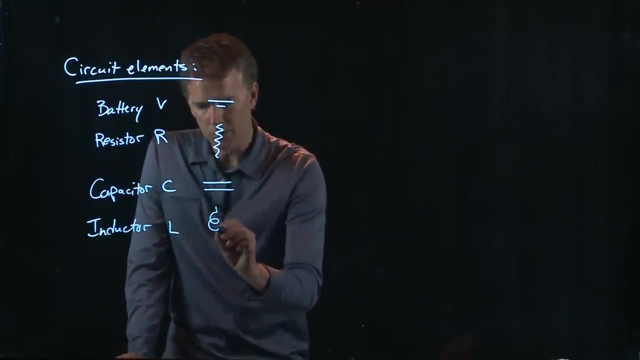 Okay, Not a long line and a short line. That's a battery Capacitor is two long parallel lines. And then the last thing is an inductor. Okay, We're going to write an inductor with an L and it actually looks like a corkscrew. 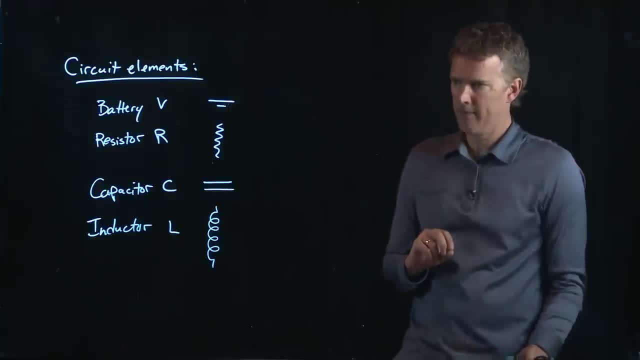 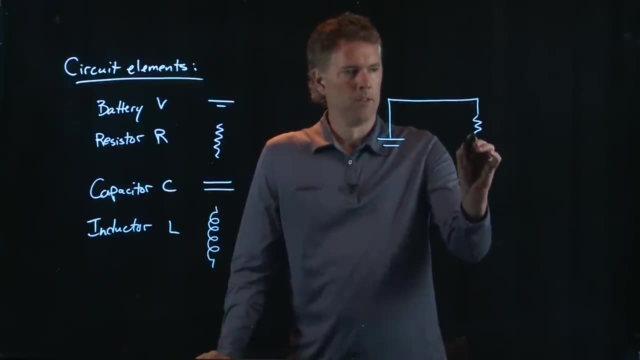 These are the four basic elements that you would have in a circuit, And so if I was going to draw this circuit, it might look like this: Resistor R, Capacitor C, Inductor L. And then if I was going to draw this circuit, 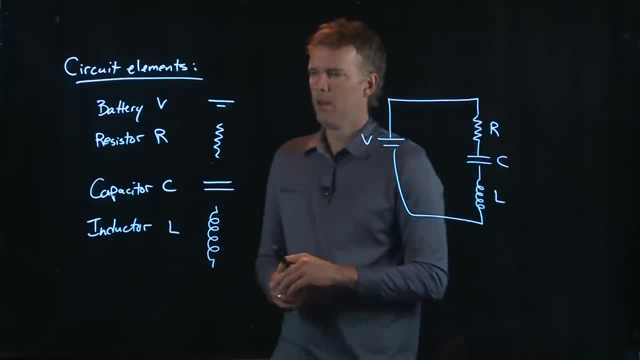 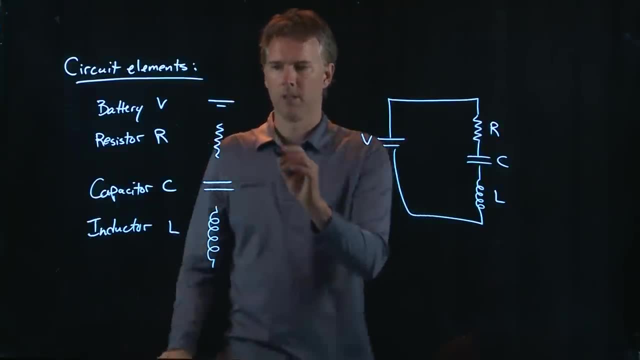 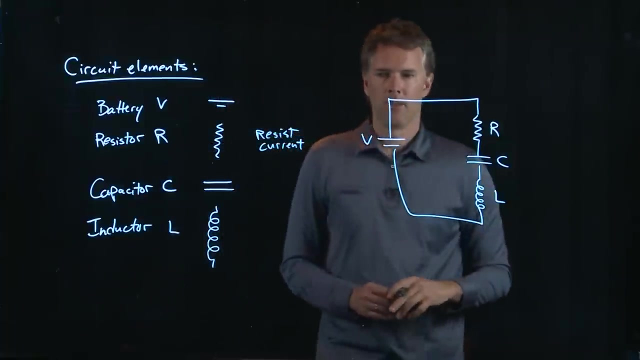 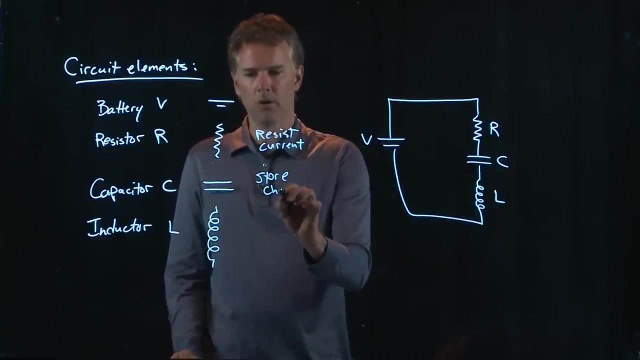 it might look like this, All powered by some voltage V. Now we know what resistors do, right, Resistors resist the current- Okay, They resist current Capacitors C. we know what those do: They store charge. 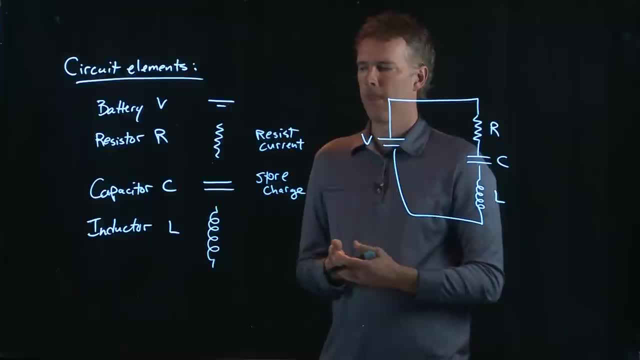 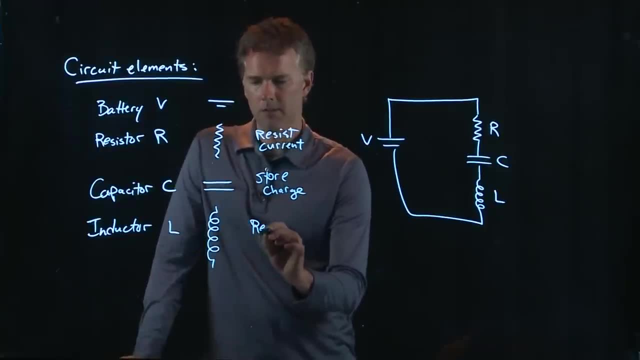 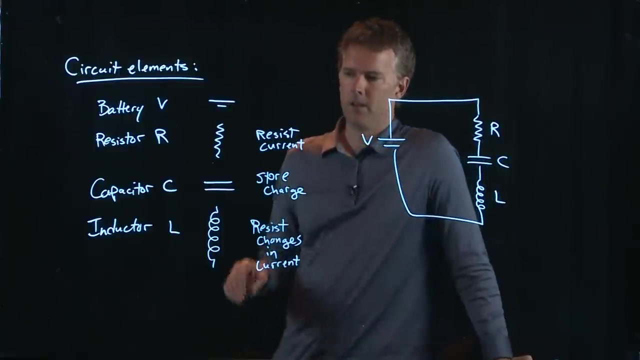 All right, You can power up a capacitor. You put a bunch of charge on it. What do inductors do? Inductors turns out they do something very special. They resist changes in current. Okay, Resistors just resist current in general. 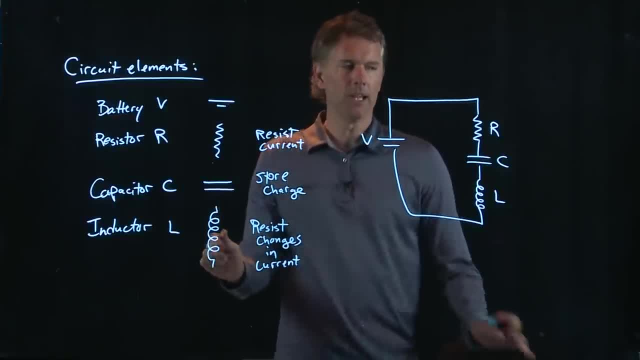 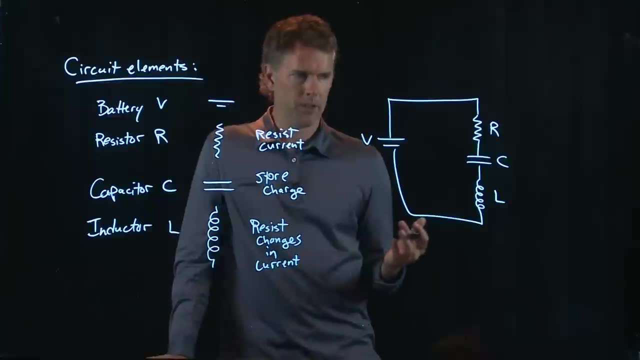 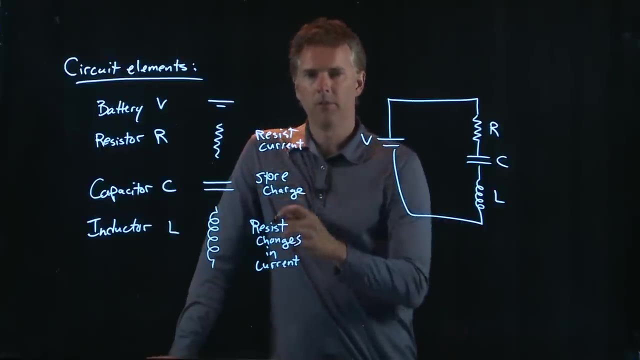 But inductors resist changes in current. Okay, It's hard to rapidly change the current through an inductor. There's another really cool way to think about this, and we haven't got to magnetism yet, but we will soon. When capacitors charge up. they store electric field, E Right. 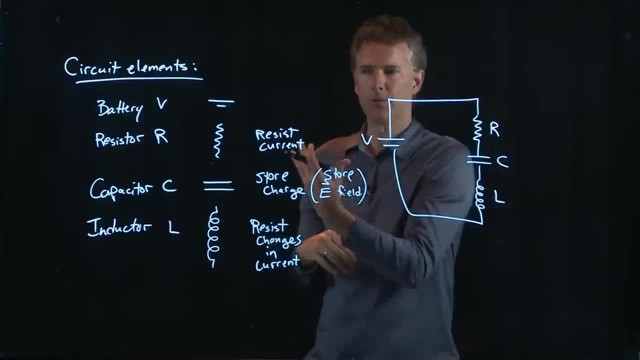 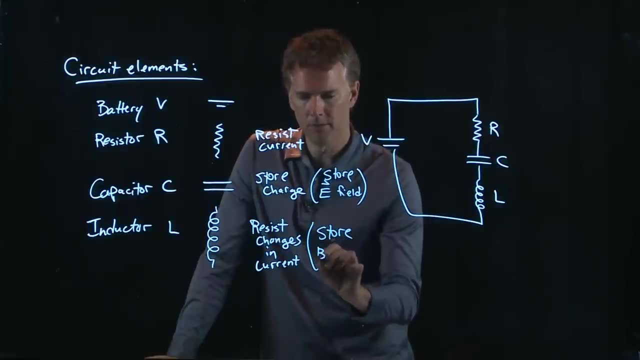 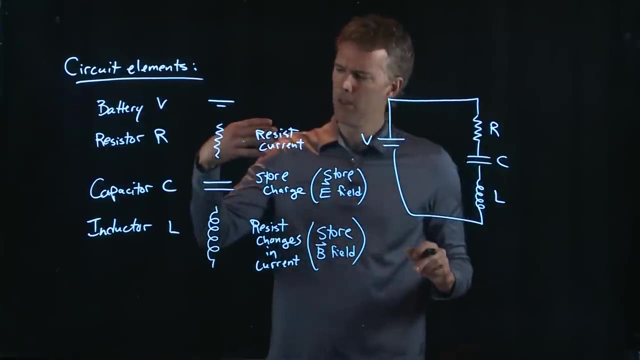 A capacitor that has a positive plate and a negative plate. there's an electric field in there, But inductors store B fields, which are magnetic fields, And it turns out that that means that they are resistive to changes in current. okay. 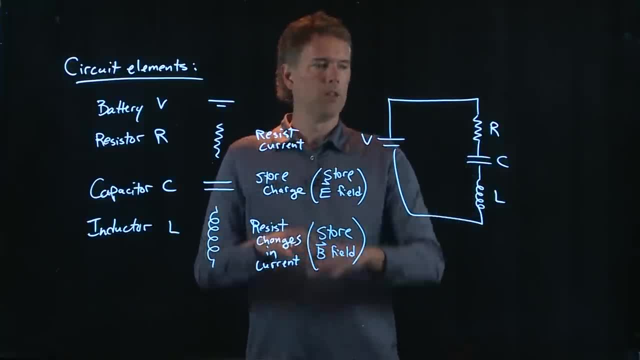 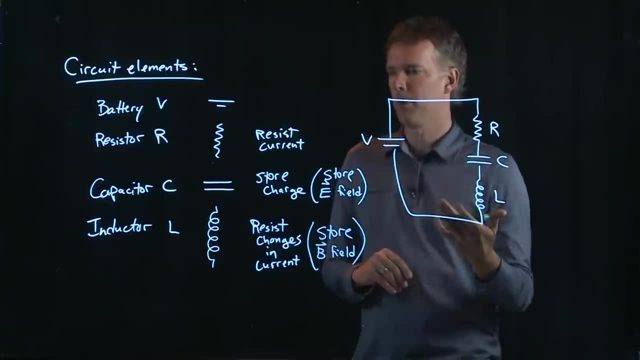 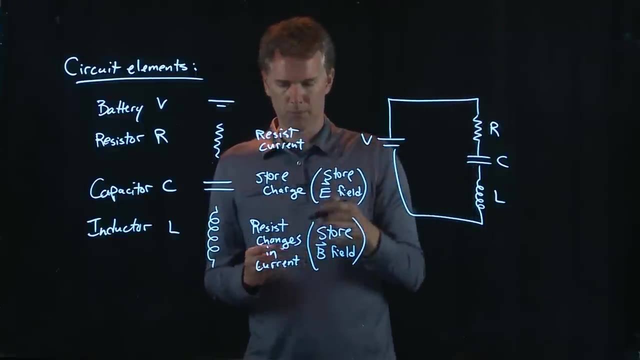 as opposed to just being resistive to current. These are the three elements We're going to learn all about how they play into the circuit and what they respond to. For now we've only introduced the resistor, But in the next couple of chapters. 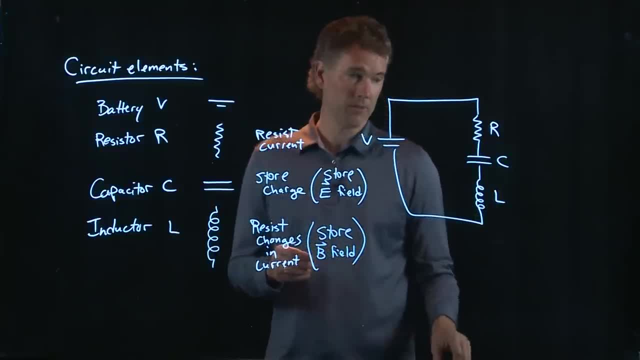 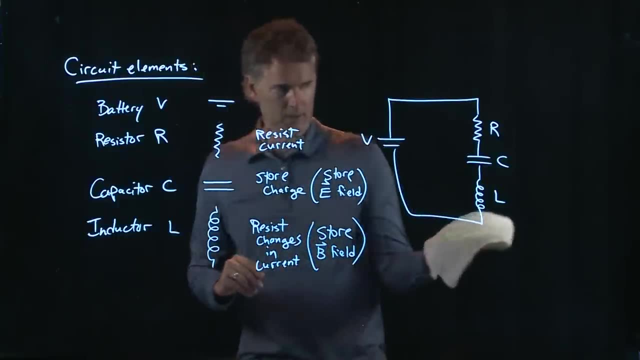 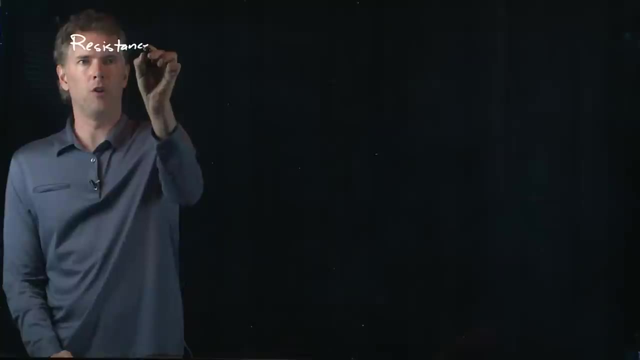 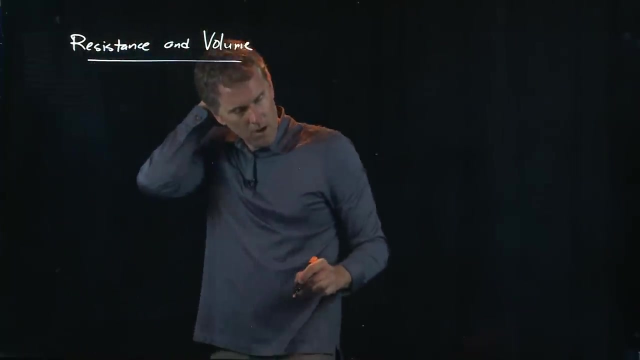 we're going to introduce the capacitor and the inductor. Maybe you guys are already looking at that in lab. Okay, Is that enough, Austin? Yeah, All right. Okay, Let's talk a little bit about resistance and volume, All right. 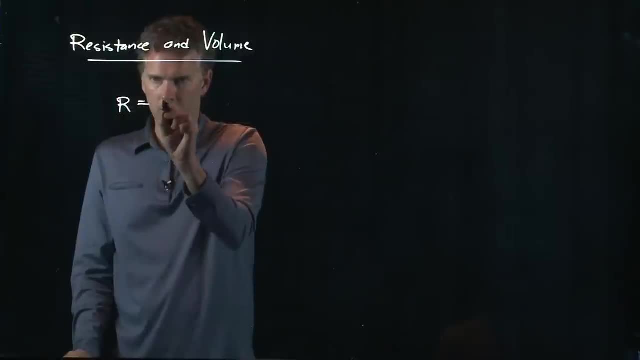 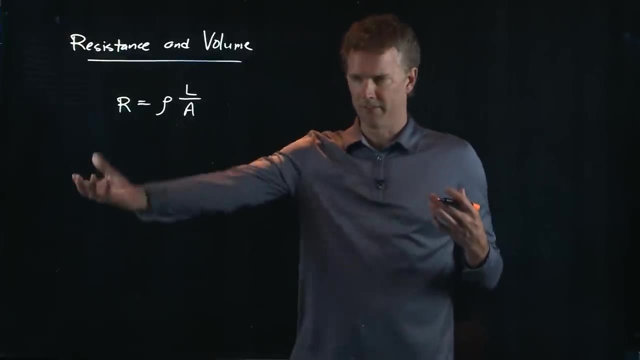 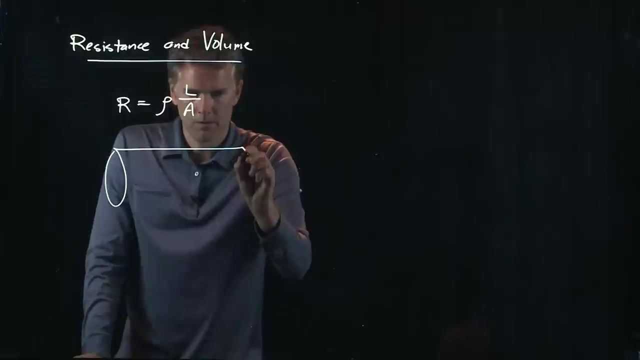 What we said earlier was: resistance is resistivity times L over A. Make your cable longer, it gets more resistance. Make it thicker, it gets less resistance. Let's think about this section of cable. here, A is, of course, a cross-sectional area. 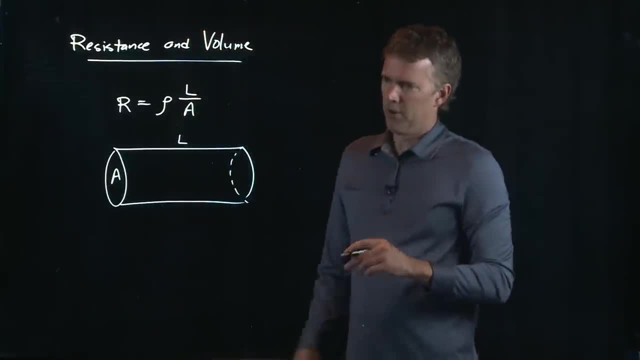 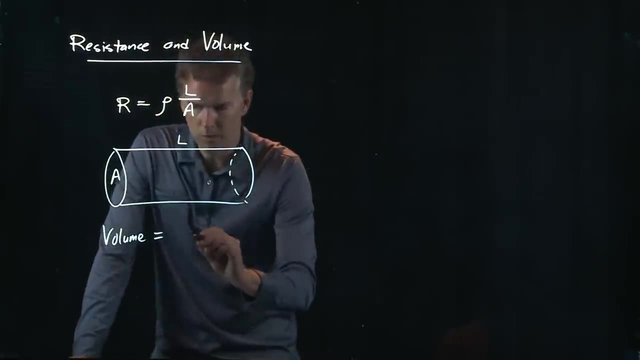 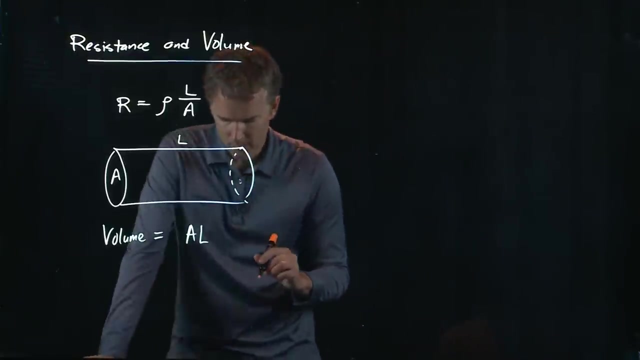 L is the length, So this is the length. This cable occupies some volume. The volume is just the cross-sectional area A times this length. right, That's the volume of this cylinder. All right, Can I factor that into the resistance? 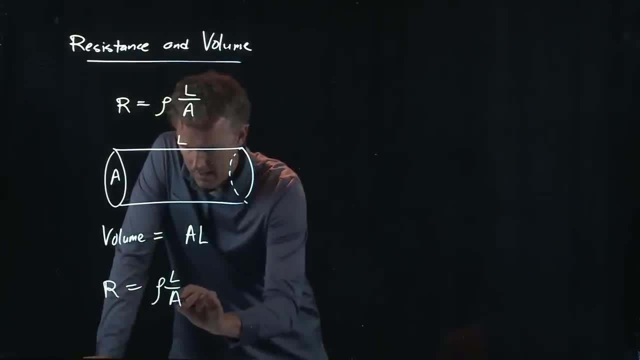 Resistance. we said was rho L over A. And I can say this is rho L over. What if I just solve this for A? I got A equals volume over L. So let's put that right here: Volume over L. And now I know what I do. 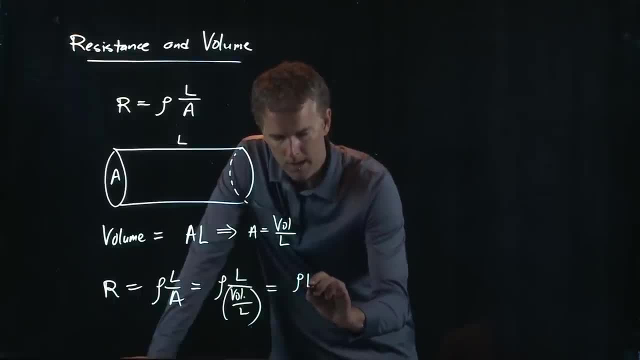 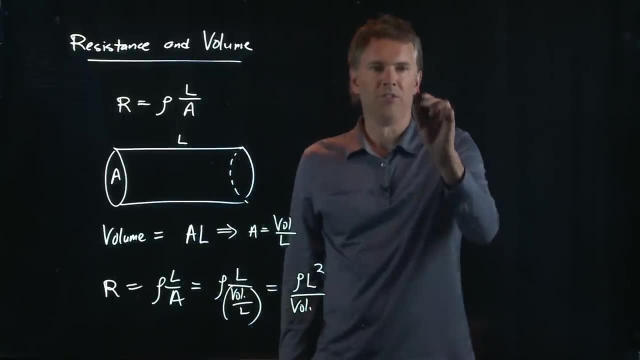 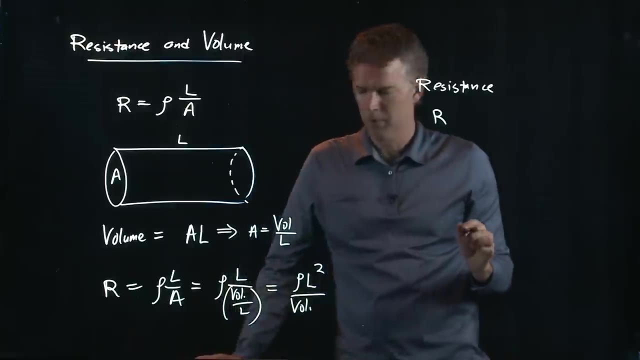 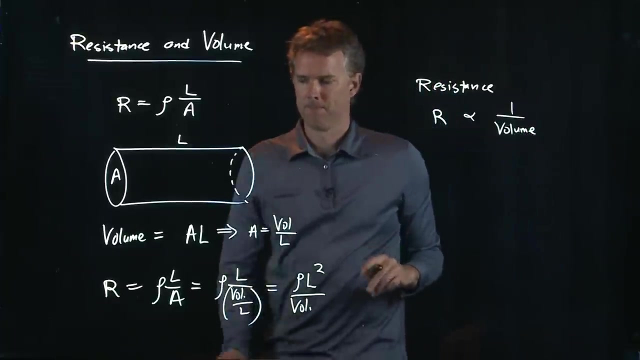 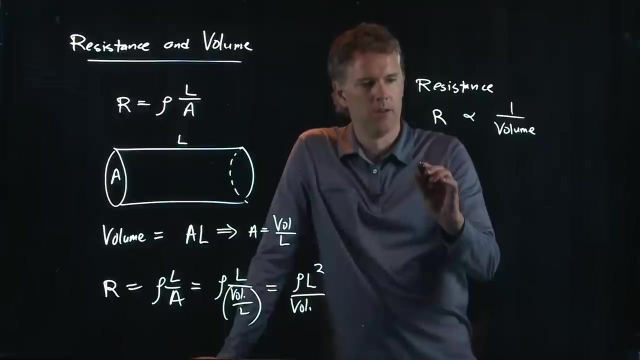 I flip the L's up to the top and I get rho L squared divided by volume. So resistance R Is in fact proportional to 1 over the volume, And this is in fact one way that you can measure stuff like blood flow. 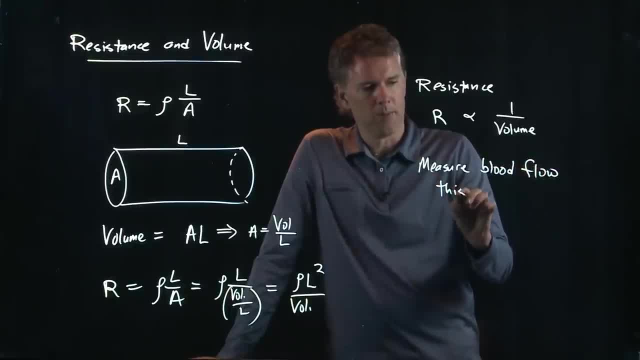 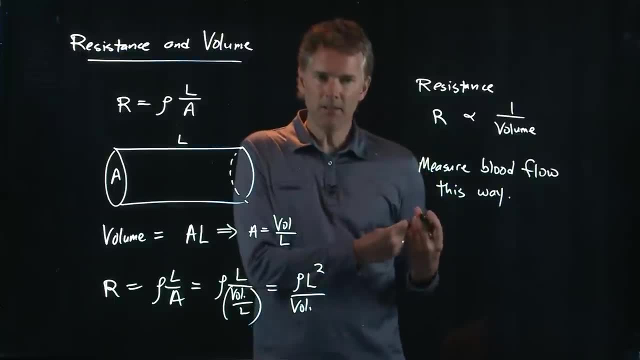 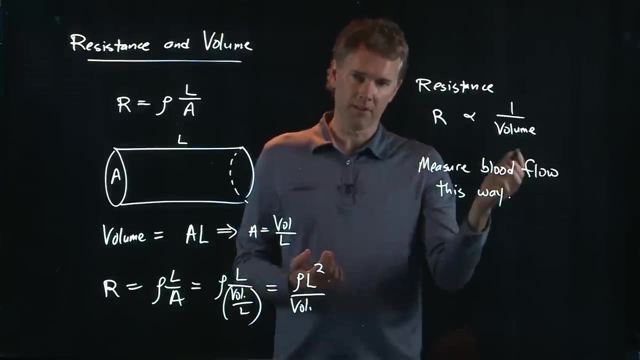 Okay, You guys are biology majors- a lot of you. You can, in fact, measure the blood flow this way, Because it's easy to measure the resistance of someone. Put an electrode here, you put an electrode there, You can measure the resistance of that circuit. 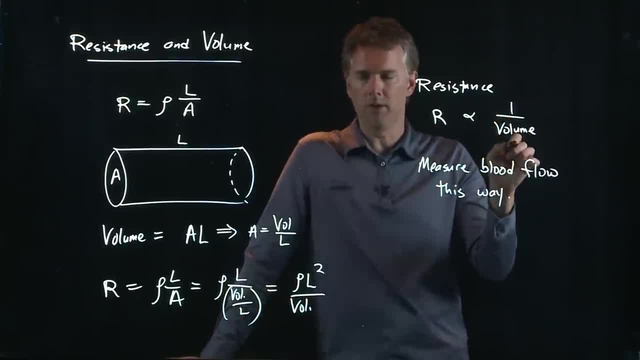 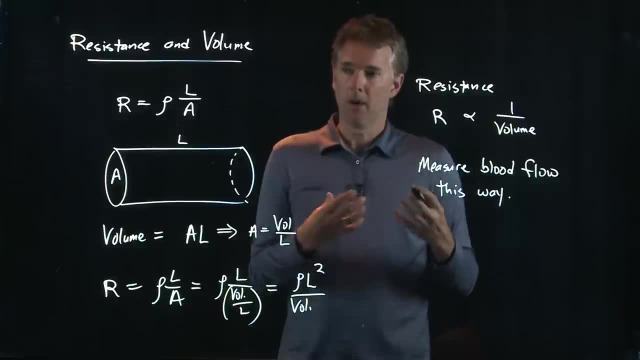 And if that resistance is in fact proportional to 1 over the volume, namely the volume of blood flow, then you can in fact calculate how much blood flow there is. Okay, Is that person suffering from high blood pressure? low blood pressure? 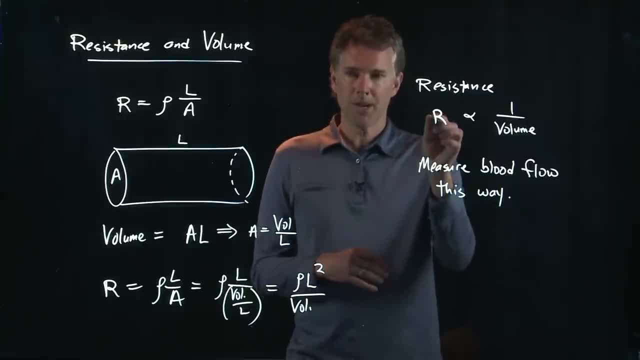 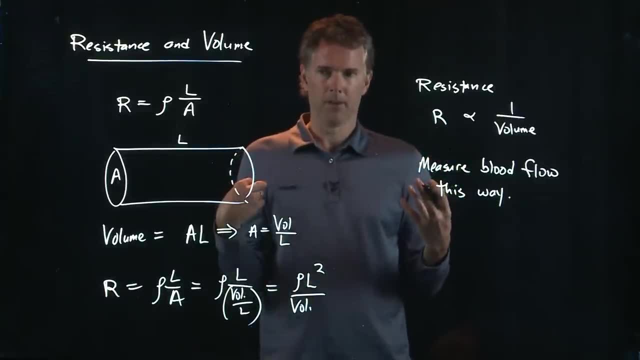 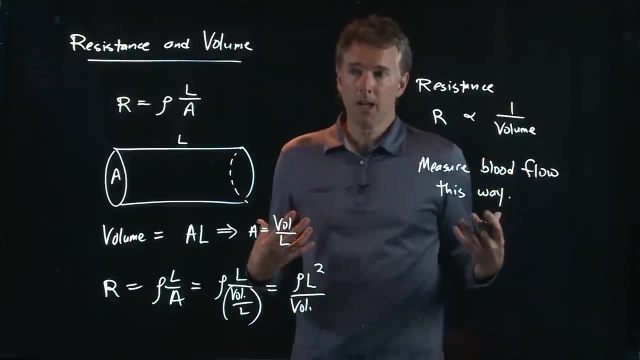 good circulation, Bad circulation. You can do it by measuring something in physics called resistance, And that's a lot of the times when you see those electrodes hooked up to people Right. One, they're measuring electrical signals from the heart firing, But two, they can also measure how much blood is in them. 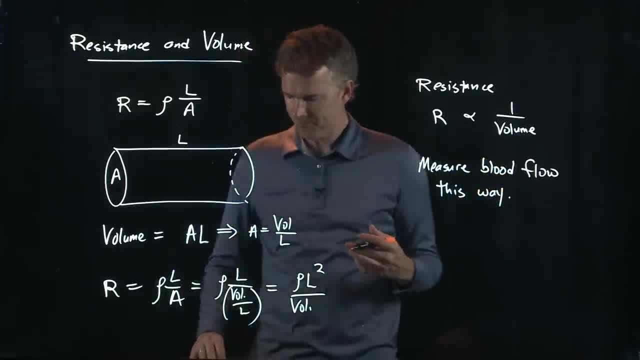 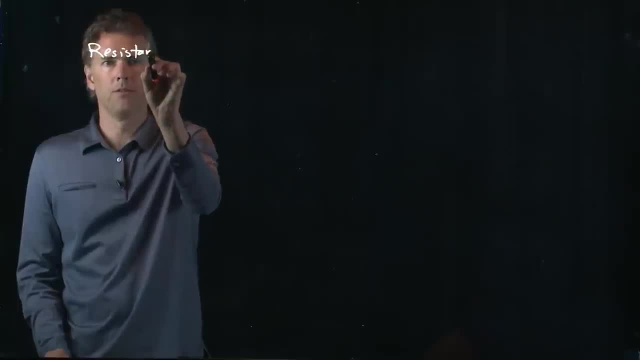 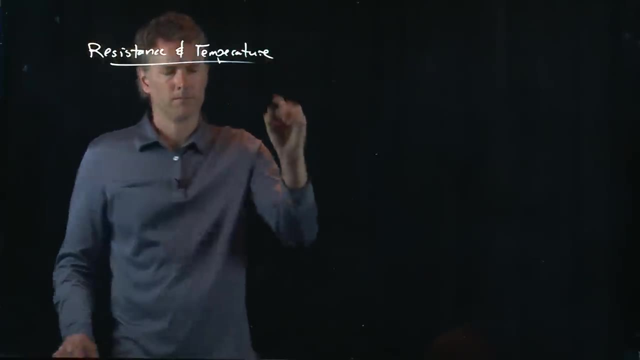 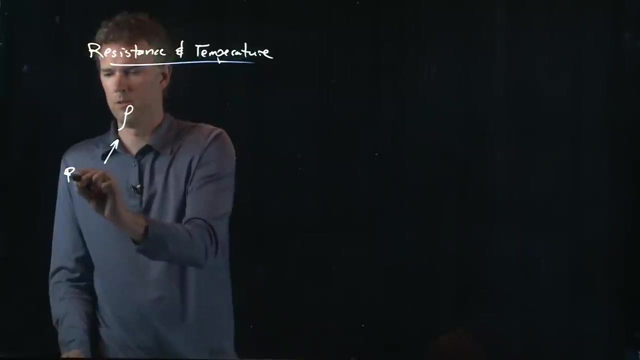 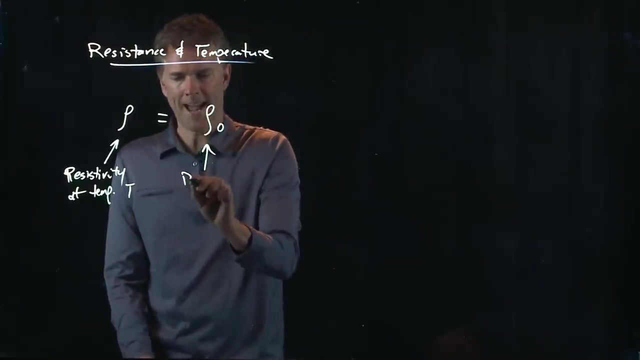 and how much blood is flowing in them, Which is kind of cool, All right. Resistance also varies with temperature. So resistivity at some temperature, rho, This is resistivity. rho at some particular temperature. T is in fact equal to rho. naught some calibrated resistivity. 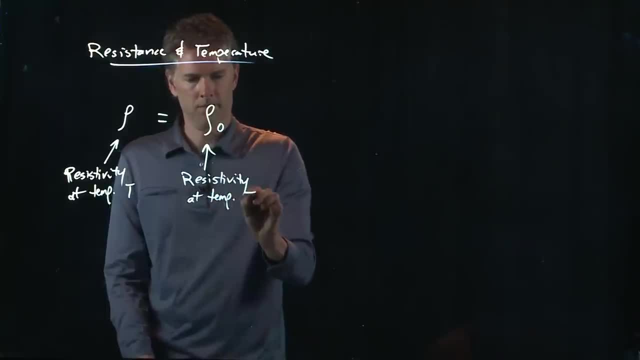 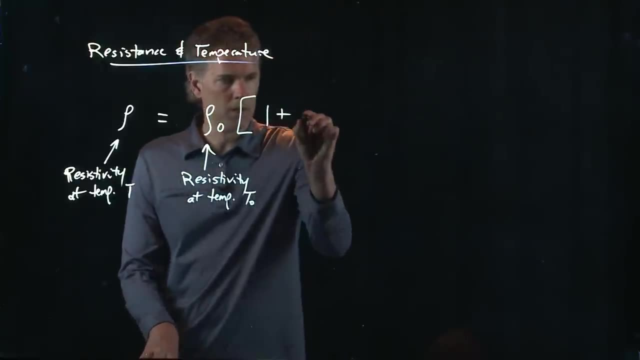 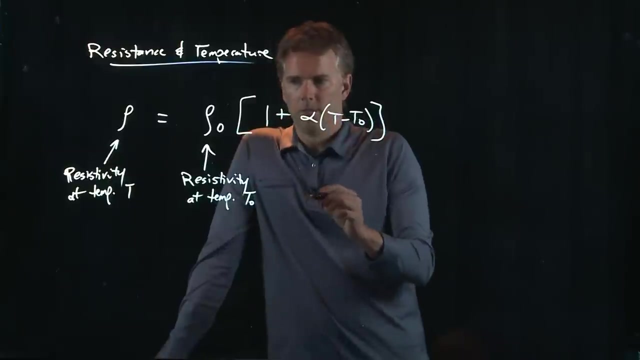 and that's the number one power. So it's a little bit less than or equal to the resistance. So it's a little bit less than or equal to the resistance. And then there is this scaling factor, which is the following: One plus alpha, T minus T naught. 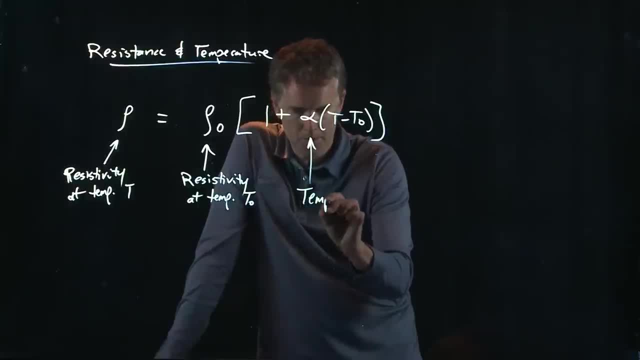 What are all these things? One is, of course, the number one. What's alpha? This is called the temperature coefficient of resistance. Okay, One is square root, One is minus. Two is minus. this is still the temp T and the temp T not. okay, this thing is rather critical. 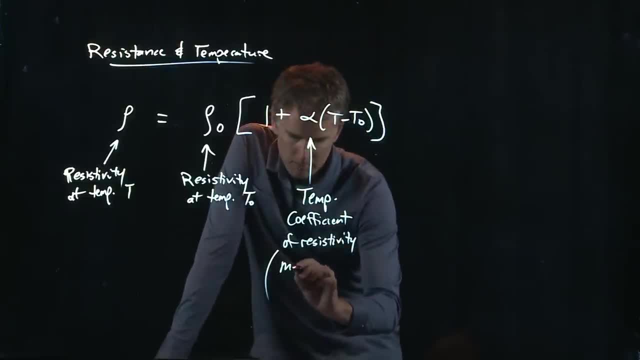 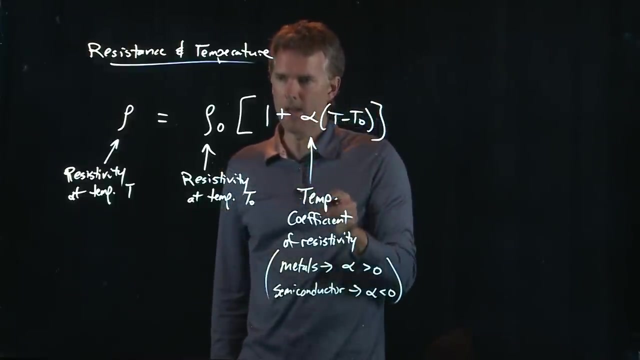 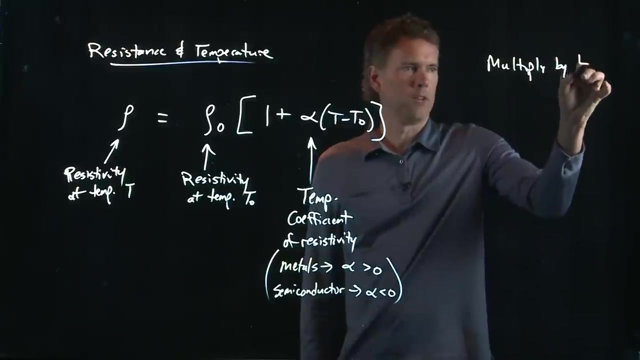 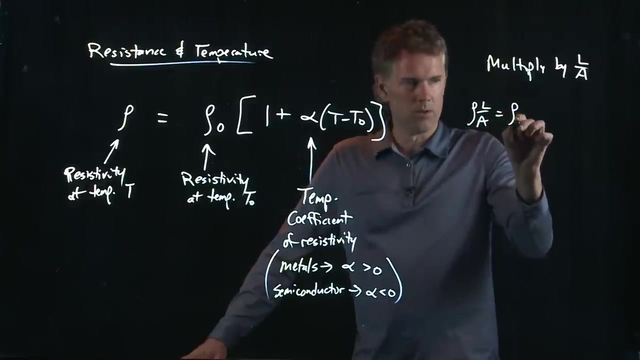 to how the resistor behaves. and if it's a metal, then alpha is a positive number, but if it is a semiconductor, then alpha is a negative number. all right, let's multiply both sides by L over a, and then we can change this into resistance. so if we multiply both sides by L over a, what do we get? we get Rho. L over a equals Rho. 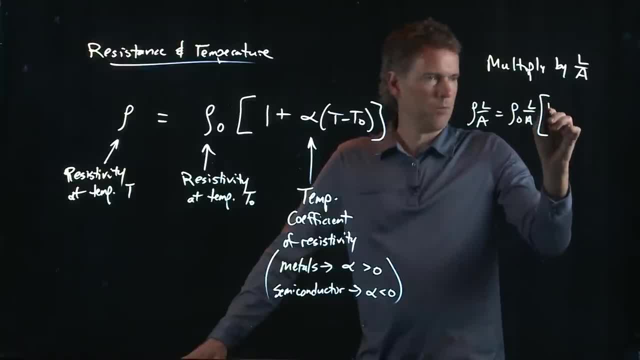 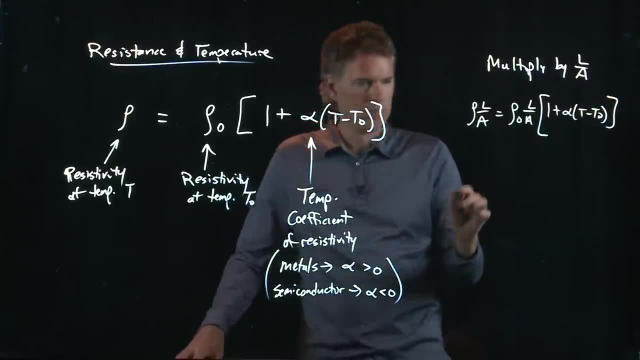 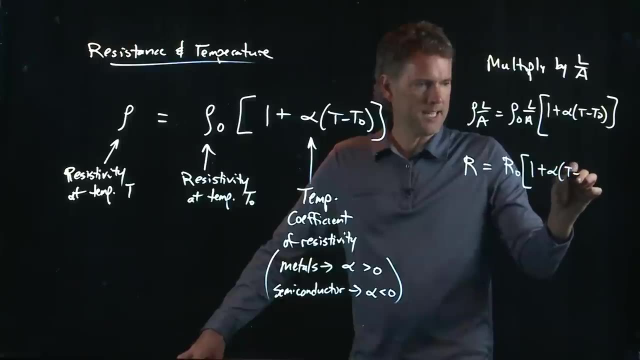 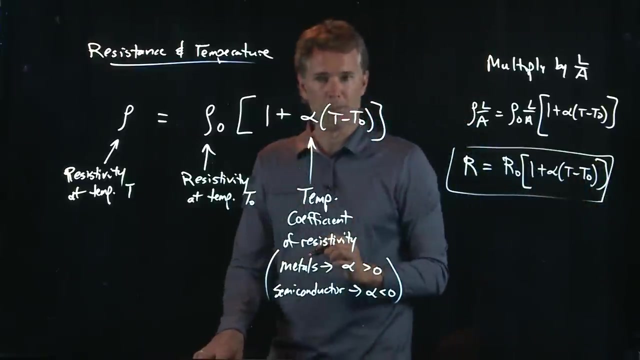 naught L over a times 1 plus alpha T minus T naught. and now this thing is just a resistance R equals R naught 1 plus alpha T minus T naught. okay, and this is a relationship between resistance and temperature. so if I have a normal metal, 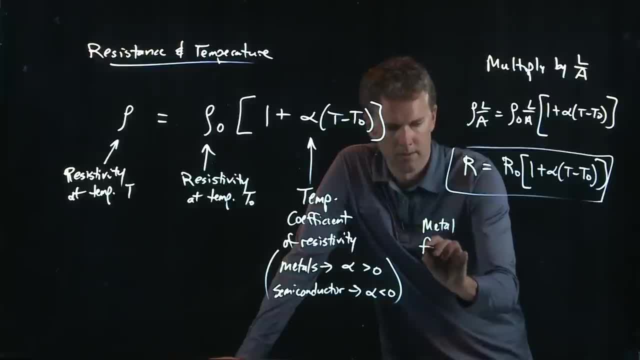 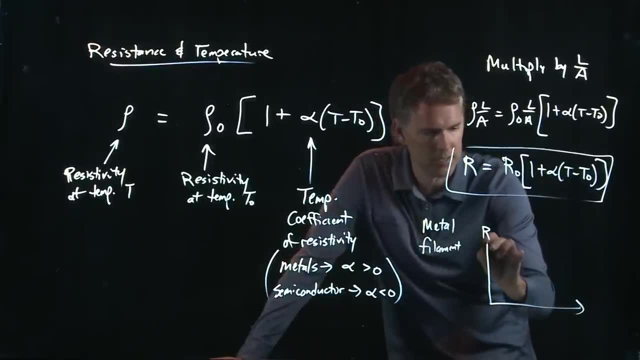 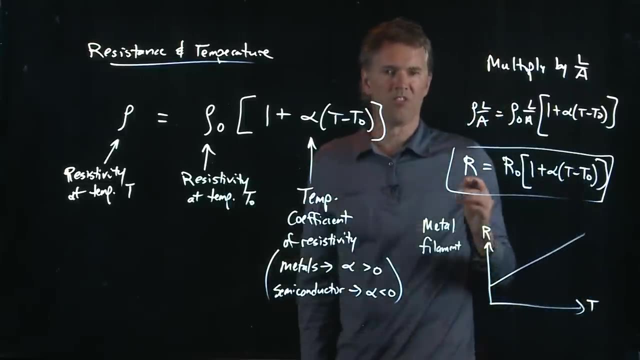 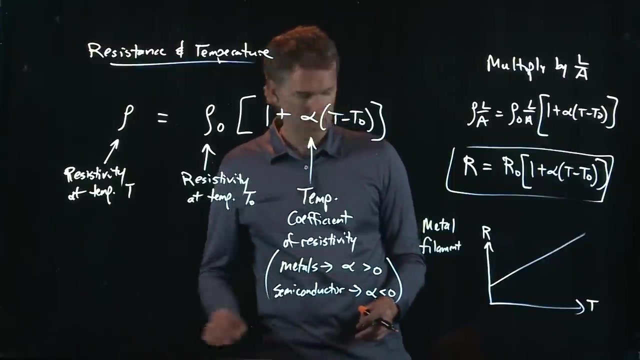 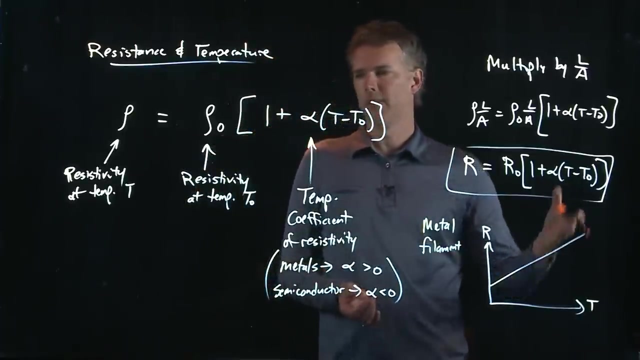 filament, and we plot out R as a function of temperature, T. what it looks like is this: and the resistance increases with temperature. and you might be doing experiments of this kind in the labs, where you turn on a light bulb and when the light bulb is cool, cool it has a very low resistance, but as it gets hotter and hotter it increases its. 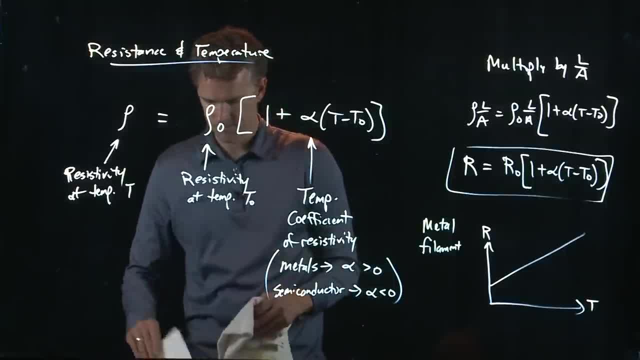 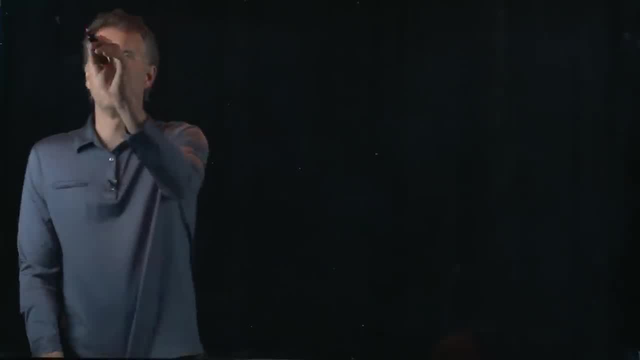 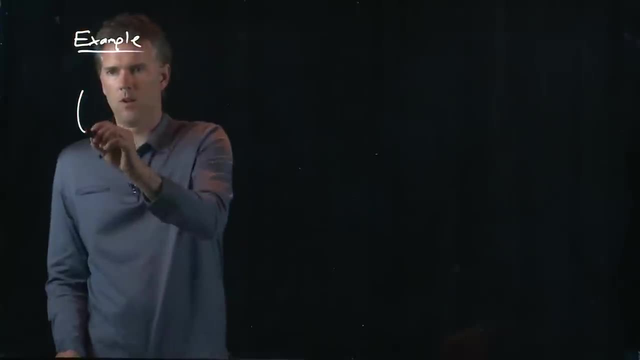 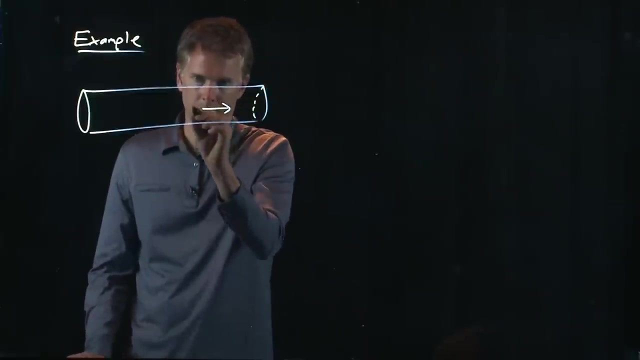 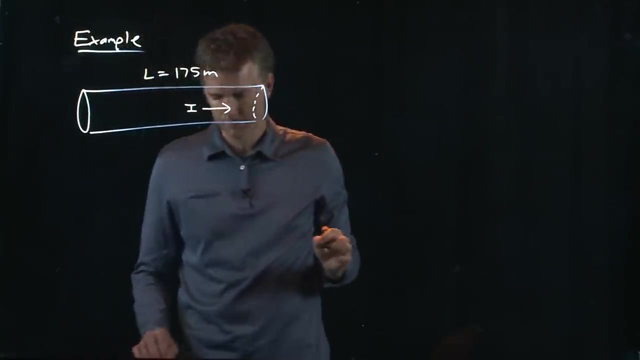 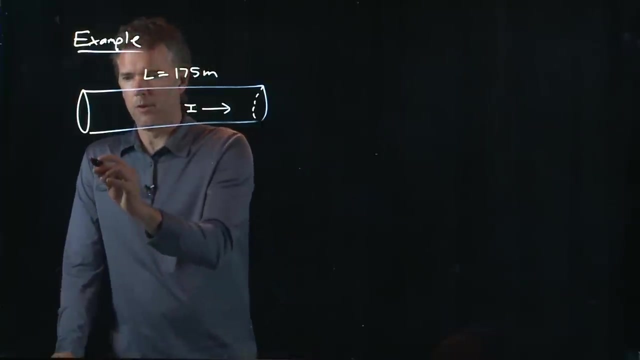 resistance. Okay, let's try another example. Let's take a long, thin wire and let's run some current down it And let's say that this thing is pretty long, L is 175 meters. There is some voltage which is driving current down this thing, and so there is some voltage. 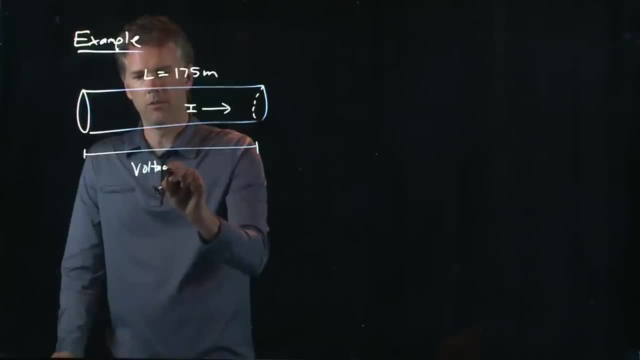 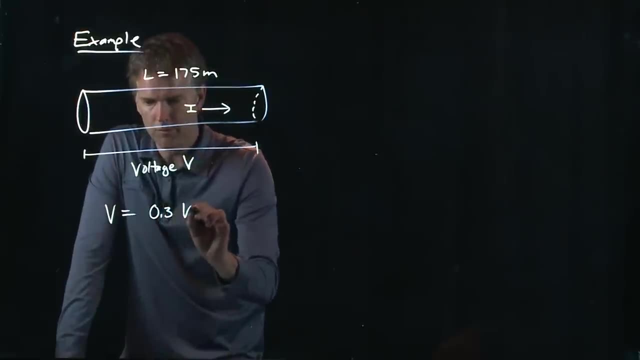 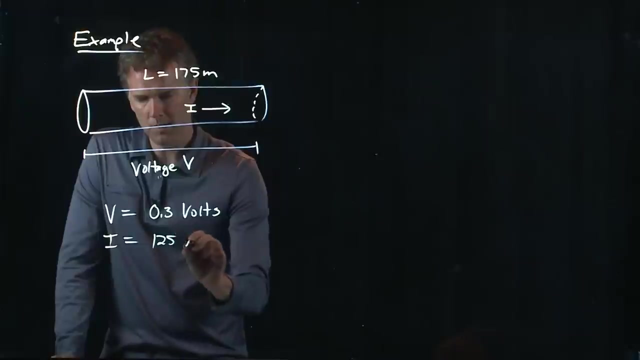 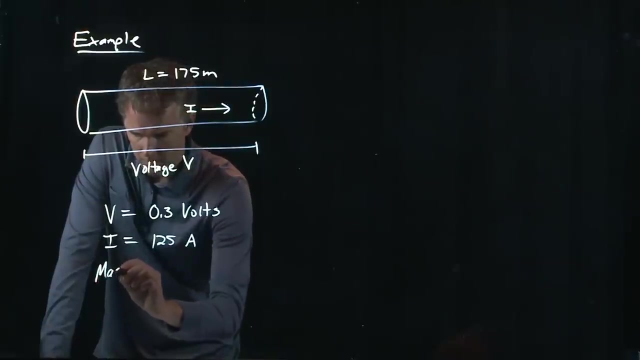 difference between the two ends, And let's tell you that that voltage V is 0.3 volts. Okay, And let's tell you that the amount of current flowing in this thing is 125 amps. And let's say that this thing is made up of aluminum. 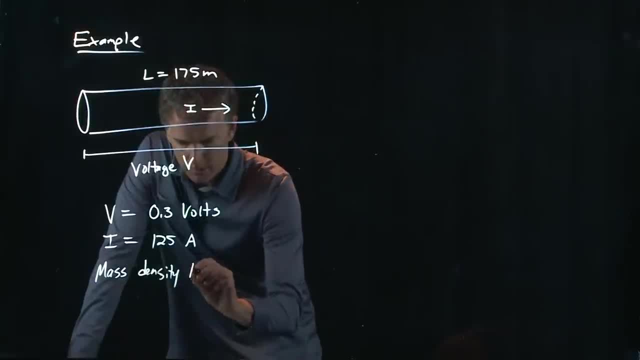 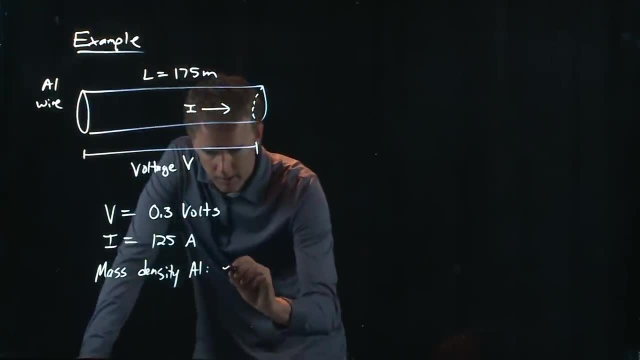 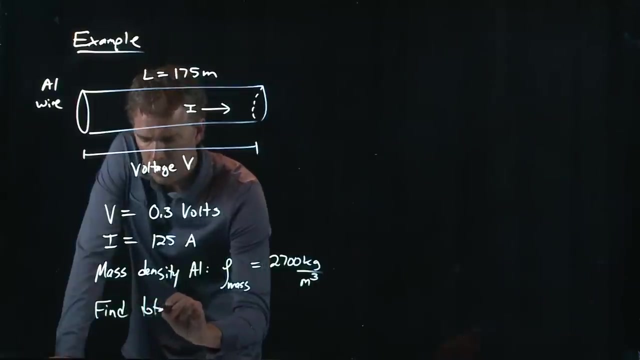 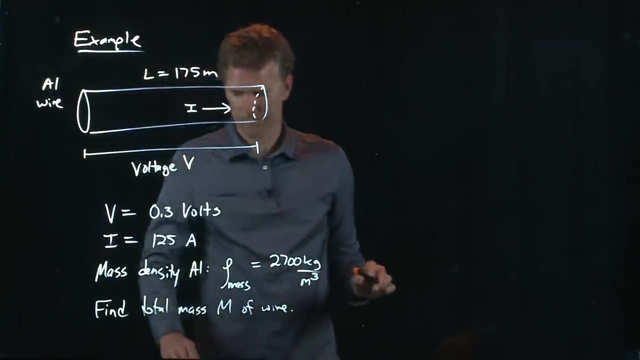 Mass density is of aluminum. so this is an aluminum wire- is the following: Mass density: rho. Mass density rho is 2700 kilograms per cubic meter And let's do the following. Let's find the total mass m of this wire. Okay, it might seem like we don't really have enough. 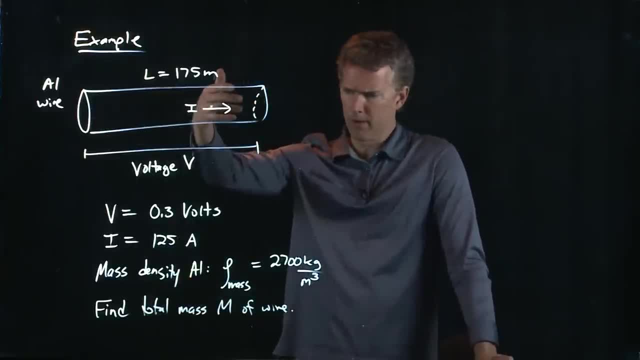 information right, Because we just talked about how much current is flowing and somehow we want to get the mass, And so let's do the following. Mass density: rho is 2700 kilograms per cubic meter, So the mass of the wire seems a little strange, but the key is that it's. 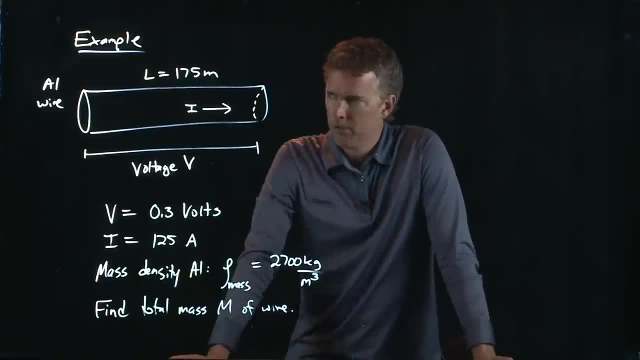 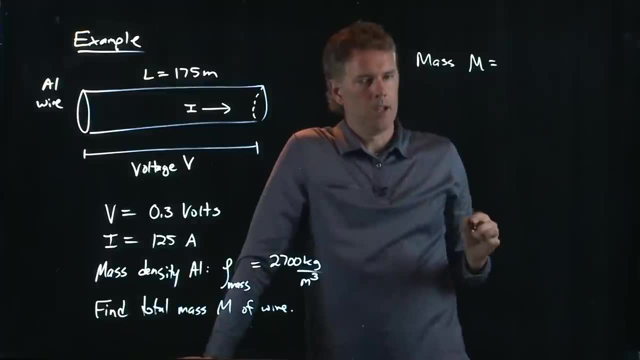 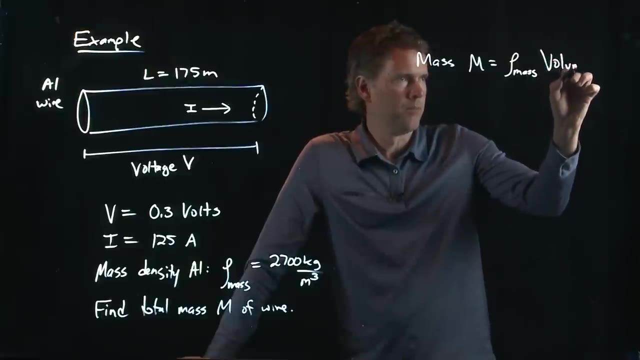 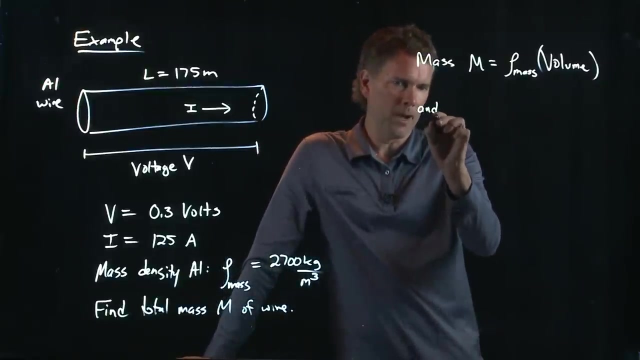 aluminum, and we know a little bit about aluminum. So how do we do this? Well, mass m is just going to be the mass, density rho times the volume. Okay, mass is density times volume. But we also know a little bit about resistance. So 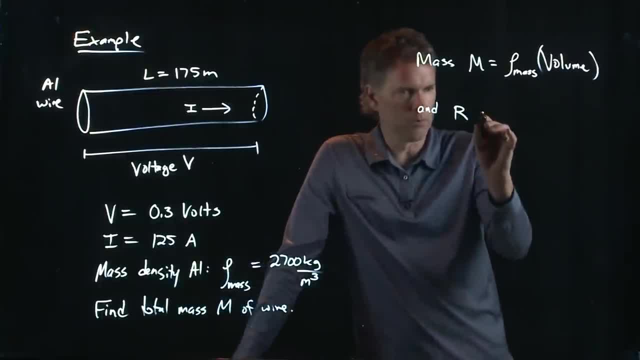 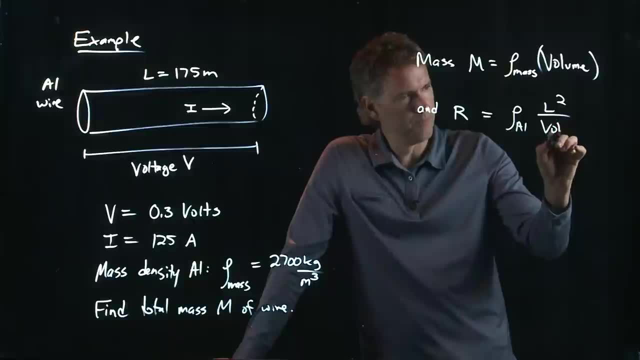 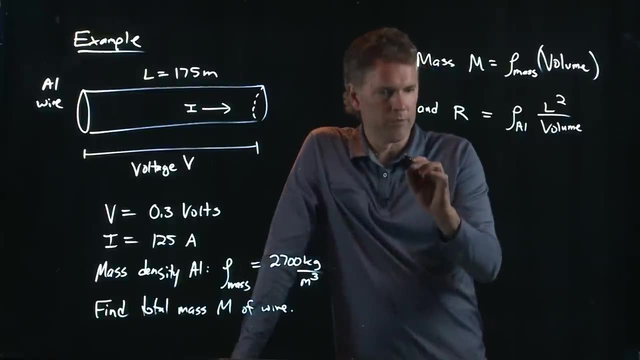 resistance. We know that resistance is going to be R of aluminum times L squared over the volume, And we derived that a second ago, And so now we can rewrite this for the volume. Volume is equal to what I'm going to multiply across by volume. I'm going to divide by R. 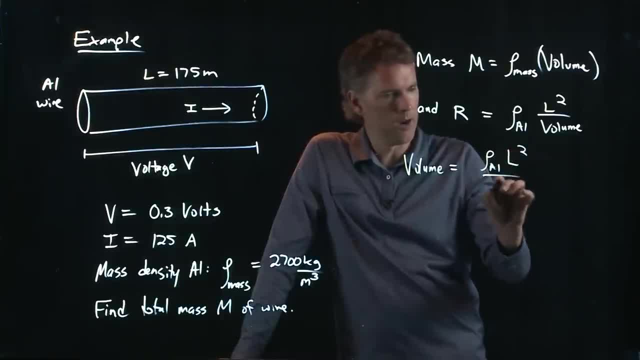 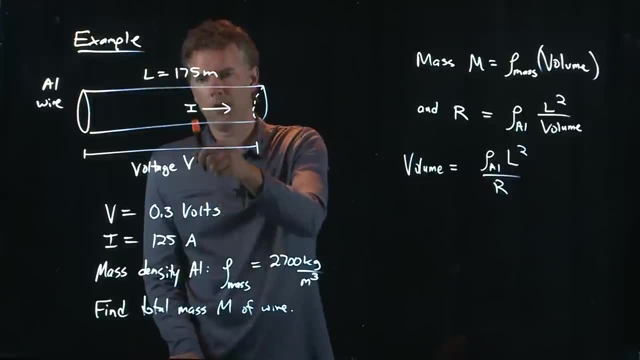 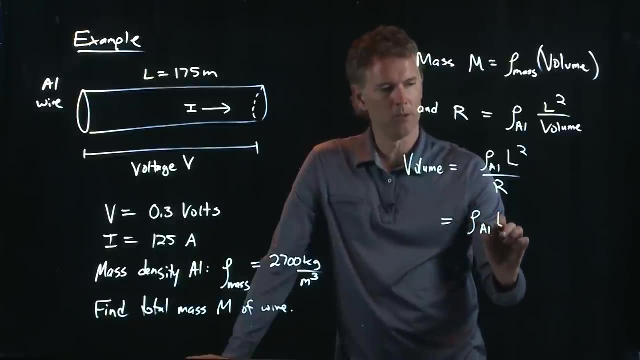 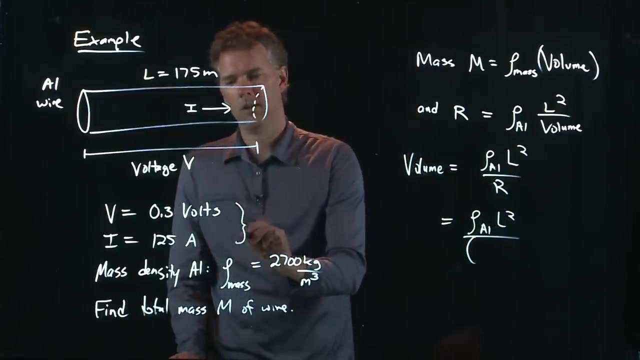 so I get rho aluminum L squared all over the resistance R, but I know the voltage and I know the current, And so in fact I do know the resistance R. This becomes rho of aluminum L squared divided by R, and we know that V equals I R, and so R equals V L squared, And 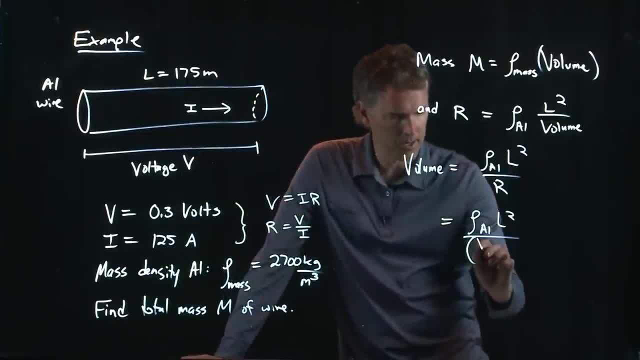 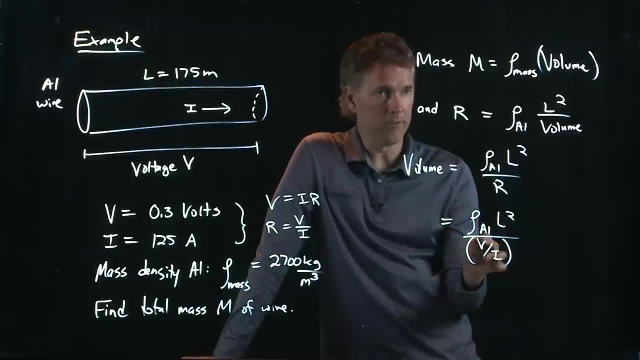 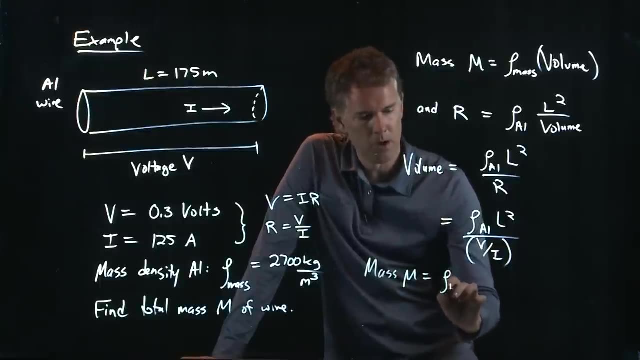 over I. So we can put that right here: V over I. And now I think we almost have all the numbers that we need for there, but we still want to get mass. So mass M is equal to rho mass. This is unfortunate that we're using rho for mass density. 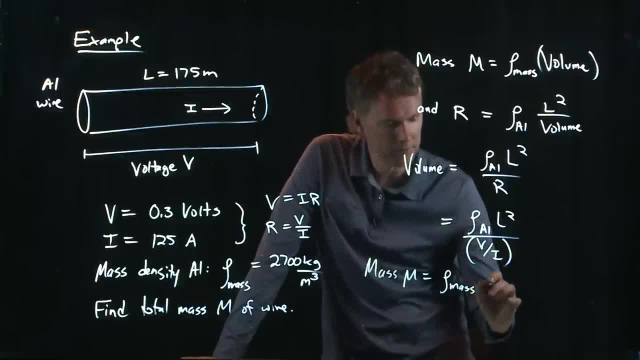 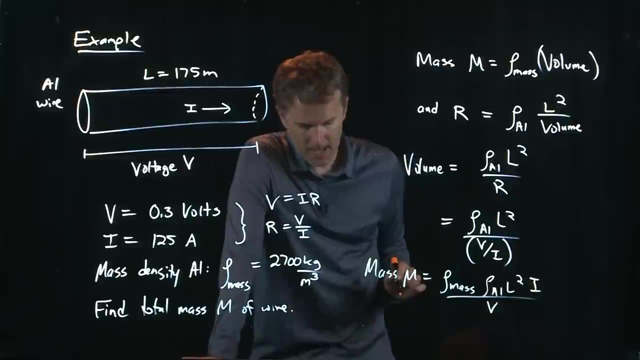 and also for conductivity or resistivity. but that's just how it goes And we've got to multiply by volume, which we said was this. So we get rho aluminum L squared, That I flips up in top and we get a capital V for voltage in the bottom And 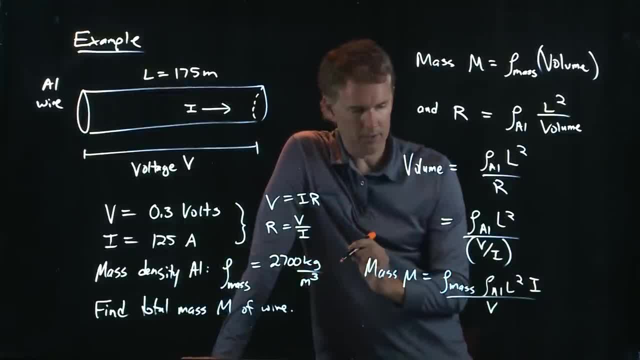 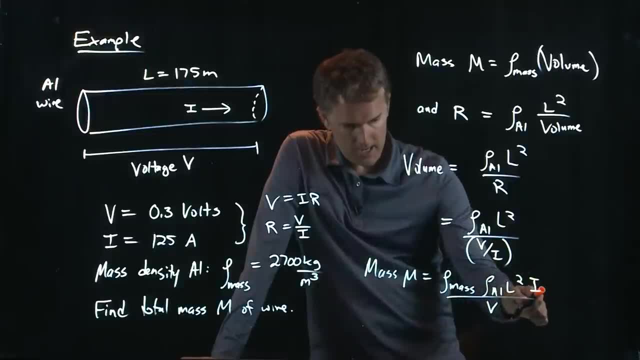 now we have all those numbers. We have the mass density right there: 2,700.. We know what rho aluminum is. We just did that earlier. We can look it up in the book. We've got I, we've got L squared and we have V, And if you plug in all, 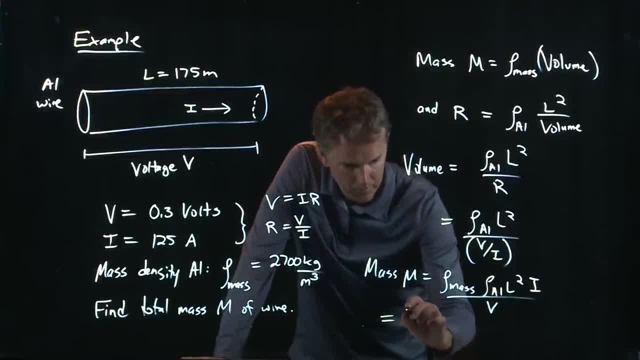 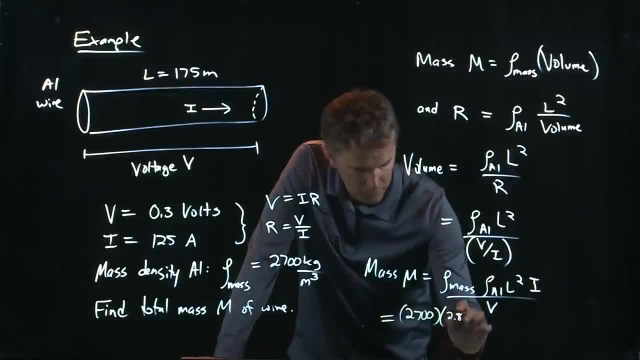 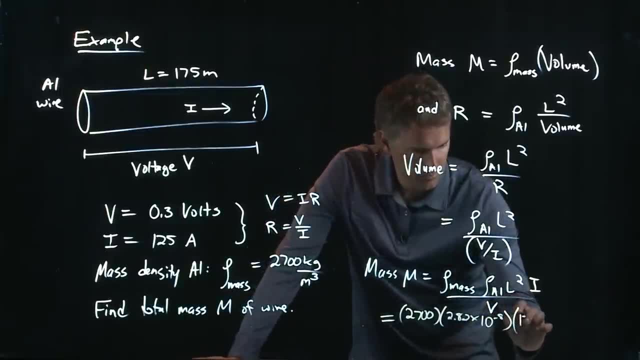 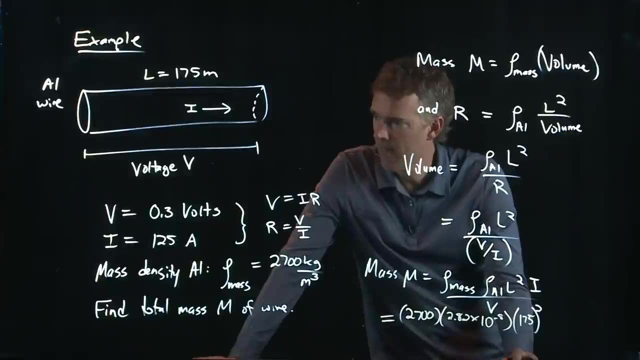 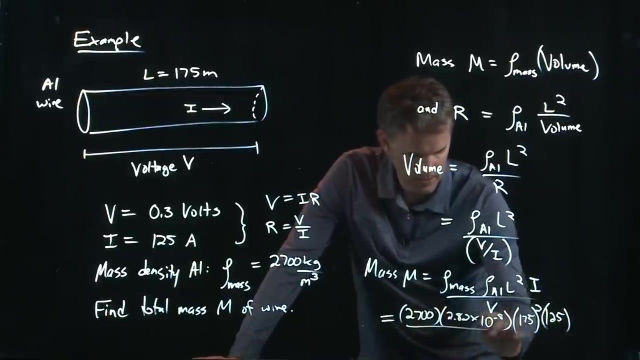 the mass density, Aluminum we said, was 2.82 times 10 to the minus 8. L was 175.. I was, what did we say for I 125, right, 125 amps. And then let's look at the. 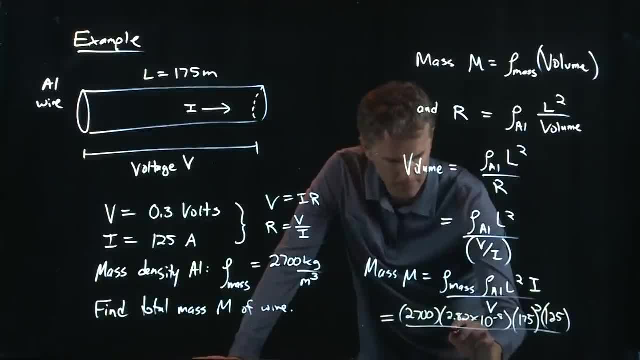 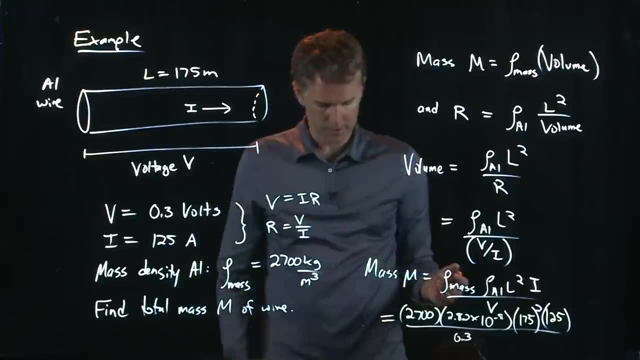 mass density. Let's just do it again. OK, We've got the mass density, that's entered into the calculator, So you get the mass density. Let's divide the whole thing by V, which was 0.3 volts. OK, And if you punch in all those numbers in, 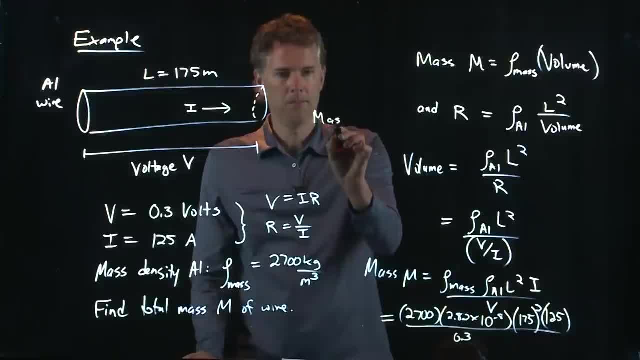 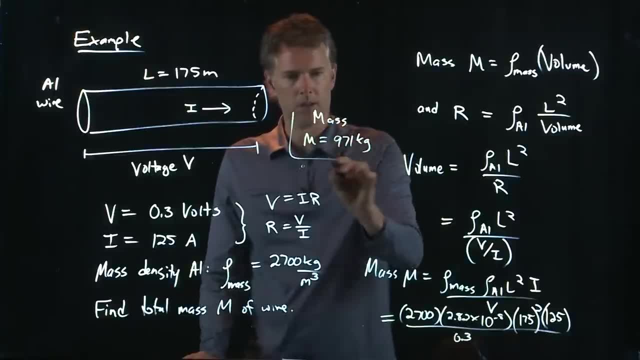 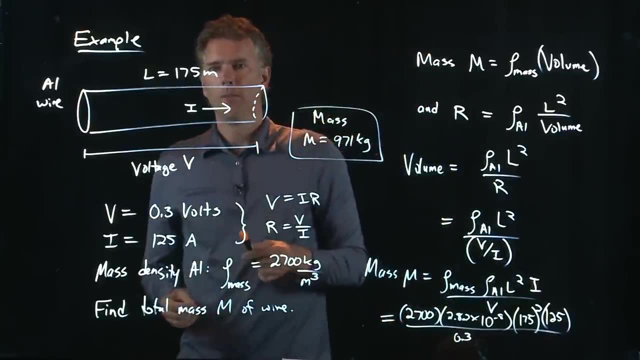 your calculator you can double check me. but I got a mass m for that wire of 971 kW. That's too much. But if you watch the video, you're going to see I'm not getting a lot of kilograms. which is a pretty big wire right, It's almost a metric ton, but it's long and 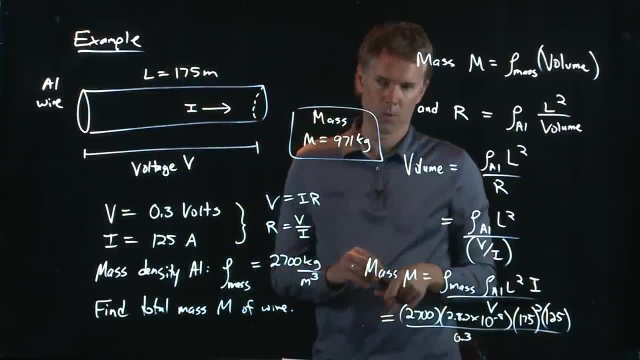 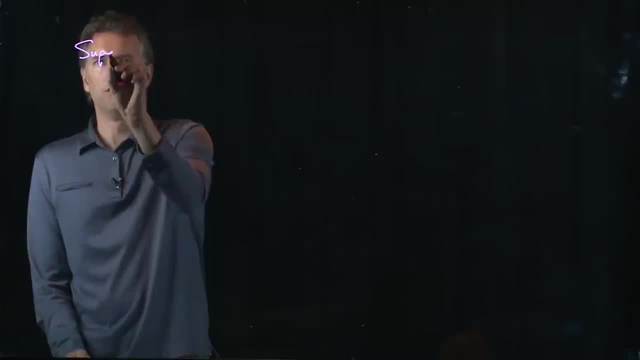 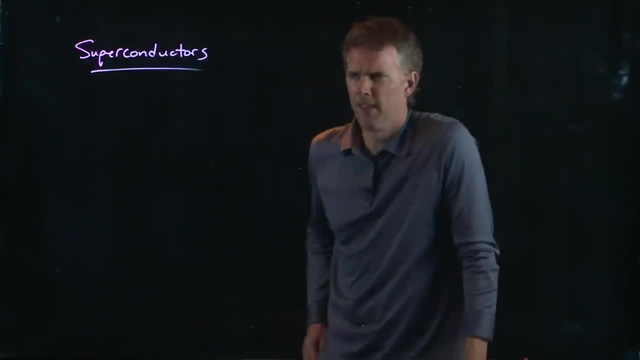 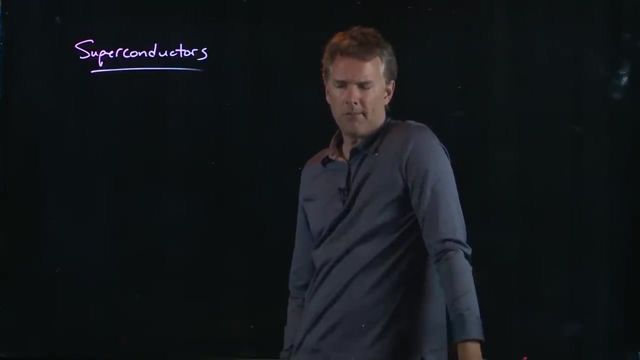 it's carrying a lot of current, which means it's going to have to be quite thick. Okay, has anybody ever heard of superconductors? Any of you guys ever heard of superconductors? You've probably heard that term in the news, right? Sometimes they talk about levitating. 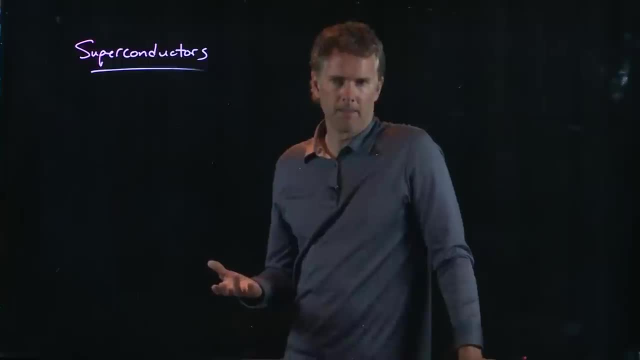 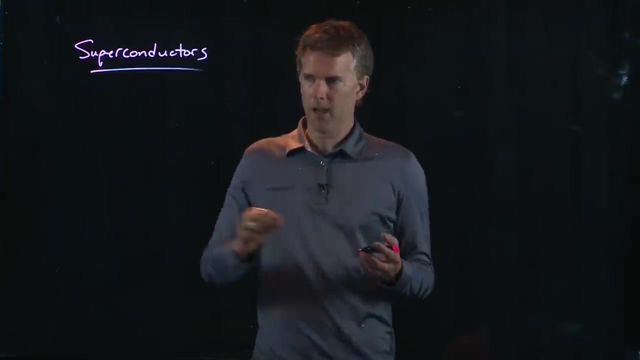 trains using superconductors in them. Okay, what is a superconductor? Anybody know What's the property of a superconductor? A superconductor is something that is super at conducting. okay, It's right there in the name. 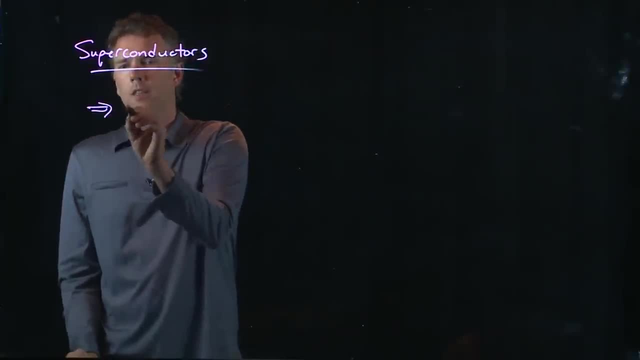 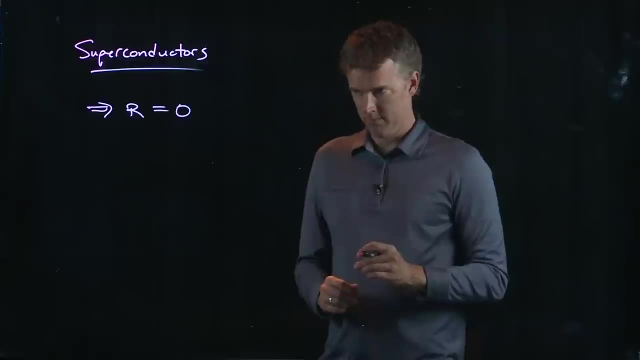 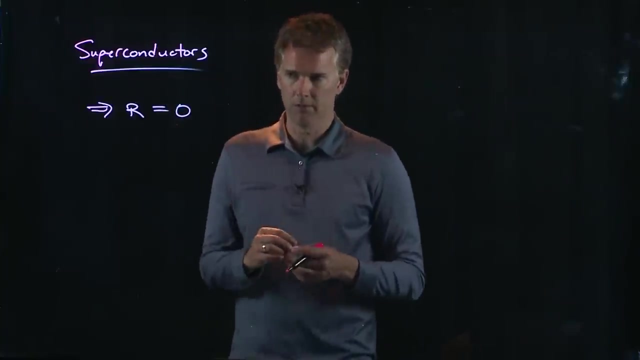 Okay, In fact, it's so super that R doesn't just go to something small, it in fact goes to zero. okay, And this is very interesting to people, right? Because if you have a resistance that goes to zero, you can run current through these wires and they don't heat up, right. 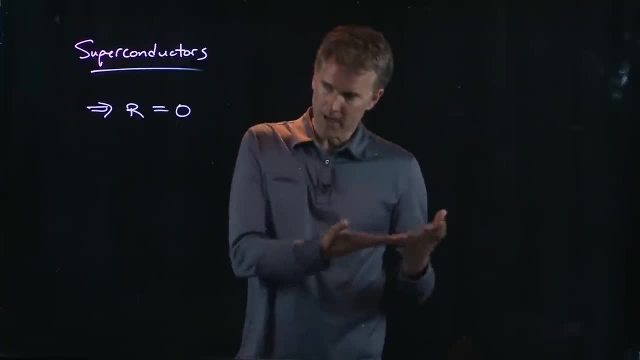 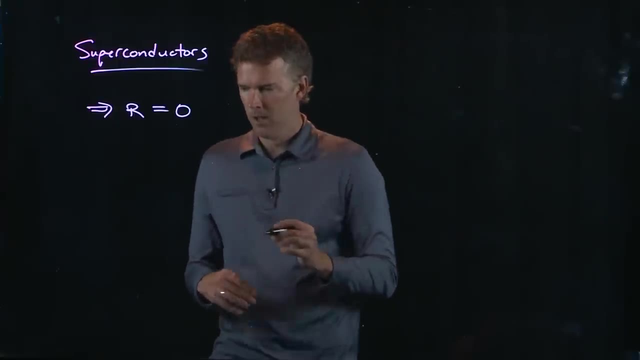 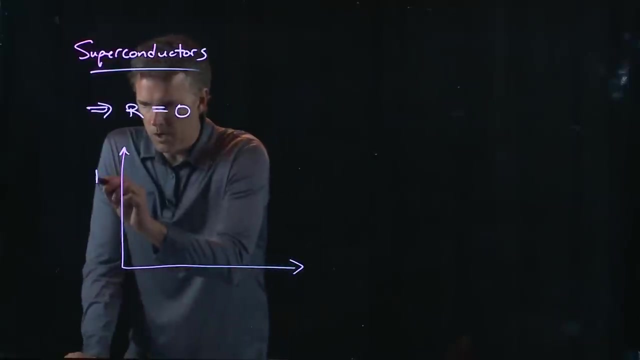 There's no resistance there. That water flowing down the river doesn't experience any rocks in the river and it just flows smoothly without any trouble at all. So if we think about our good old metals, what we said was a metal looks like this: 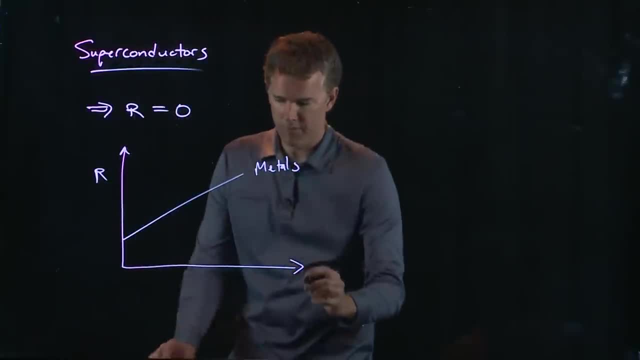 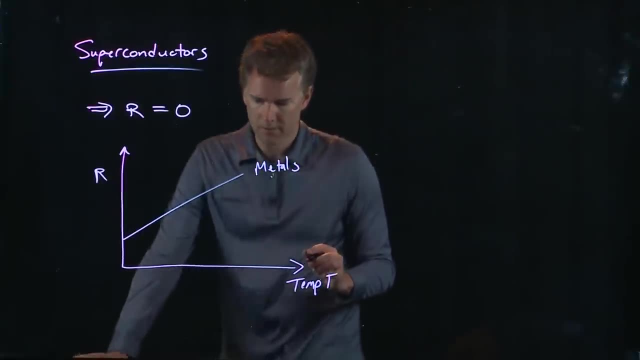 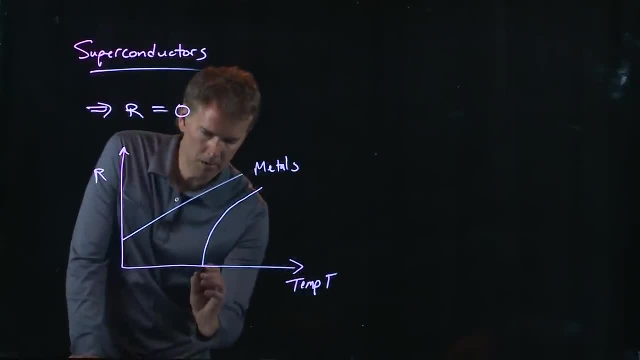 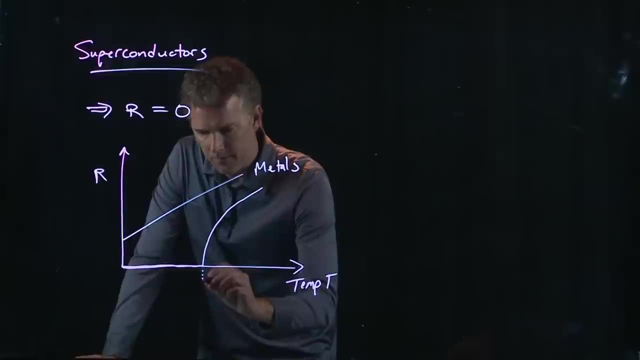 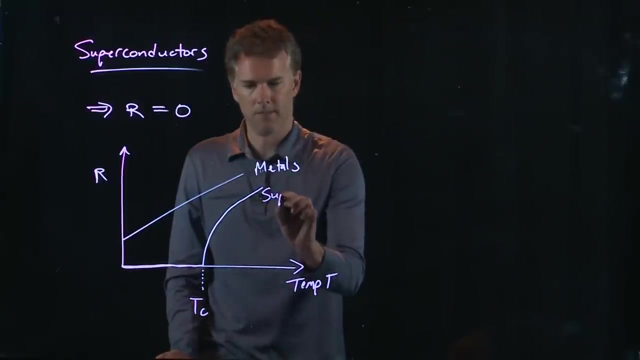 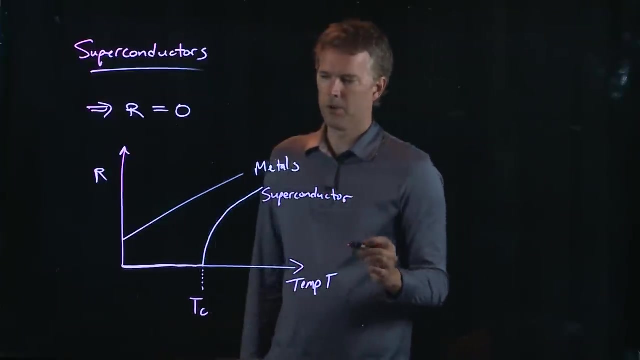 It quickly drops to a resistance of zero and then, from there on out, it has a resistance of zero all the way down This temperature. where it does. that is called the critical temperature. okay, Superconductor drops to zero at some temperature that is not at absolute zero. 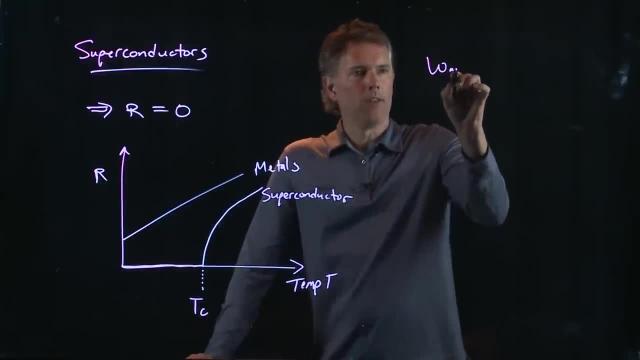 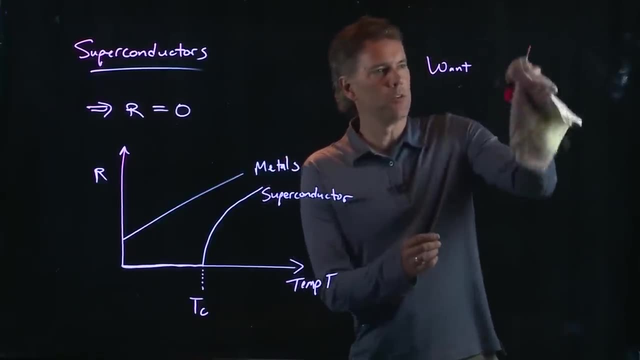 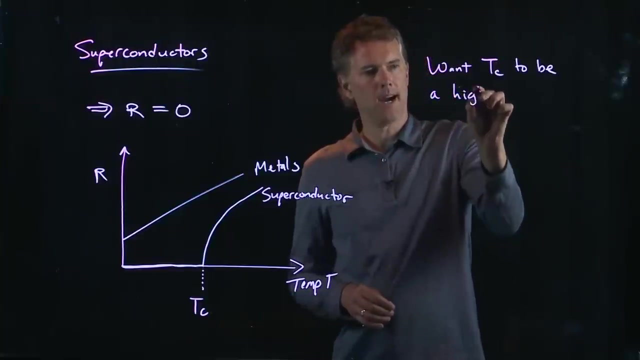 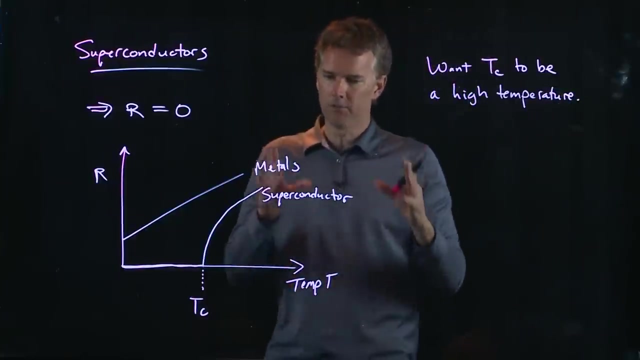 So the goal of superconductors is to find a temperature that is reasonable. You want that to be a high temperature, And this is where all the research in superconducting materials has gone into. How do we push that temperature higher and higher? 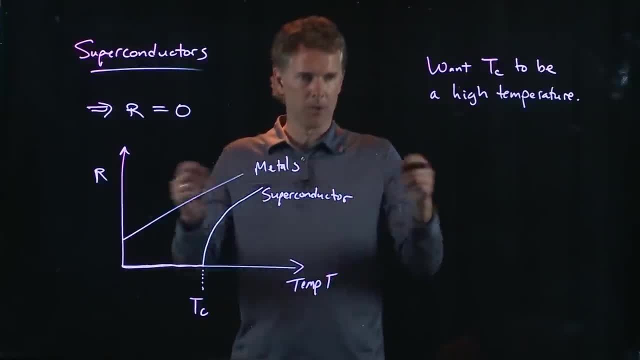 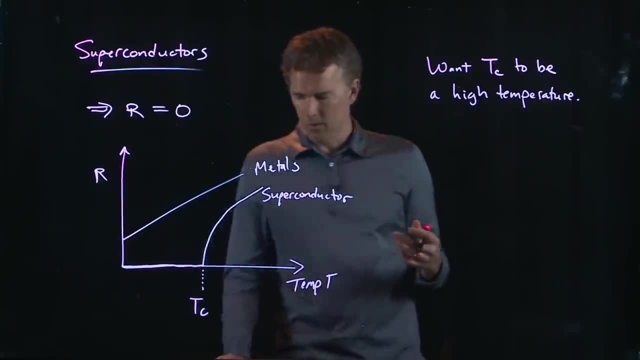 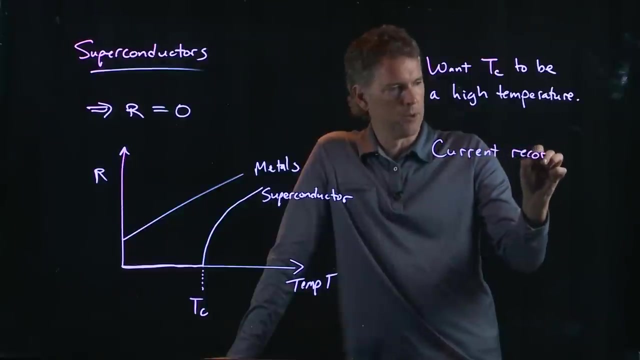 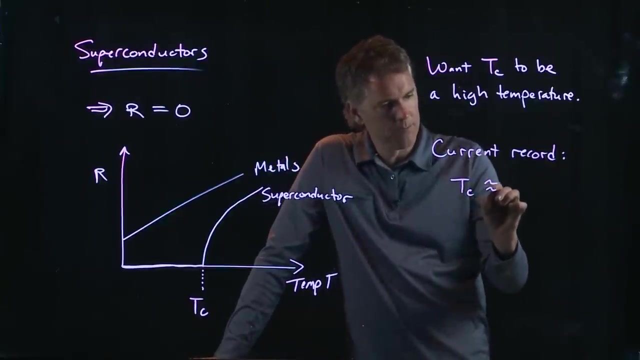 You want your metal wire to be able to operate at room temperature, or at least something remotely close to that. So where are they now? The current record, at least of a couple of years ago. you can double check me on this. maybe they're up a little bit higher now, but the current record is about 125 degrees.